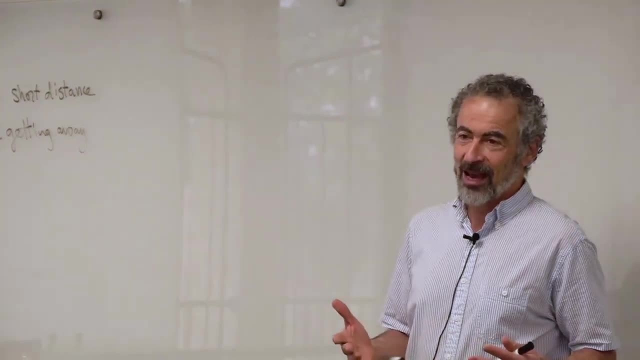 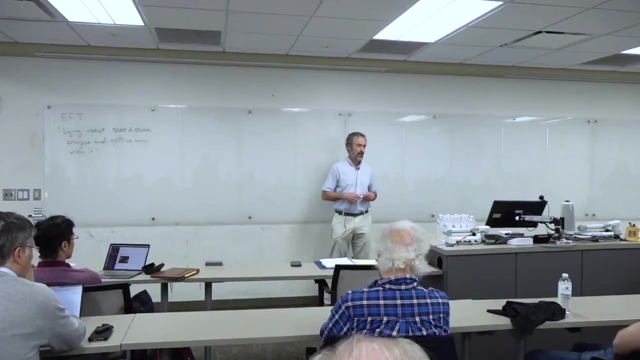 where the accelerators can reach have any reality to them. And in fact, the interesting thing is, you can change your description of short distance physics and the long distance physics will still be the same. So a lot of the problems that Dirac saw in QED are probably fictitious, because they have to do with this incorrect. 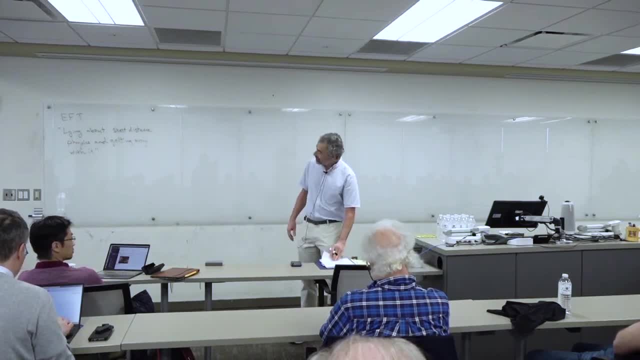 theory of short distance physics. But effective field theory is a lot more than that. It's an extremely useful tool and it becomes sort of a way of thinking that affects how one does physics in almost any field. You'll find that these techniques now are used in things as far away from quantum field. 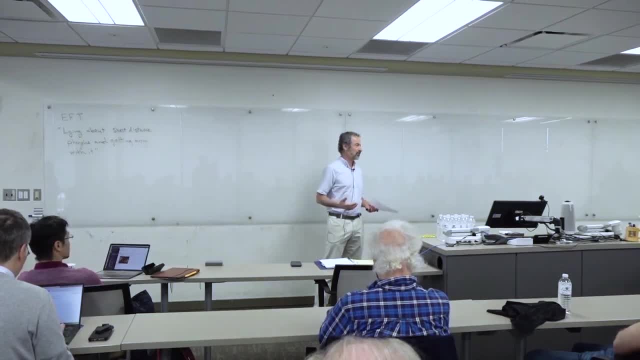 theory as the classical in-spiraling of black holes and the production of gravitational radiation, or the discussion of high energy collisions, when particles are going very fast but are collinear. That's a different type of effective field theory, And so basically, it's being used wherever there is a big hierarchy of scales and it's an extremely powerful and 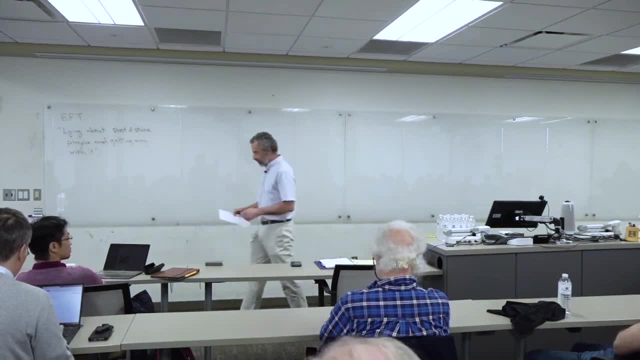 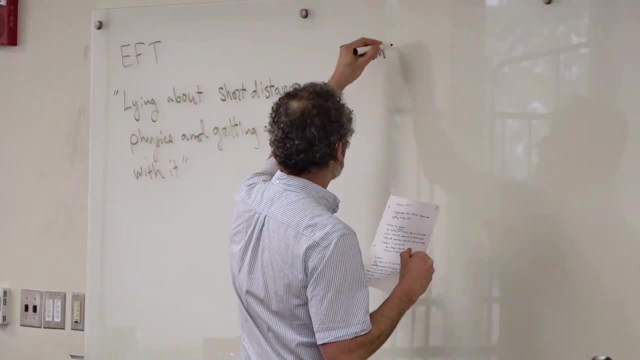 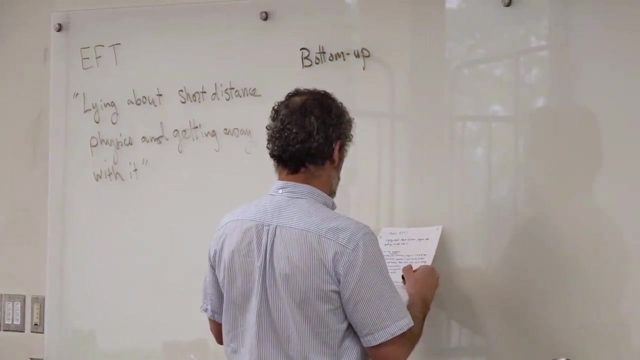 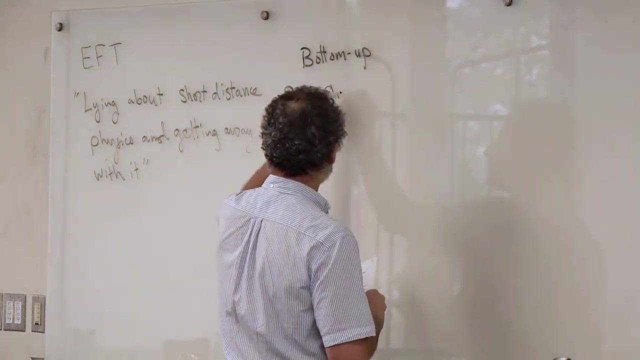 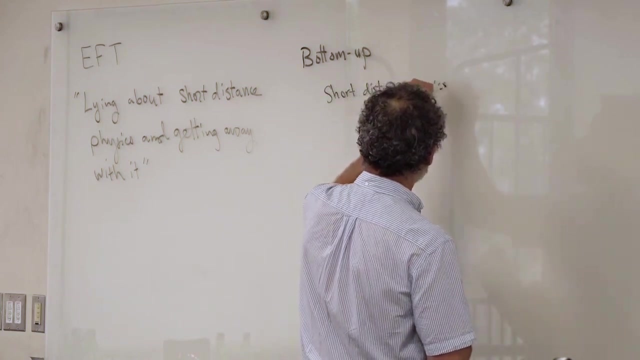 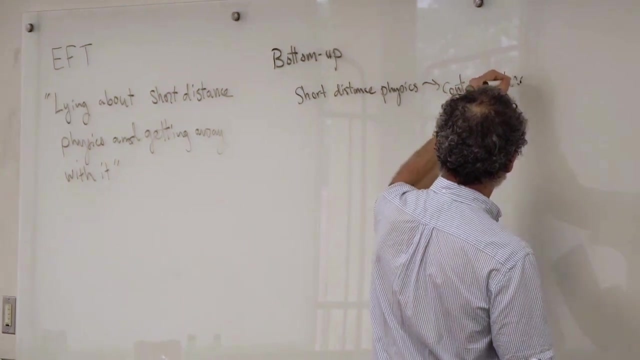 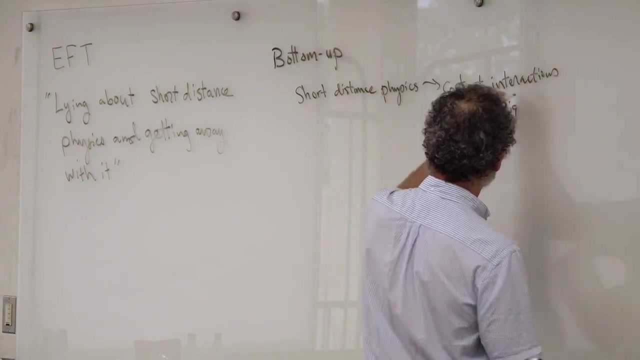 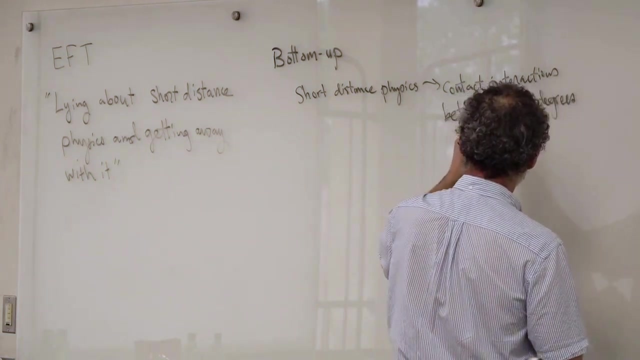 pretty simple idea to apply. So there are sort of two different uses of effective field theory. One is the bottom up approach, So you describe all possible short distance physics in terms of contact interactions. So it gets reduced to contact interactions between light degrees of freedom. 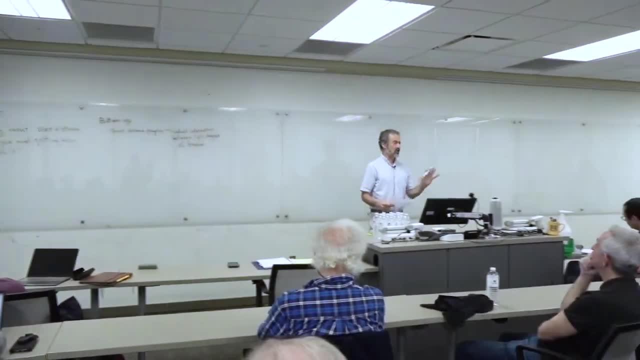 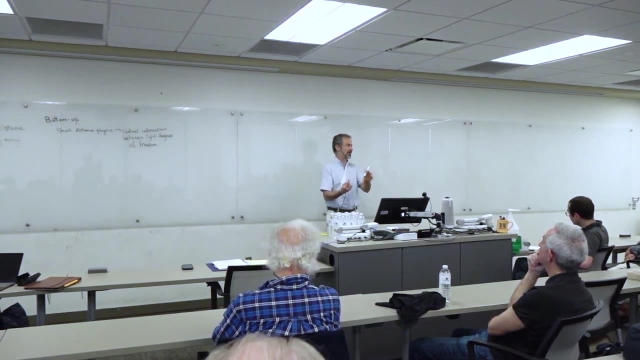 So you don't have to know what's going on. in short distance, You replace everything with delta functions. The low energy particles get close together. I don't know what's going on there. I'll approximate that they are sitting on top of each other. 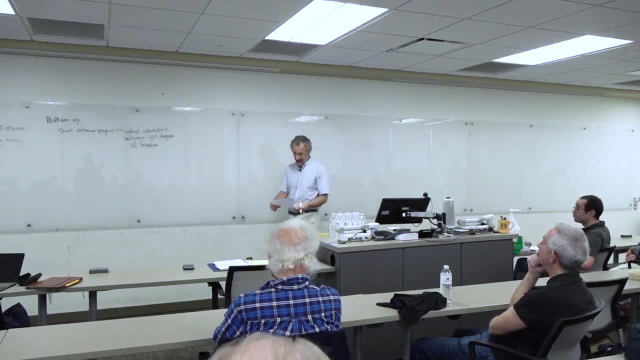 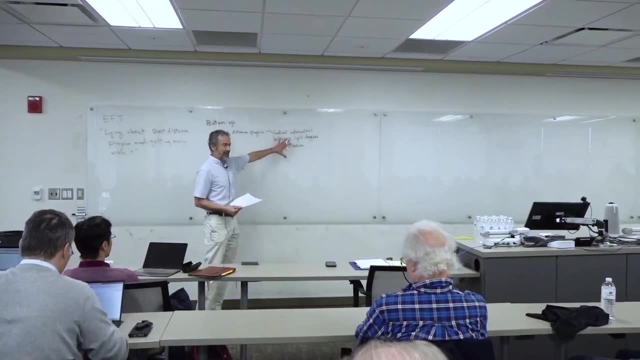 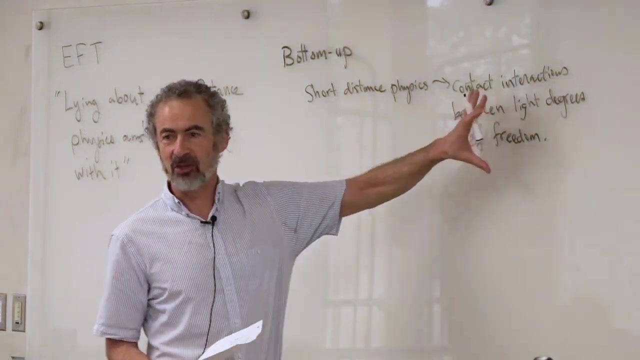 Something happens and they bounce off. So the reason why this is so powerful is because we know something about the light degrees of freedom, We know the symmetries that control the theory, And so we can write down a limited number of ways that they could interact at short distance. 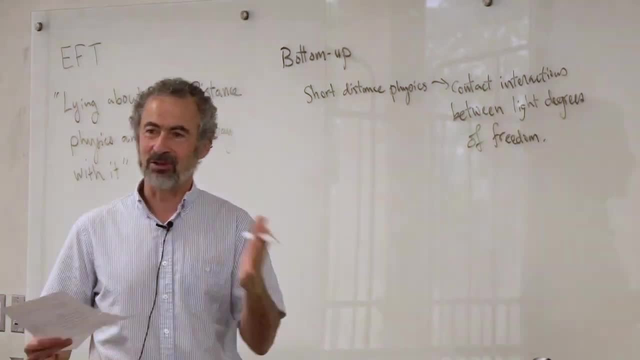 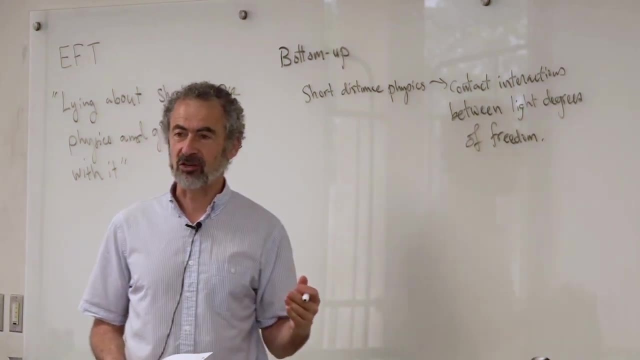 And each will come along with an unknown coefficient, how strong that interaction is. And then we can go and we can study experimentally and figure out what those constants are numerically- Maybe they're 0. And then try to figure out what the short distance physics is. 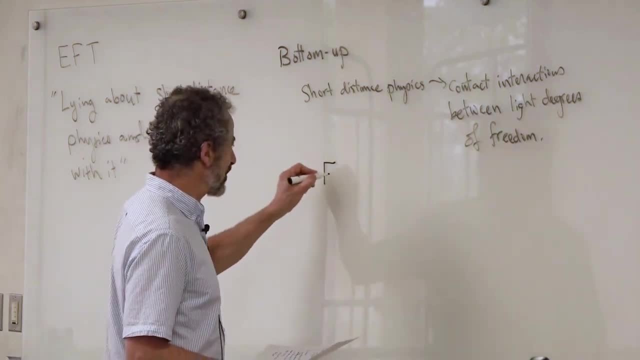 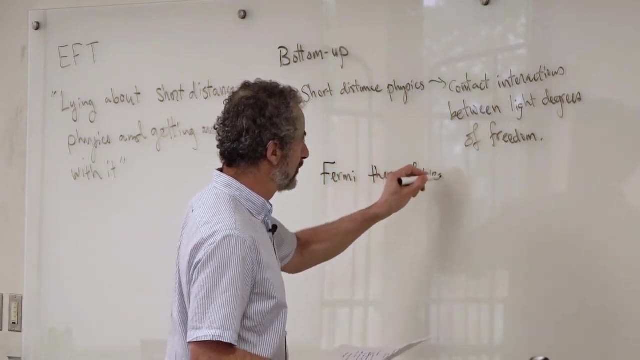 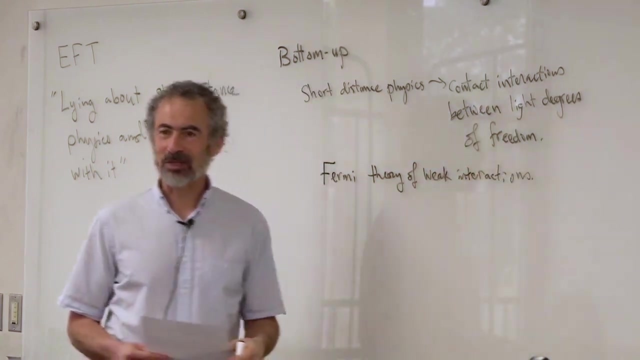 based on that, And so the quintessential application of this is Fermi's theory of weak interactions. He was an unusual fellow in that he was a great theorist and a great experimentalist, And I don't think the world's seen anything like that. 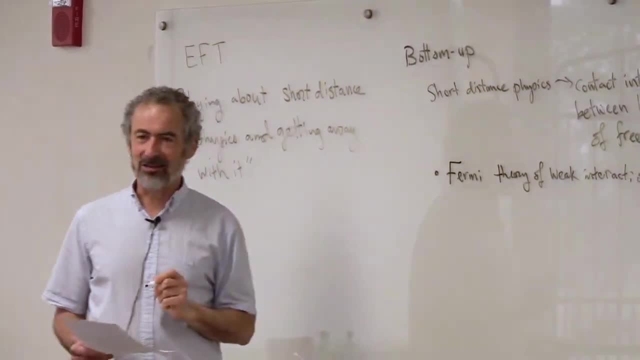 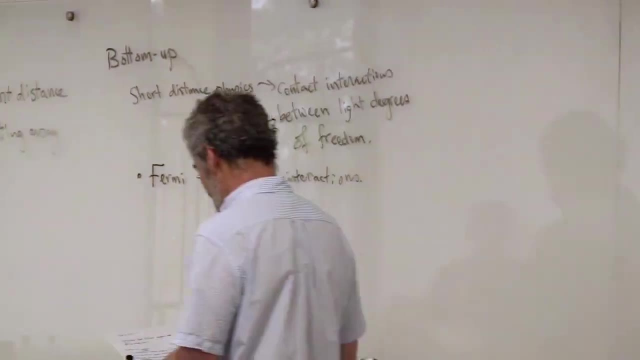 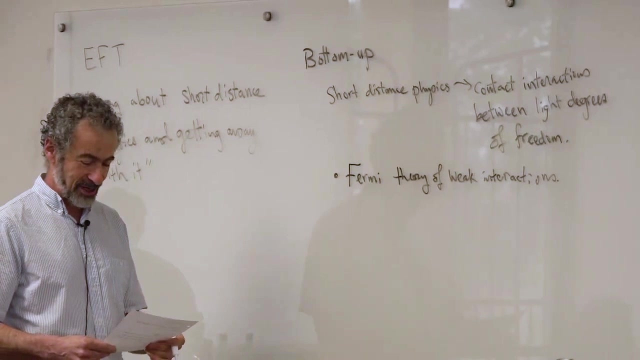 since then. So he didn't let problems of infinities get in the way of trying to describe the physics he was actually seeing, And in particular he was looking at the weak decay of the neutron into a proton and an electron and wanted to understand that. 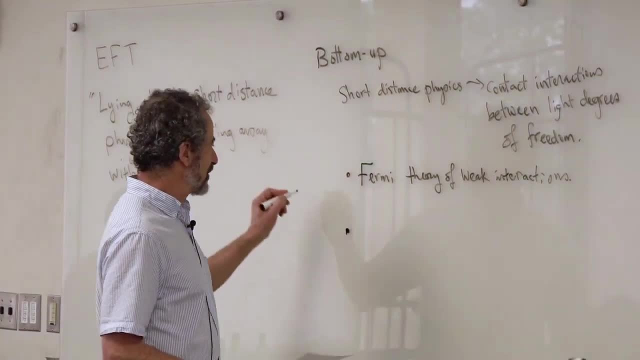 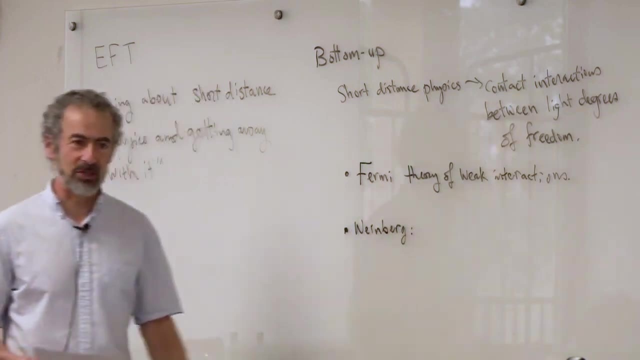 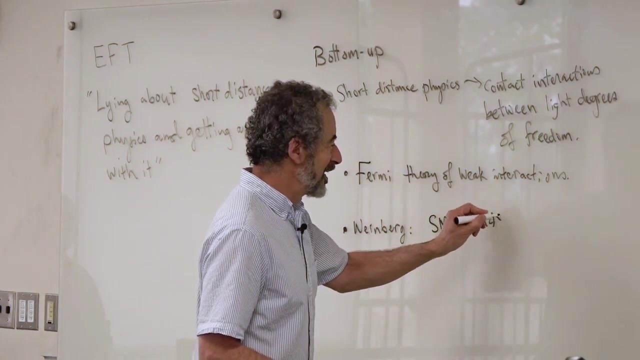 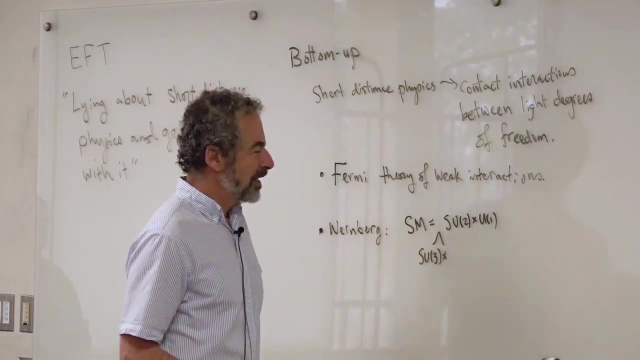 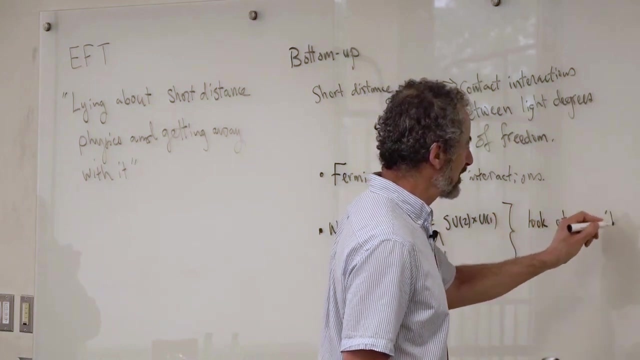 We'll talk more about that. And then another use of effective field theory, pioneered by Weinberg mostly, was to take the standard model, which is in particular the SU cross U1 part of it. Well, I should put the color there too And look at possible extensions, not by trying. 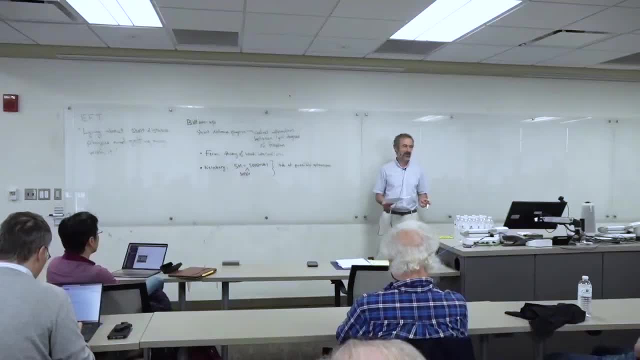 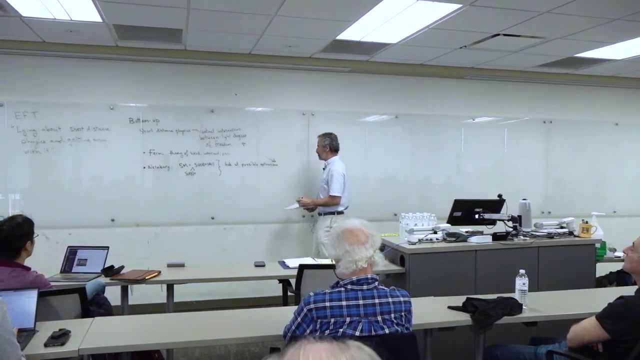 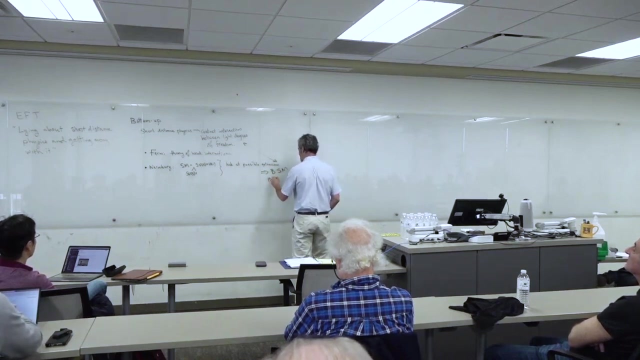 to guess a theory of everything, which is another activity people do, but rather to look at all possible contact interactions arranged in a hierarchy of importance and use that to gain information about physics beyond the standard model, normally abbreviated as that. Another application is what I'll call top-down. 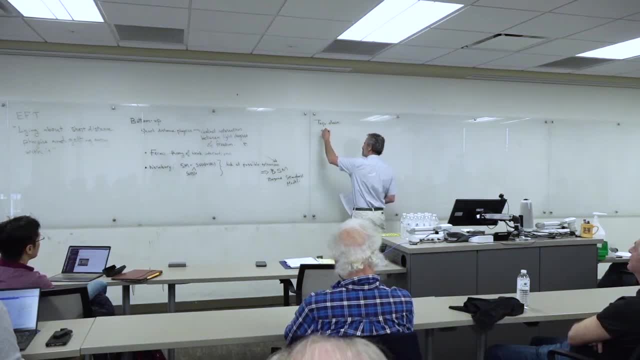 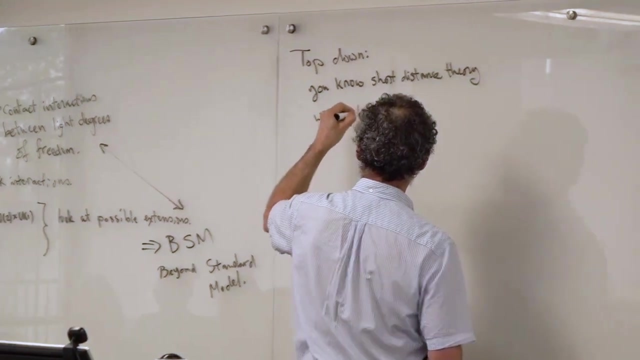 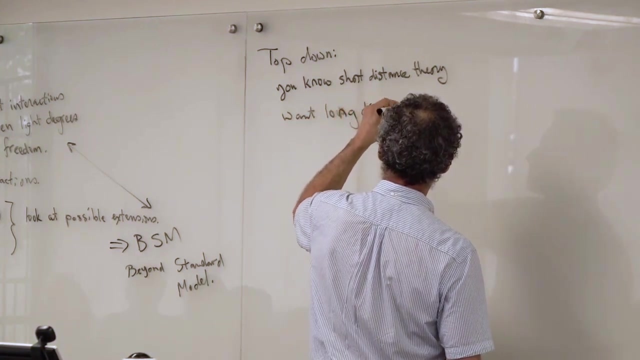 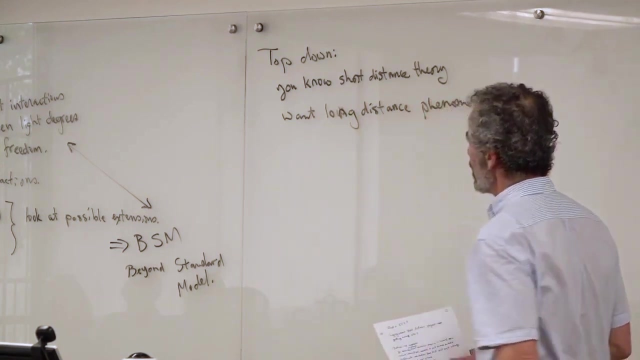 where you know there's short-distance physics And you want long-distance phenomenology, And you want low-energy phenomenology, or I say long-distance phenomenology. So in this case, what you do is you take the DOM, you take the criterion. 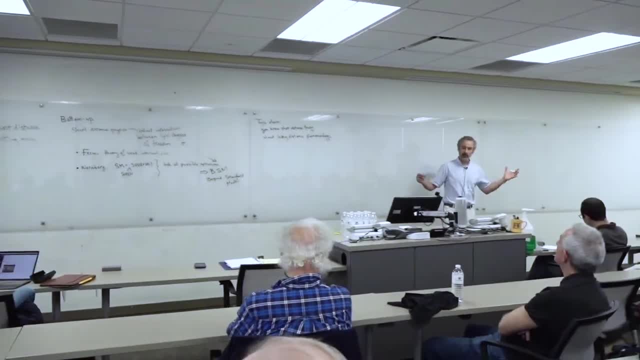 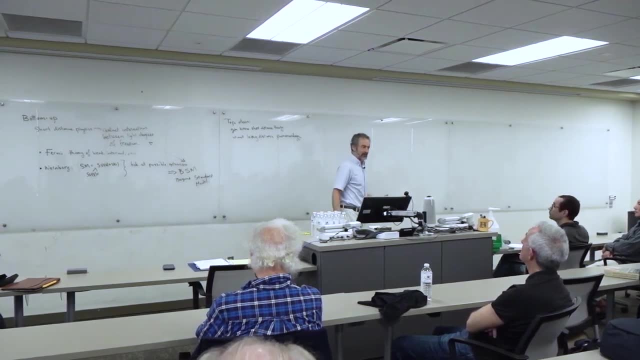 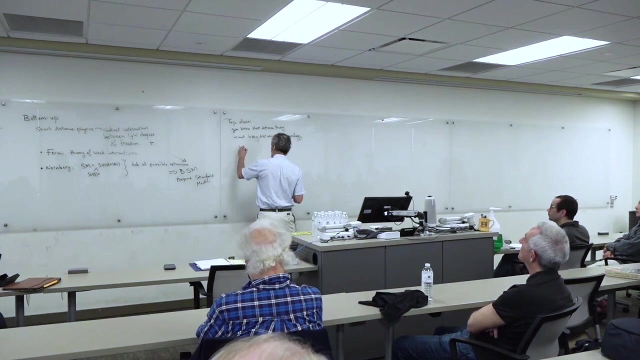 take the long distance physics, which may be very complex, and you reduce it to a few contact interactions between the light degrees of freedom, which can greatly simplify your calculations. Examples of this, for example, are when you take the standard model and you 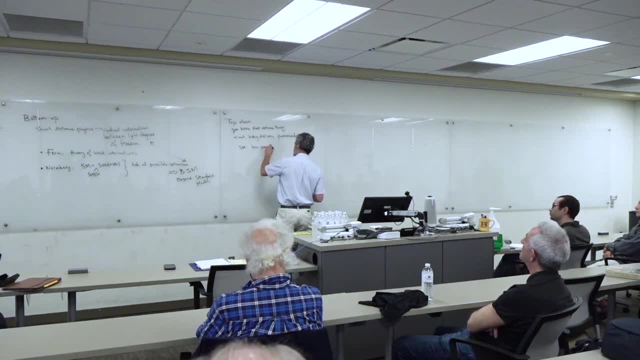 want the low energy flavor physics which you're going to hear more about in this series. It turns out that the effect of the strong interactions on the flavor physics can look very complicated but in an effective field theory way it becomes very clear how to sum. 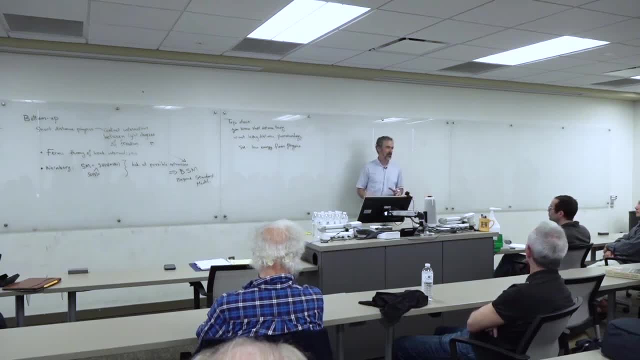 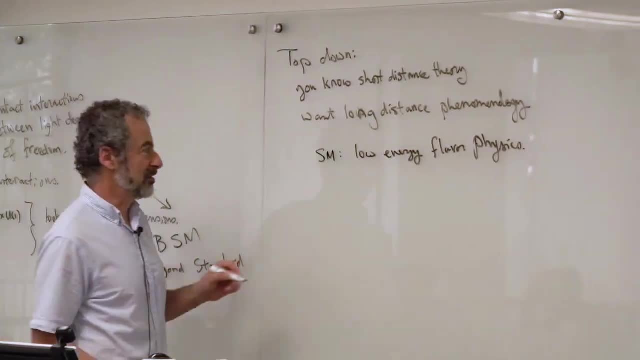 up the important stuff and ignore the less important stuff, So it's a very useful tool to make the problem tractable. This still involves perturbative QCD, but then another place where it's applied is non-perturbative QCD. 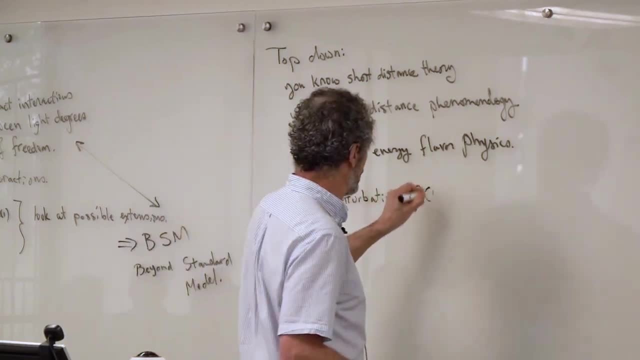 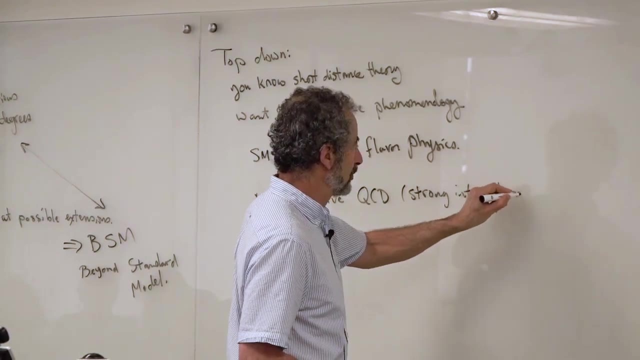 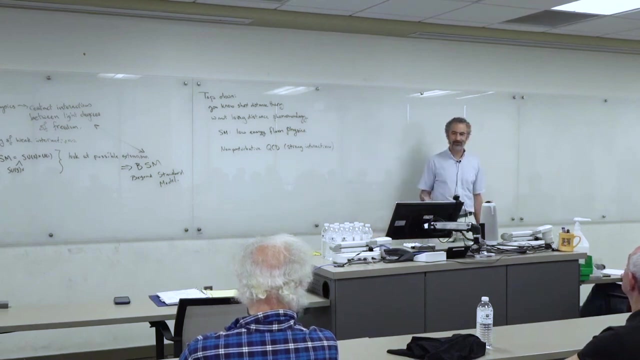 namely down at very low energy where it's strong. This is a theory where we know the theory. This is a case where we know the theory. We can write down the Lagrangian in a very short little expression, but we don't know how to compute with it because it's non-linear. 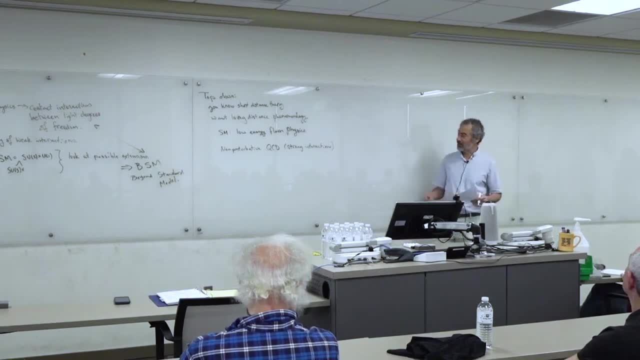 and it's very difficult to compute with the Lagrangian expression. So we're going to write down the Lagrangian expression. So we're going to write down the Lagrangian expression. It's got infrared divergences. It's very difficult, But the very low energy form of 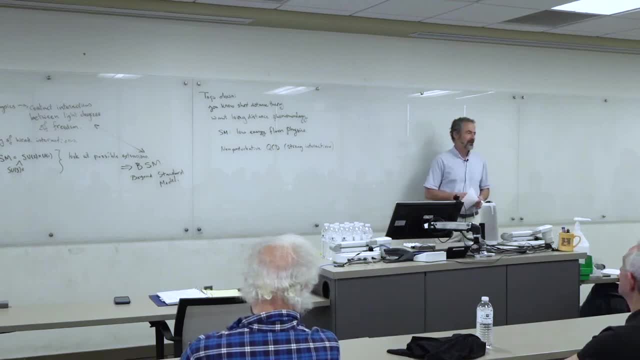 QCD is not that complicated. It involves mesons and nucleons, And so we can discuss the theory of mesons and nucleons, the low energy degrees of freedom constrained by the symmetries of QCD, but otherwise replacing all of that complex stuff of gluons and quark-anti-quark. 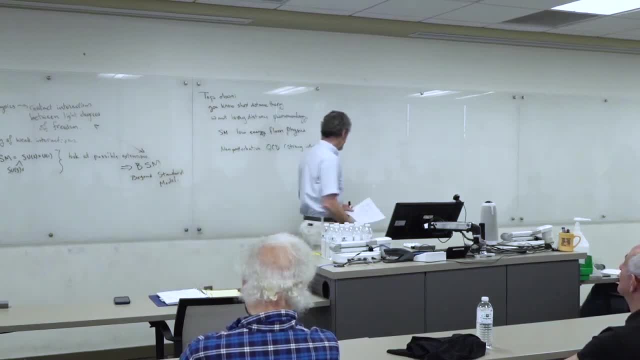 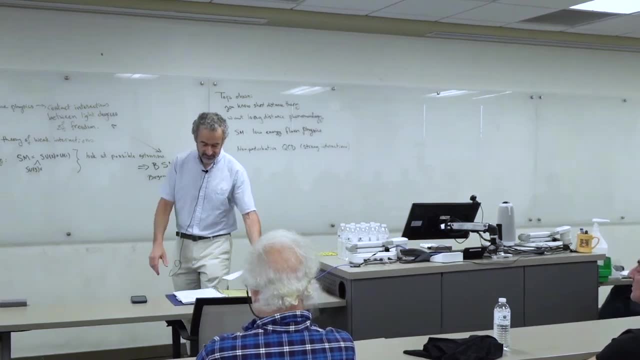 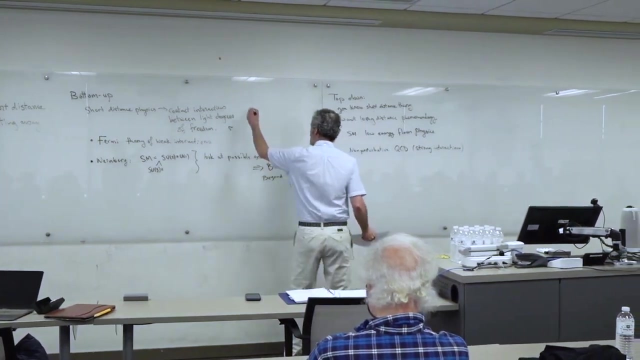 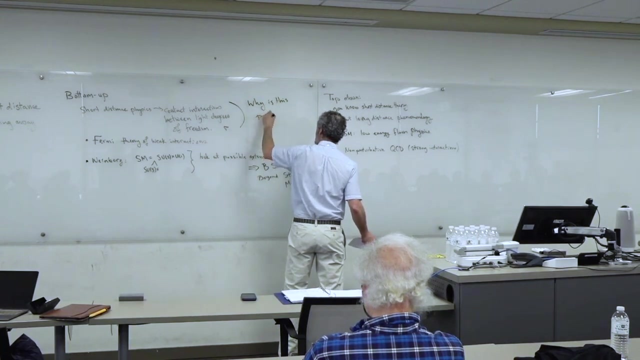 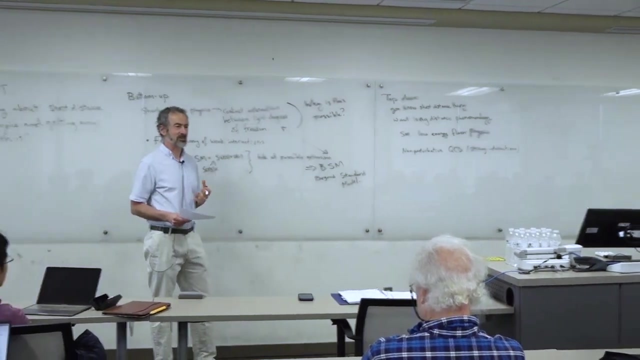 pairs with contact interactions, So that's another case where the top-down approach is very powerful. So why is this possible? There are some cases in physics where there is no separation of scales. I think the most famous one is turbulence, where the long-distance behavior depends on. 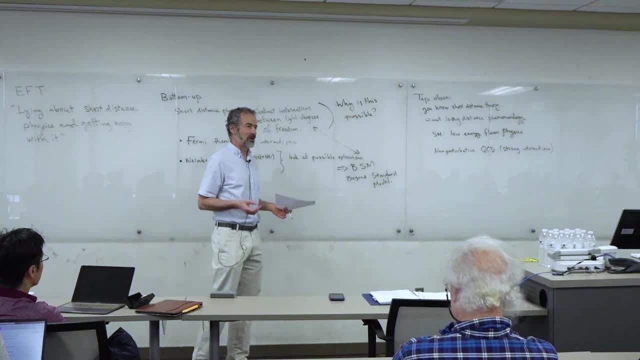 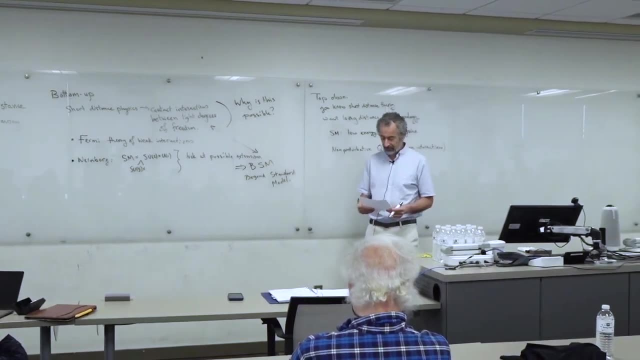 what's going on at short distance. But it's not always the case. It's not always the case And that makes it an extraordinarily hard problem to understand. But luckily most aspects of quantum mechanics, you don't have to deal with that. 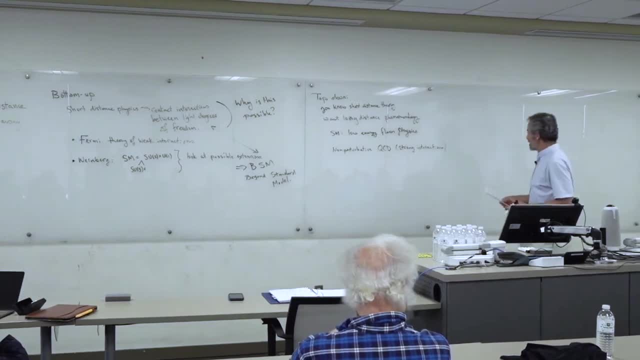 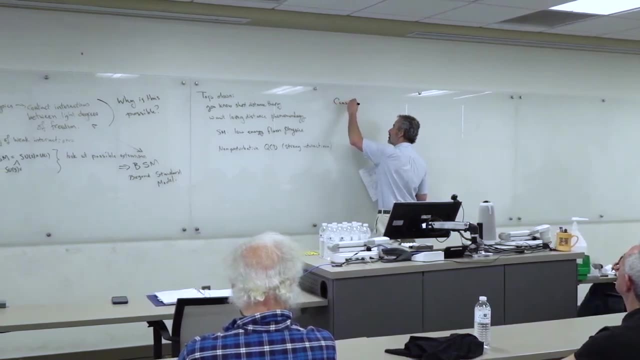 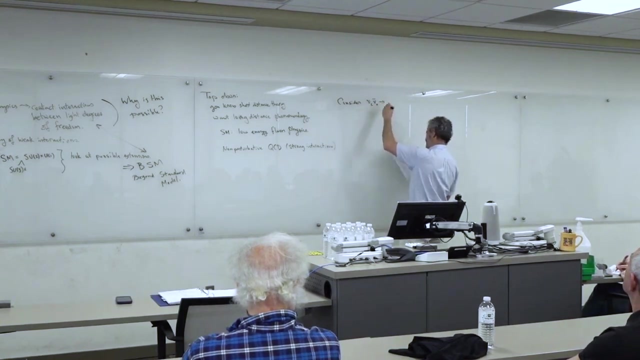 So, at a very basic level, what we're talking about is a Taylor expansion. We're going to go well beyond that. But let's consider. I chose a hypothetical experiment which is very difficult to do experimentally, Namely scattering of two neutrinos off each other. I choose this because it's simple. 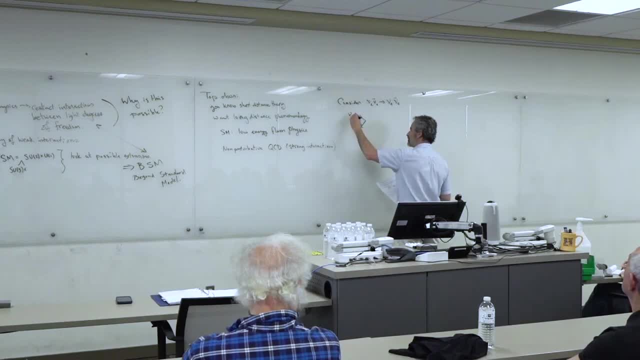 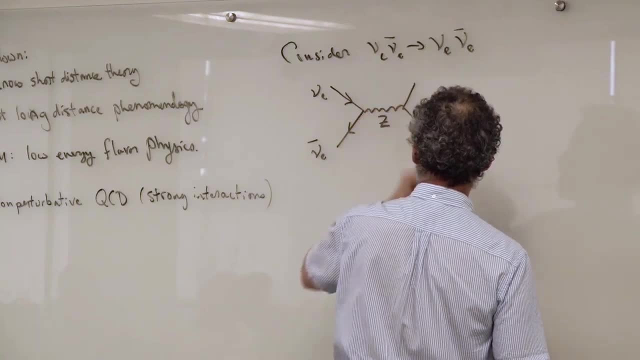 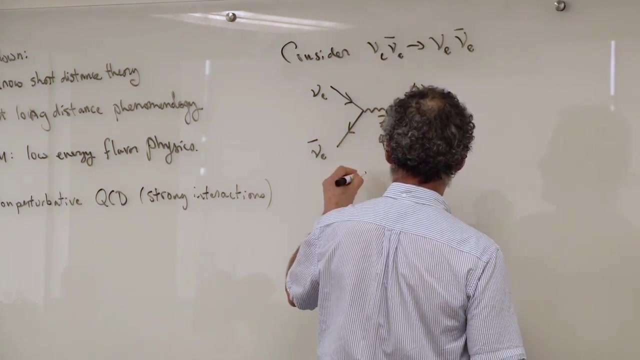 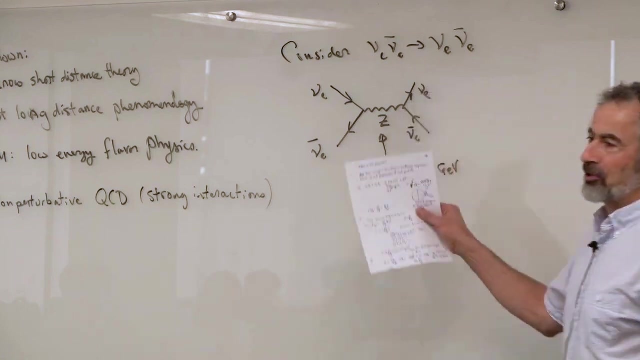 There are not many ways they can scatter And in the standard model the primary way they'll scatter is through a Z boson And this has a mass of about 90 GeV And we're going to do that. But I might be interested in neutrino scattering in an astrophysical 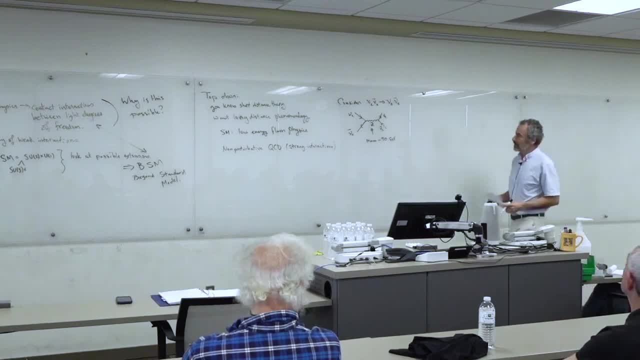 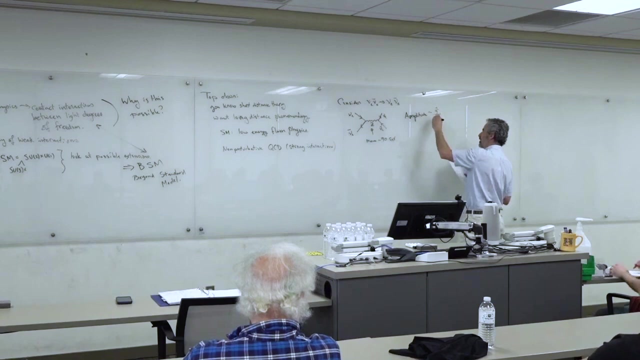 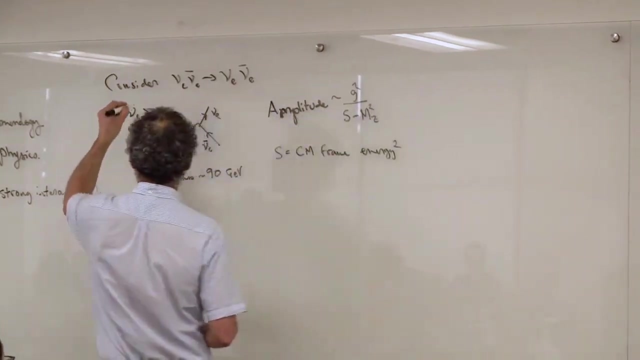 context where the energies are MeV. Well, if I look at the scattering amplitude, I'm going to get something that looks like G squared over S minus Mz squared, where S equals the center of mass energy, Frame energy squared. So, in other words, if I have E over 2 and P coming in and on, 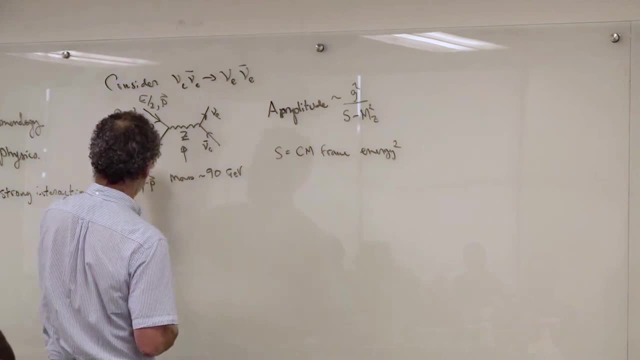 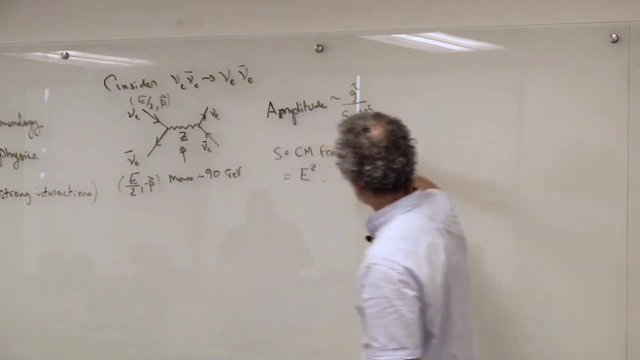 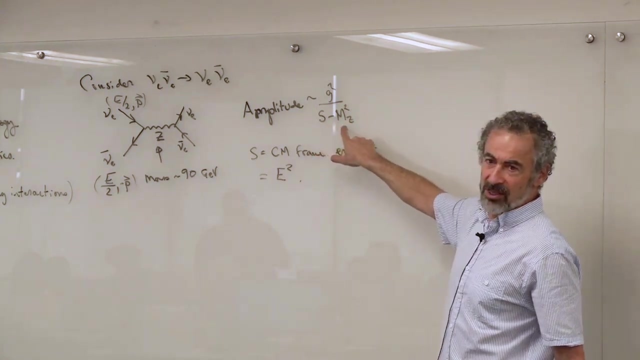 this one, I have E over 2 and minus P, then this would just be E squared. And so what this tells you is that this is the propagator for the Z. When S is near Mz, I get a big amplitude. That's because I've created a real z that can wander around the universe for. 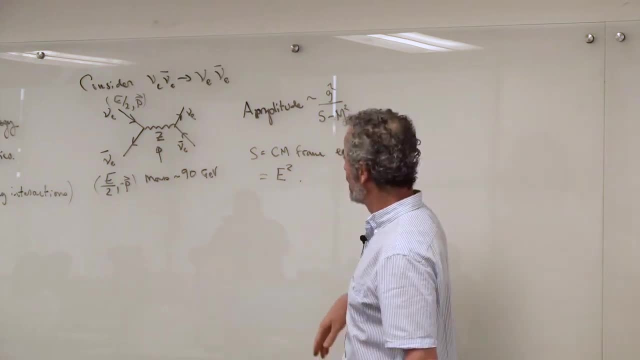 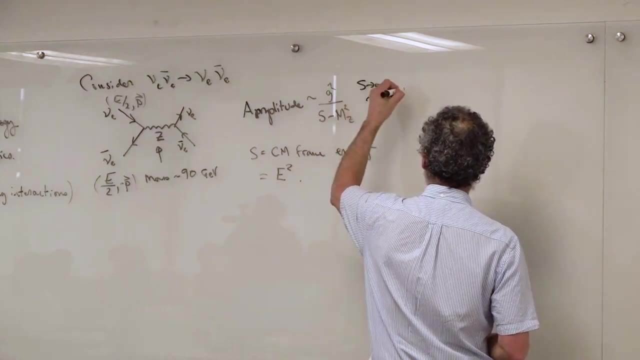 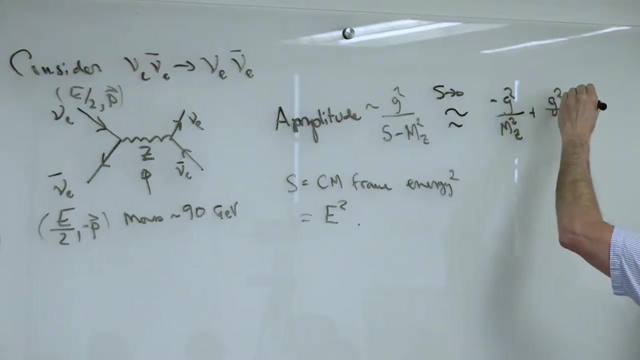 a long time before it decays into a neutrino-anti-neutrino pair, But at very low energy. so as s goes to zero, this is just minus g squared over mz squared, Or, if I want a little bit more accuracy, I plus g squared over times s over mz to the fourth. And this is possible because 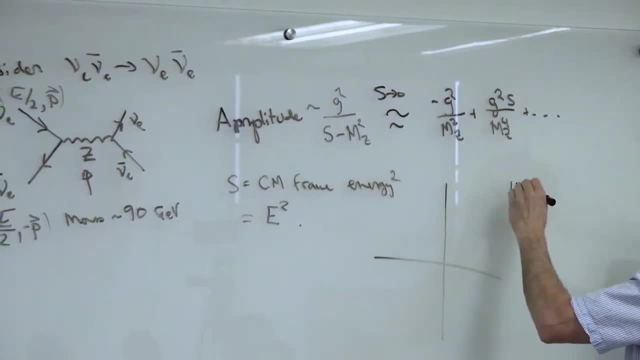 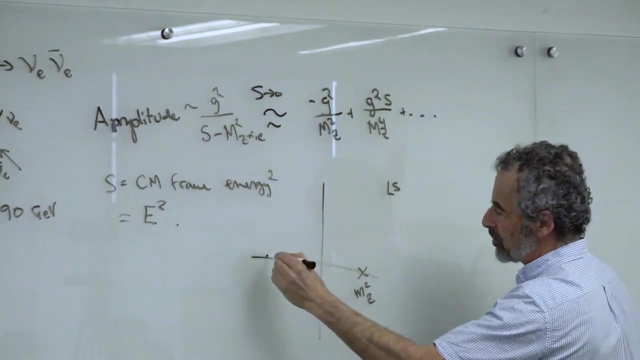 if I look at this amplitude sort of trivial here in the complex plane. there's a pole here at mz squared And I'll get it off the real axis typically. so it's a little bit below the real axis, But you know from complex analysis that I can then do a Taylor expansion. 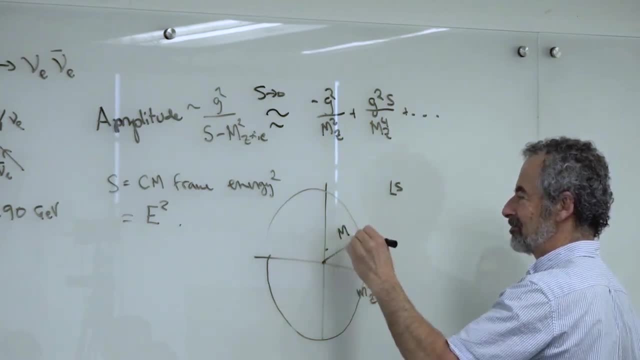 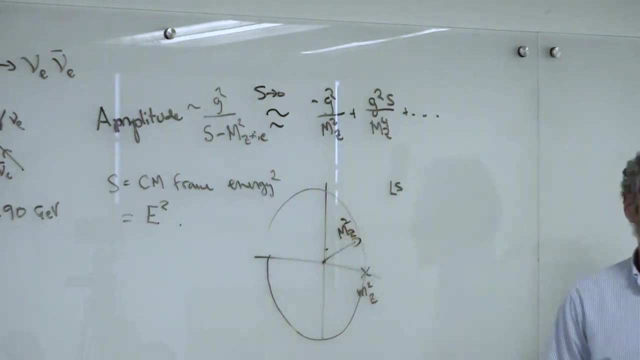 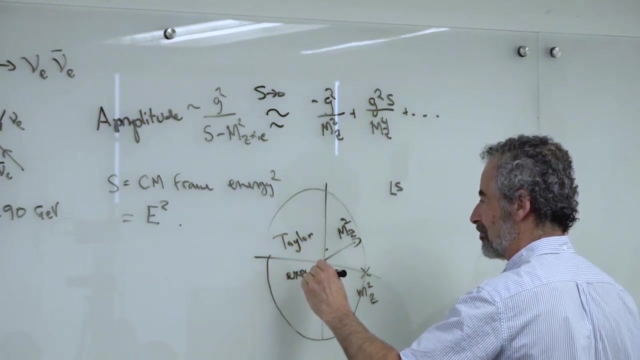 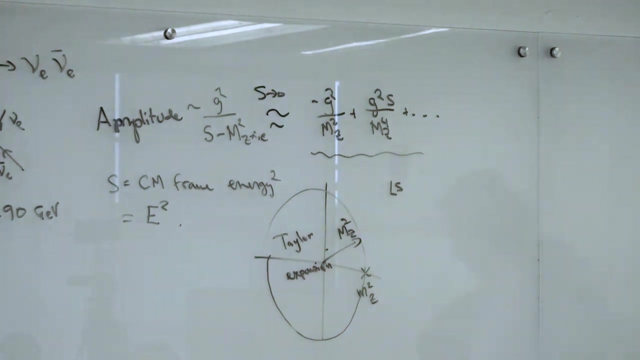 around here with the radius of convergence of. I guess this is squared. So as long as you're in this region here you can do a Taylor expansion, no problem, And so this expansion is good. Now what happens if I go to slightly higher order in quantum? 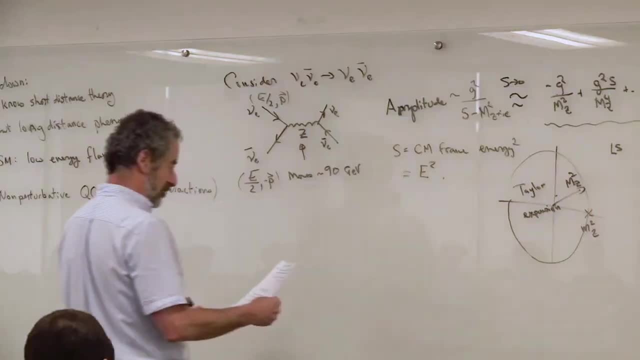 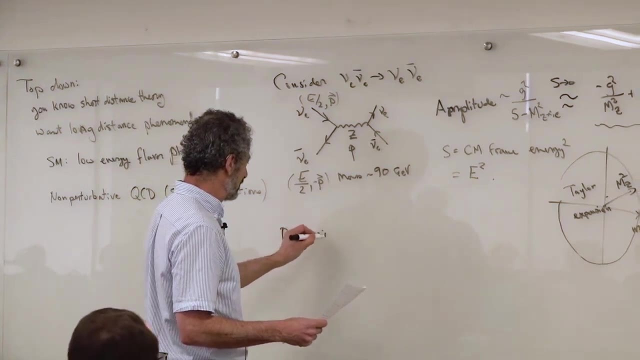 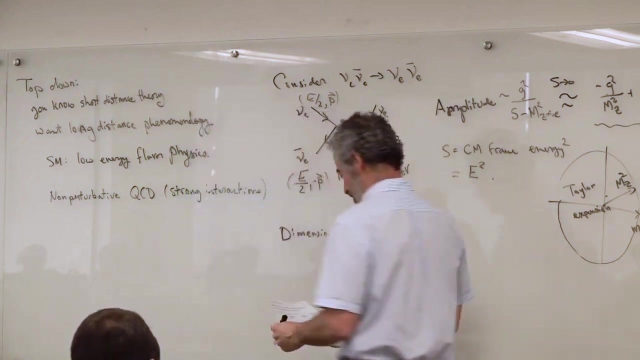 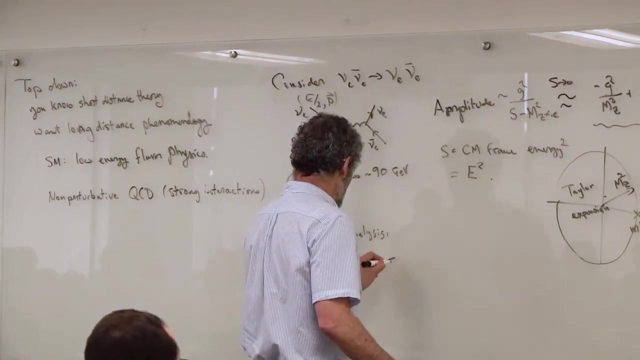 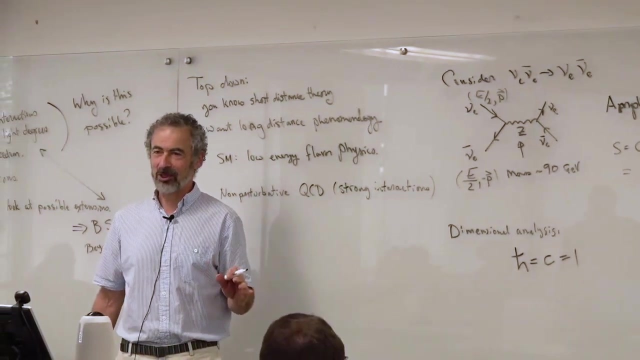 effects. Well, before I do that, what I want to do is mention some dimensional analysis. So we've got that. So some dimensional analysis says that H bar equals, c equals one. You can tell what sort of physics people do by what they set to one. If you're doing non relativistic, 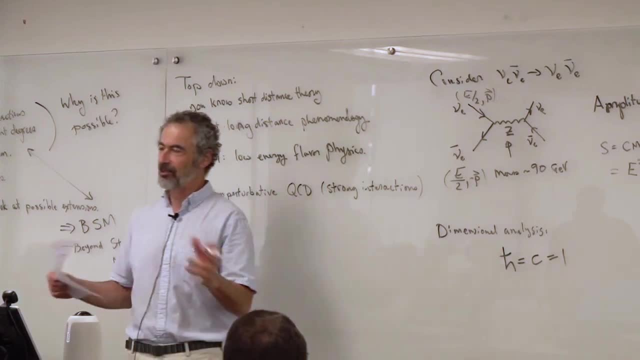 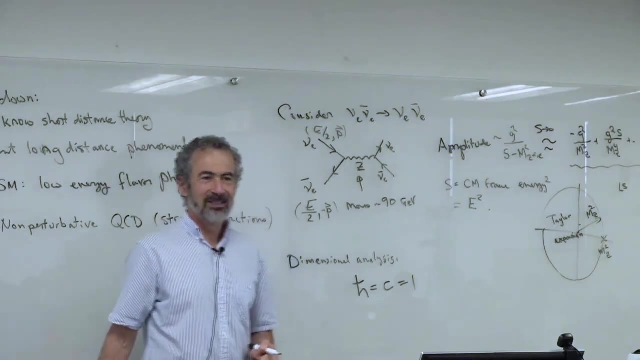 physics, it's usually not convenient to set c to one. If you're doing classical physics, like soft condensed matter, polymer foldering, where quantum mechanics doesn't play a big role, You don't want to set h to 1. If you're a, 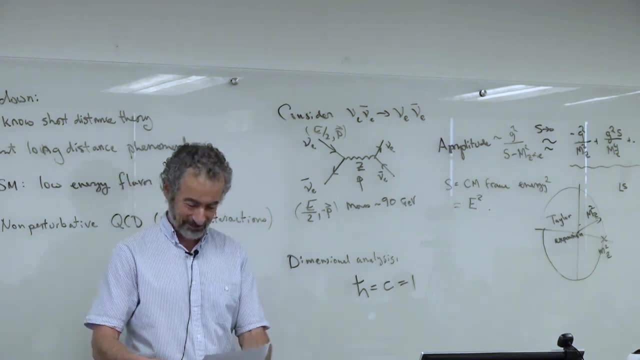 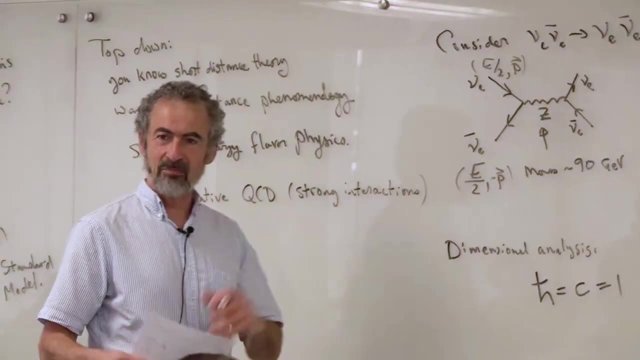 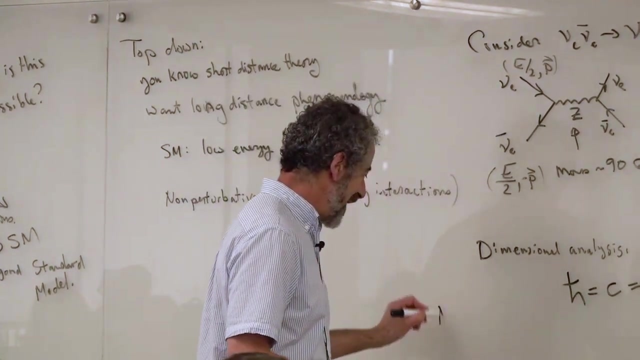 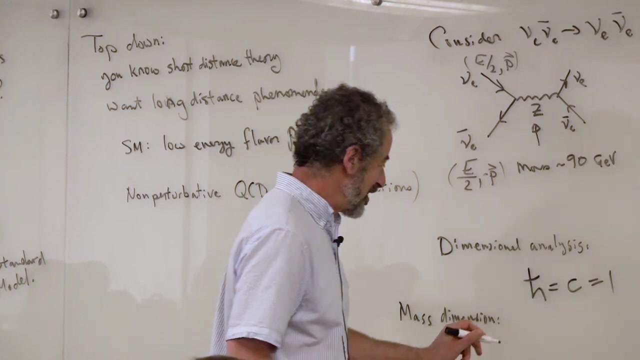 string theorist, you set everything in the world to 1 and claimed you've solved everything. So when you do this, then you find that length and mass are related in dimension. So I'm going to talk about mass dimension And I'm going to use this notation, which I don't. 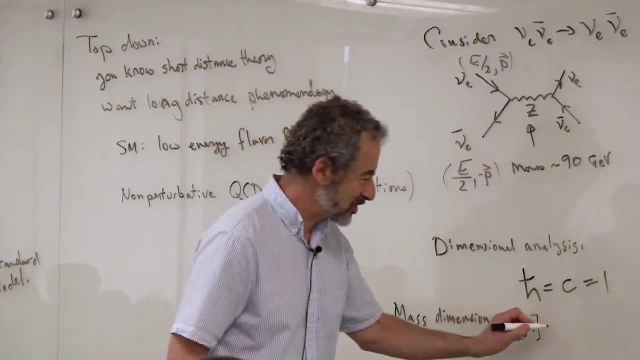 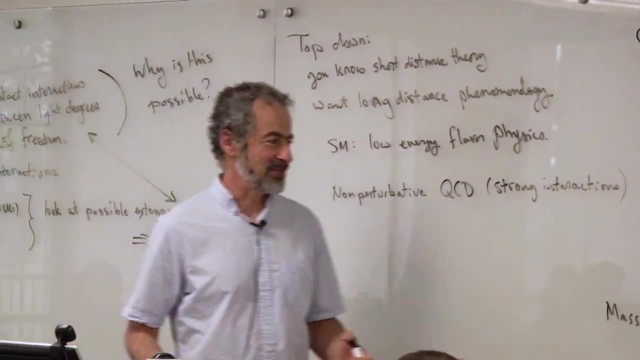 know how widespread it is. I'm going to say that the dimension of m is 1. That is mass dimension, 1. It comes in units of mass or, if you want, energy. So I might say a particle has mass GeV, But so do a whole bunch of other things, Energy. 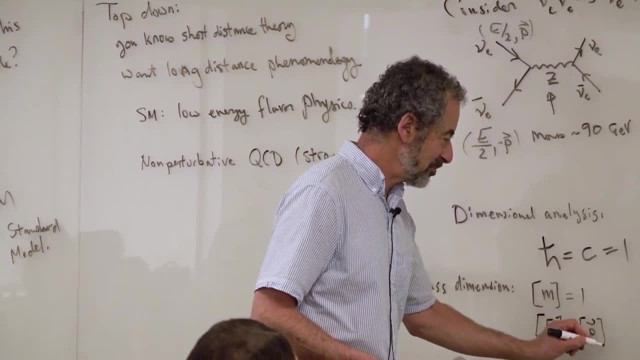 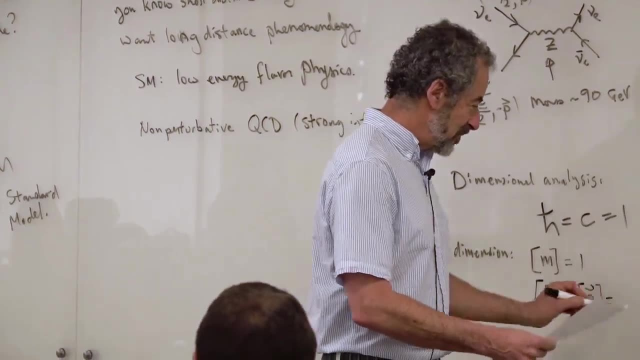 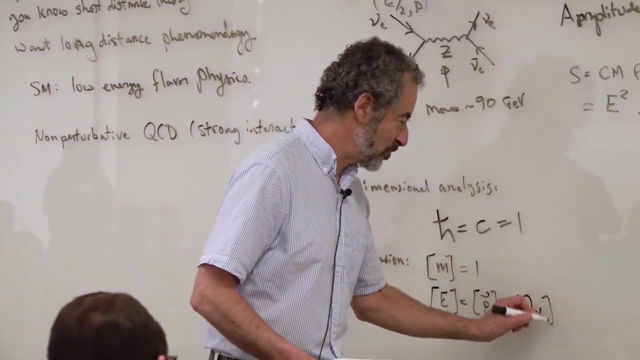 does have mass And momentum has the same, because mass times, velocity and velocity is set to 1.. Or it's in units of c. But also we know from de Broglie that p and 1 over x have the same dimension. So d by dx has dimension 1.. They all have mass dimension 1. While x and 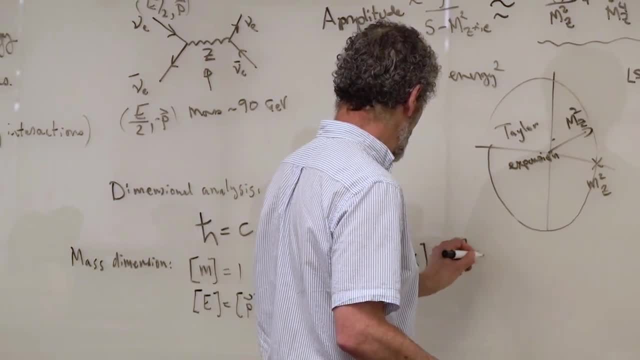 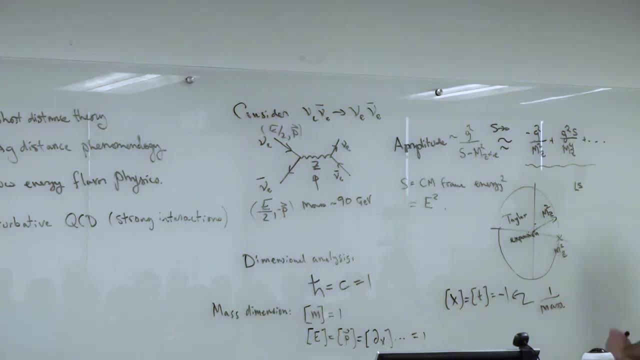 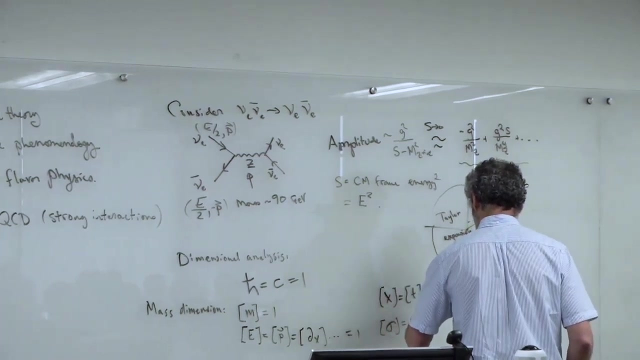 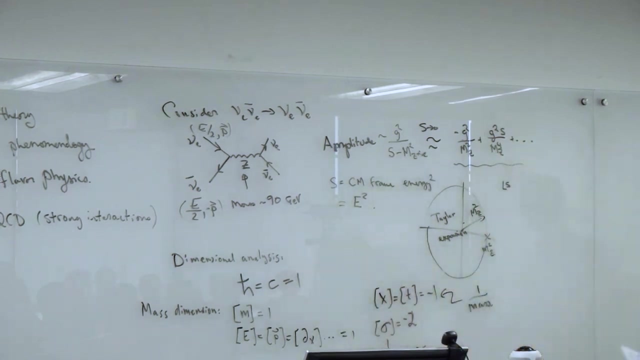 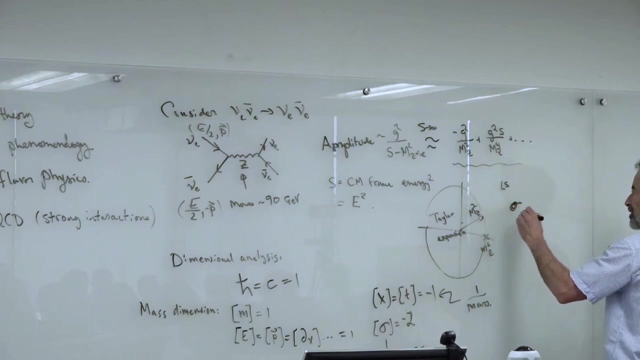 t have dimension minus 1, 1 over mass And a cross section which is an area, therefore is minus 2.. So if you want to study, the cross section for new new bar goes to new, new bar And you just take this leading term here. 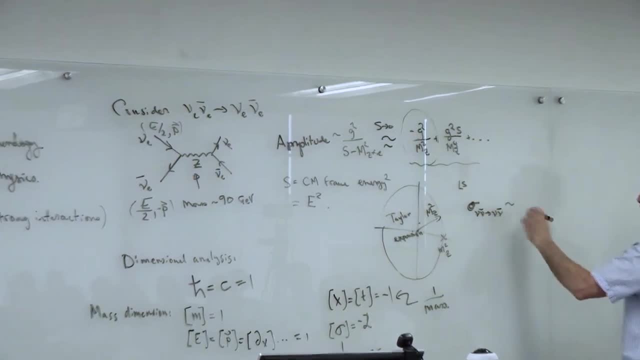 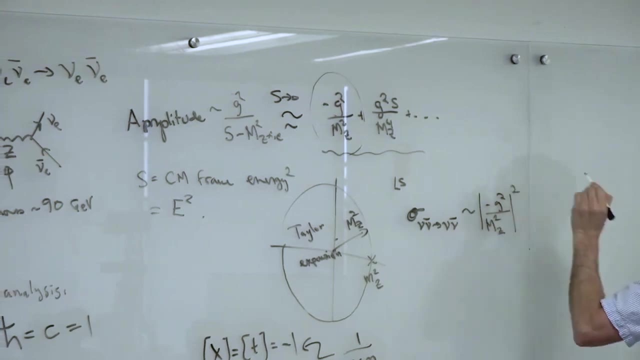 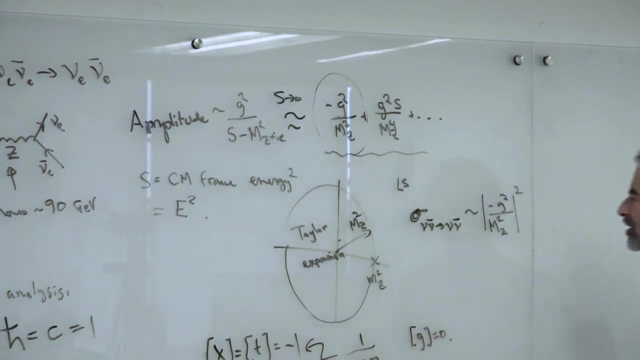 well, we know that this goes like the amplitude squared, So I'm going to approximate it with that leading term, Okay, oh, and I have to tell you that gauge couplings are dimensionless, So this goes like 1 over m to the fourth. but I just told you that the cross section 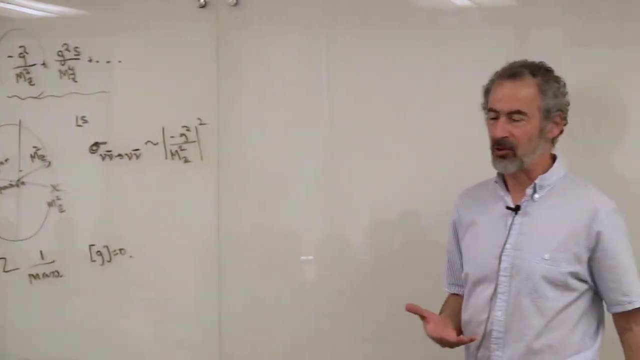 has to go like 1 over m squared, So something has to come in to give you another mass squared upstairs And that will come from the phase space integral when you multiply that by the mass squared. So I'm going to approximate it with that leading term And I have to tell. 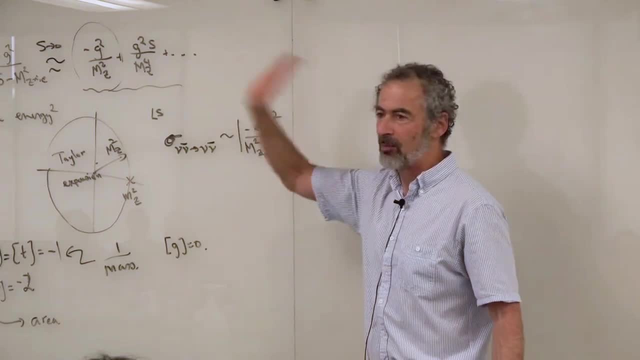 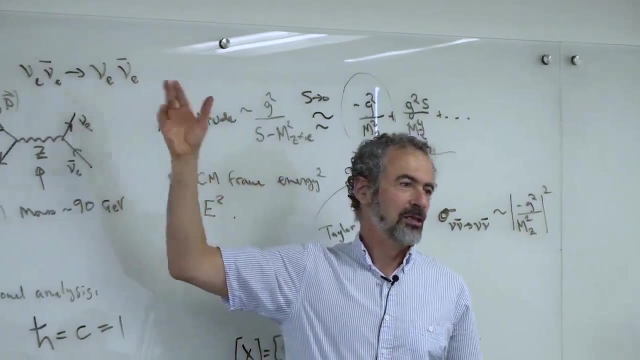 integral when you add up your amplitude, squared over all possible final states, And there's no dimension in the problem. really, The neutrino mass is so small and I'm going to assume, where the energy is well above the neutrino mass, that the only dimension is the energy. 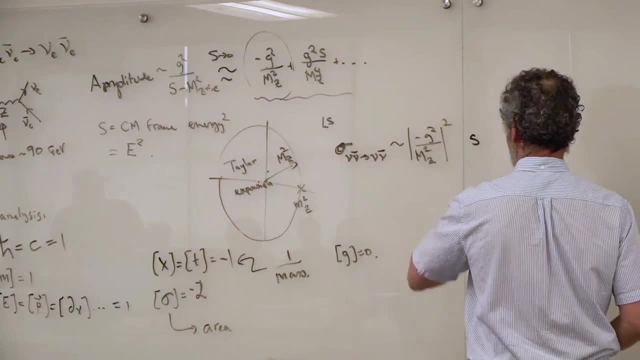 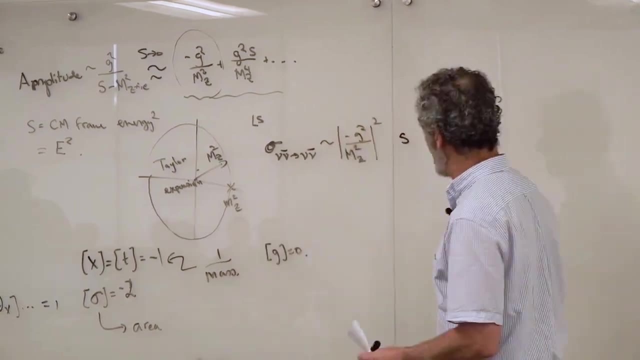 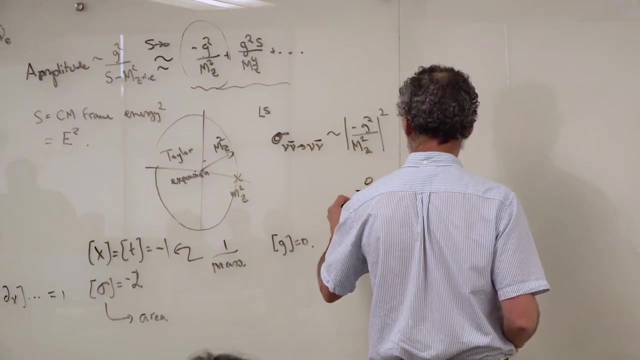 you're doing the experiment at. So you're going to get a power of s out in front which has dimensions mass squared, because it goes like an energy squared, And this has important consequences. That means that this goes to zero as s goes to zero. That's sort of simple. 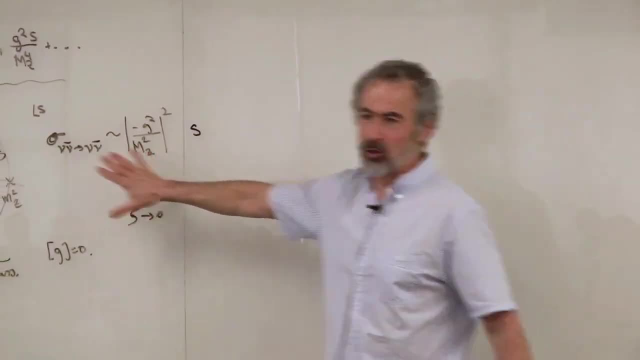 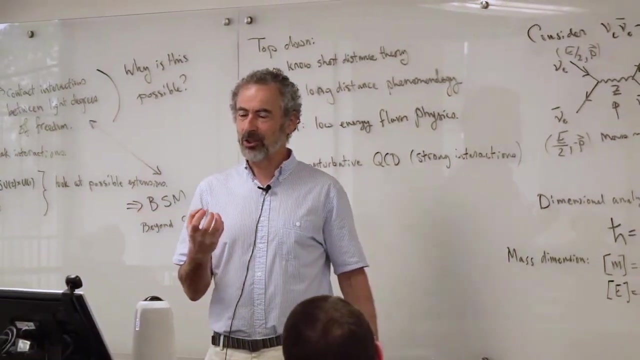 dimensional analysis. But it explains why this is such a weak interaction And in fact that's where we get the name weak interactions. Fermi's theory described an interaction which in itself, intrinsically, it's hard to say it's small because there's no small dimensionless. 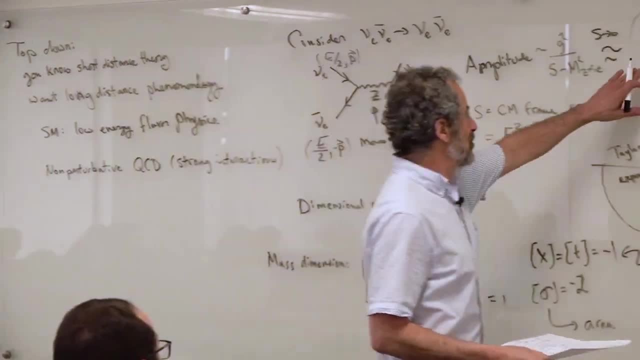 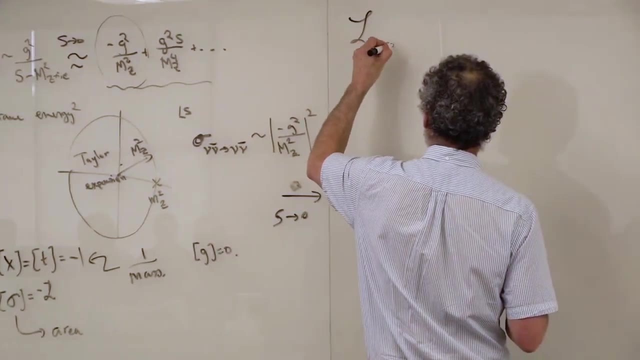 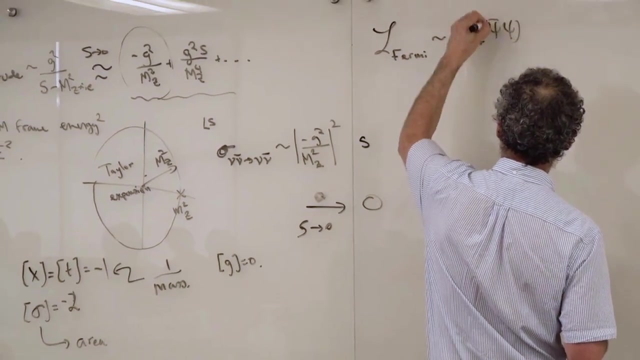 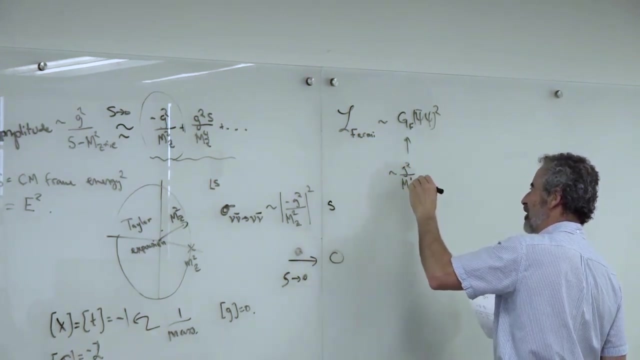 number associated with it. Rather, he said: let's just use this as our starting point. And so the Fermi theory was that this goes like G Fermi, psi, bar, psi squared, where this goes like G squared over, in this case Mw squared, which is about equal to G squared over Mz squared, You're going to 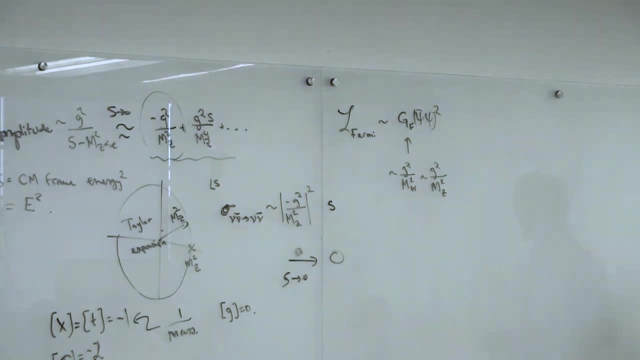 see a lot of squiggles in my talk. I'm not going to talk about them. I'm going to do numbers that are very accurate. I'm not interested in that. So he did something which is sort of interesting here. Over here I was talking about Taylor. 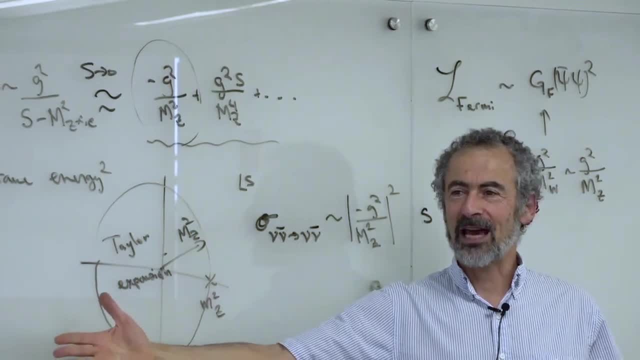 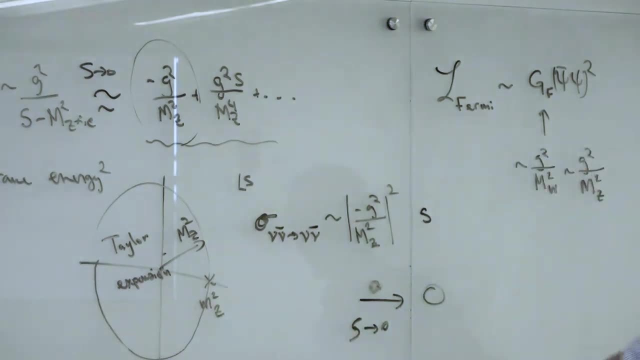 expanding an amplitude. But that's sort of stupid. Why would you want to calculate an amplitude in a complicated theory and then just Taylor expand it? That doesn't really gain you information. But the cool thing is that this expanded amplitude can be computed directly from a simpler theory. 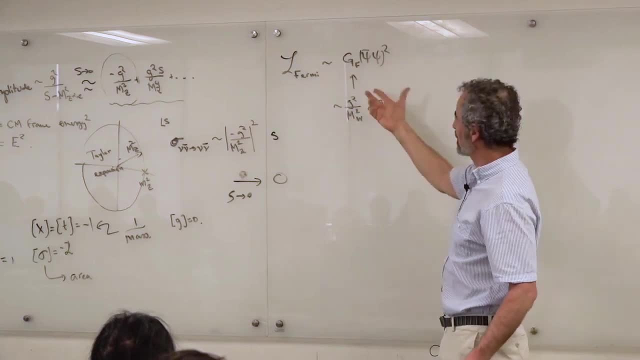 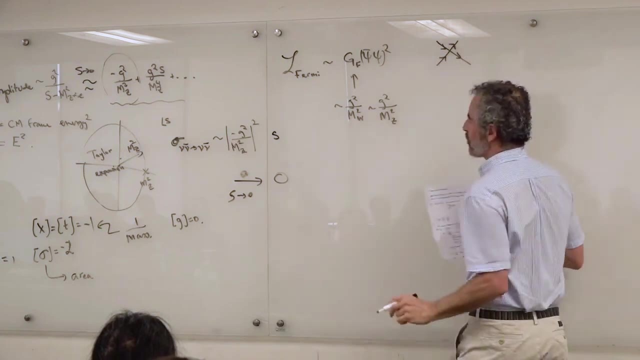 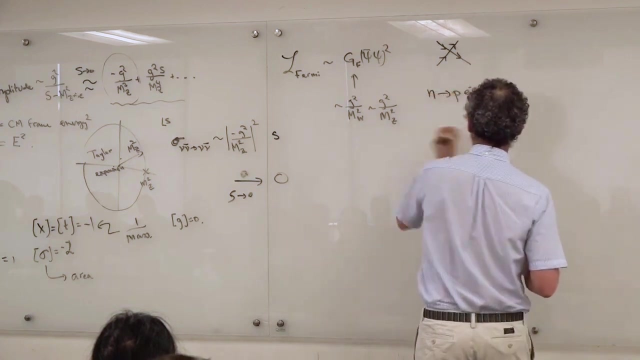 This is much simpler than the standard model. It just says that there are four particles, There are four fields which come together at a point. And of course Fermi was not interested in neutrino scattering, He was interested in n goes to p, e, minus. And then they knew: 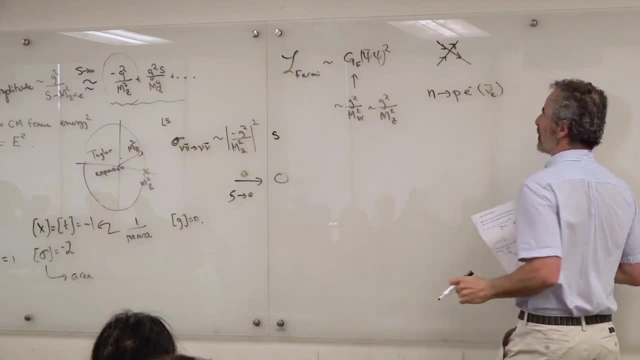 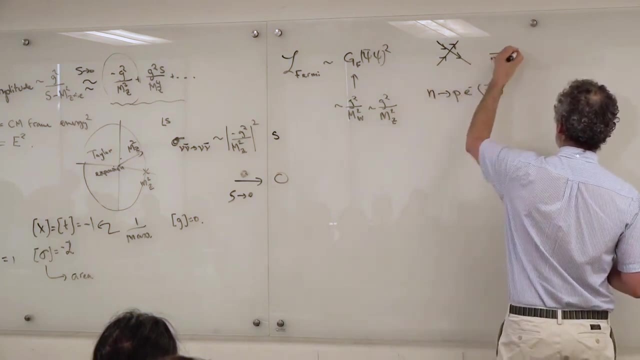 there was missing energy, which we know is an anti-neutrino, But of course they hadn't detected it then. So you turn this around and you say this is a neutron, And it turns into a proton and an electron and an anti-neutrino. 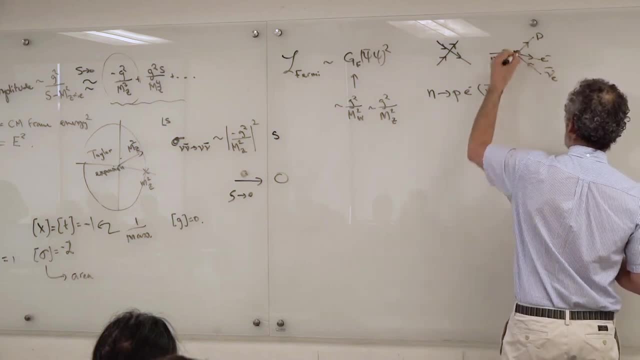 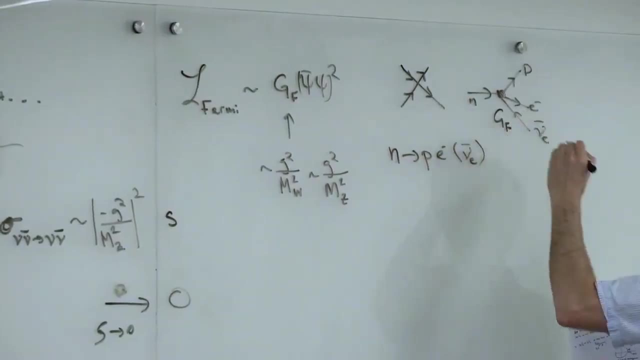 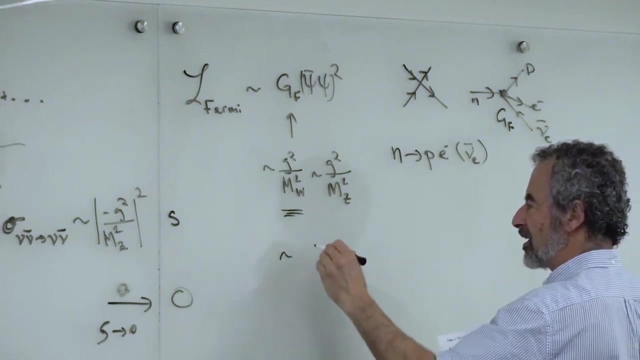 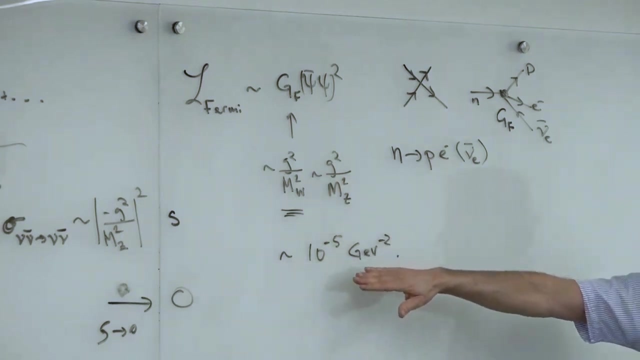 Right neutrino, And this is the tree-level application of this interaction, which is just basically G Fermi And G Fermi numerically. so it's this quantity here which is about 10 to the minus 5 Gv to the minus 2.. And so a Gv was more energy than was available to Fermi at 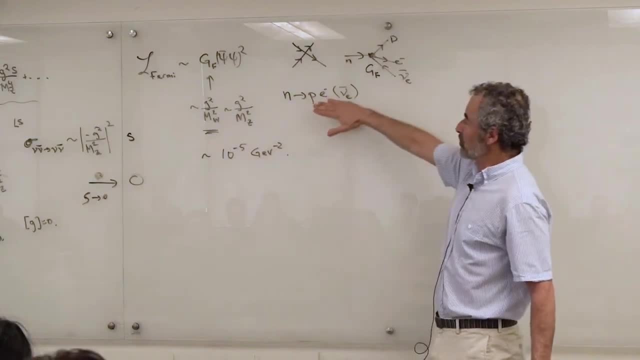 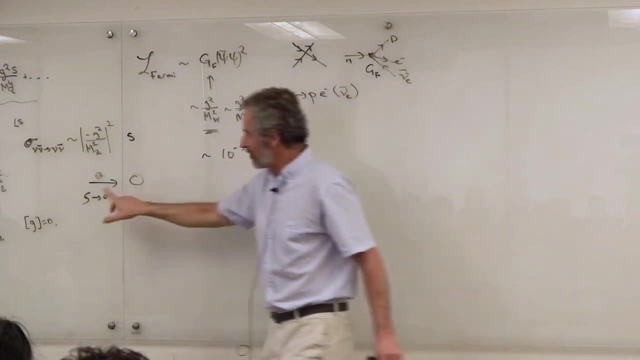 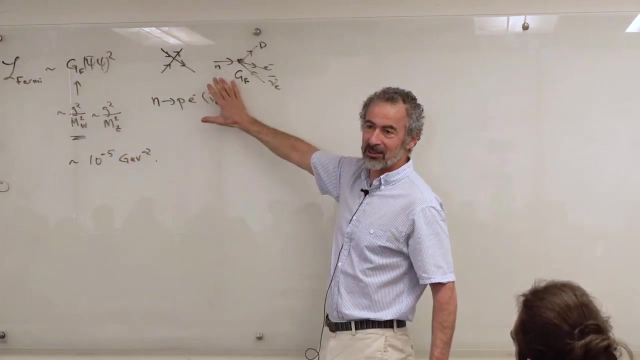 the time and there's a 10 to the minus 5.. So this was, you know, this decay. the energy exchange is about MeV. So when you put in the phase space factor- same thing as that happened here- to get the dimensions right- you find that down at MeV. this is an incredibly 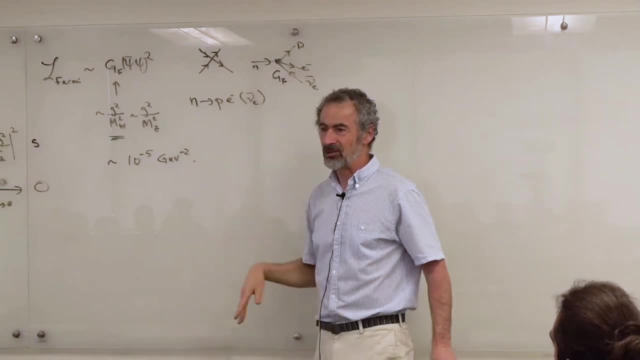 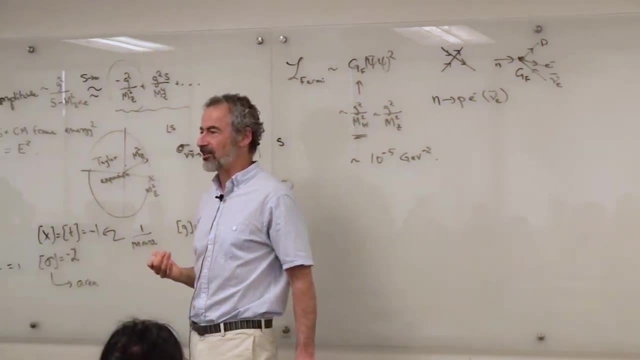 slow interaction. on the scale of particle physics It's, like you know, order 10 minutes, While if you ask how long does it take for a strong interaction particle to decay, like the rho or the delta, it's 10 to the minus 5 Gv to the minus 2.. So it's about 10 to the 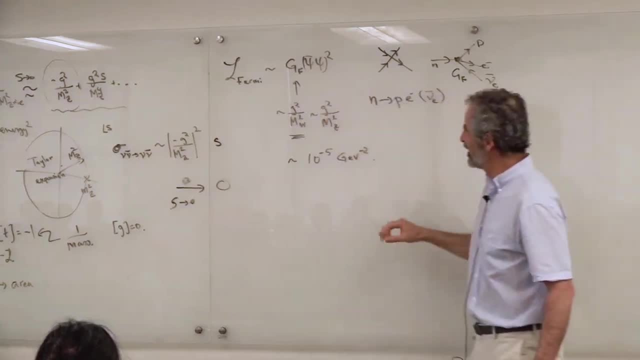 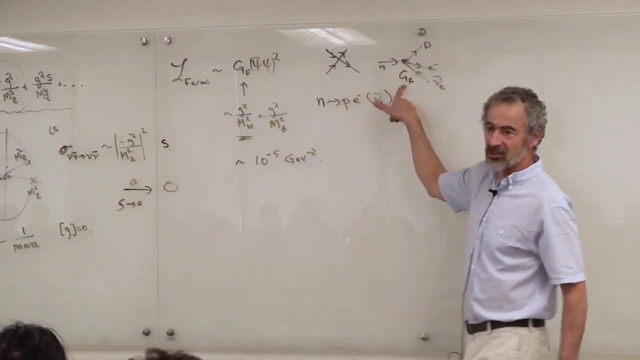 minus 24 seconds. So this is really weak And it's very simply understood just by dimensional analysis, because- but it's important to note that this is not intrinsically a weak interaction in the sense that if I go to high energy on the order of Mz, if when S is on the order, 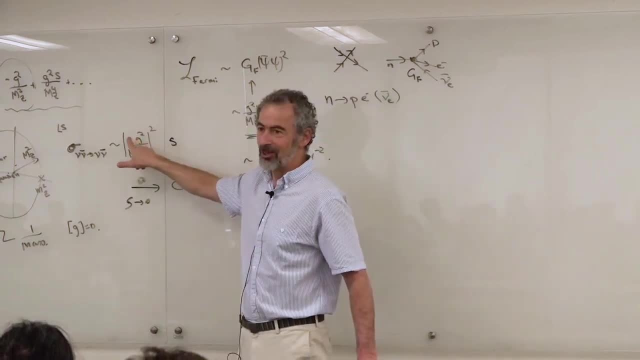 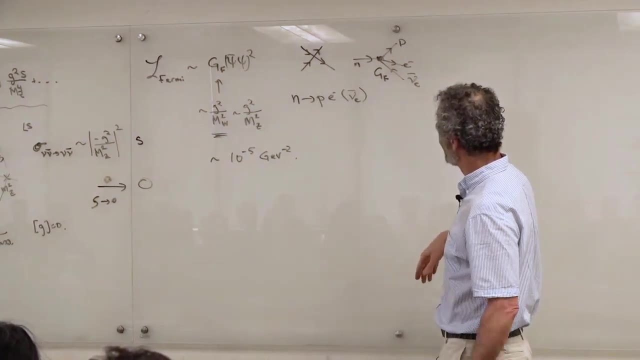 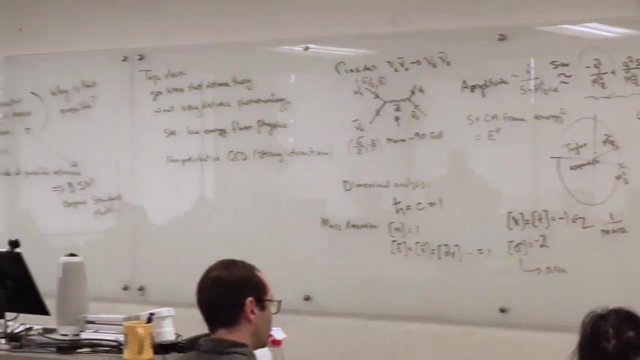 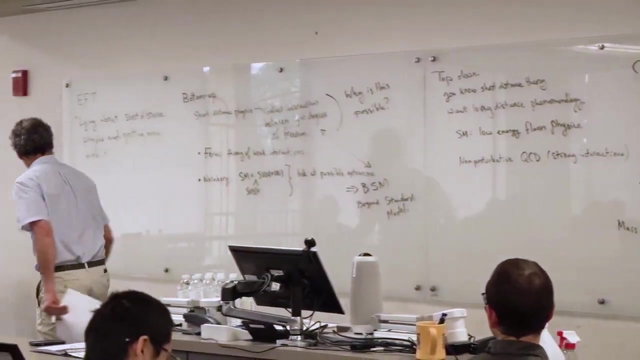 of Mz squared, then the size is set by G, And G is not small. It's order like the electron, electrical, electro, QED coupling. Okay, Okay, Okay. Well, what happens now if I start computing with loops in this theory? Radiative corrections. 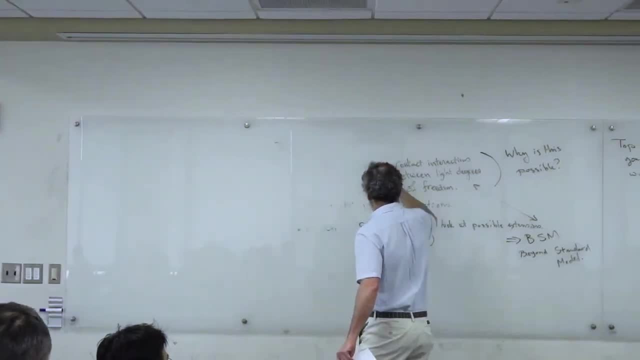 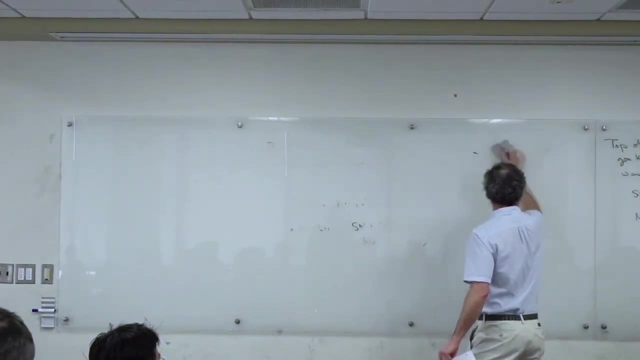 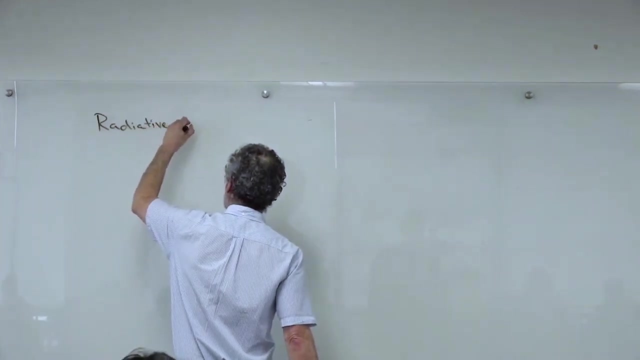 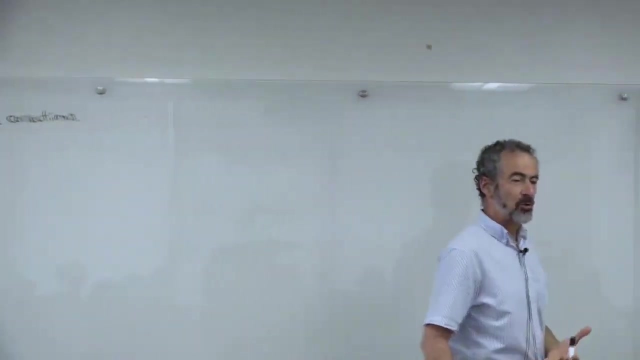 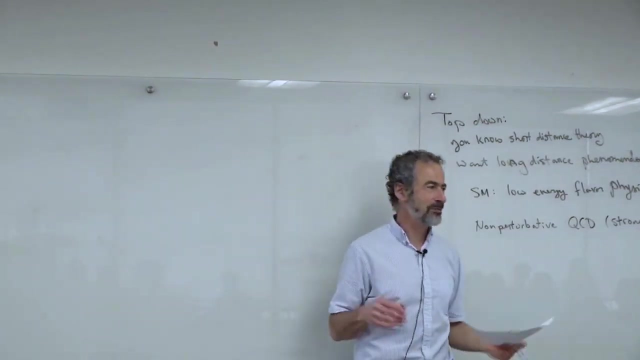 Two interesting things happen. So radiative corrections. it's just a statement that we're doing perturbation theory. We don't know how to solve these nonlinear theories exactly, except for in a few special cases in, you know, one dimension, one plus one dimensions. So we're doing perturbation in. 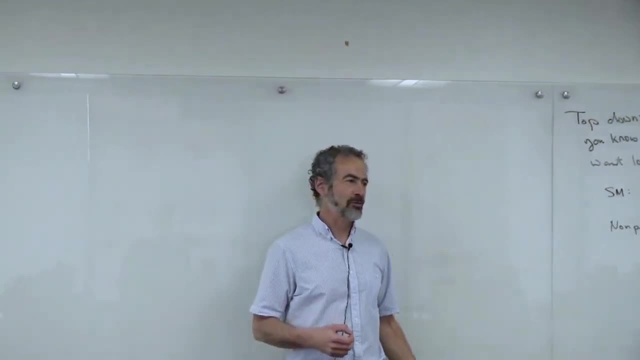 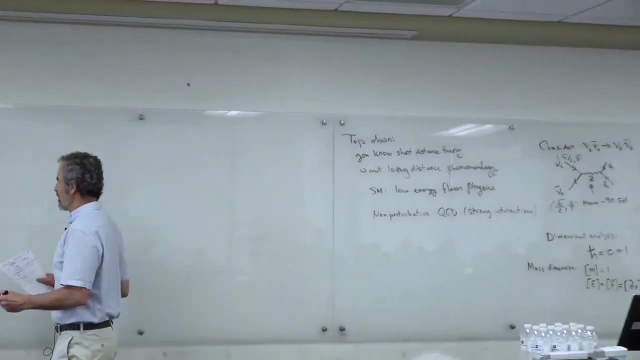 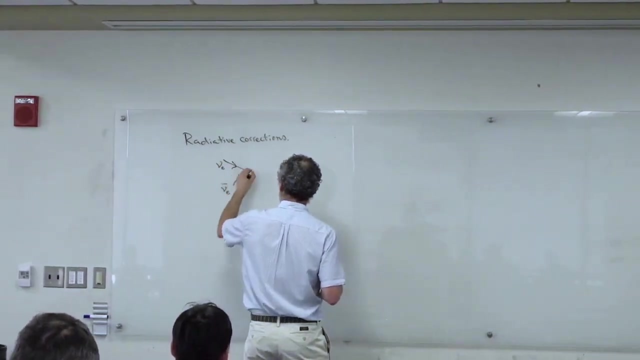 one dimension, one expansion and a loop expansion is equivalent to an expansion powers of h bar. So you're looking at more and more quantum-like effects as you go to higher loops. So let's look at one thing you might imagine is Z an internal loop of neutrinos, And we're 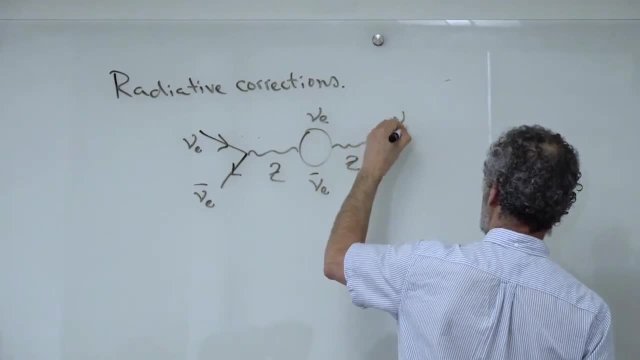 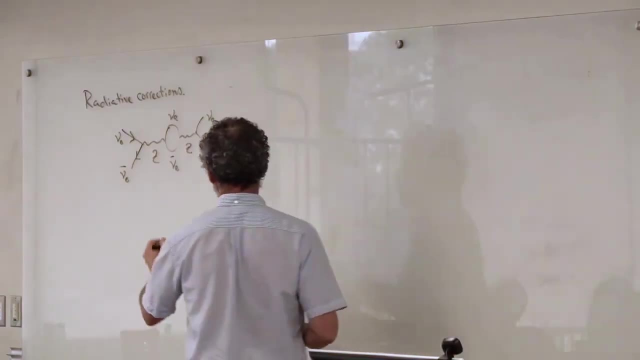 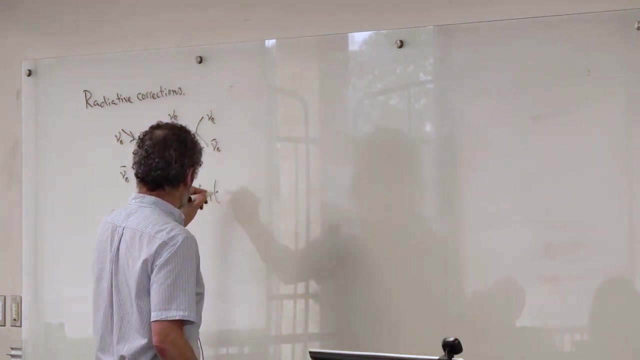 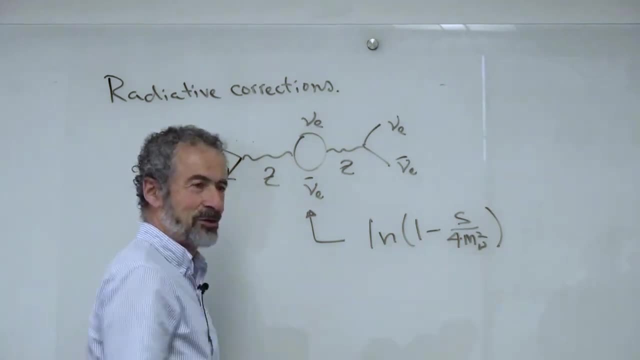 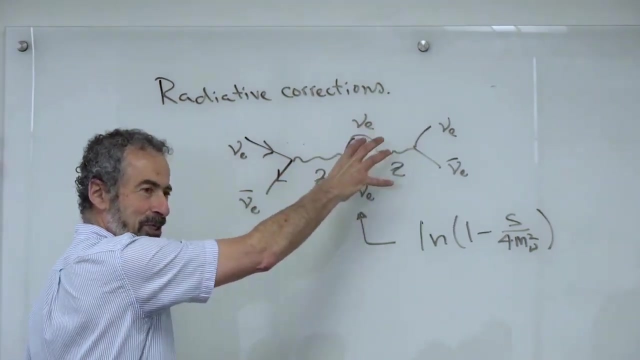 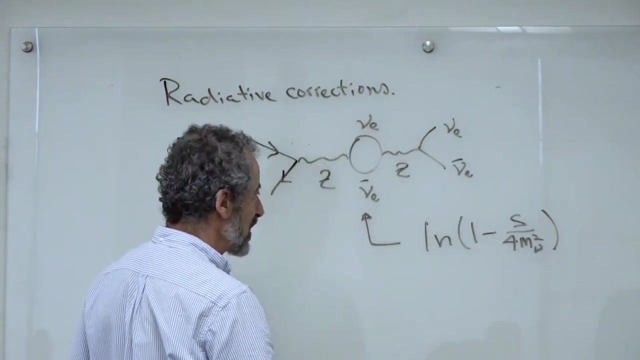 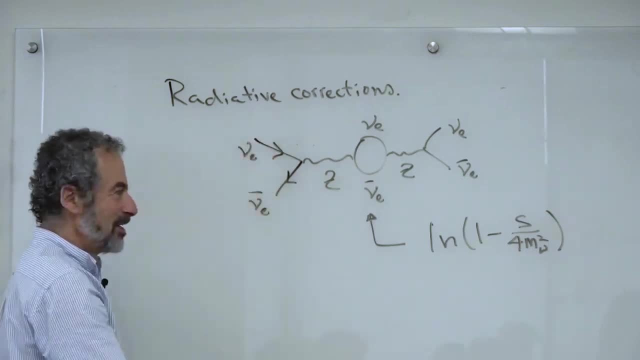 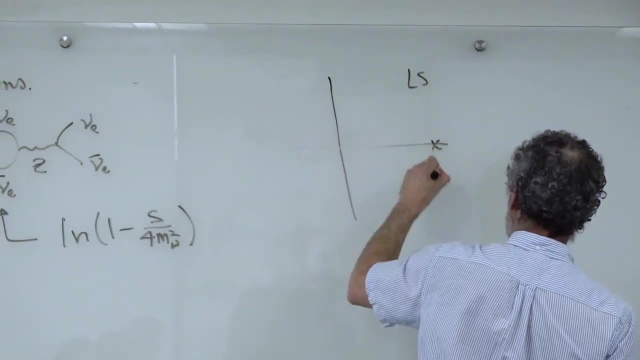 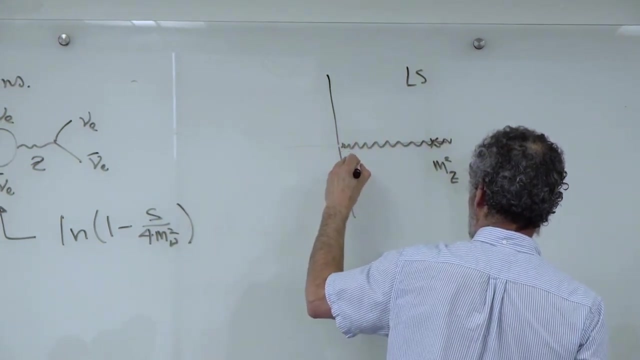 I know I have that much energy coming in because these were real neutrinos. So this looks terrible because now, when I look at the analytic structure here, I have this pole at mz squared, but now I have a cut that goes all the way down to 4 m neutrino. 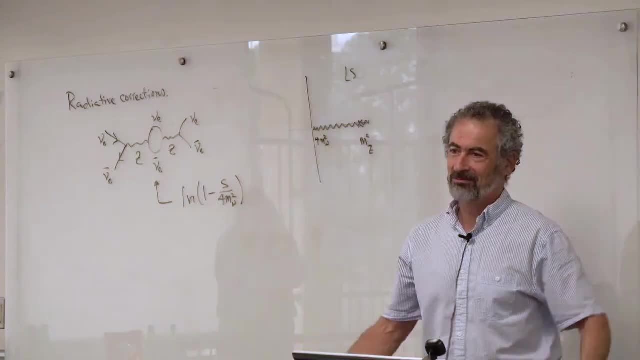 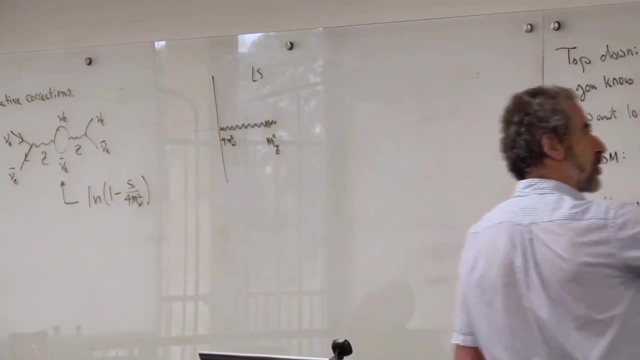 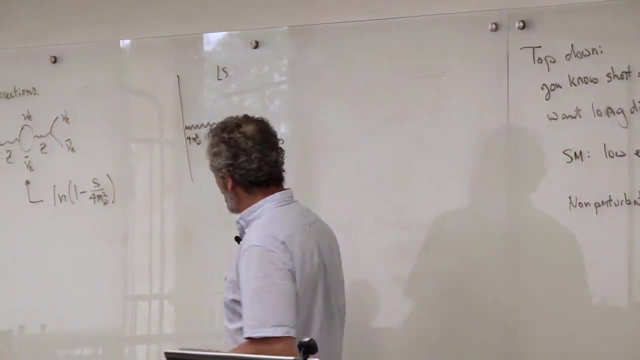 squared, which is incredibly low. it's less than an eV. m neutrino is less than an eV, maybe much less so. now it looks like how in the world could this Taylor expansion ever work? You can't expand this for low s if s is bigger than m neutrino. 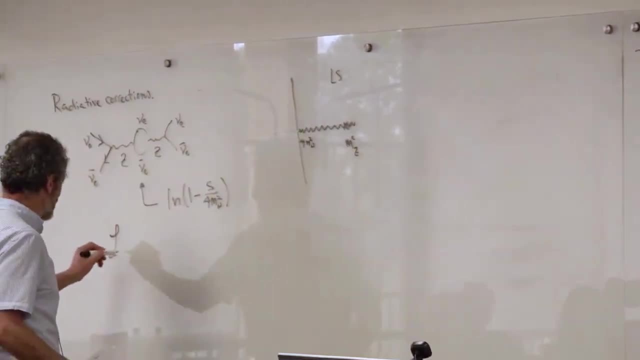 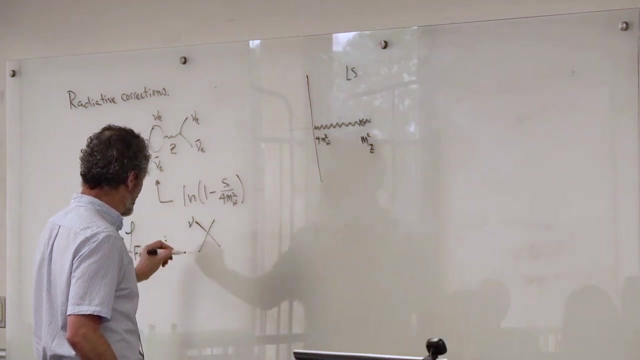 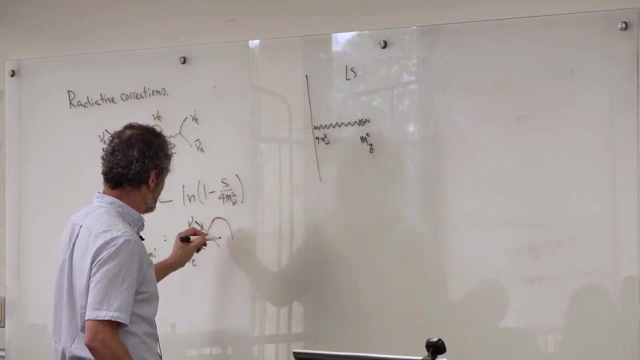 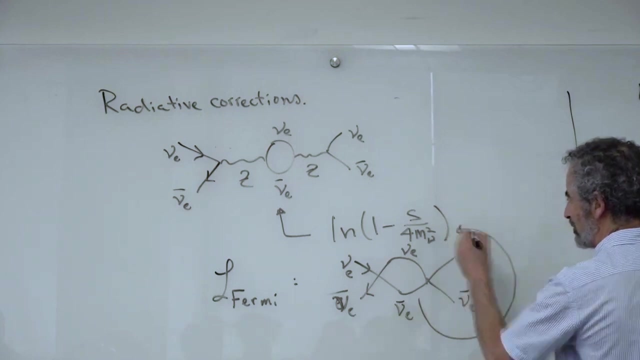 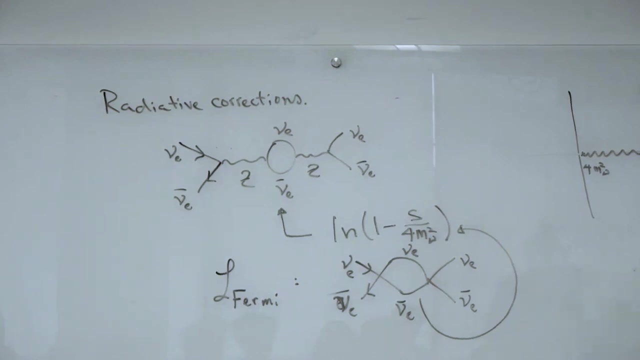 But the nice thing is that in the Fermi theory you have a graph where your neutrinos bounce off each other like that, and this loop has exactly the same log with the same coefficient. So in fact you're not asked to Taylor expand this part of the amplitude, you get it for. 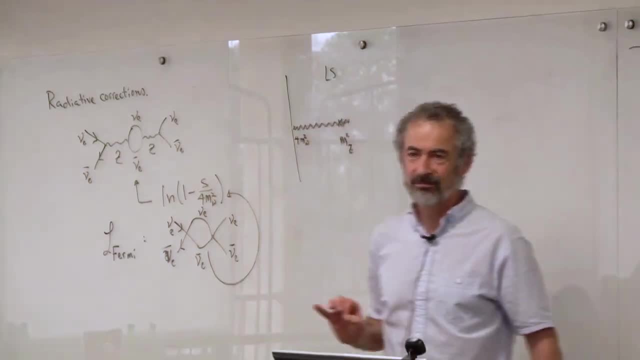 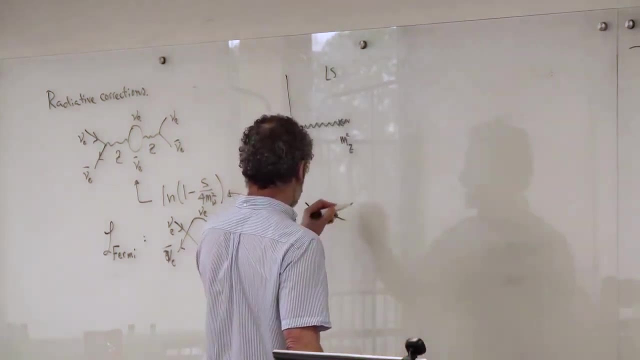 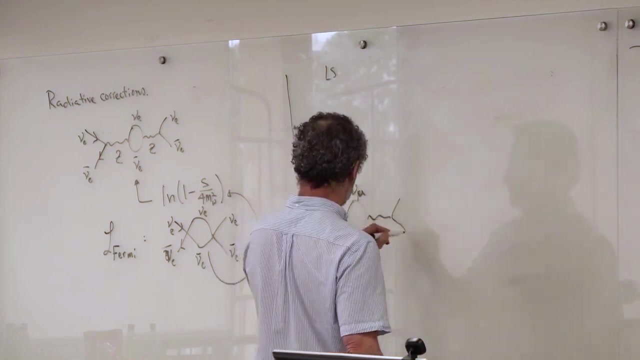 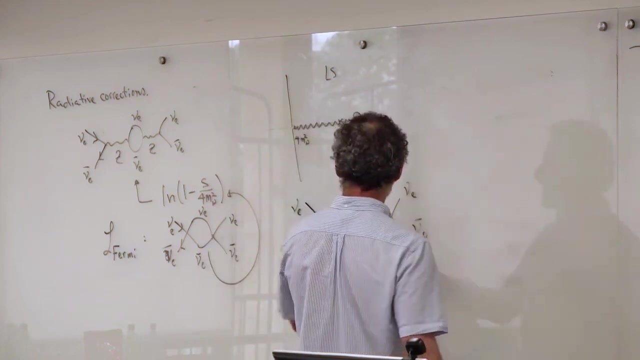 free in your effective field theory. So that's nice. so I dodged the bullet there. But what happens when I look at a mu-1 neutrino in here? So the electron neutrino is out here, but I put in a mu-1 neutrino here, this will also. 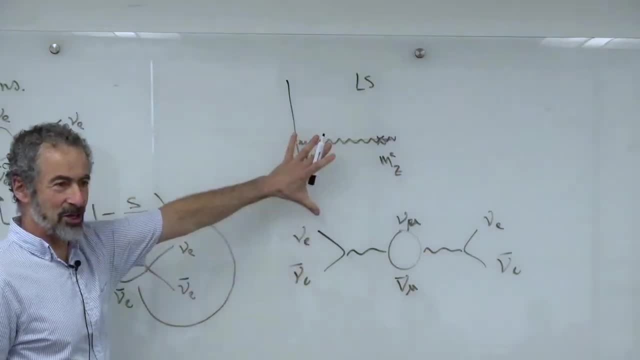 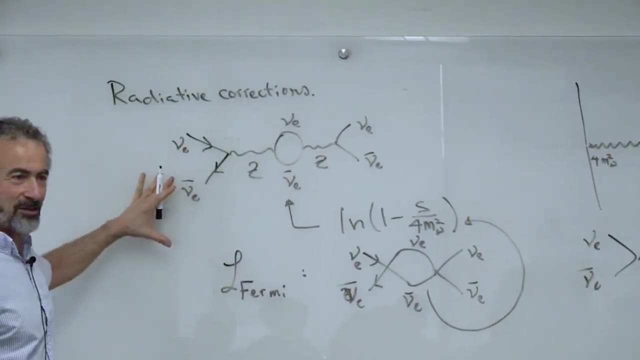 have a similar log which will destroy the expansion. And there is no new. if there's no new mu in the Fermi theory, then I'm screwed. okay, I've tried to expand something, but there are all these non-analytic things. 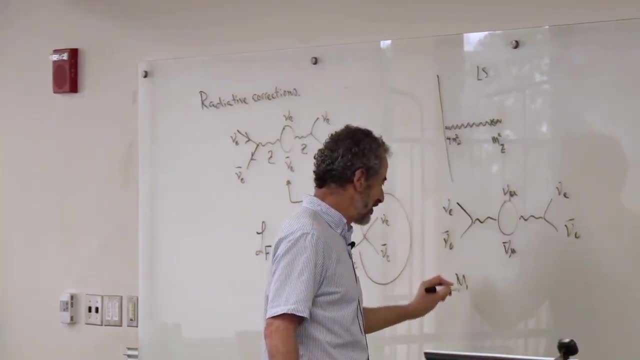 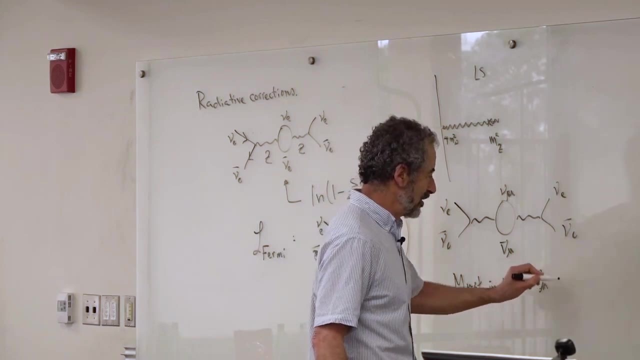 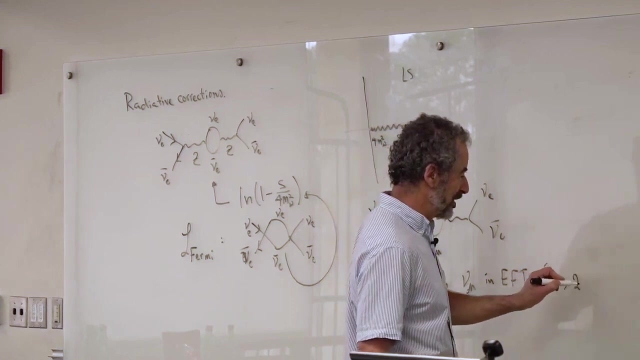 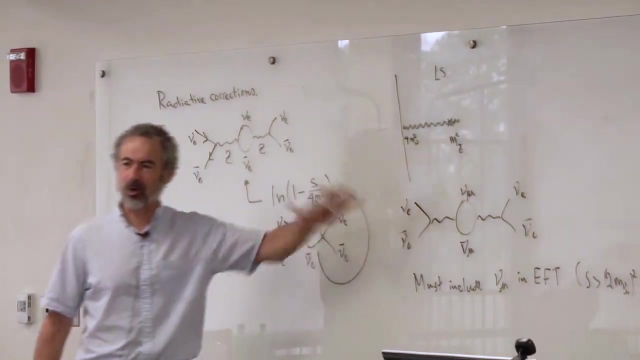 getting in the way. So the moral is: you must include new mu in the effective field theory for energies greater than two mu squared. Then I'll get that non-analytic part for free and I don't have to try to tailor expand it. 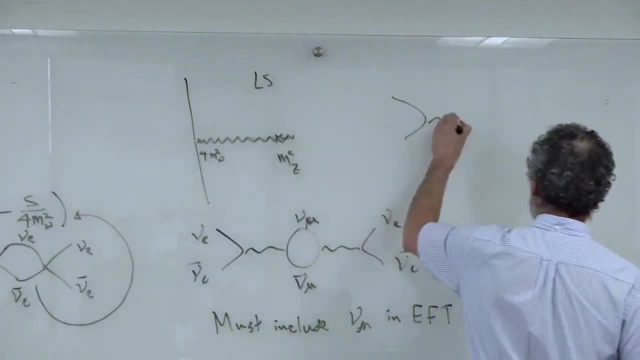 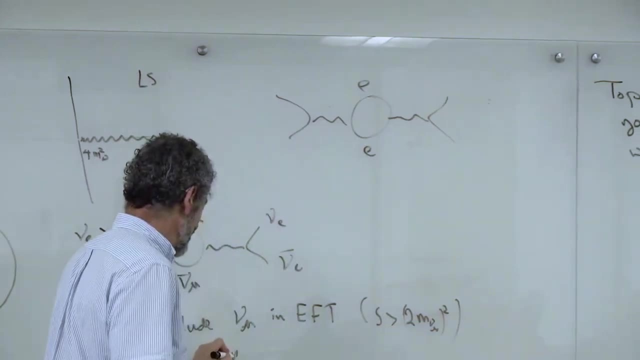 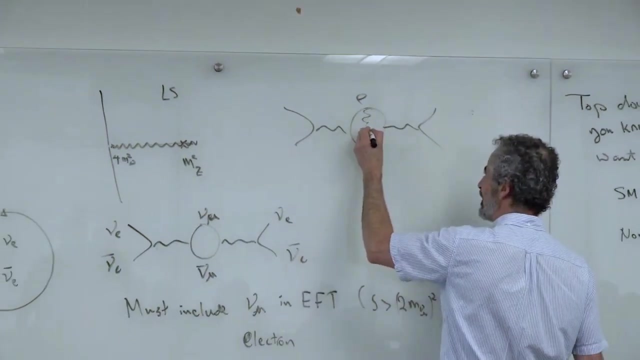 You can keep going with this. I could do. I could put an electron here. Suppose I wanna look at energies bigger than half an MeV, I have to add the electron And then, if I go to another loop, I could put a photon here. 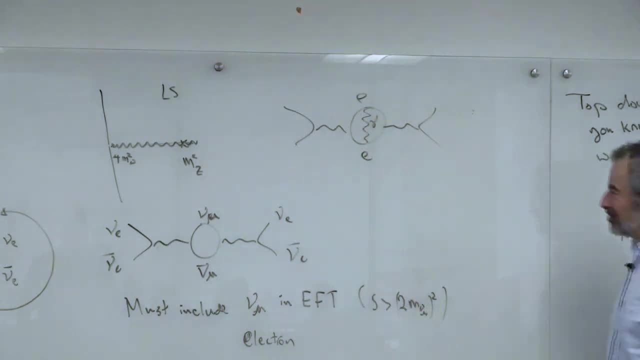 That'll lead to more non-analytic behavior. because I have enough energy to produce a real photon. Anything you can produce for real will cause all sorts of non-analytic stuff to appear in your amplitude, So I have to include the photon. 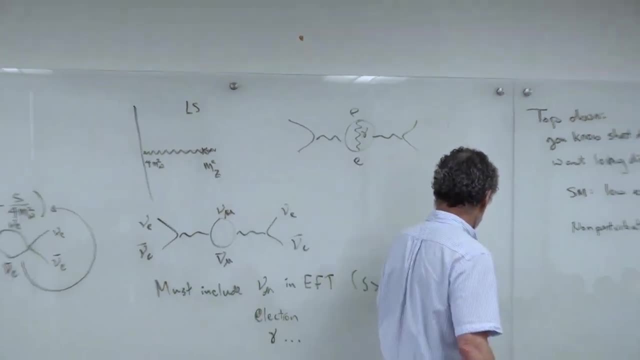 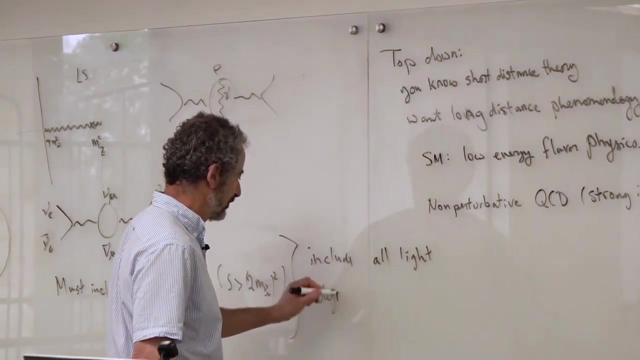 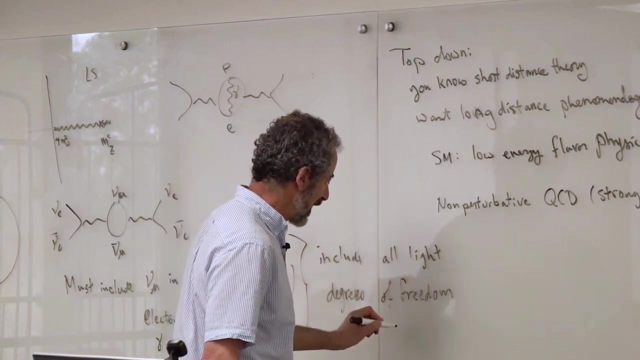 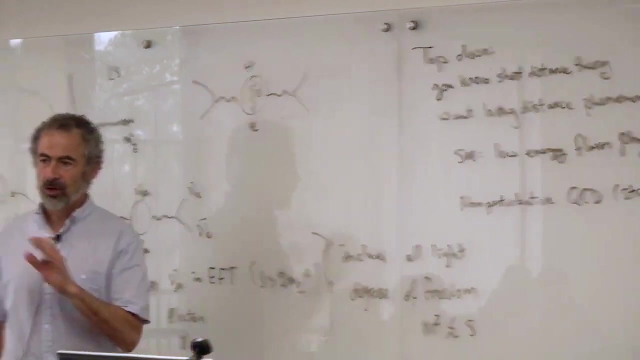 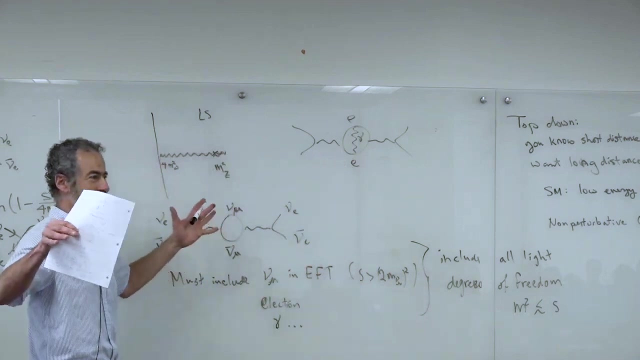 And so on. what I have to include is all light degrees of freedom where light means m squared, less than about the energy where you're working on With an understanding that, as s gets close to m squared, I'm gonna start getting big corrections because I'm reaching the limit of my radius of convergence. 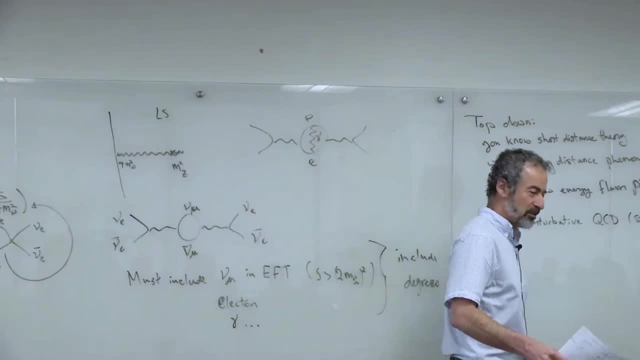 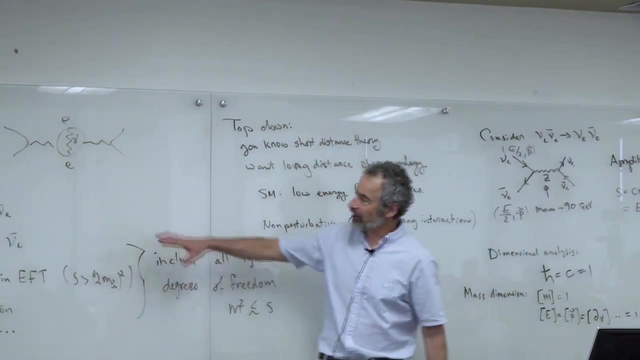 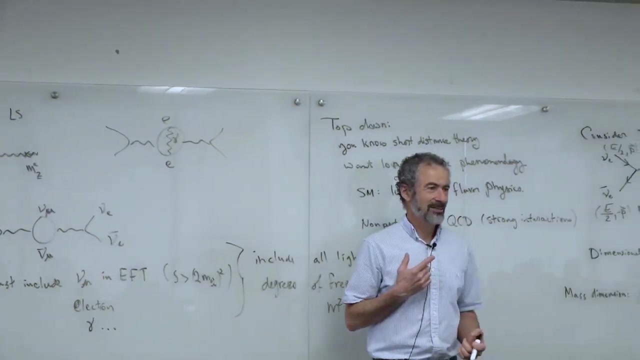 So there's a couple of cool things here, which is that if you include your light particles and you have your effective theory and you find that as you go to higher energy, it starts behaving worse and worse, that is a sign that you're getting close to a new particle. 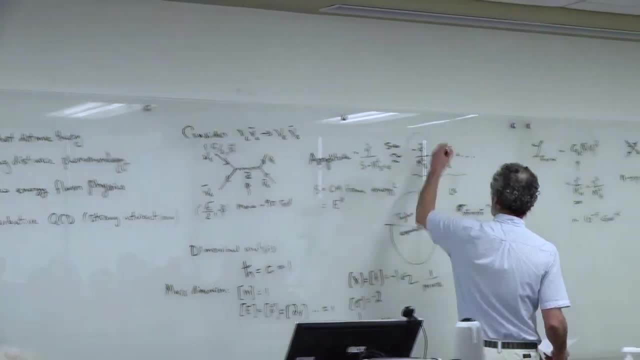 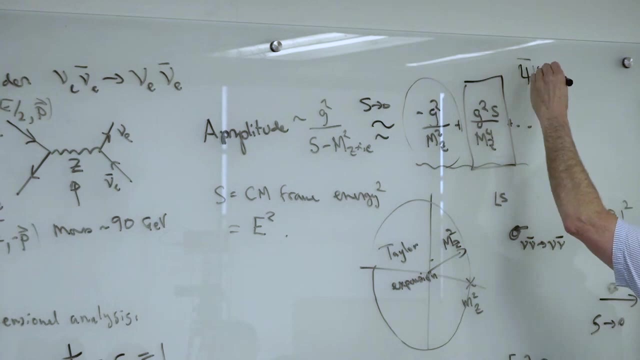 So what would happen? Well, if s gets bigger, you have to start including this term here. Okay, and the way I'd include that in the Fermi theory is I'd have something that looks like psi bar psi d squared, psi bar psi. 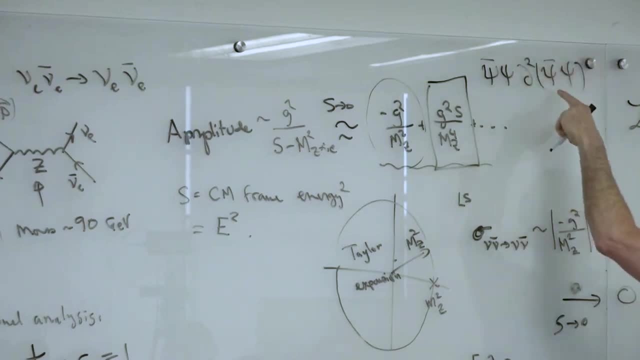 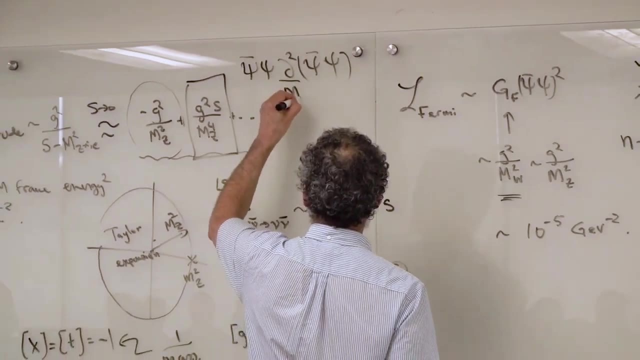 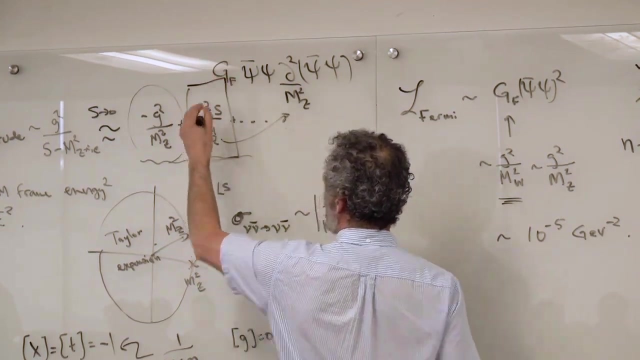 Because this would pull in the energy being carried by those neutrinos And I'd have to have this divided by mz squared to reflect this extra power of mz there, with the g Fermi out in front, which does the other g squared over mz squared. 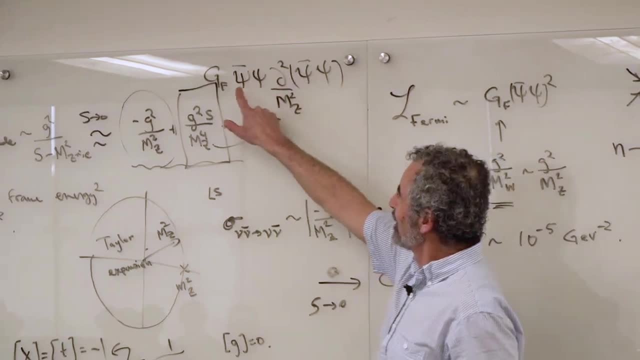 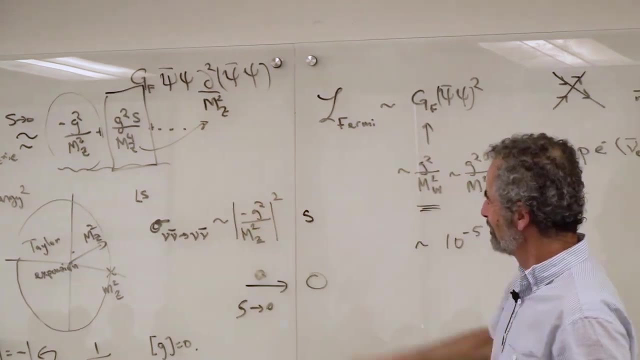 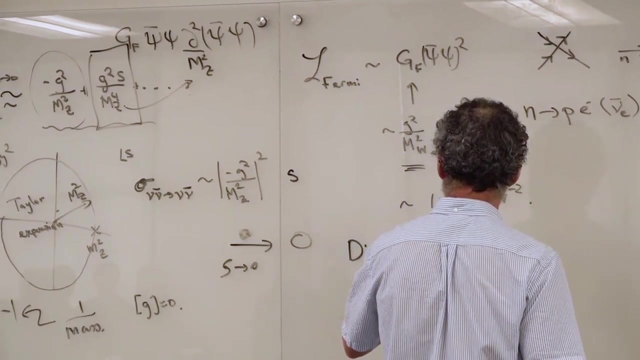 So it's a higher dimension operator in the sense that this d squared has dimension two. so I have to divide by a mass squared, to put it in my Lagrangian. So let me go back to dimensional analysis. We know that s, which is the action, 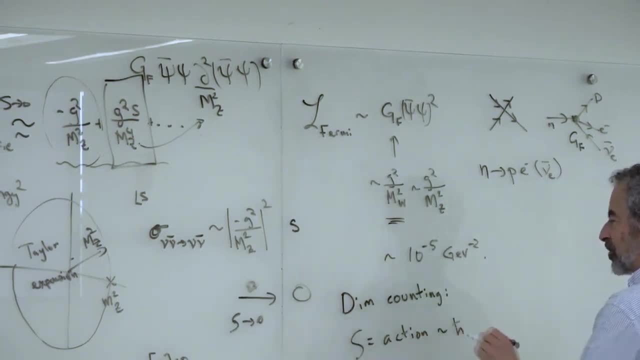 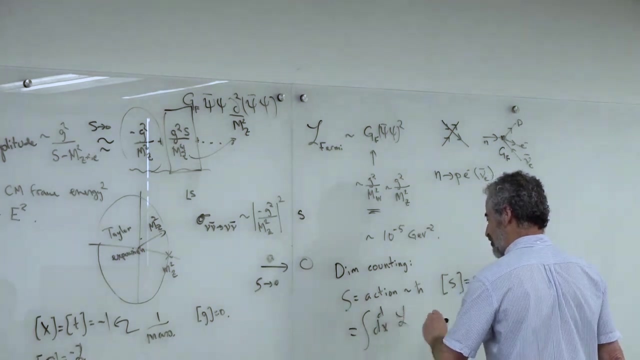 has the same dimensions as h bar, which is set to one. So we know that the mass dimension of s is zero. It's dimensionless in our units, But it's also equal to the integral over spacetime of your Lagrange density. 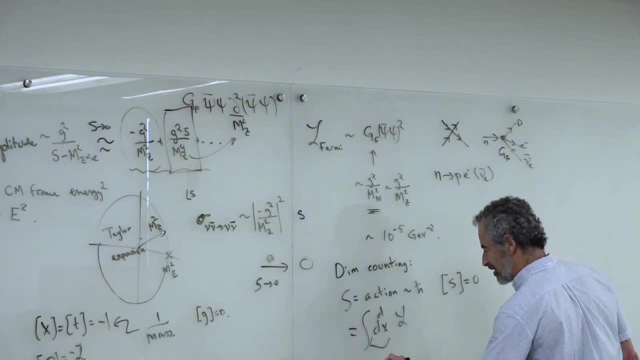 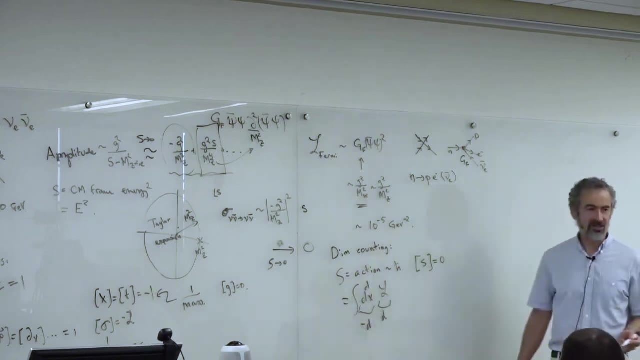 And this goes like dimension minus d and therefore this must have dimension d. So the Lagrange density has to have the dimension of the spacetime you're working in. All Fermions are described by the Dirac theory, which is psi bar i d slash minus m psi. 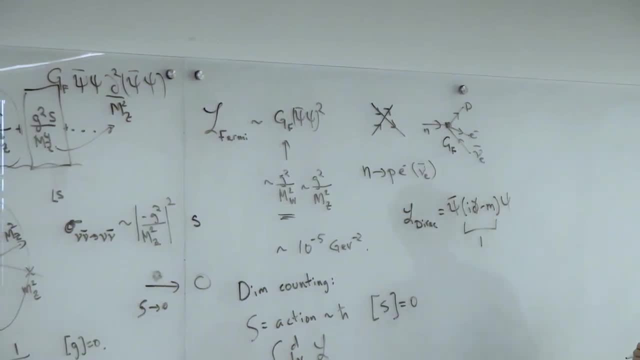 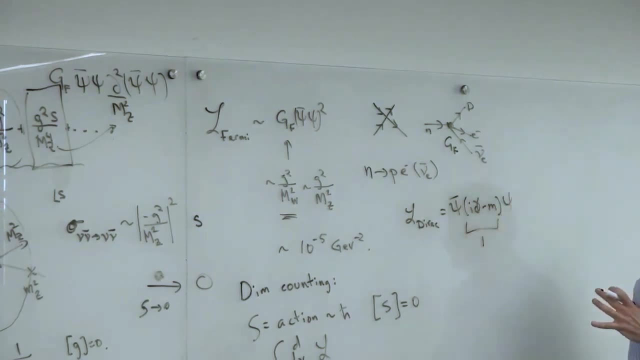 This has the mass dimension of m, which is dimension one. If we're in d equals four, three plus one spacetime dimensions, then the whole thing has dimension four and psi and psi bar have the same dimensions. That means that the dimension of psi is three halves. 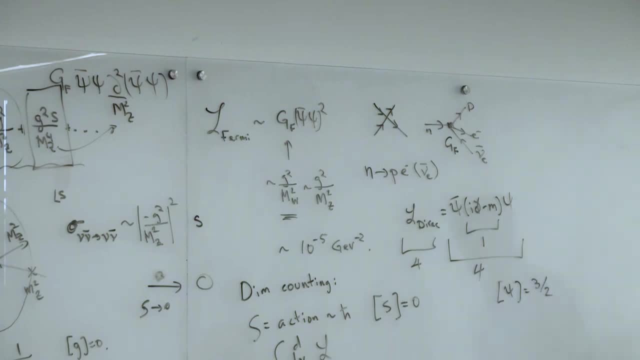 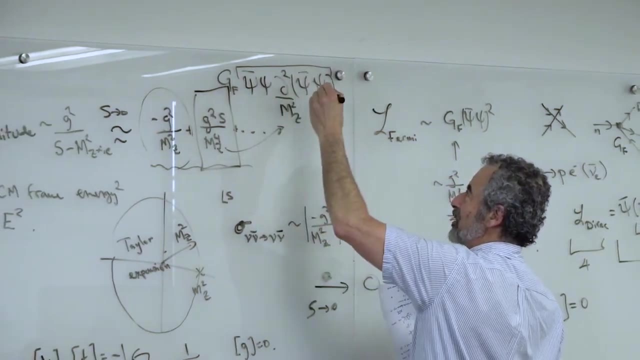 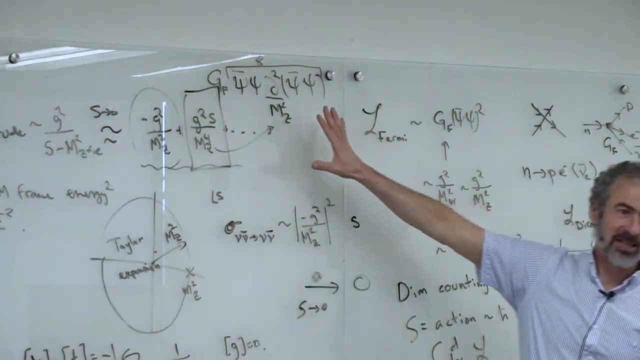 because psi bar psi has the dimension three. So if I look at this operator I can say this has dimension three plus three plus two, So that's eight. Our Lagrange density has to have dimension four if we're in four spacetime dimensions. 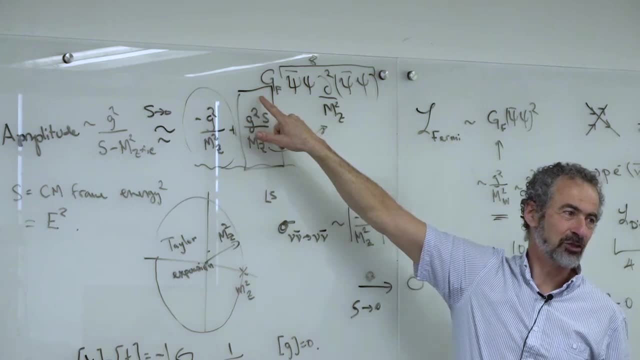 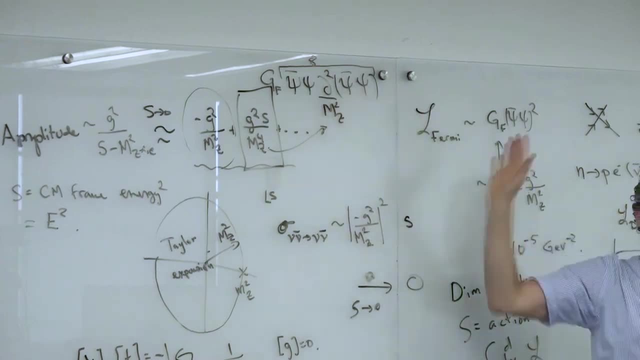 So there are two inverse powers of mass. One is hiding in G Fermi and one's this explicit power here. So this extra d squared is what we call a higher dimension operator. Higher dimension operators go with higher powers of m, z, So at low s. 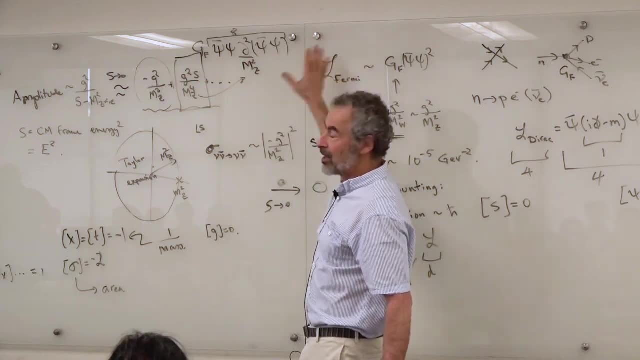 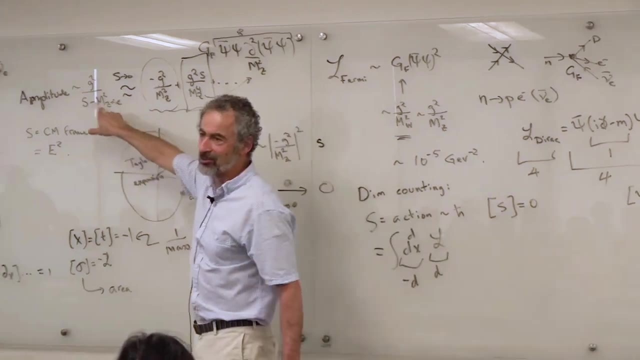 these are smaller and smaller effects and I can ignore them. But if I start finding my theories breaking down, then I have to start concluding them, and that is telling you: oh, I must be getting close to something. There must be some new physics on the horizon. 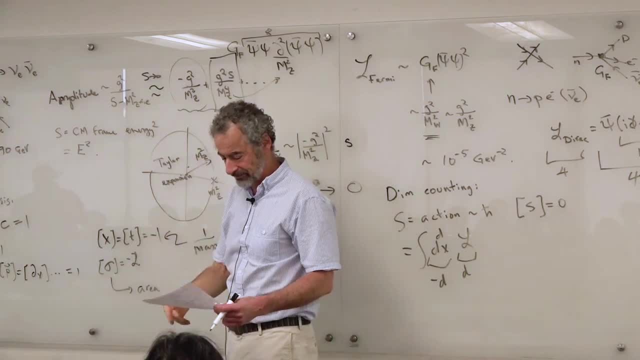 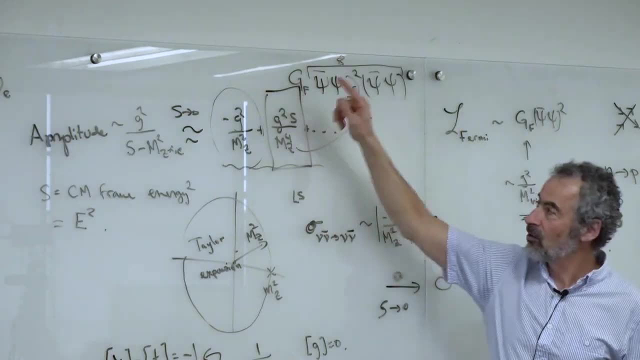 that's starting to make my theory break down. Note that, even though they knew the dimension of G Fermi, if G Fermi is given by G squared over m z squared or G squared over m w squared, you actually don't know what the w mass is. 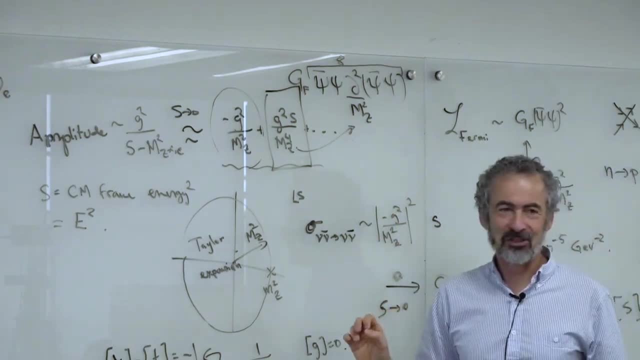 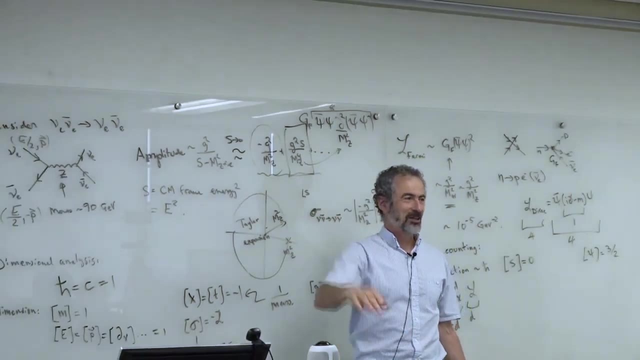 Because you don't know what G is. And when I was a student undergrad student, I once saw a huge stack of letters that were being thrown out and was sitting in the hallway of the physics building and I just started thumbing through them. 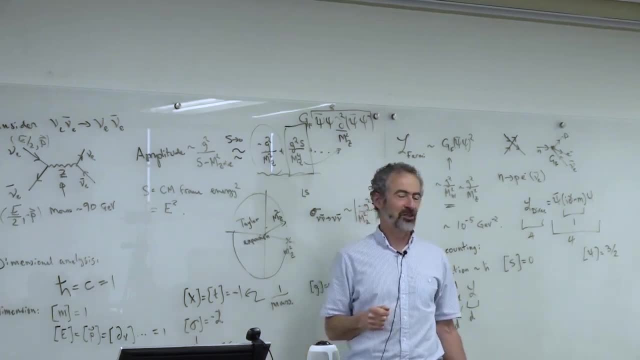 And I found one which had the theoretical explanations for the discovery of the J psi which had just happened. And there were five theoretical papers, one of which was completely right, by Applequist and co-authors, and four which were completely wrong, And one of them was by Schwinger. 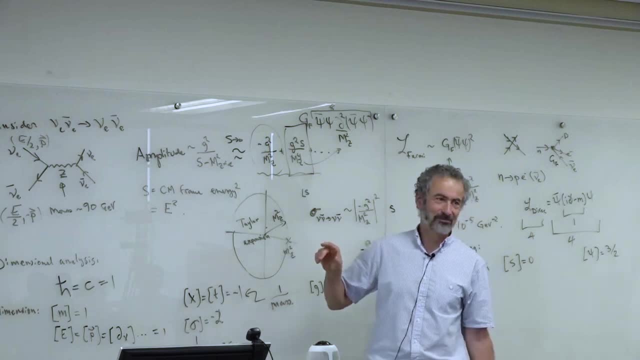 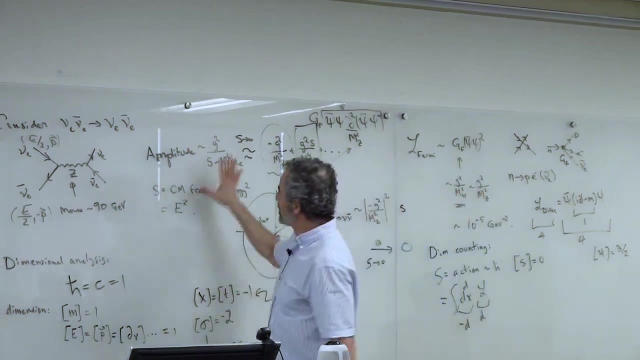 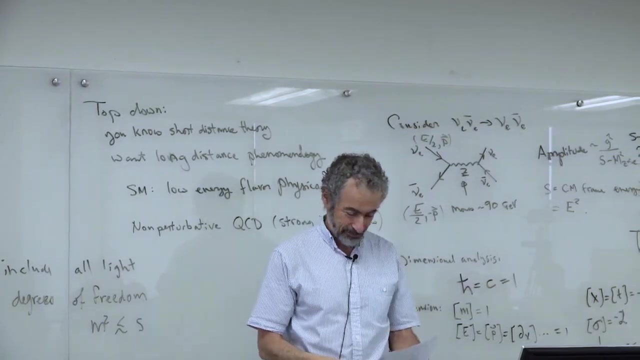 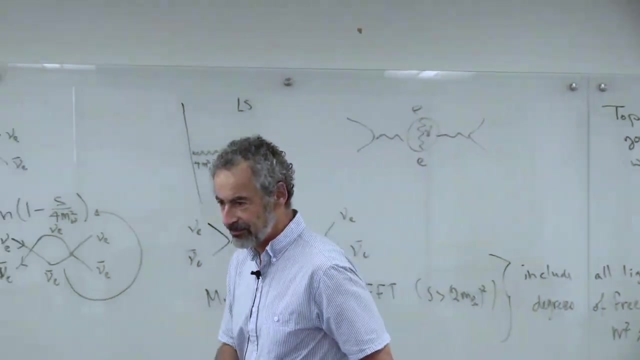 and Schwinger said it's the w. You're seeing the resonance coming from this propagator? Because he thought that the effective theory had broken down. we were actually at an energy where it could produce the w. Yeah, So you're already going to get, say, 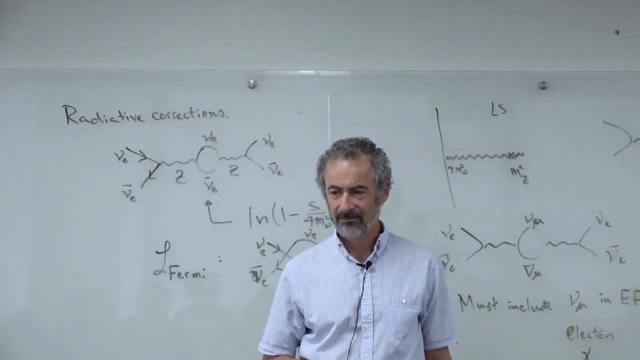 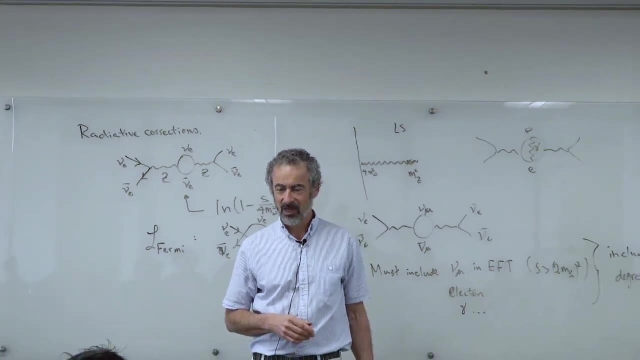 the expected energy, right, Yeah, And then nothing. but if you open the box of the data- the high energy- actually the data doesn't show any. The data what? The data doesn't show any like. Ah, so that's where we're at, right. 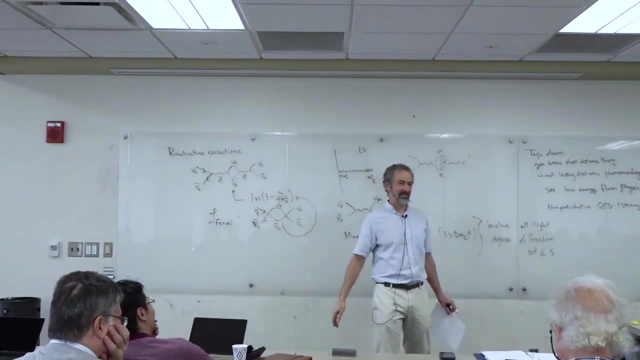 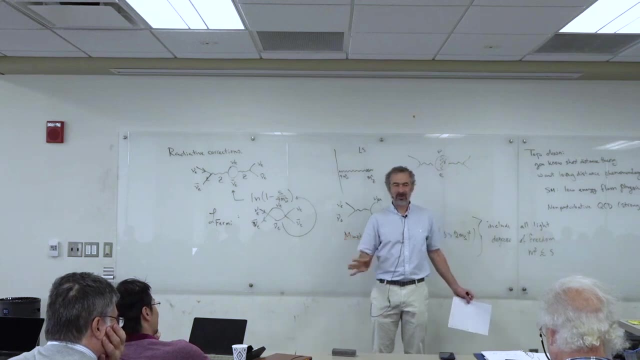 Yes, exactly, We're right. Everybody thought you'd see new particles at LHC. but if you don't see new particles, not a problem, because maybe everybody was sure there'd be particles at 10 TV or something, so we'd be able to see them. 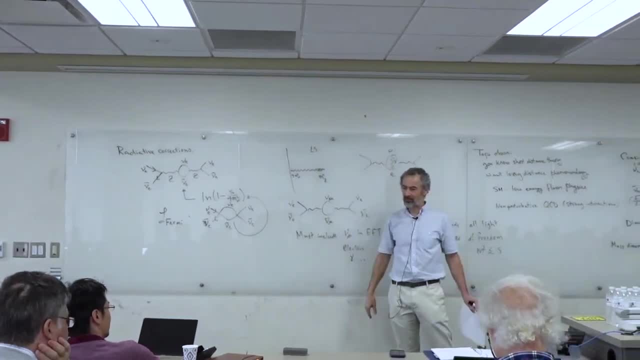 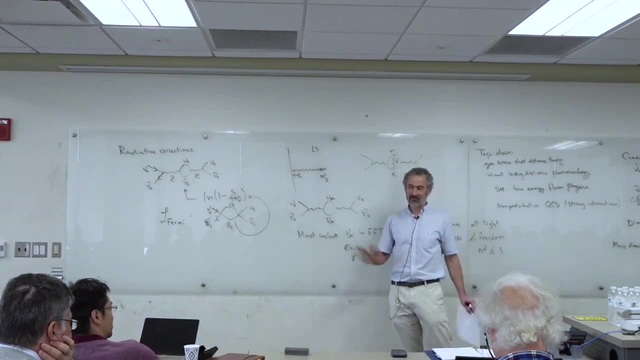 through radiative corrections or through these little deviations from the standard model. And it's not correct to say there have been no deviations, because one thing that's been discovered- not at LHC- are neutrino masses. Neutrino masses don't occur. 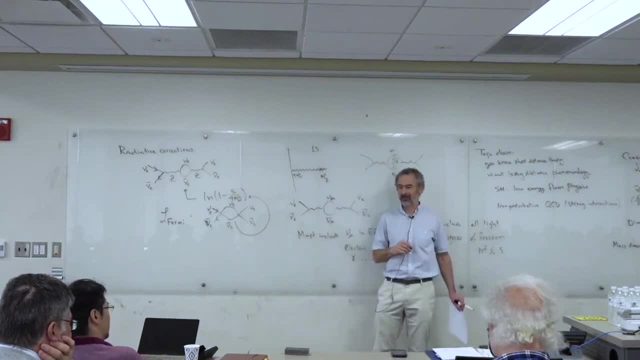 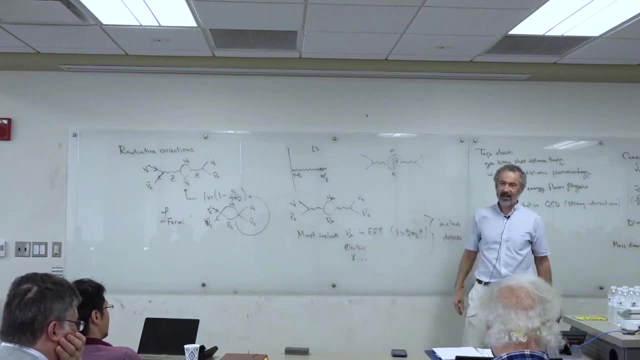 in the standard model and, as I'll show you, they come from a higher dimension operator. But overall, the LHC accelerator physics has not found traces of this new physics and it's what people who, in the early days of Grand Unified theory, 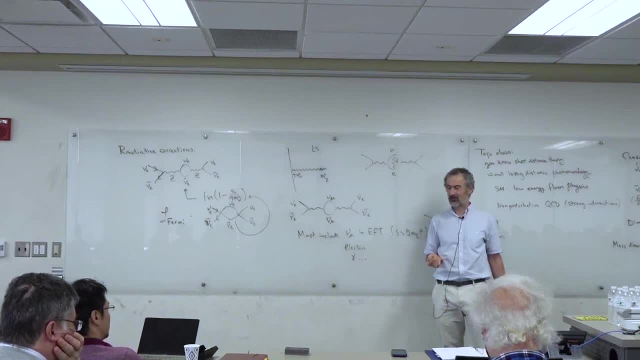 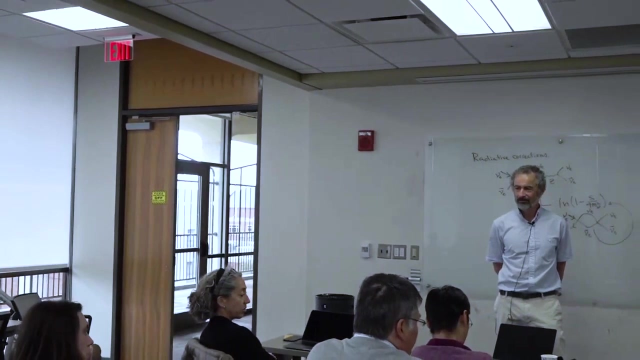 is called the desert. The desert was the absence of new particles between the standard model and the Grand Unified scale at 10 to the 16 GeV. You had a question. Yeah, So when we're adding terms of our expansion, was there any like? I guess historical intuition as to like how many terms they were adding before. they were like: there's something there. So physicists are lazy, They like simple theories. If you have to start adding too many terms, you feel like you're like. 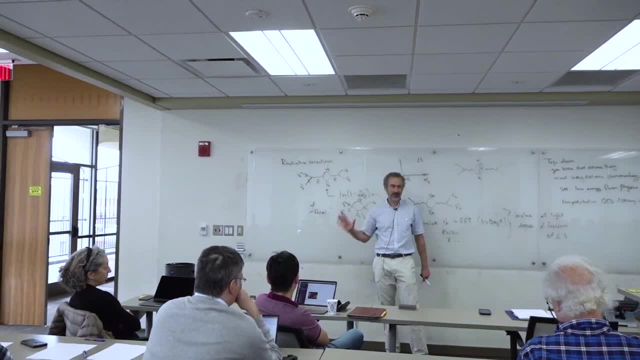 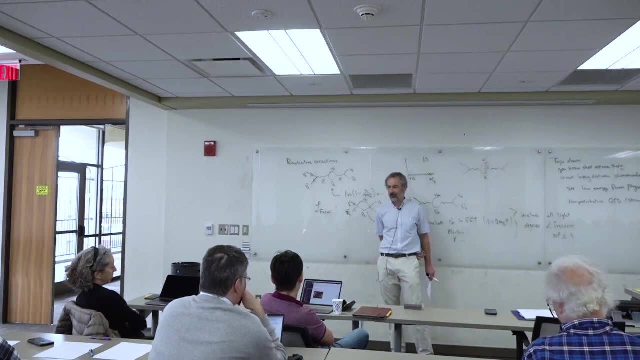 totally adding orbits on orbits and it's not worth your time. you should start over with a new theory, And that is the effect of field theory: telling you that your old theory is breaking down. It's time to really start looking for a new one. 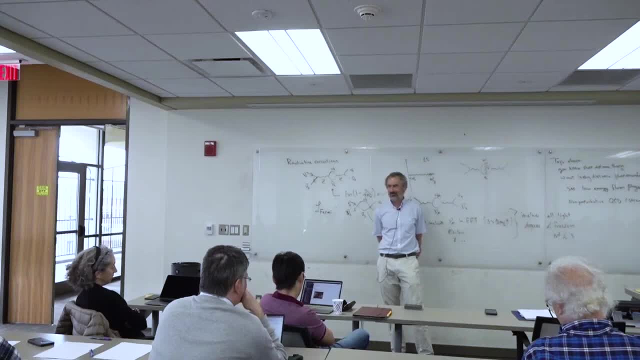 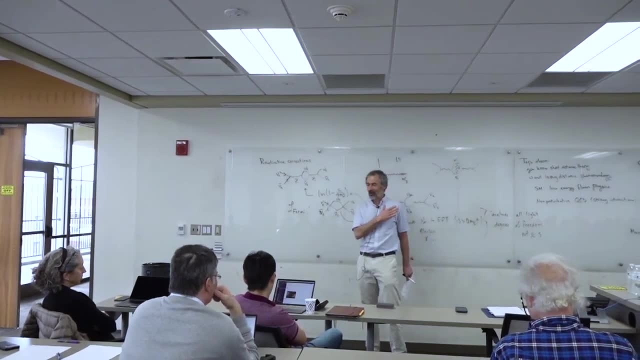 So you typically do not take many terms, Say anything beyond linear or So in this case I don't know anybody. Go on, You're going beyond the Fermi theory. I know in the strong interaction where you study meson interactions. 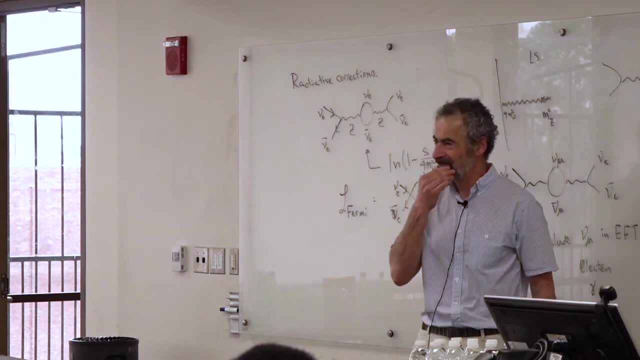 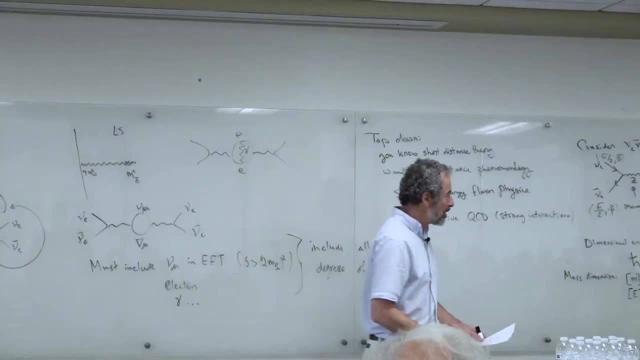 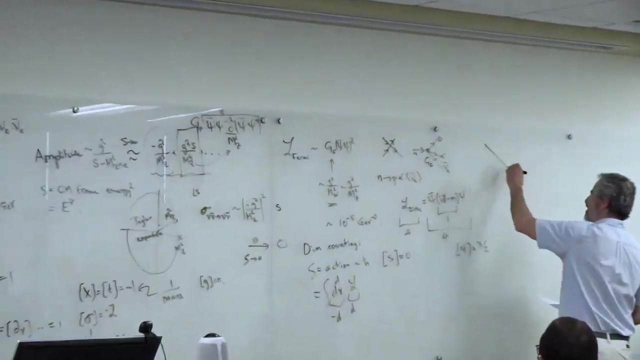 people go to like third order or something like that. Okay, So what we've learned here? is that really what an effective field theory in this case is? you're taking this interaction and if you looked at it with a microscope, that you would see. 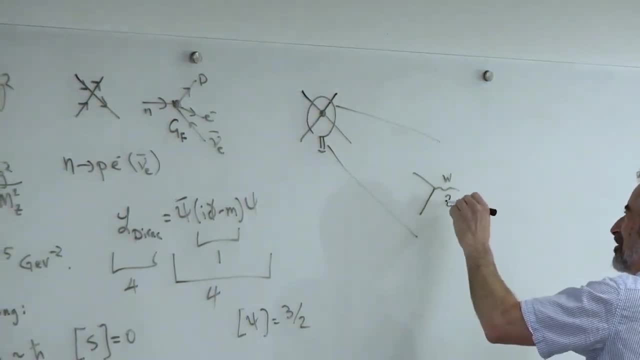 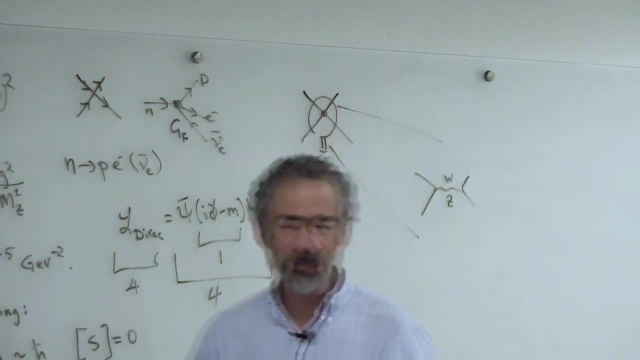 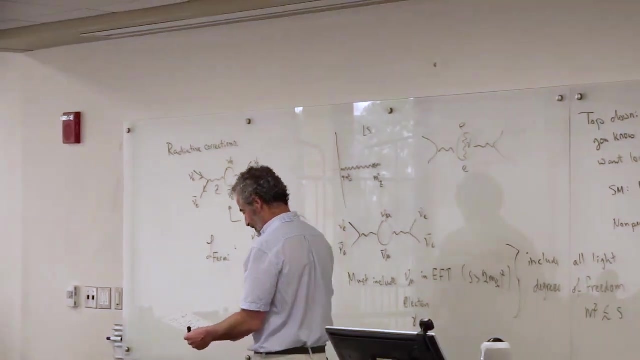 the W or the Z And we're just shrinking this down. We're saying that our eyesight is not very good. It looks like a point to us Okay, Because we're probing with low energy. You can't resolve short distances with low energy. 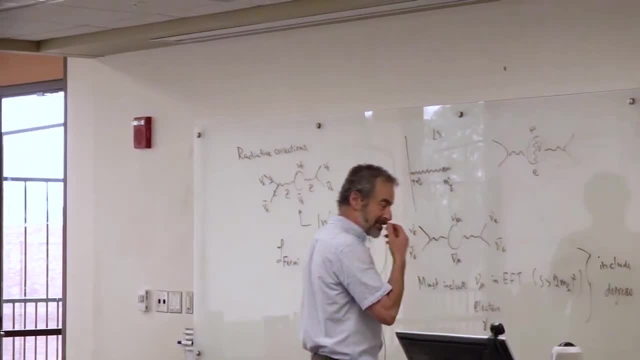 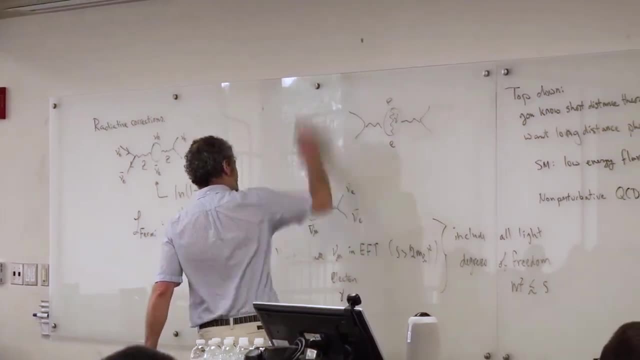 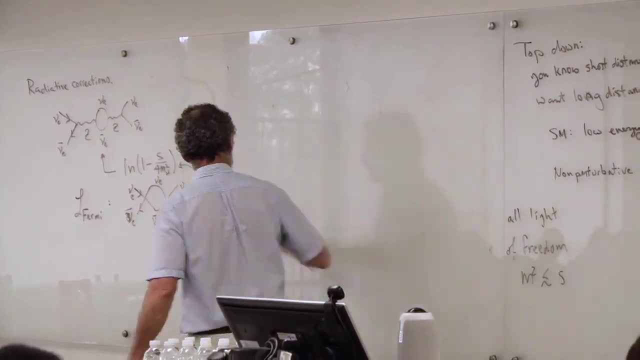 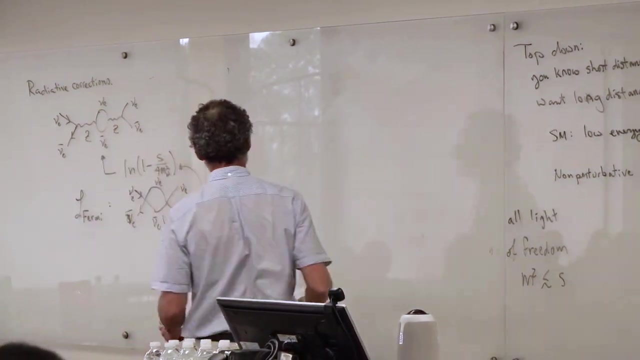 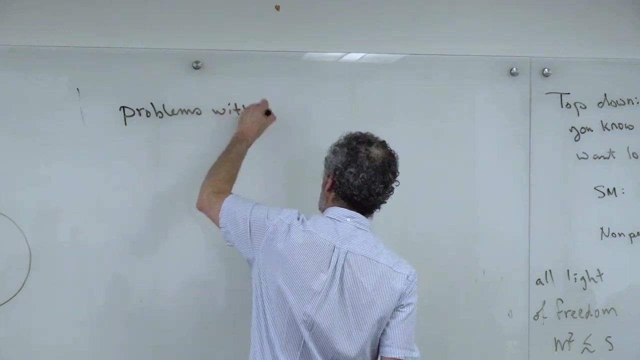 So this looks good, but it was regarded with horror by most quantum field theorists from the time Because, yes, at tree level they gave a nice phenomenological description of neutron decay. but So I just showed you that loops are fine if you included enough. 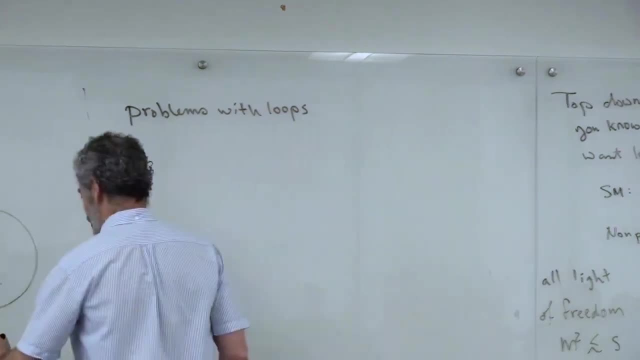 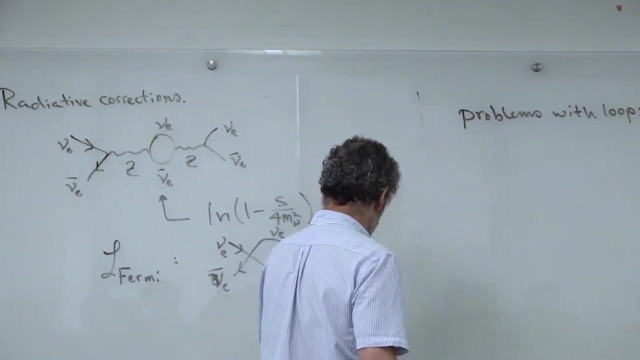 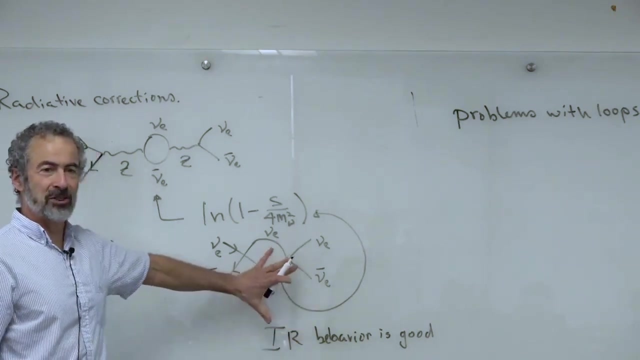 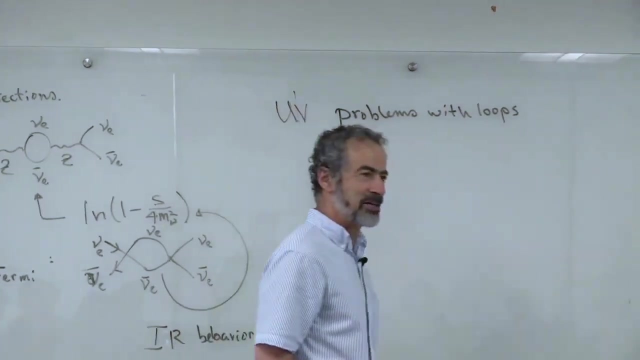 light degrees of freedom. I showed you what's called the IR behavior, which is the singularities that occur at low S, And we got that right by including all of the light particles in the world. But there are UV problems with loops, The high energy part. 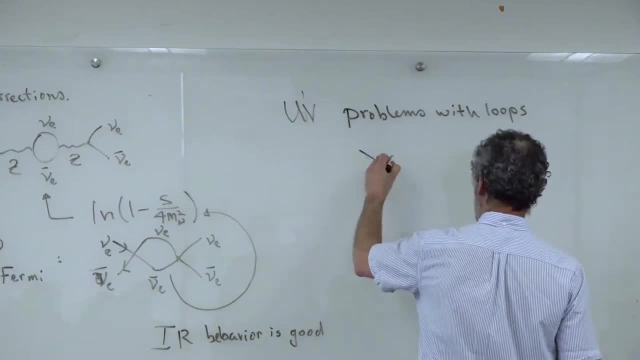 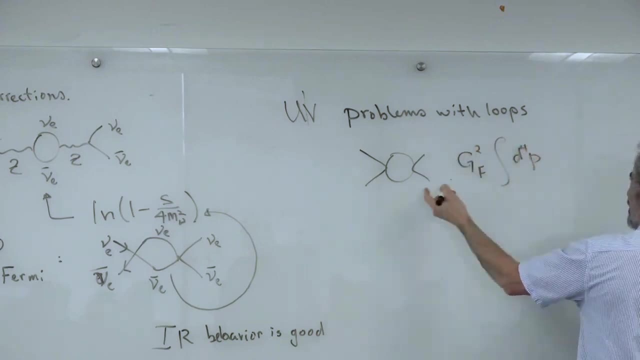 of the loop. If I look at this diagram here, I get a G Fermi squared and I get an integral before P, And then I have two propagators, two Fermi and propagators that go like one over P squared, And this is a divergent integral. 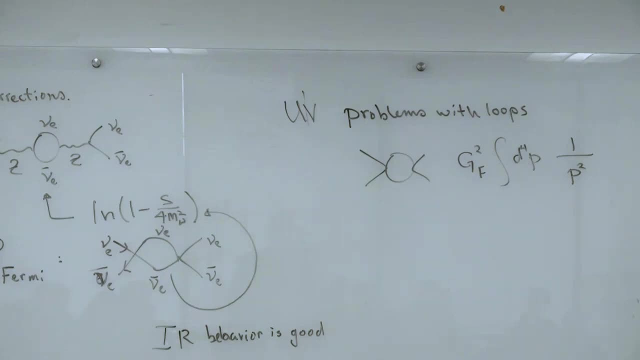 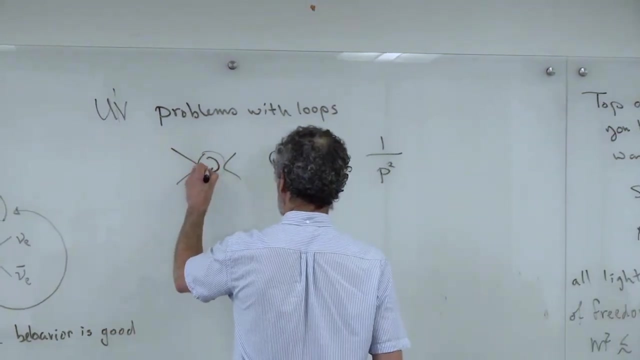 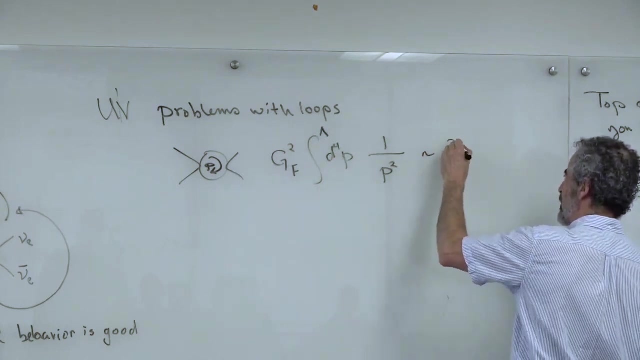 It diverges for large P, Not P near where I'm doing my experiment, But virtual P that lives inside that loop. So if I have to put a cutoff on the theory then it goes like lambda squared times, G Fermi squared, It's infinite. 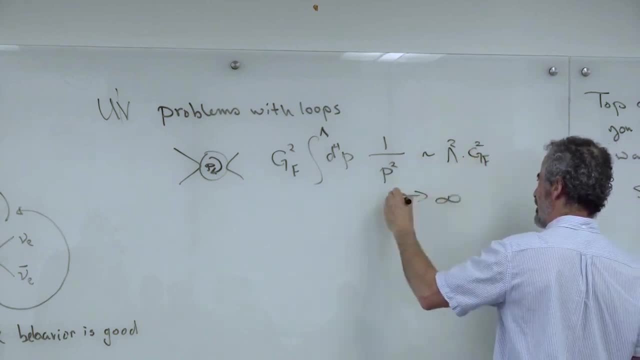 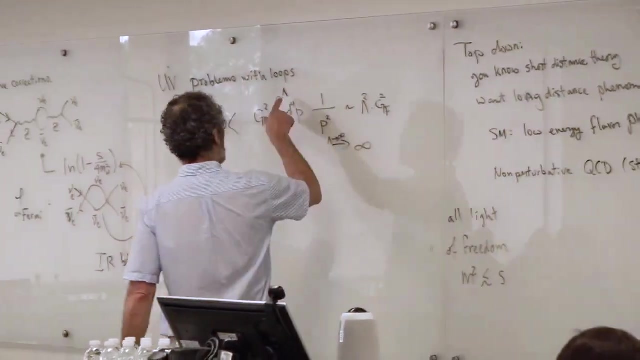 as I go to, lambda goes infinity. Lambda's not real, I shouldn't have to keep it finite. So the Dirac's generation thought you had to have all your cutoffs go to infinity, or else the theory really didn't make sense. So this is called 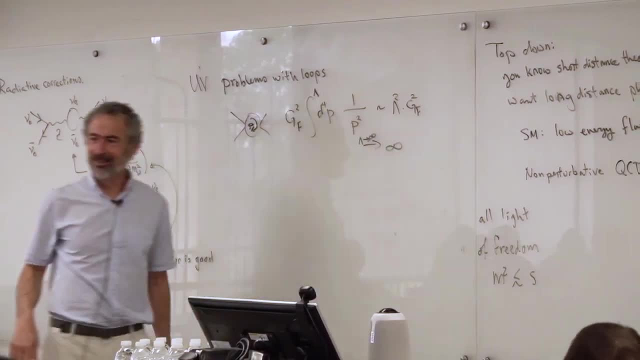 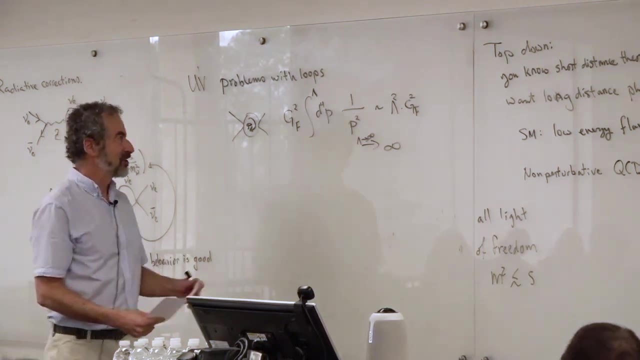 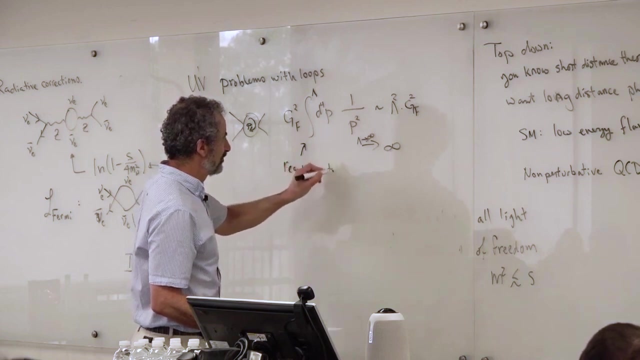 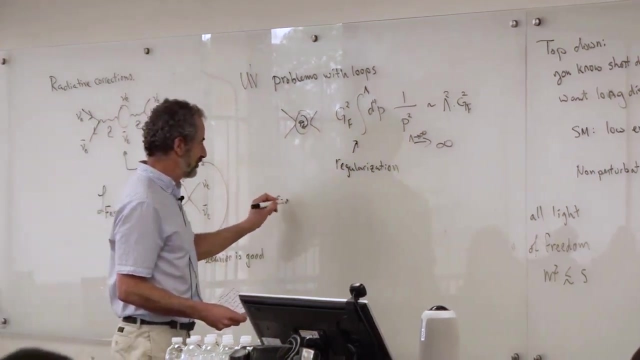 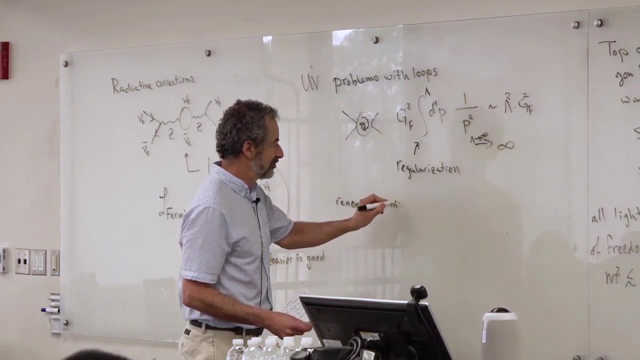 regularizing the integral, which is a fancy way of saying: kick the integral until it's finite. So the next stage is this is regularization, and then there's renormalization, This short distance behavior- remember I said that when you're at high momentum. 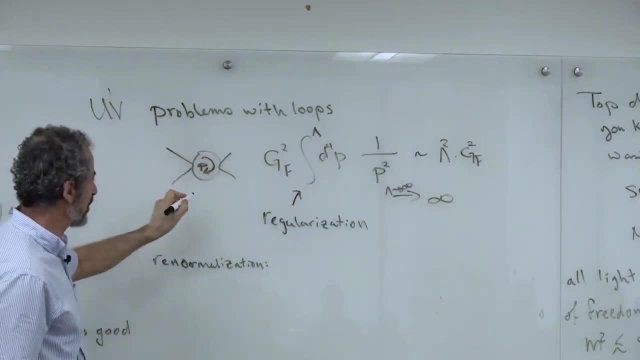 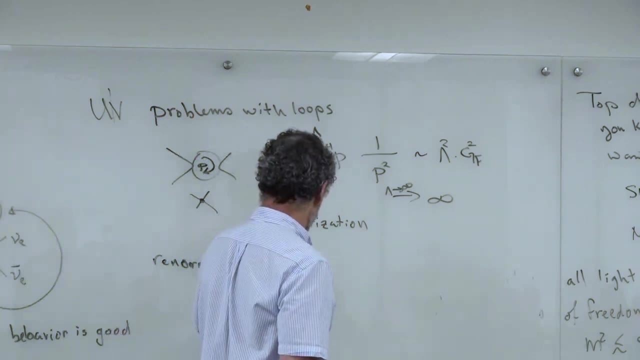 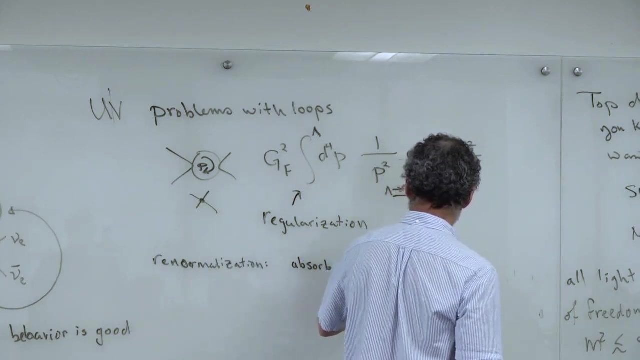 everything looks like you're at very short distance. So we're talking about short distance behavior, where this looks again like that. That looks a lot like the Fermi interaction. So you absorb into the Fermi interaction. So you say that G Fermi. 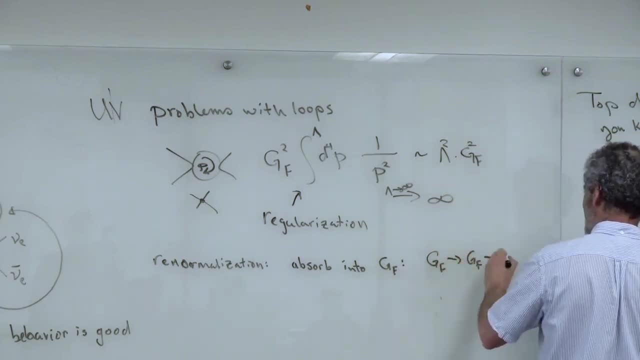 goes to G Fermi minus G Fermi squared- lambda squared, so that you have a piece at tree level now which cancels off some of the energy. that's there, And what's left over is something finite that you can then measure in the lab. 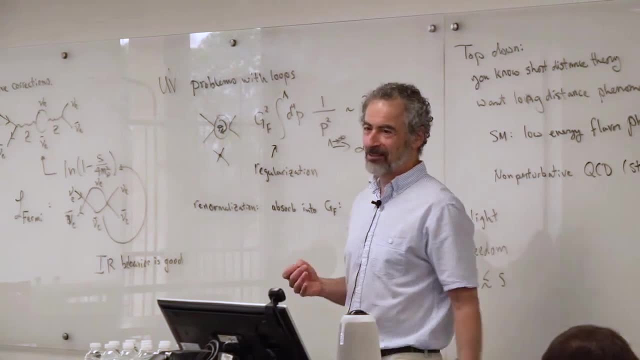 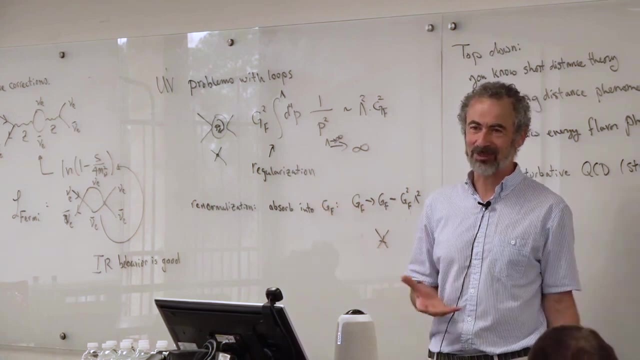 So this looks sort of revolting, but you actually see this in classical electromagnetism too. If you try to calculate the mass of the electron, including the energy in the electric field, it's divergent, because the electric field goes infinity fast near the electron. 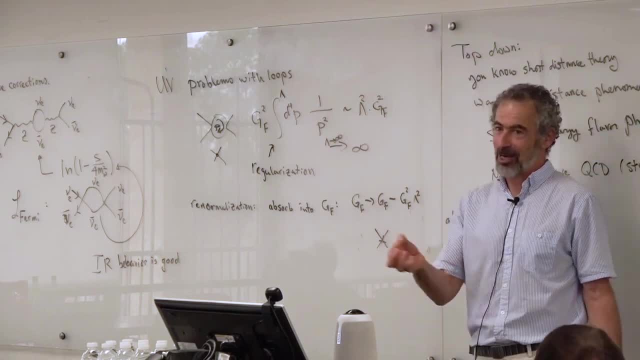 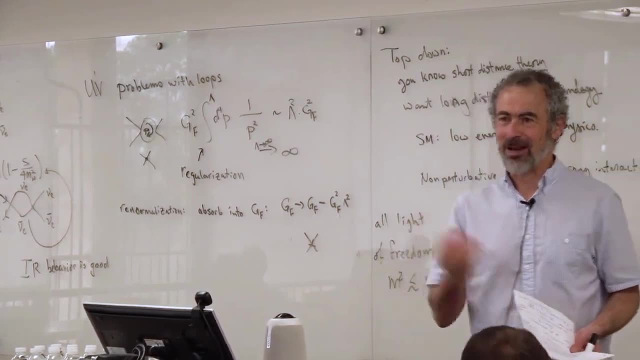 So you have to say: well, okay, I know, I can move an electron. It doesn't take an infinite amount of energy to budge it. So somehow this electromagnetic energy can bear energy which has to be negative to cancel it out. That's sort of weird. 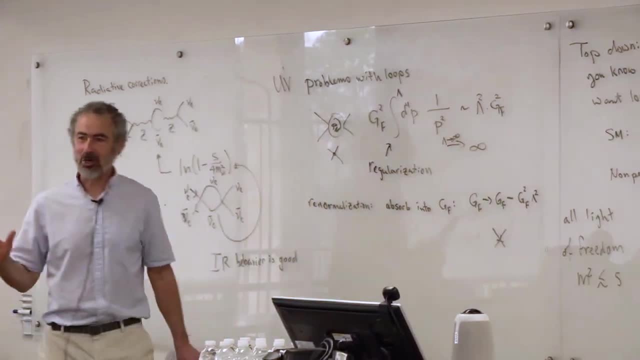 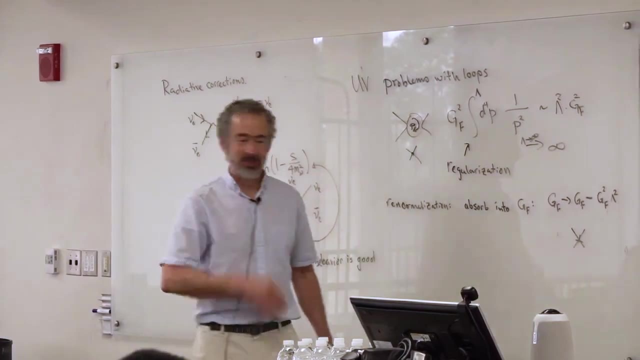 but okay, It's got to be an artifact of how we're calculating things. It can't be a property of nature. So we say we're doing something weird with this perturbative expansion and we have to do tricks to make it work. 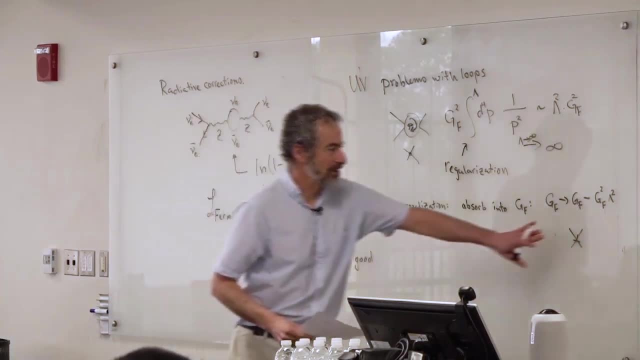 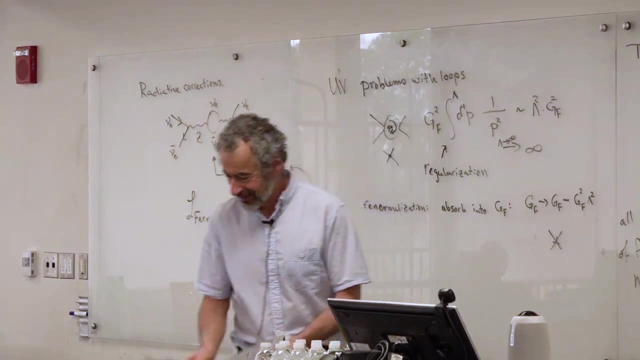 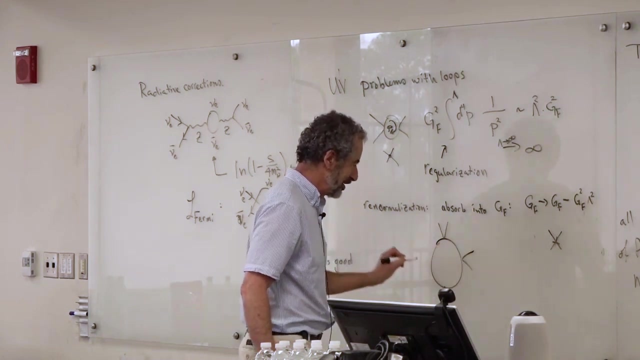 But we can make it work. We can absorb this graph into G Fermi and continue our work, But there are other graphs in the problem. So if I look at this loop now, I have integral d4p times 1 over p to the fourth. 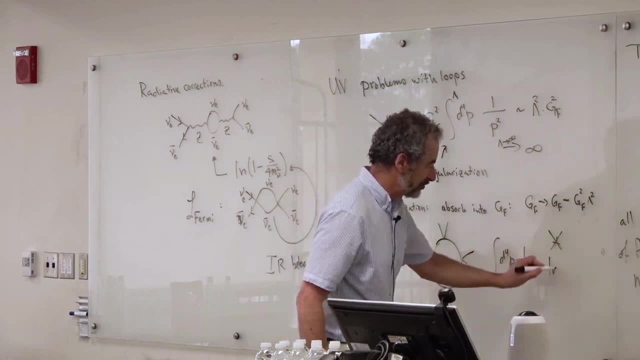 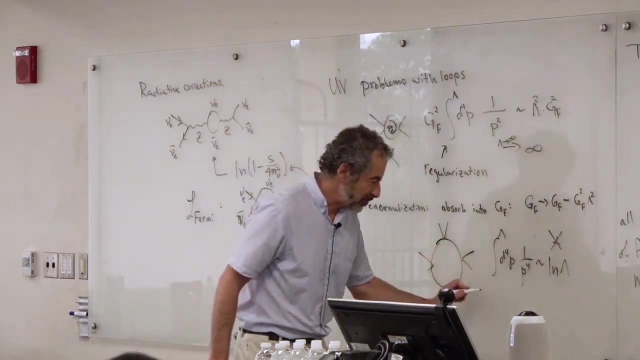 that is still divergent. It was like the log of lambda And this was. therefore it requires a counter term, an interaction that looks like that in the Lagrangian to absorb that infinity. Well, I hadn't wanted to put that in. 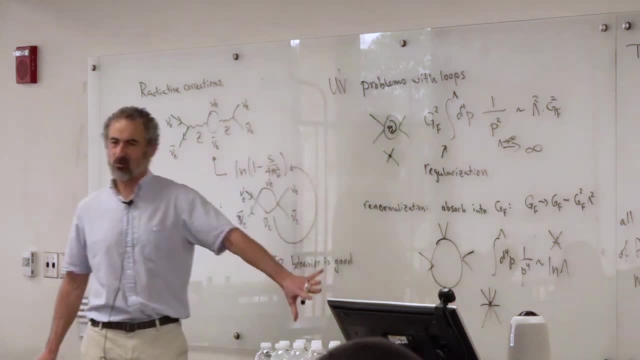 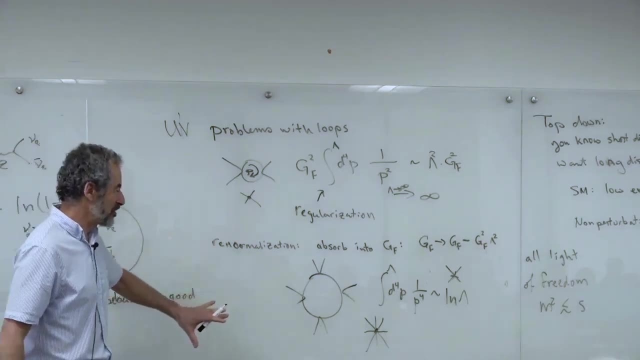 I was never going to do the scattering of infinity in the Lagrangian. I was just going to do the scattering of four neutrinos off four neutrinos, Or four neutrinos off each other. But this says I need to have that interaction. 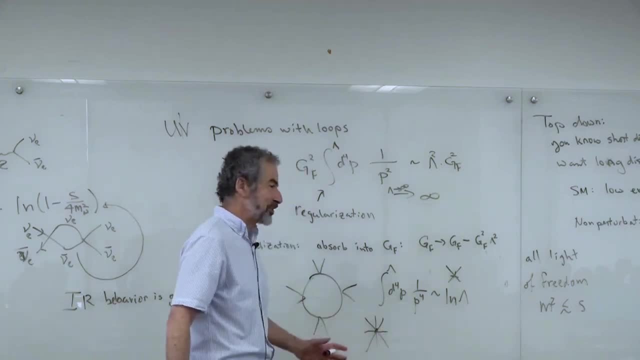 in my theory, if I want to make sense of my calculations, So I throw this in. I don't know how to measure the finite part, though, So I don't know what to do with this, And then you start sticking this in graphs: 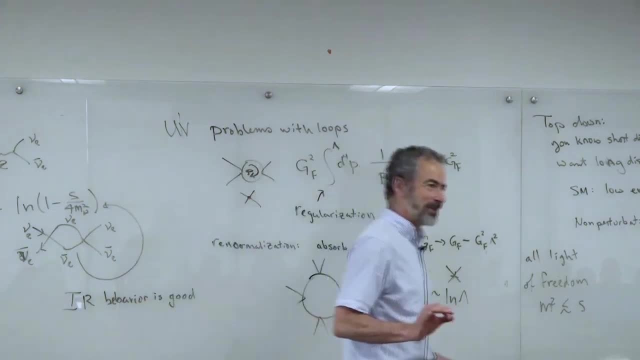 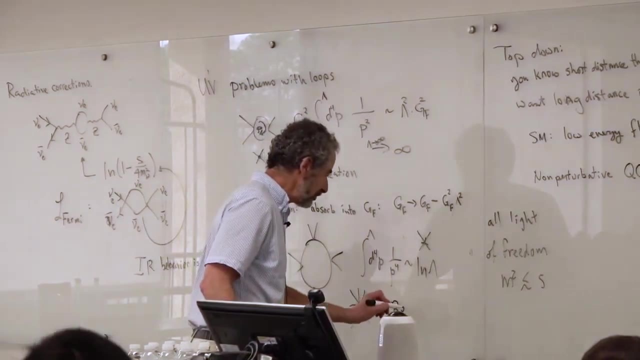 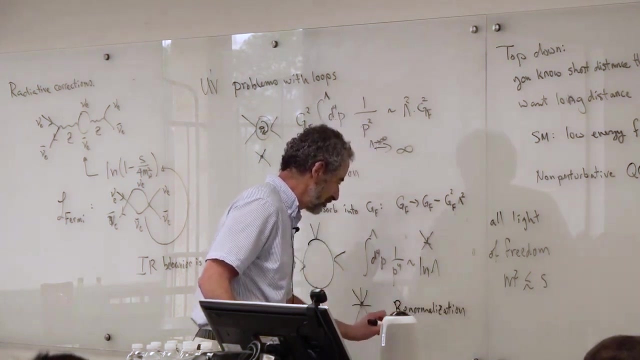 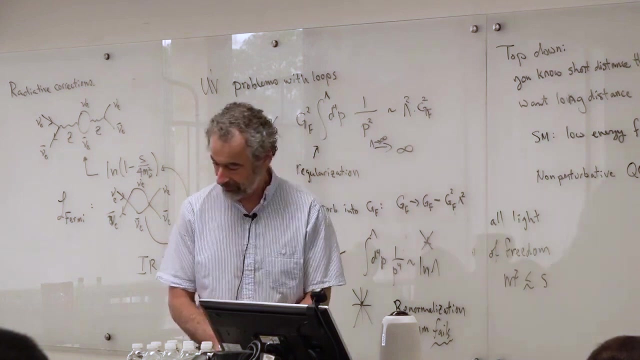 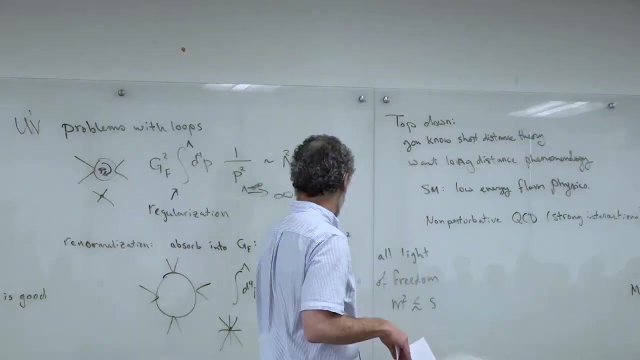 and you generate more and more, And pretty soon you're going to be able to do experiments in order to fix their values. So renormalization fails And you can see that the problem is not from the fact that I have a coupling constant. 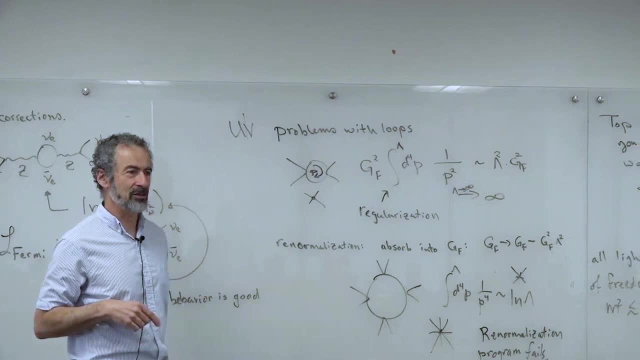 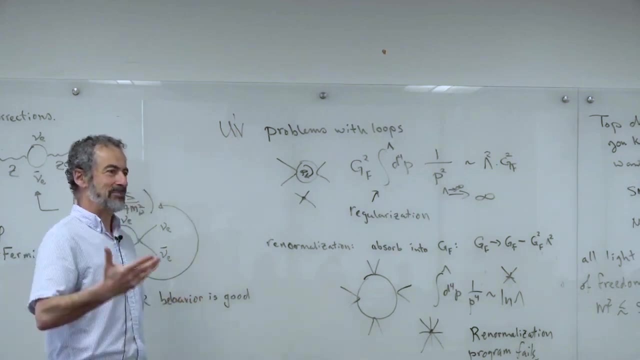 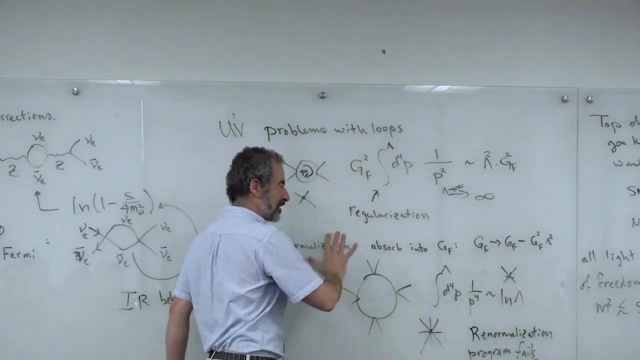 here that goes like inverse dimension, because the more interactions I include, the more powers of inverse mass I put in and the more powers I'll get of lambda upstairs to get the dimension right. And so high powers of a coupling like G Fermi will lead. 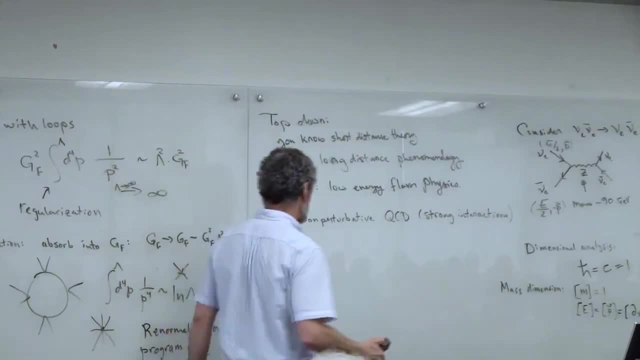 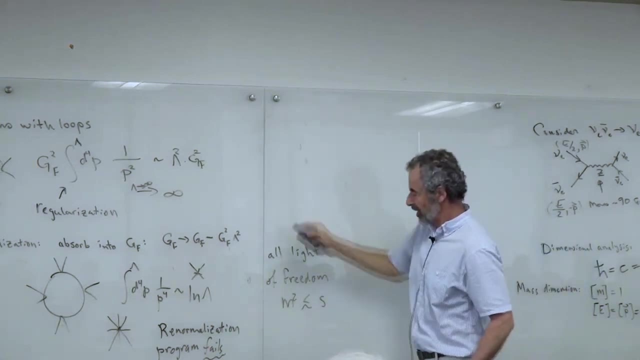 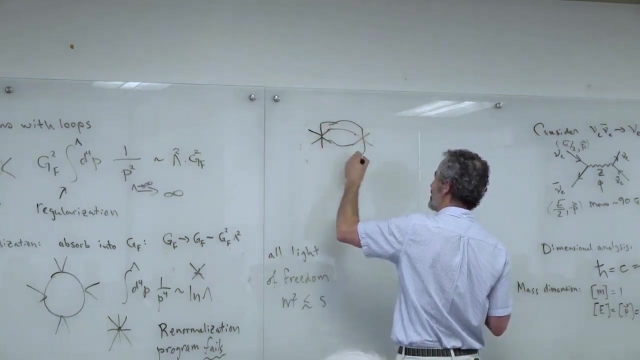 to high powers of lambda typically, Or high powers of lambda will lead to high powers of lambda. So if I took my that one of these, an operator like this, and I tie these graphs, these lines, together, well, this, this came from psi bar. 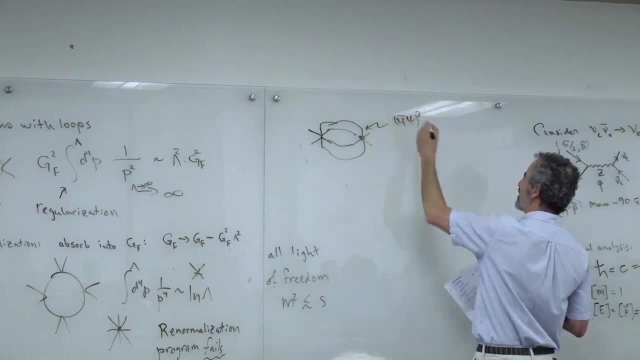 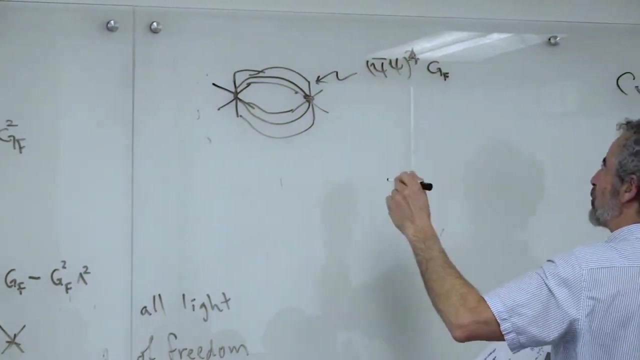 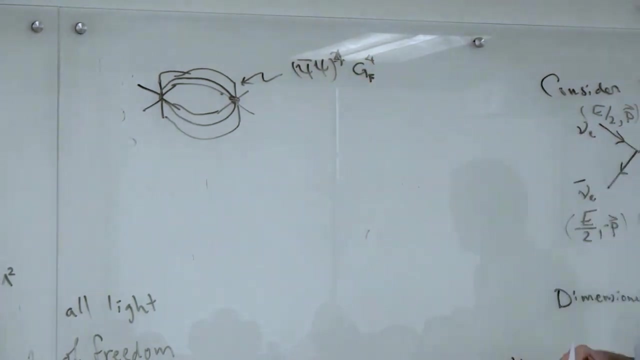 psi cubed interaction, which is what we would have to do if we were to have something like G Fermi. let me put an extra one, so this would be fourth, which is dimension 12. so I'd have to have G Fermi to the fourth out in. 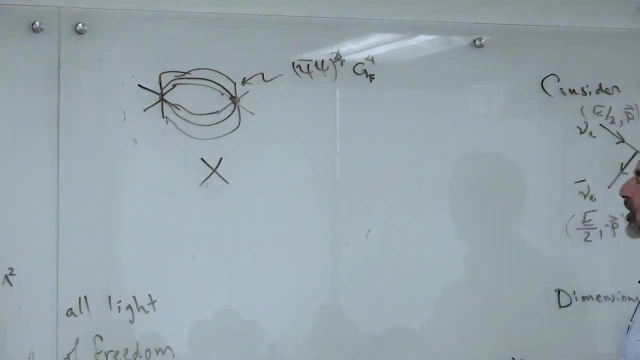 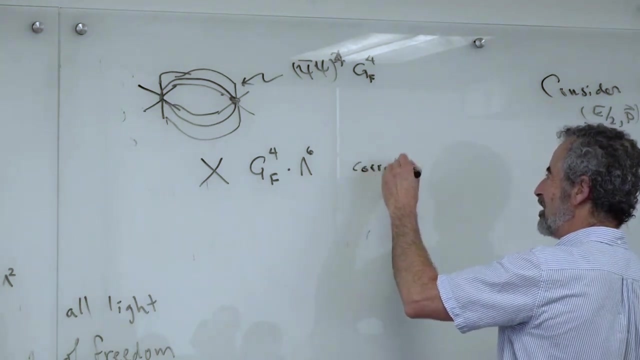 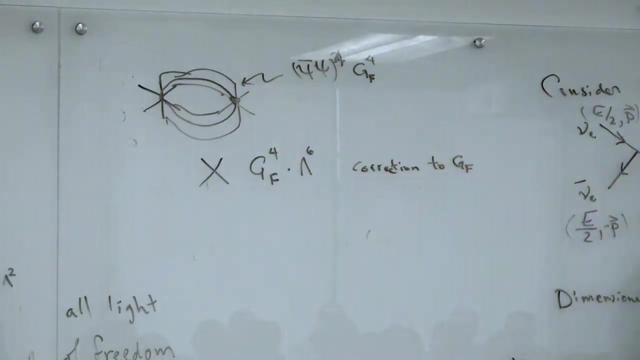 front to get the dimensions right. So now this looks like a lambda to the sixth out in front of it in order to get the dimensions right, because this has to look like a correction to G Fermi and you see that getting operators with many external fields. 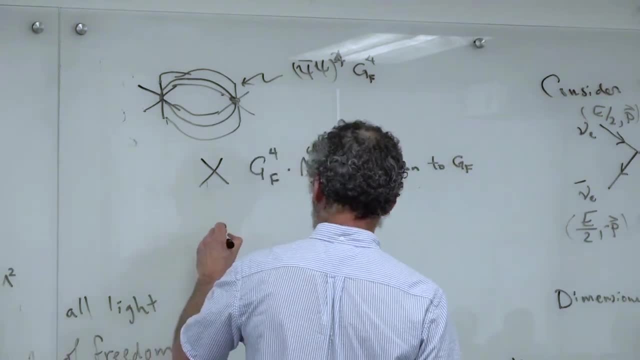 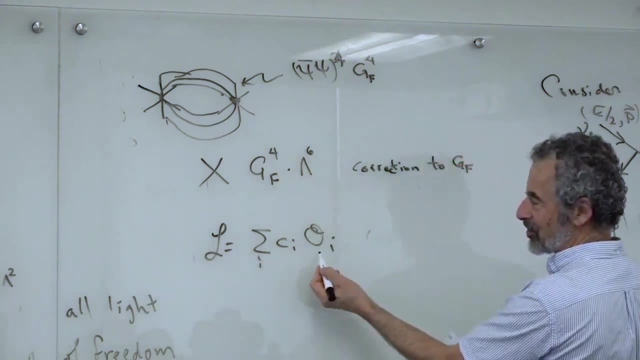 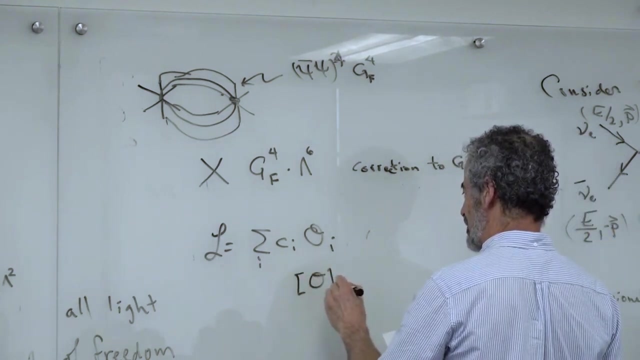 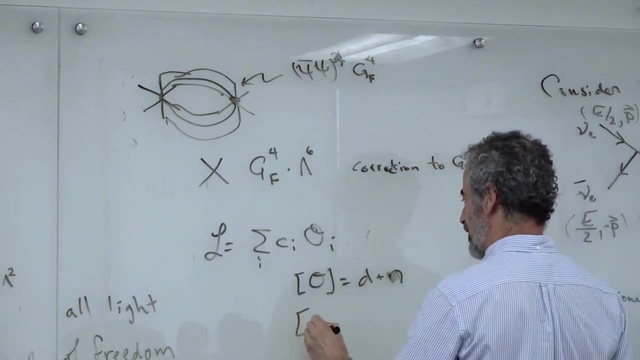 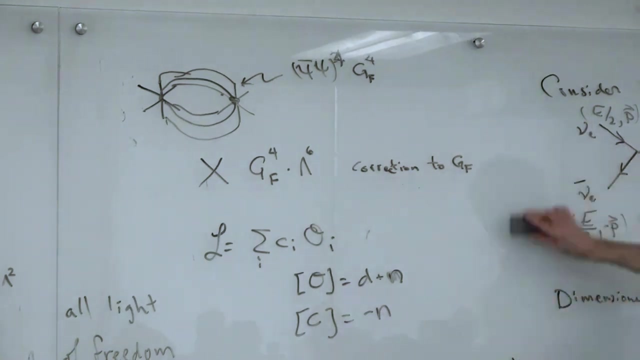 is bad because it feeds back to the low dimension operators, times, coefficients. so these are numbers, these are, or these are, the coupling constants and these are the operators. and if I say that the operators dimension is D plus little m, let's say little n, then the dimension. 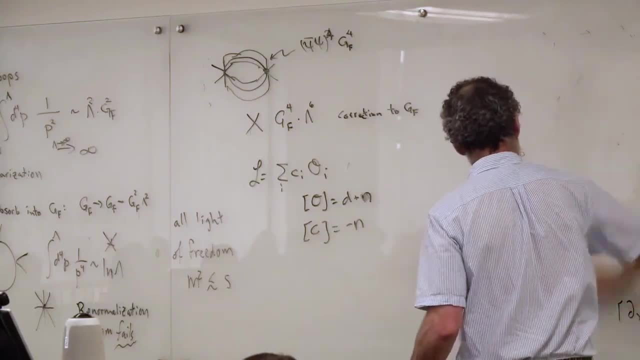 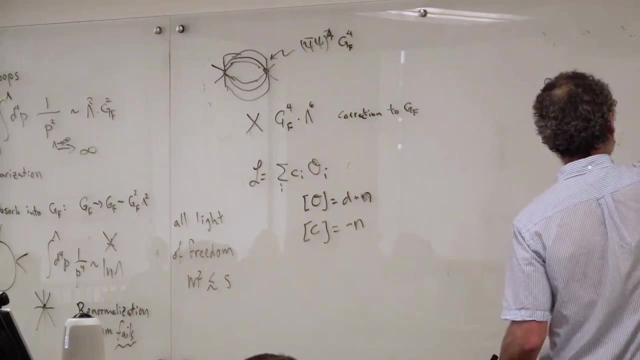 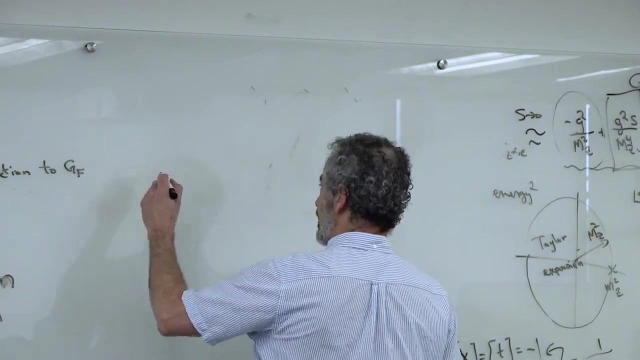 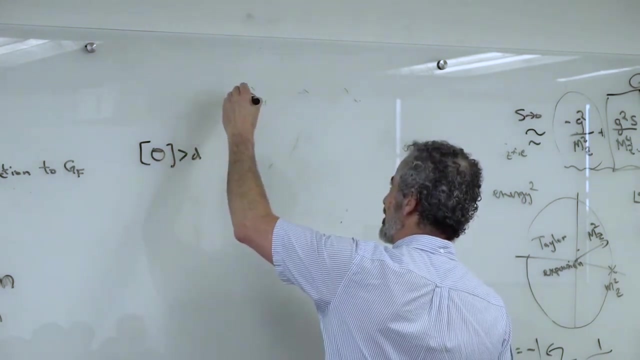 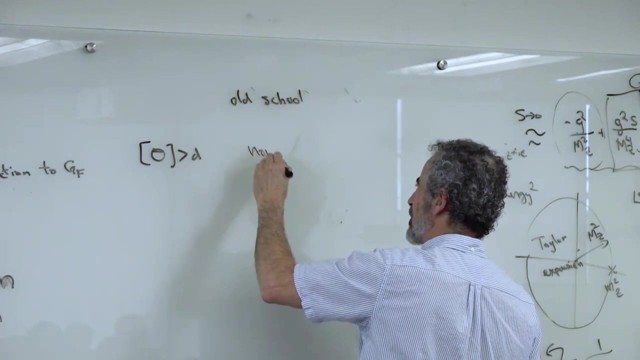 of C or zero or negative are going to have different behaviors, where when the dimension of C is negative we have problems with renormalization. so if we have operators with dimension greater than D, the old school discussion of this is non renormalizable, but the new 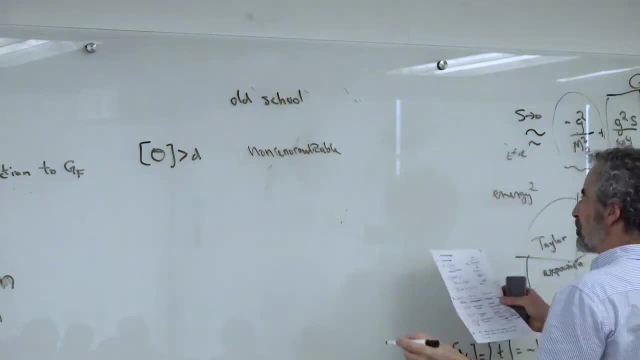 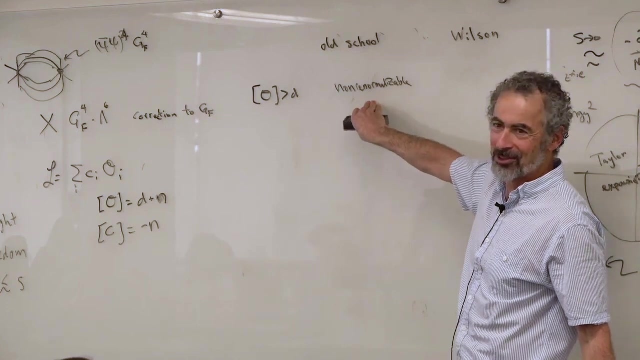 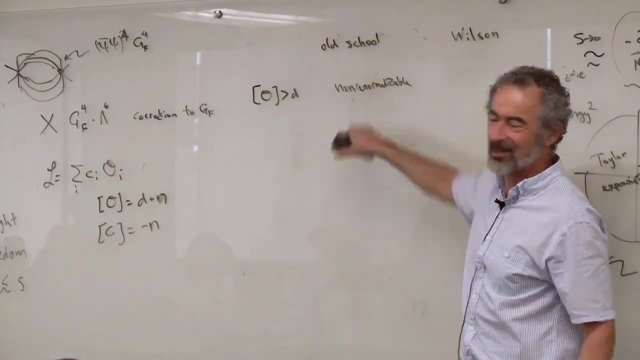 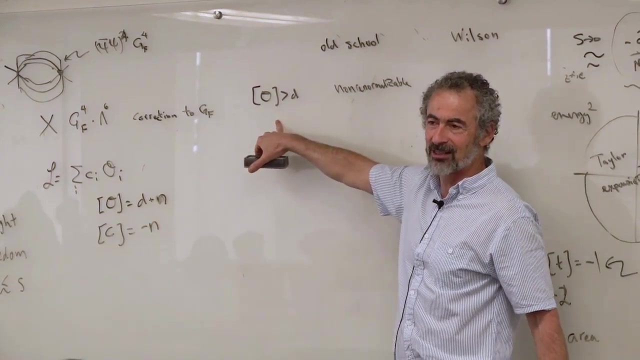 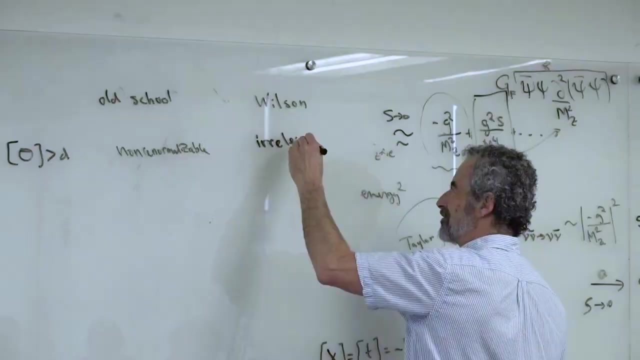 school, which is largely due to Wilson. Ken Wilson says this is sort of foolish. when you say non renormalizable, you're looking at the low energy stuff that's important. we've seen that for high dimension operators like the family interaction, which is dimension six, it is. 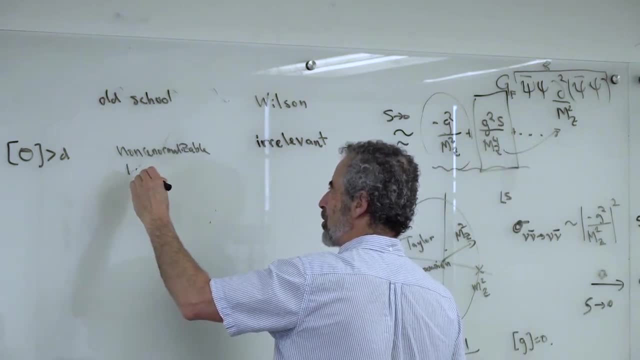 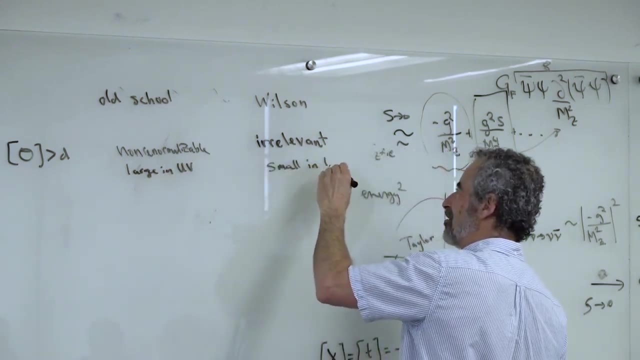 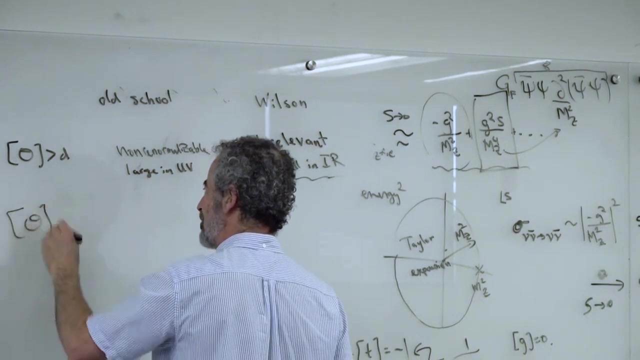 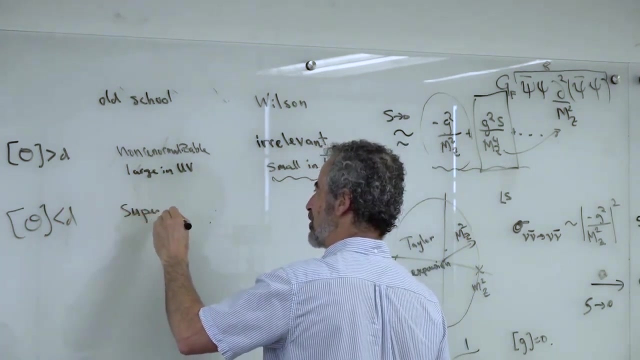 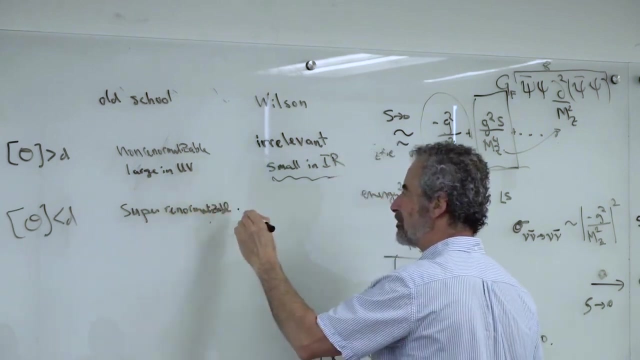 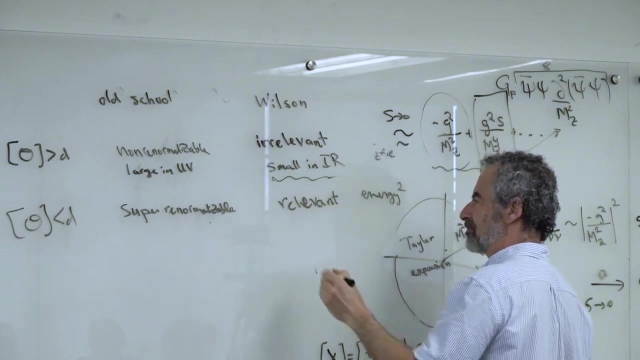 unimportant at low energy. so he says: focus on the dimension, and this is what's important. if you have an operator whose dimension is less than D, the old school picture was that this is super renormalizable and very good, and, as I'll show you later, 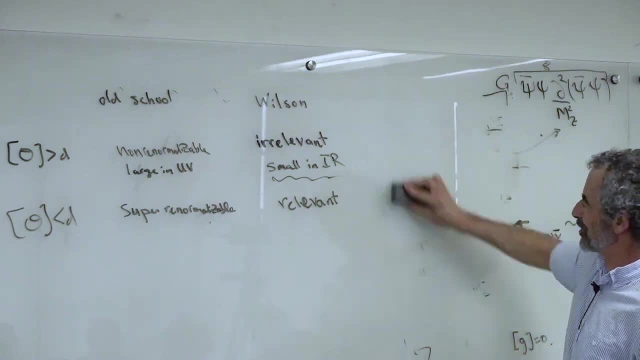 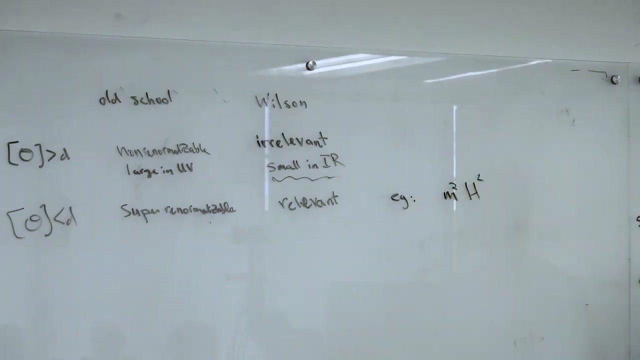 this is actually considered a problem in Wilson's theory, these things. an example: we've talked about irrelevant operators in the fermion interaction, but an example is a scalar particle of dimension one and it's got a mass squared in front of it. why is that bad? well, 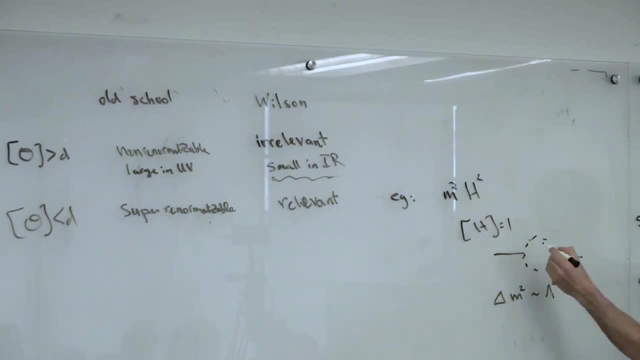 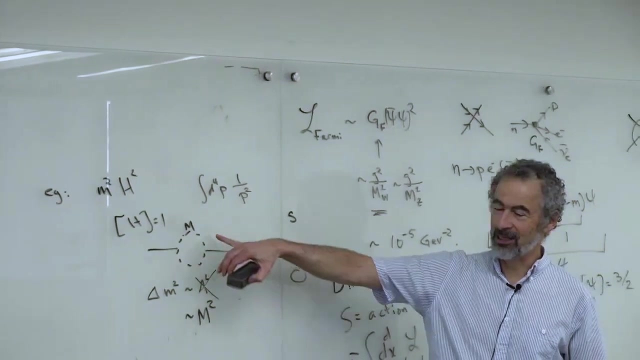 if I take this Higgs boson and say p squared if that's a fermion, so that looks like it blows up quadratically with the cutoff and this is bad because even if you renormalize, the finite part should be: if this is a particle. 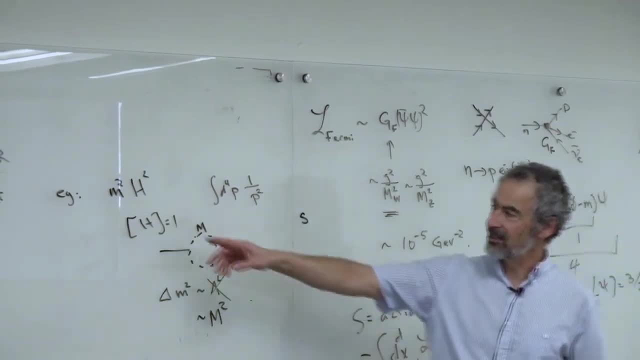 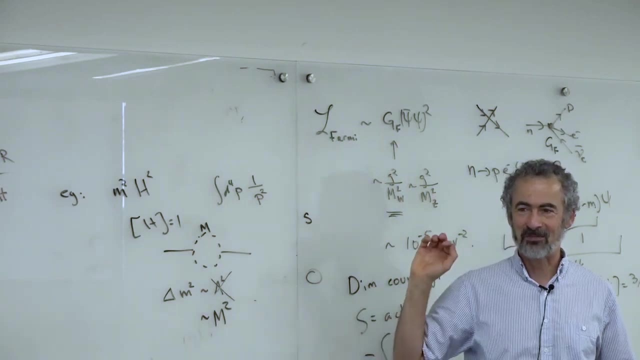 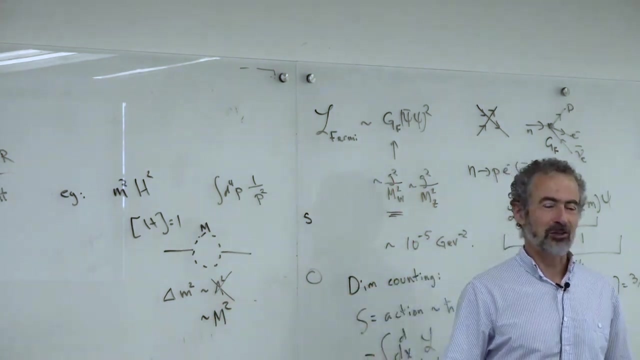 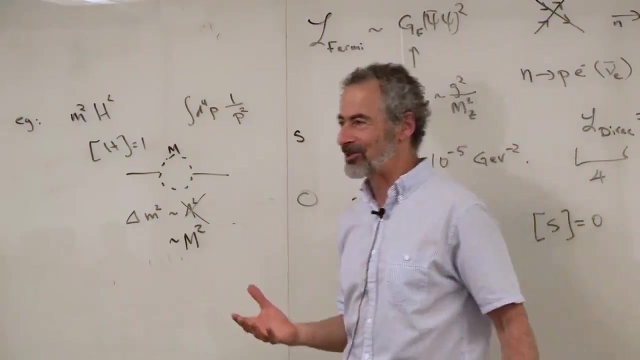 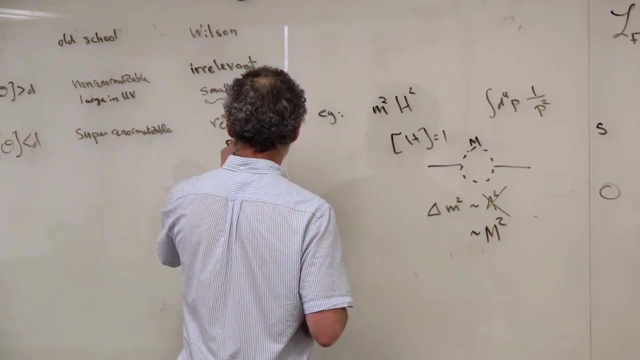 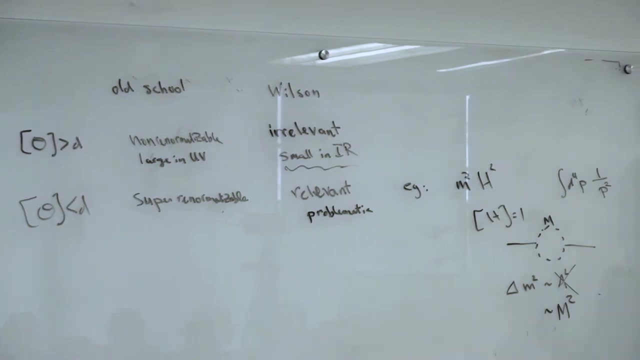 of mass M. you then even it's sort of like- and you know that the theory has heavy degrees of freedom in it- like, say, you believe that there's a gut or something with mass, a constant, and even worse example is the cosmological constant. that's the. 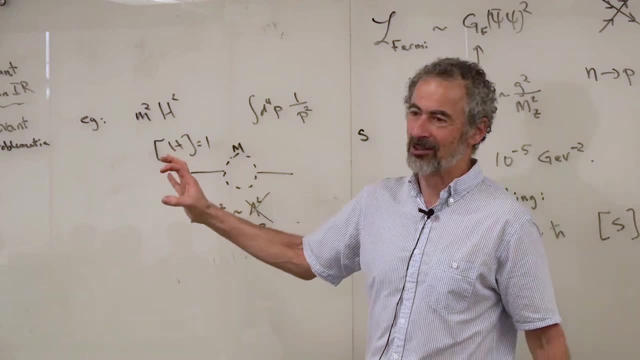 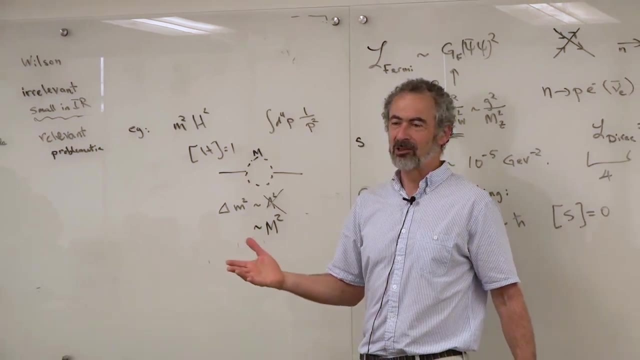 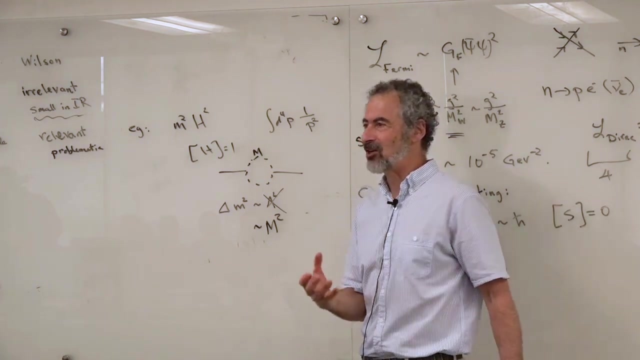 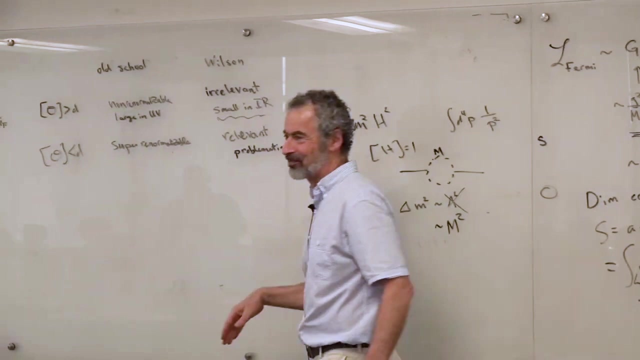 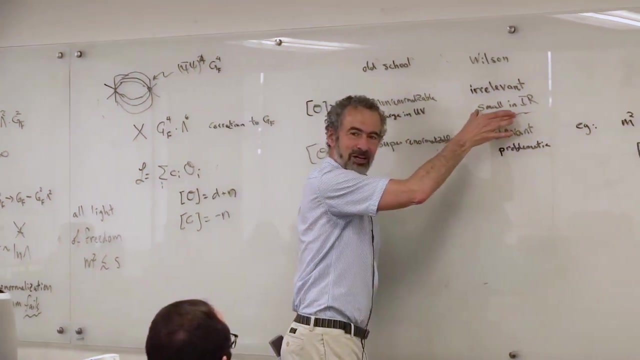 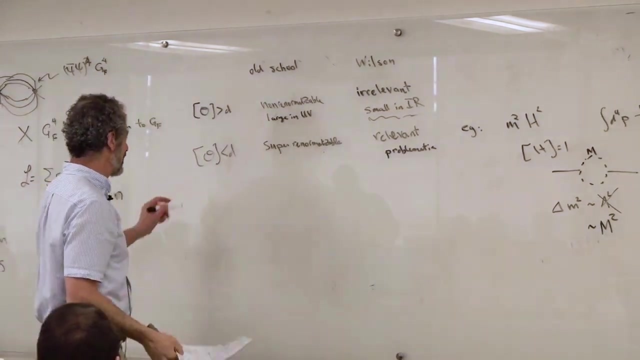 operator one. it's just, it's a number you add to the Lagrangian and normally you'd say, well, I don't have any particles, like we know of particles that go up to, like you know, 170 GeV for the top quark. so it's. 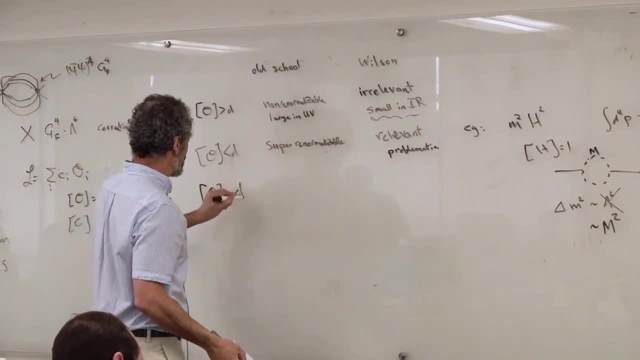 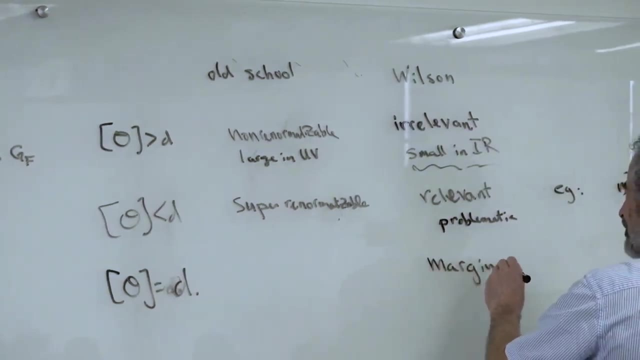 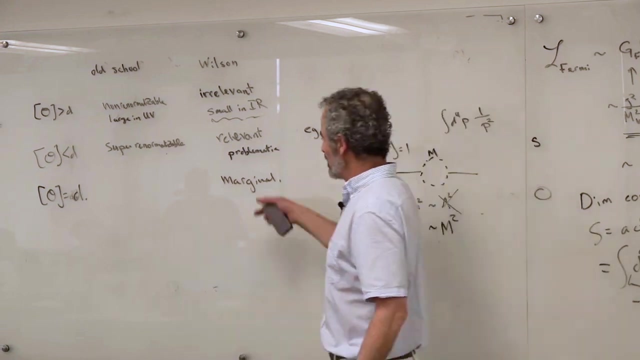 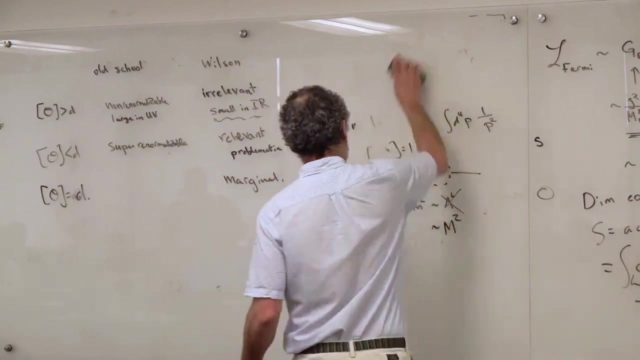 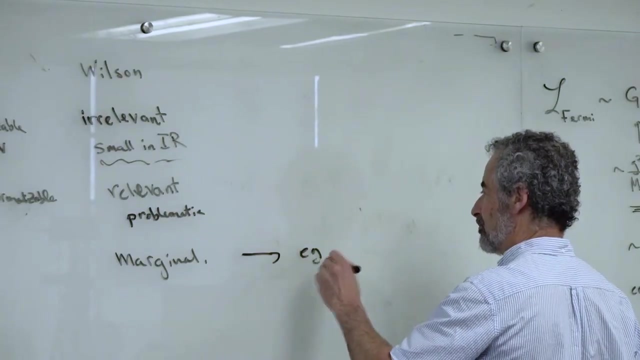 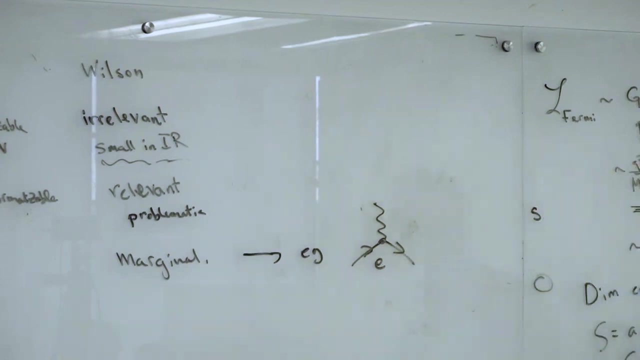 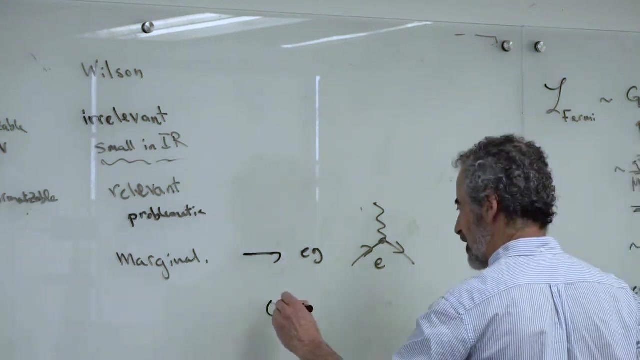 been turned on its head, these operators which are called marginal. marginal means we don't really know if it gets more important or less important in the IR. naively it stays equally important. so an example would be this: electric charge is a number which doesn't have dimensions. 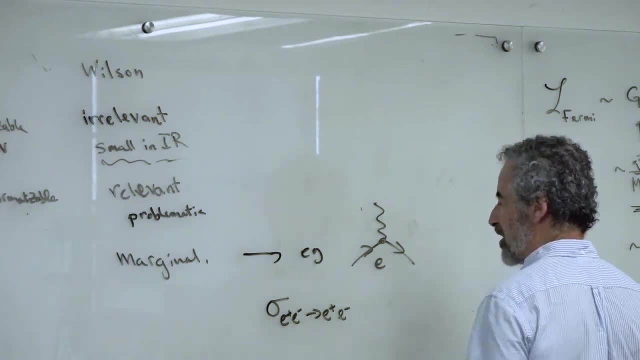 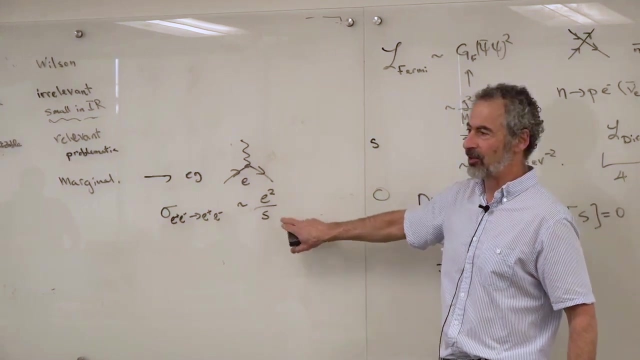 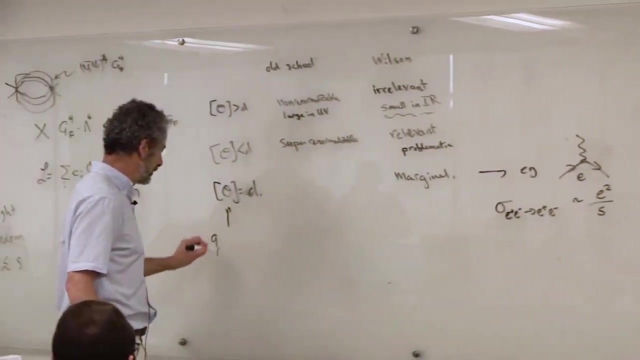 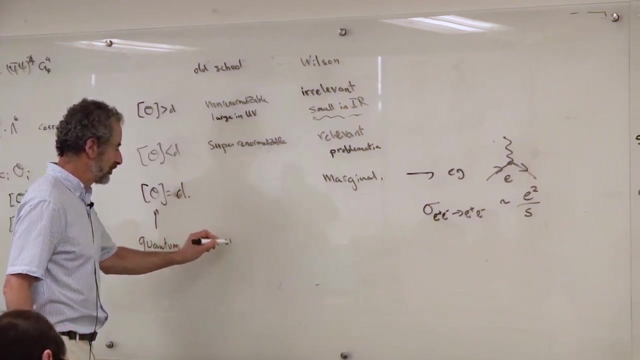 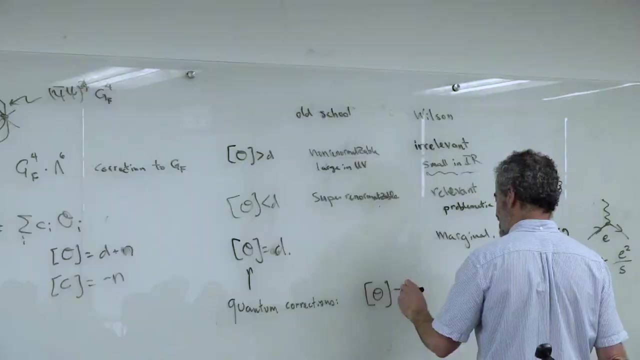 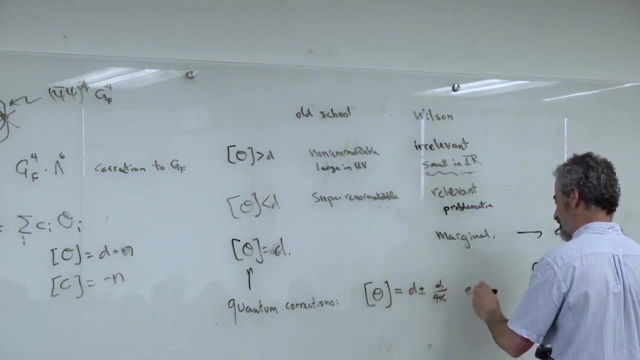 and you look at the cross section, then for say, E plus E minus goes to E plus E. but when you look at quantum corrections they actually change the dimension of the operator and if you're in a perturbative theory might be something like alpha over four. 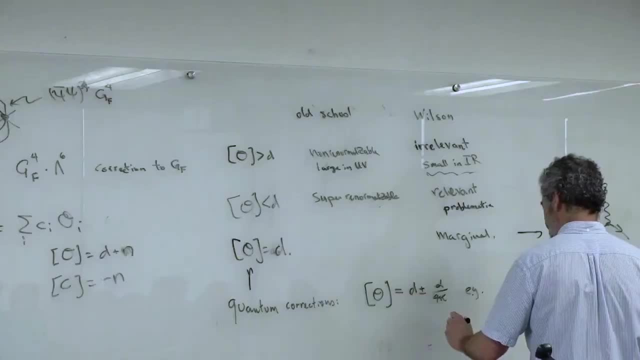 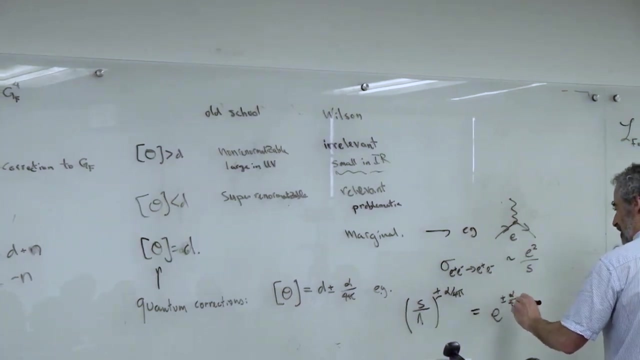 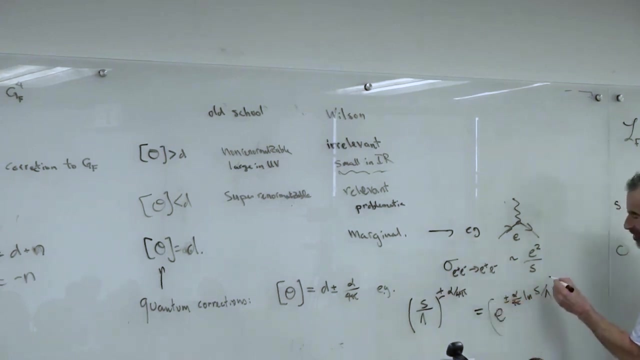 pi. what's its sign? so now I'm going to get an extra factor in my Lagrangian which looks like S over lambda. my cutoff to the plus or minus alpha over four pi log S over lambda. so I get this extra factor multiplying my cross section. 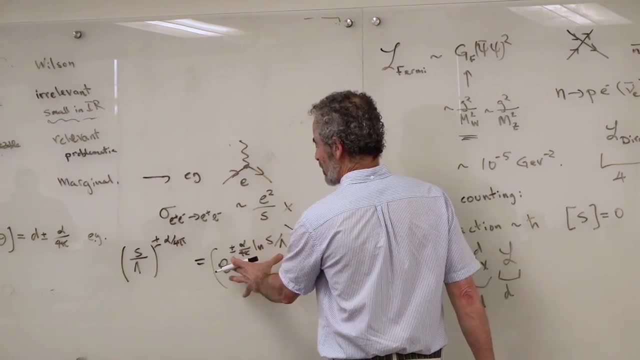 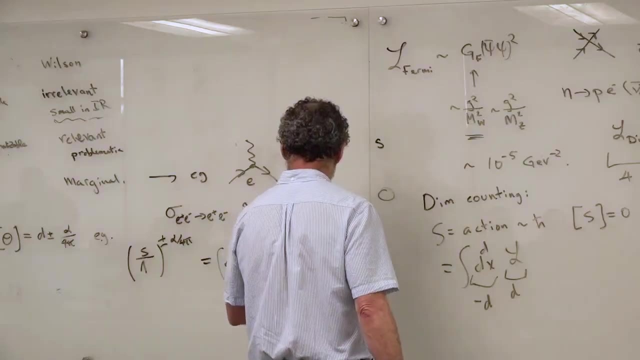 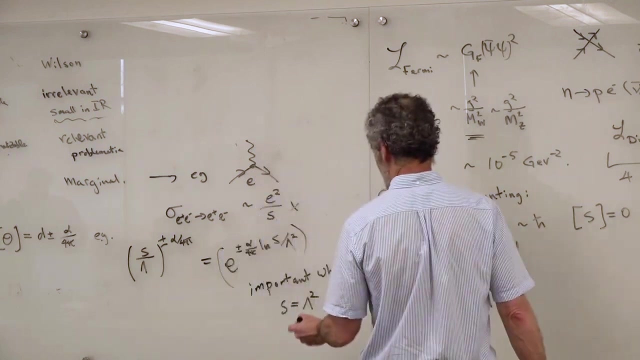 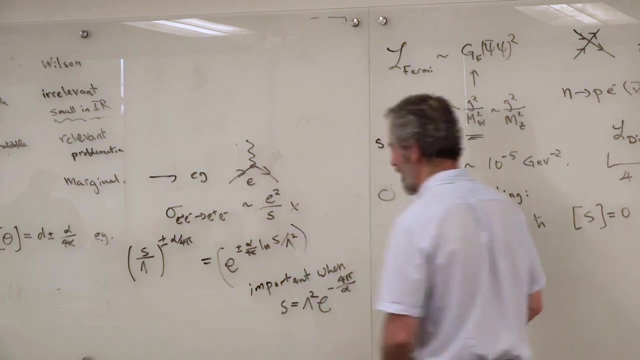 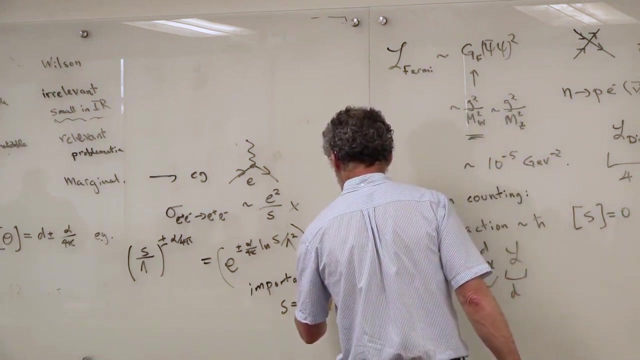 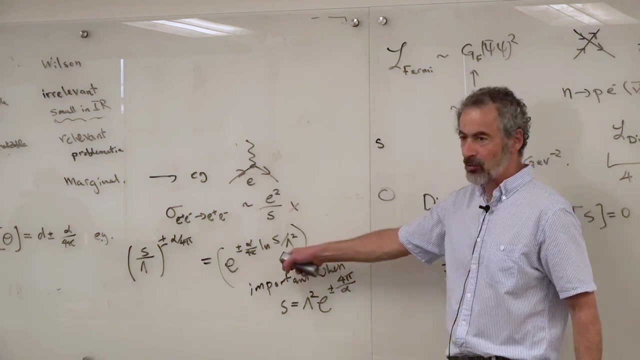 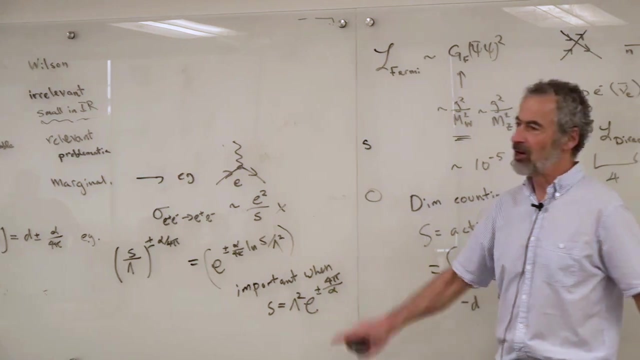 well, this becomes important when you have a very big- this is squared sorry- when you have an exponential hierarchy between your cutoff and your energy- and I should have put in a plus or minus here and maybe there's cutoff, say the Planck scale. we know we don't. 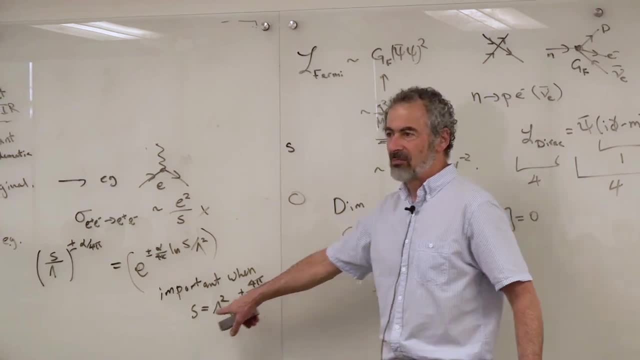 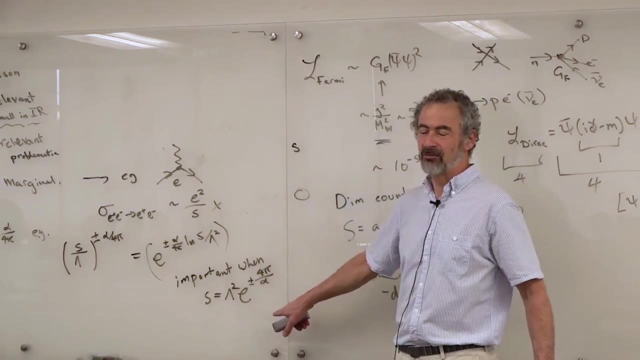 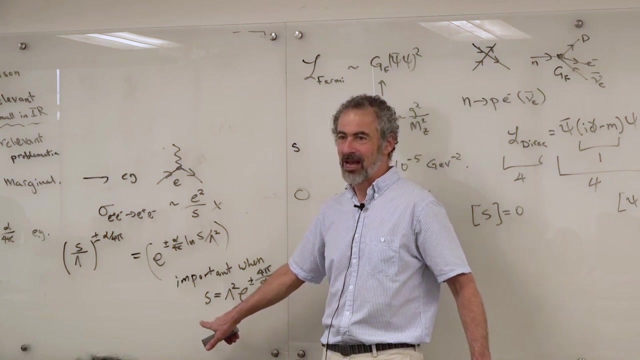 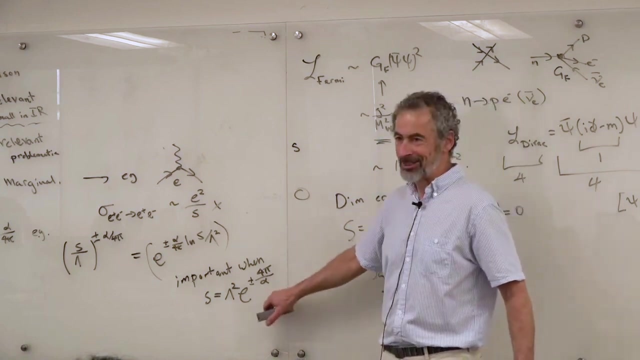 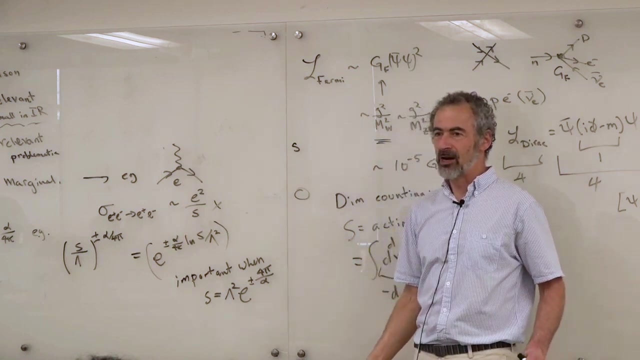 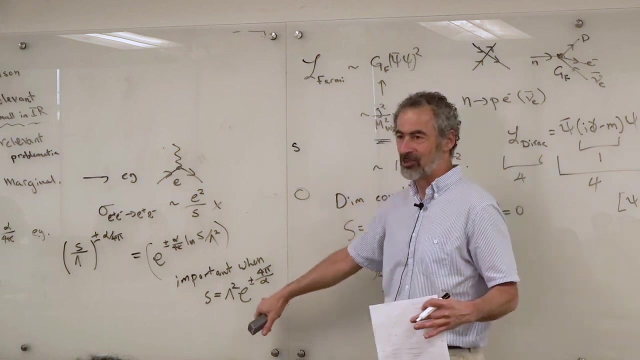 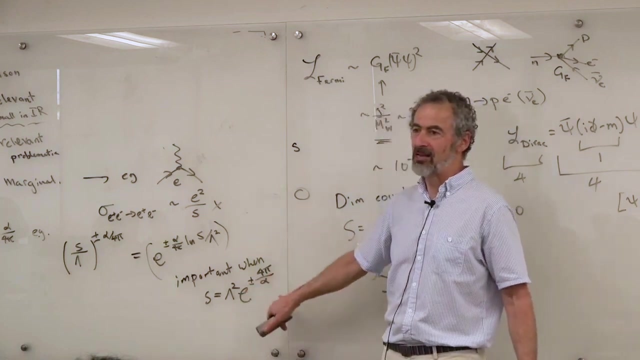 know, understand quantum gravity. we're not going to take our integrals above that. well, if I had a minus here, then this would tell me that I could have a very, very low energy, and this is really cool because it tells you you can start from a weak. 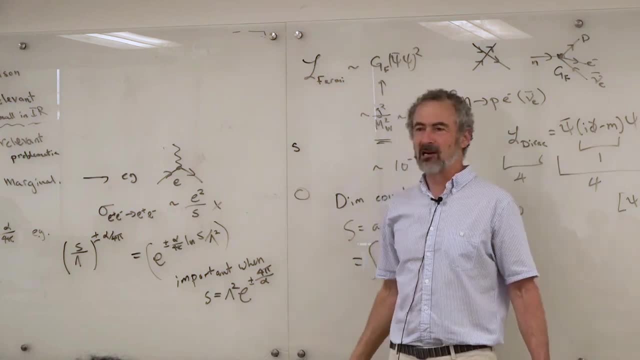 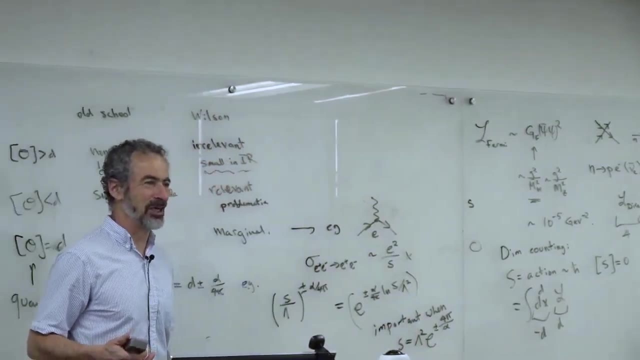 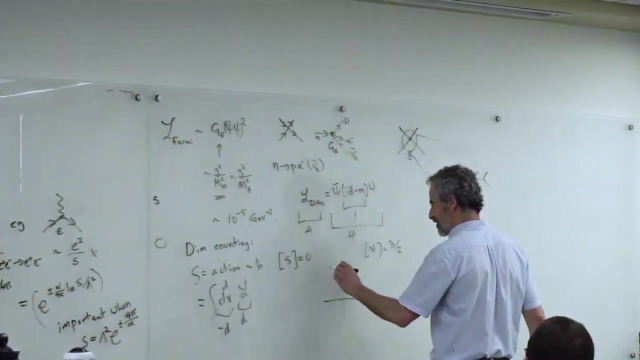 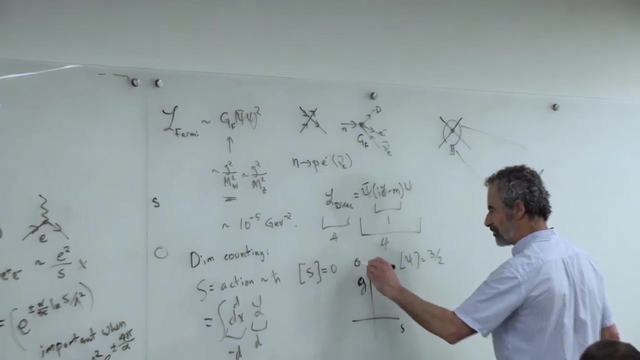 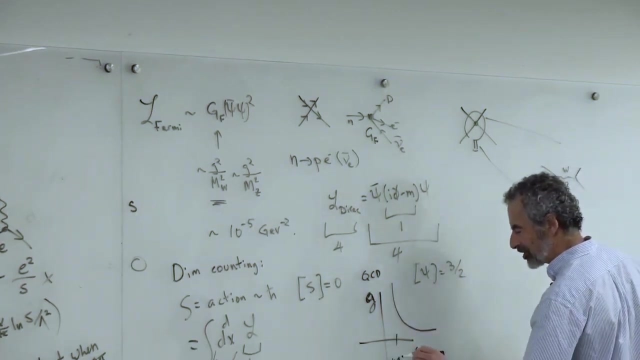 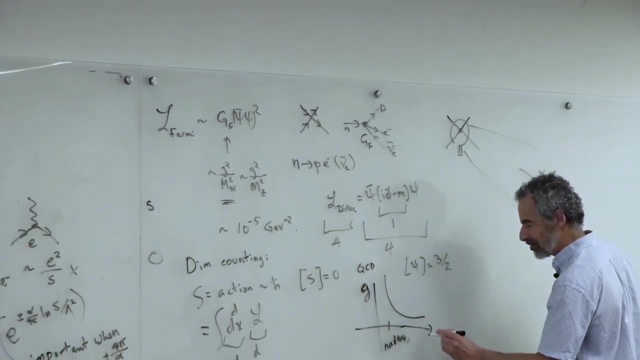 theory at high energy, and for people like Dirac that was a serious problem, because what do you do with the theory if the coupling basically blows up? so what you find then is that you can bind up with each other in confinement. so that's sort of cool. 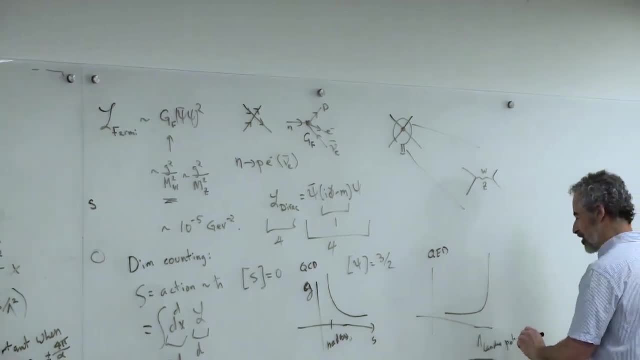 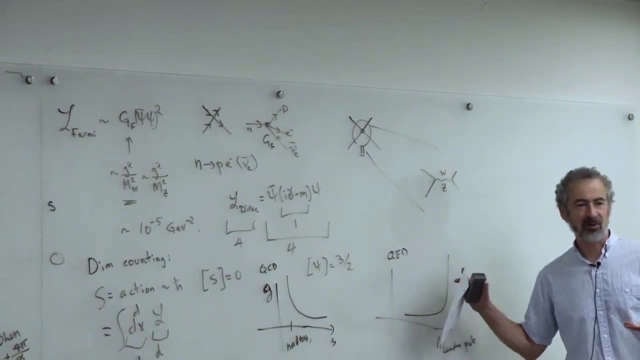 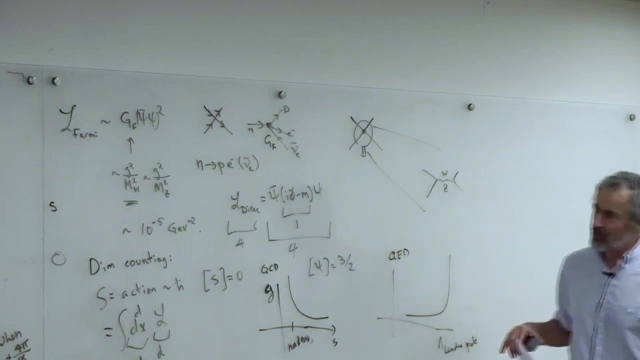 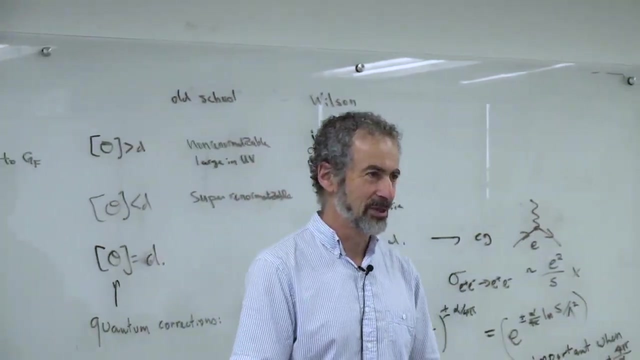 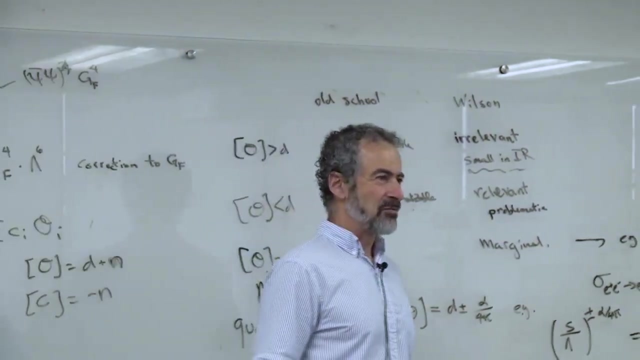 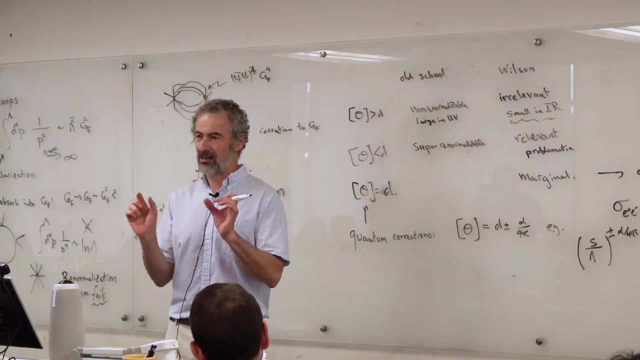 and for QED you have the opposite behavior. it blows up at something that will happen with these theories. when we look at it from Wilson's point of view, Wilson was driven by an interest of actually computing quantum field theory, putting it on a computer. so you have. 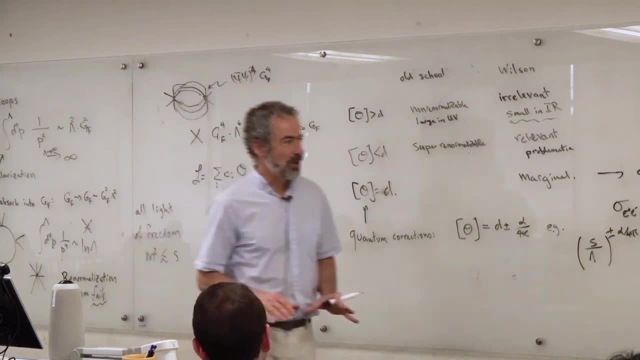 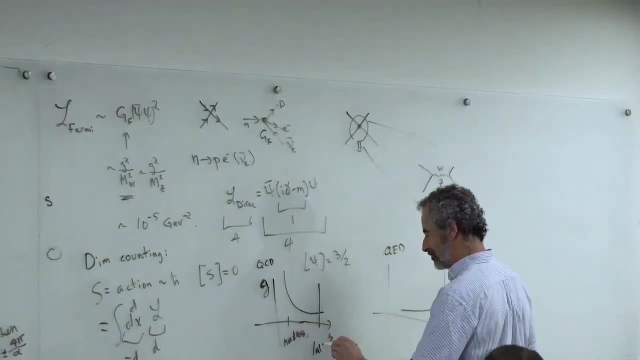 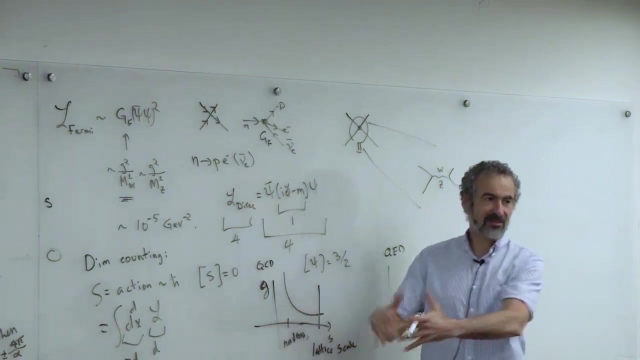 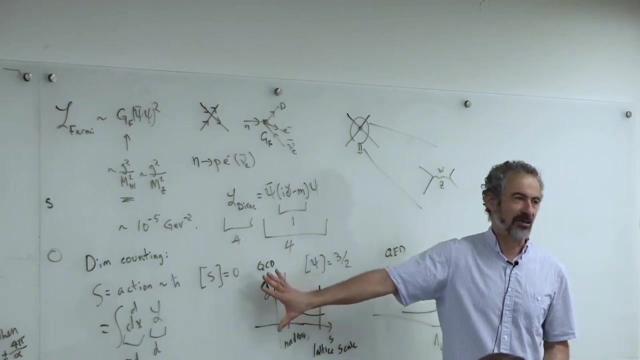 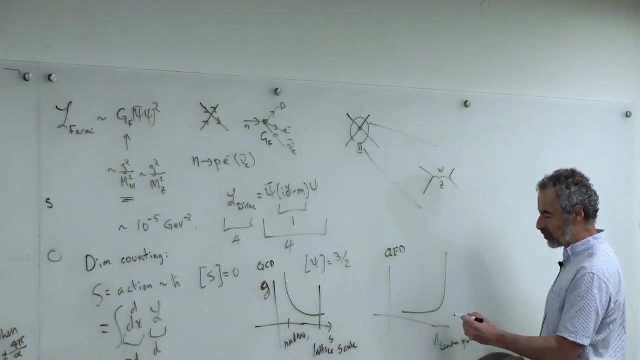 to define your theory at that lattice scale. so if you did QCD, suppose here's your lattice scale on your computer and you want to look at long distance and to take your lattice spacing to infinity, what if? if I tried to take the lattice spacing here, well, 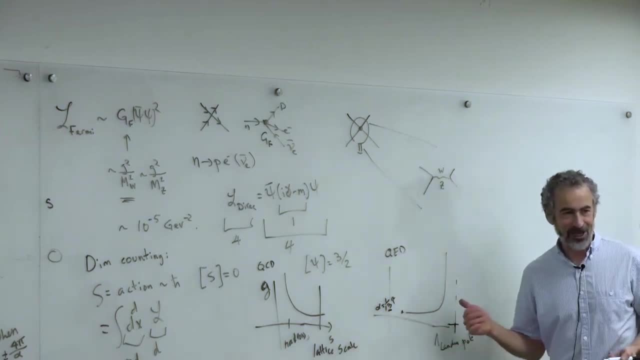 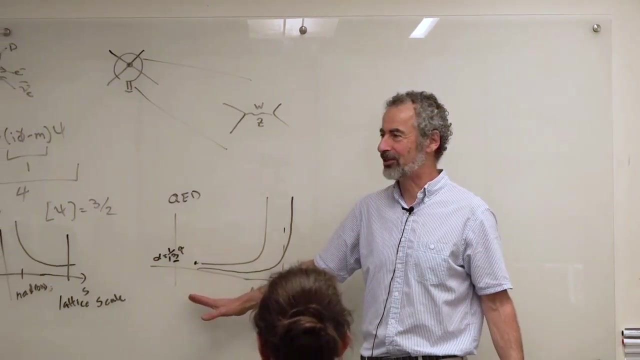 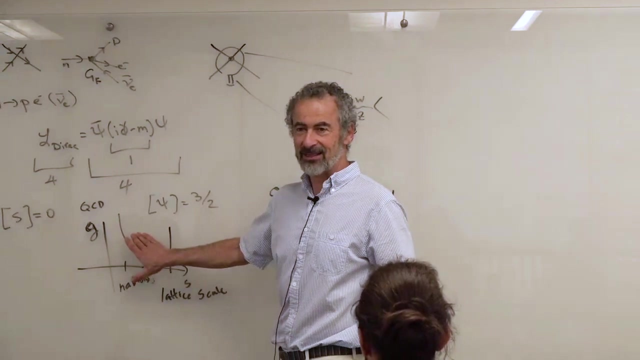 there's no way to do that. if I want to keep down here, I want alpha equals 37 and if I try to take this lattice cut off to zero, to try to go back to the continuum world, I'd find that at the hydrogen scale there's 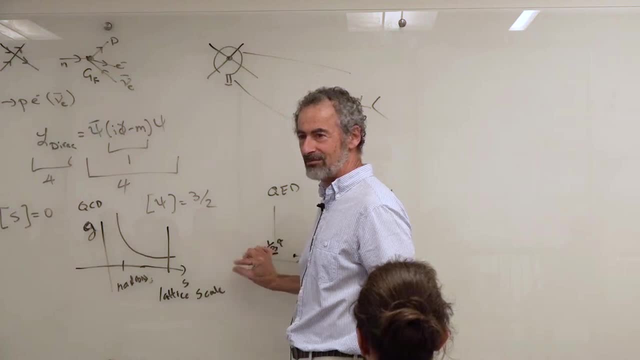 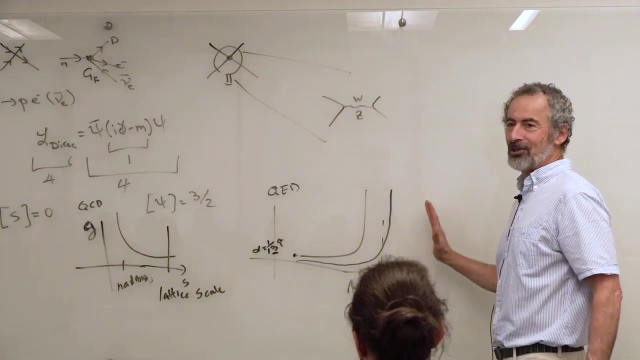 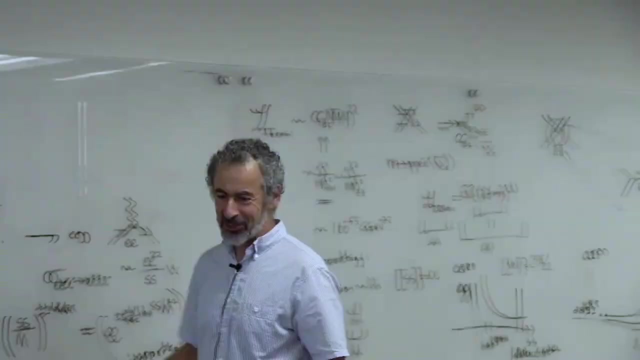 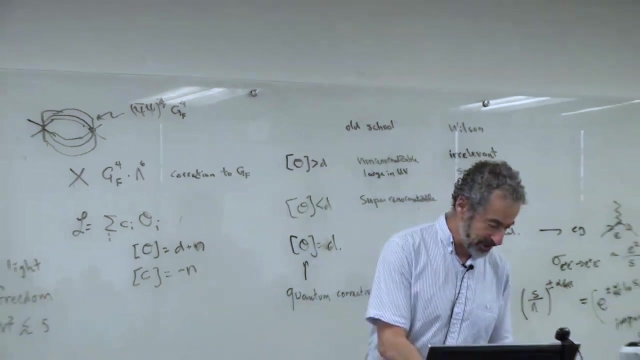 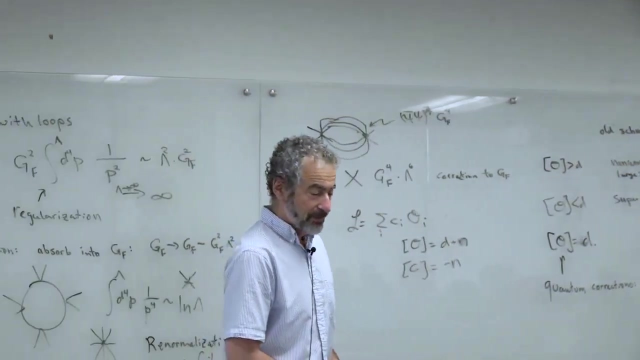 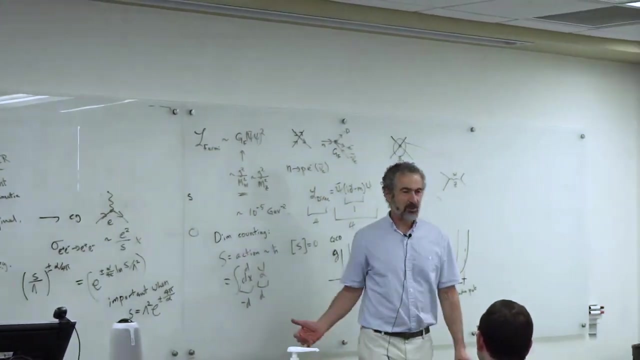 no interaction at all. it's called a trivial theory. even if I take the coupling huge at the lattice scale, I end up with zero down at the hydrogen scale. this doesn't really worry us anymore because we know that electromagnetism is embedded in the system, remember? 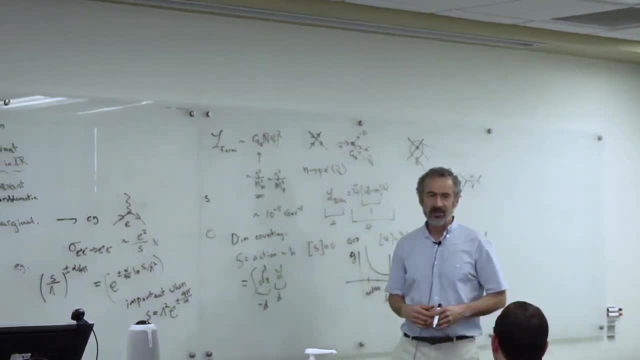 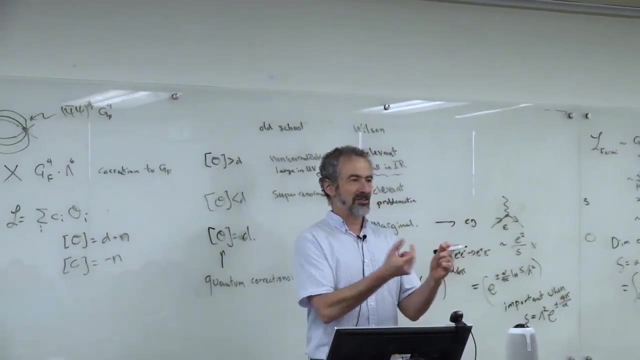 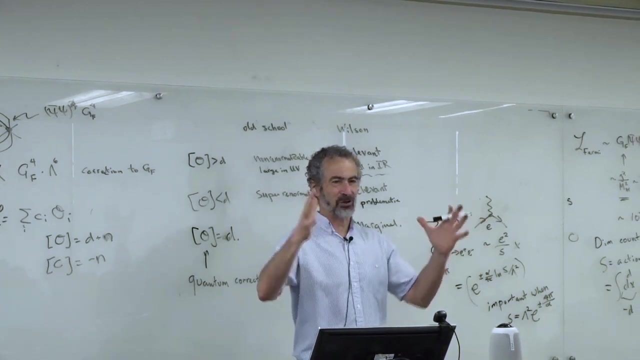 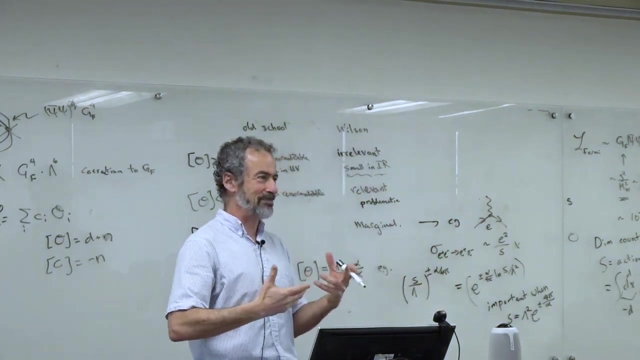 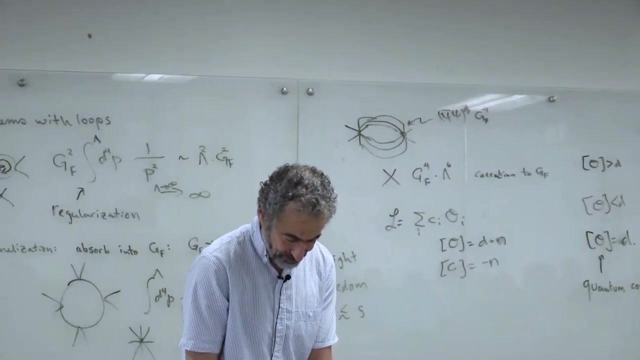 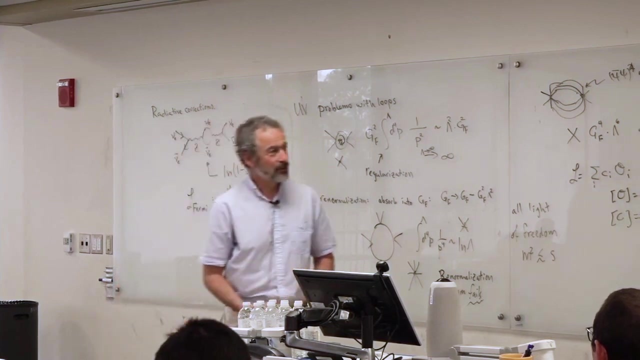 I said, what's cool about this is that protons can be so much bigger than the Planck scale. there's a similar phenomenon in condensed matter systems, which is super conductivity. it's the same way. so, for the rest of today's lecture, what I want to 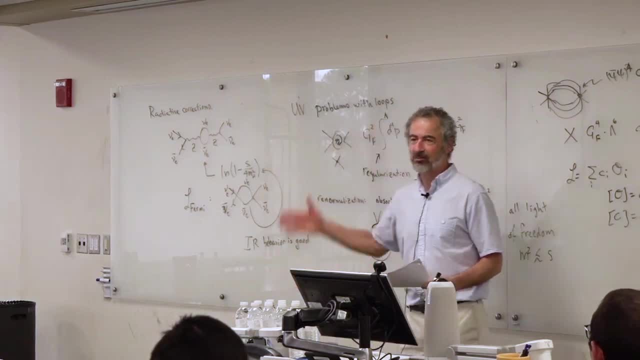 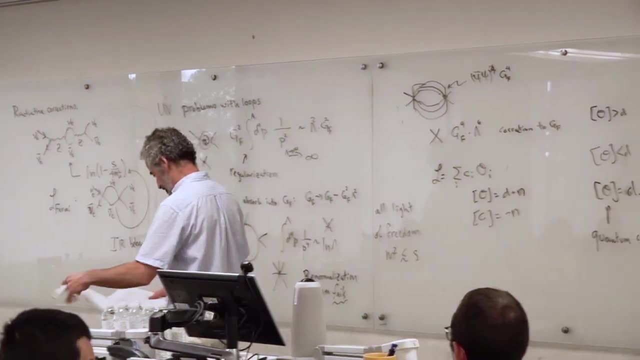 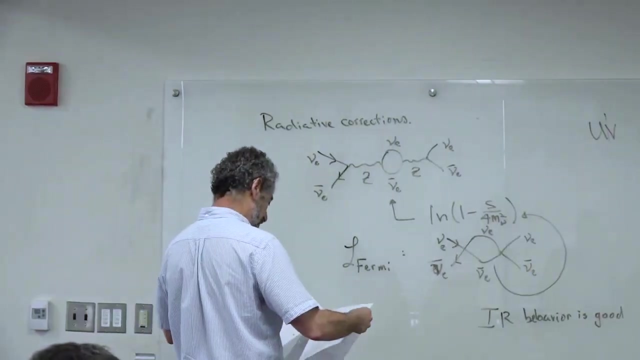 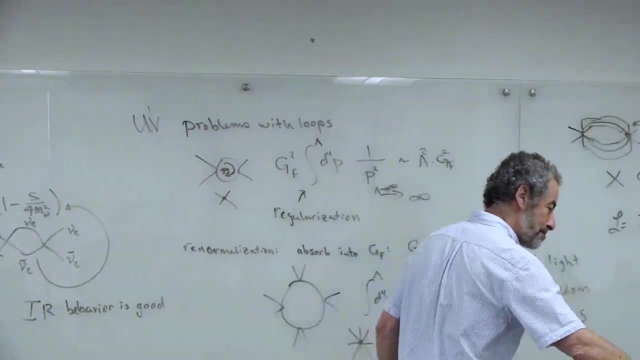 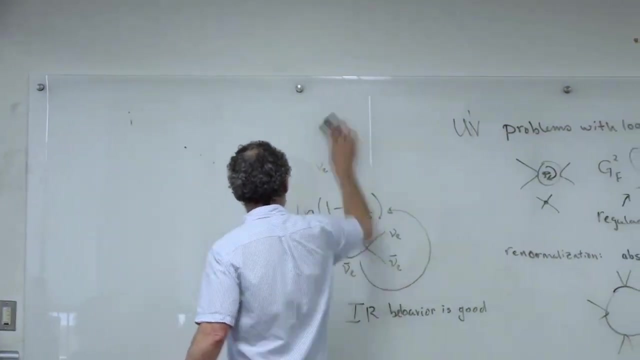 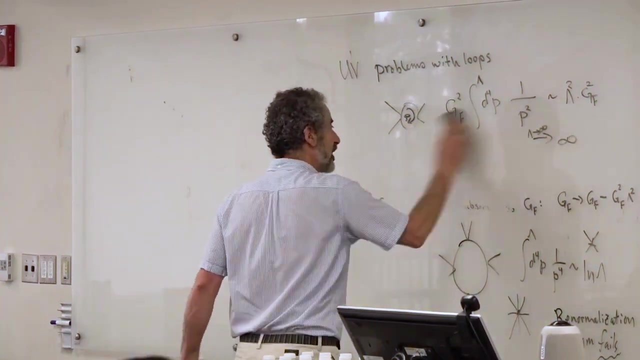 do is let's channel Fermi and say: we're going to pick the low hanging fruit. we're just going to follow the same line as what Fermi was thinking about, namely particle interactions. and what I'll tell you about is the program that Steve Weinberg 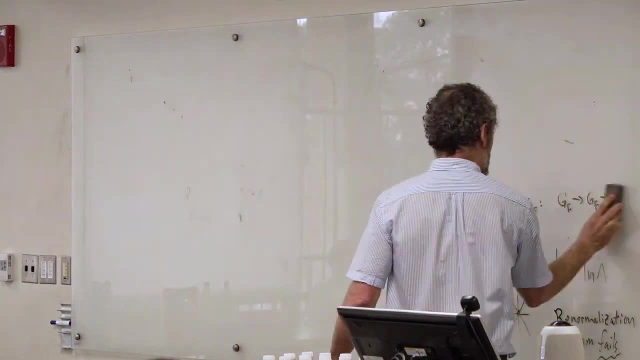 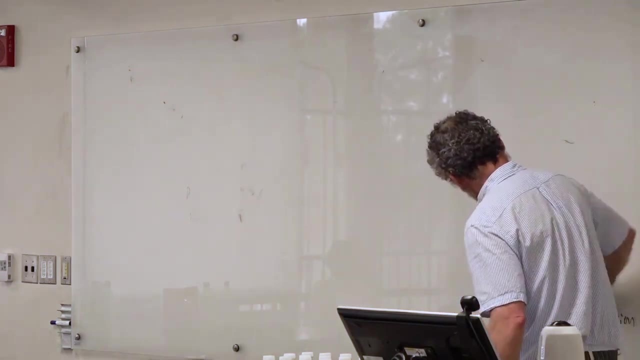 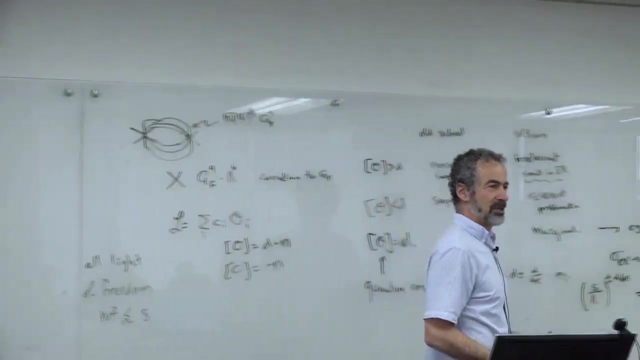 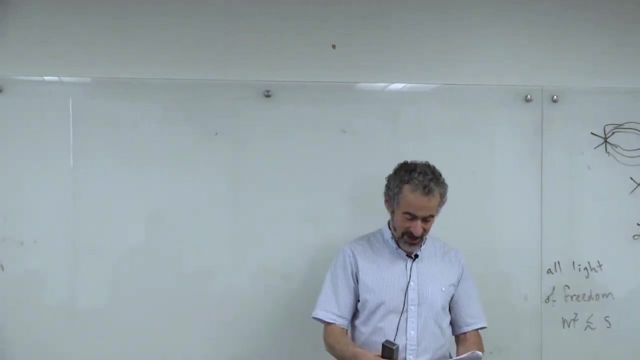 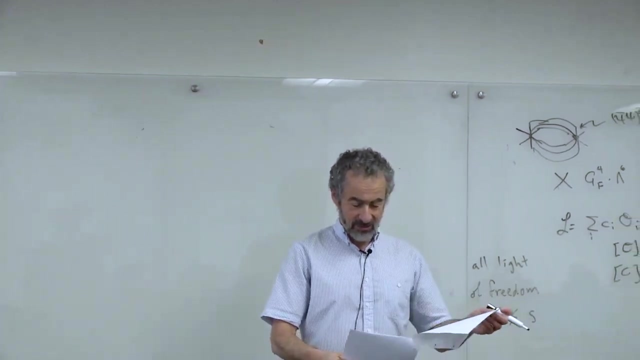 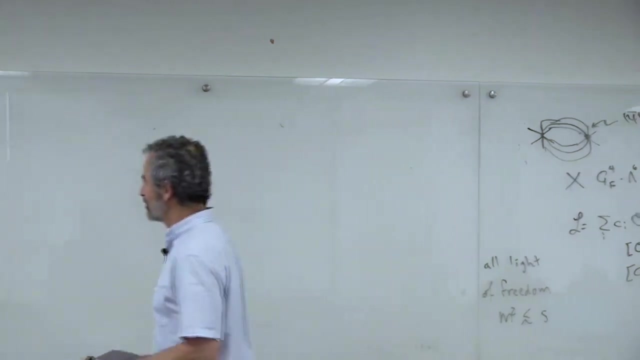 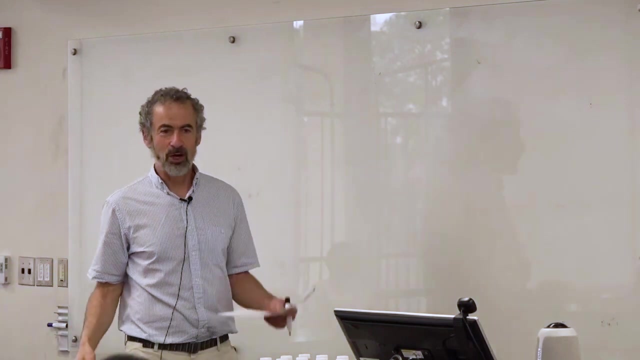 sort of pioneered. he wasn't interested in doing computations on a computer, he wanted to do analytical calculations, and so what he pioneered was ways of using effective, developing tools for doing effective filtering, using data and understanding what might lie beyond the standard model. so why was the Fermi? 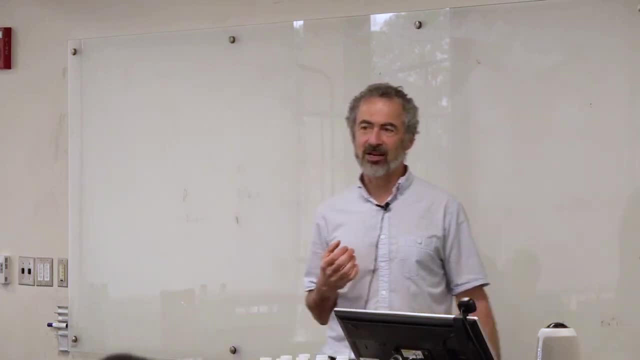 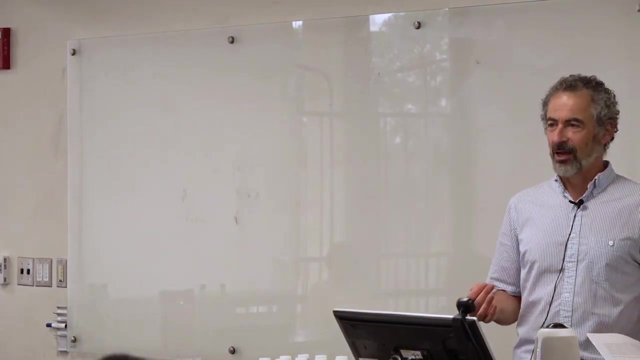 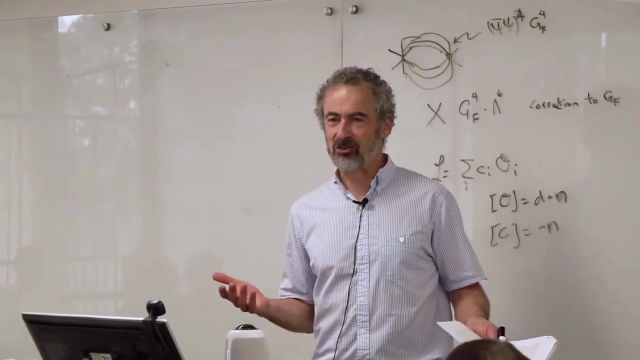 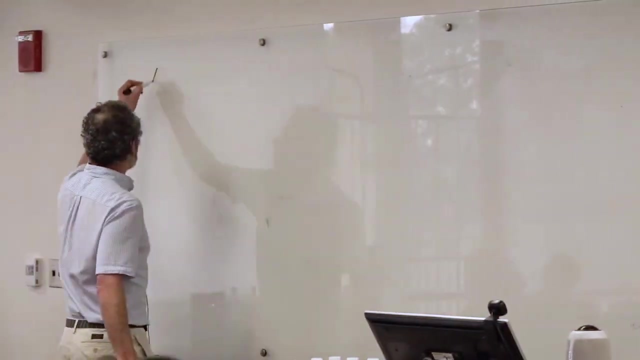 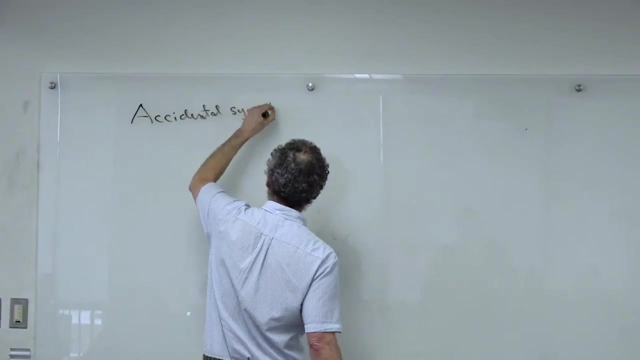 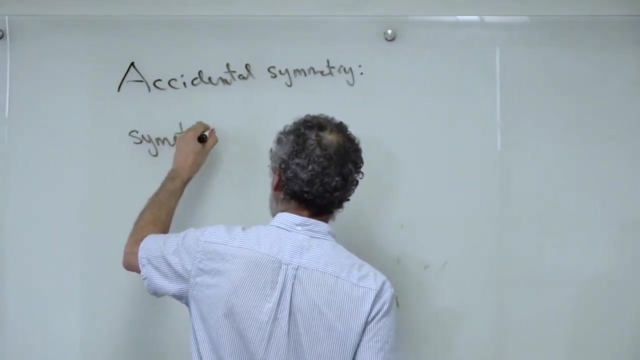 interaction so interesting. well, if you get rid of it, the neutron doesn't decay. you'd say there's a conservation law for neutron number and you say, oh, there's a symmetry. every conservation law goes with the symmetry. but we know that symmetry doesn't have symmetry. so 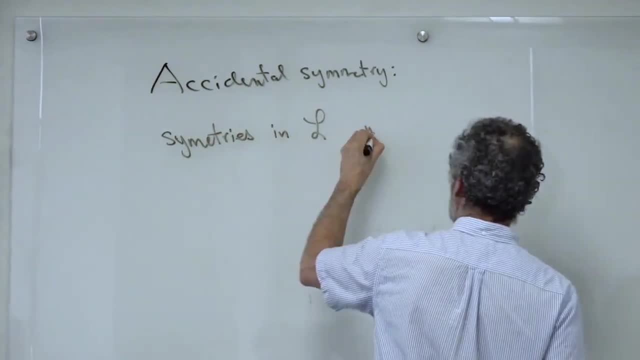 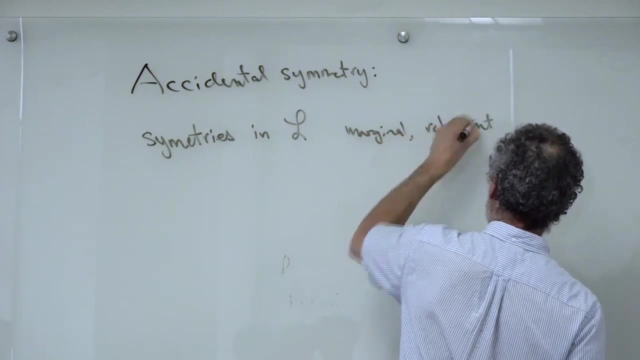 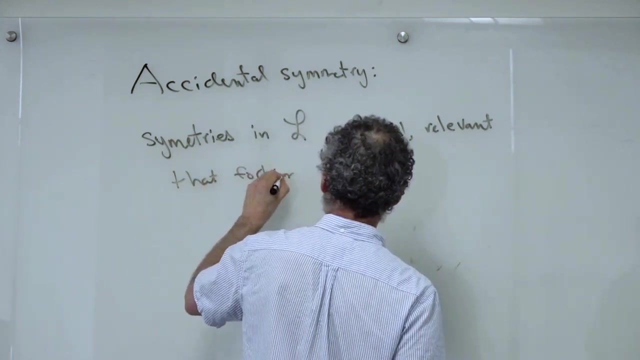 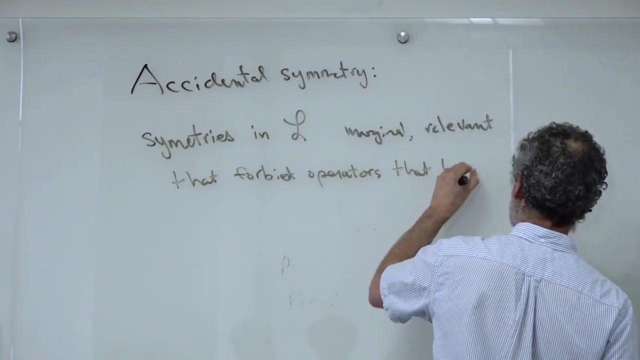 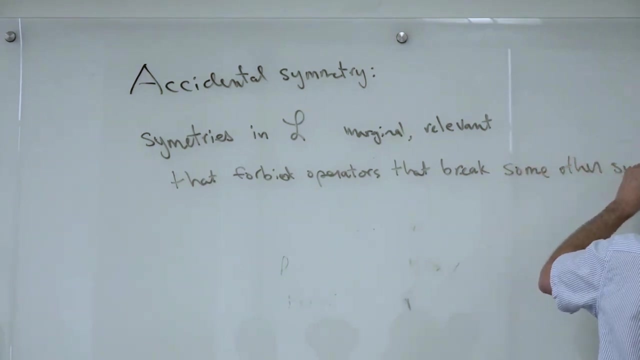 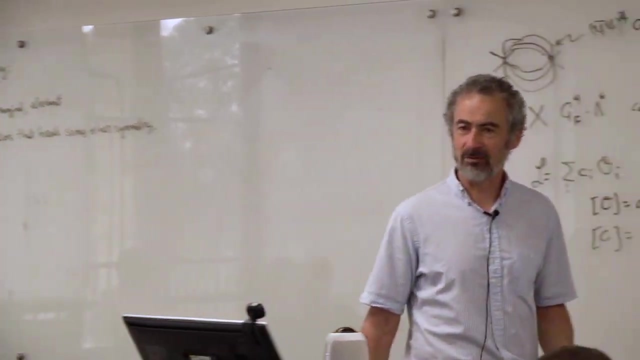 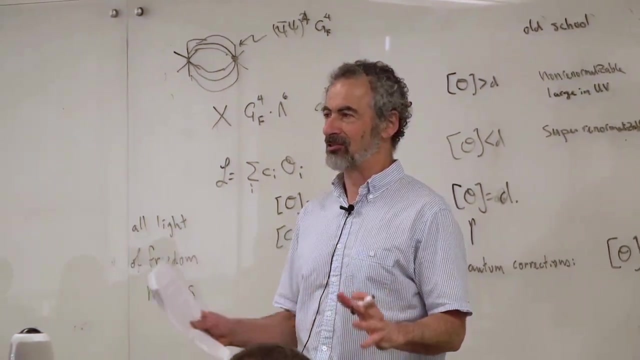 you have a certain set of symmetries in your Lagrangian for marginal and relevant operators that forbid operators that break some other symmetry. so you can write a dimension four or less operator with quarks or leptons that is consistent with su3, cross, su2. 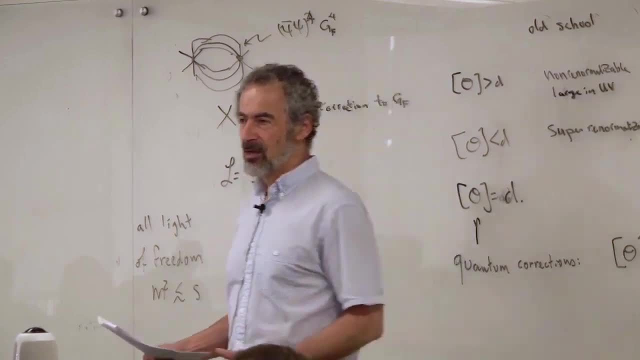 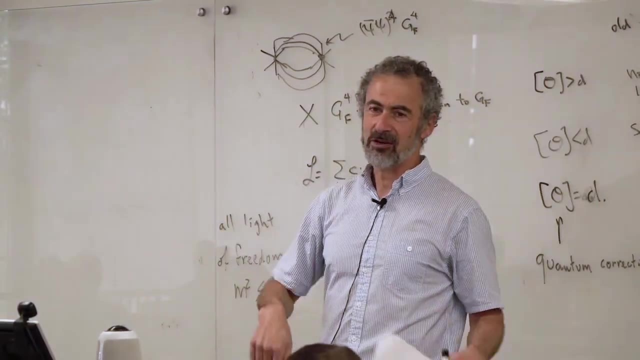 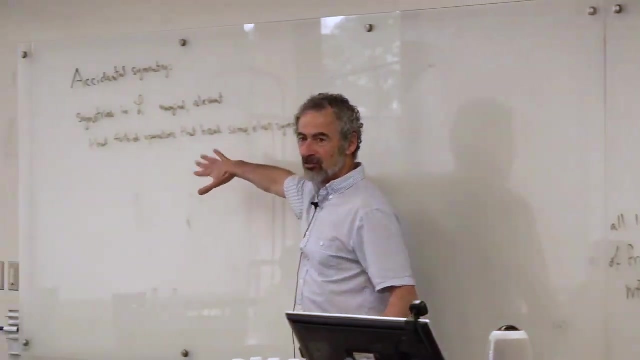 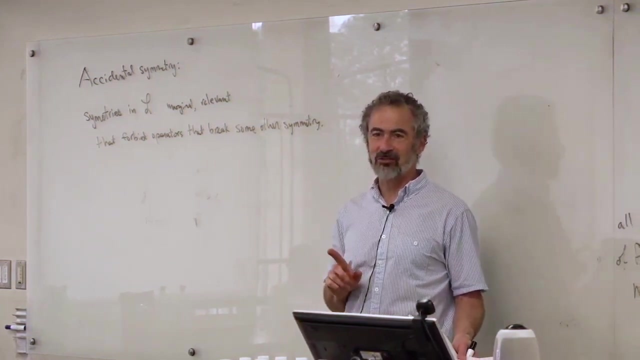 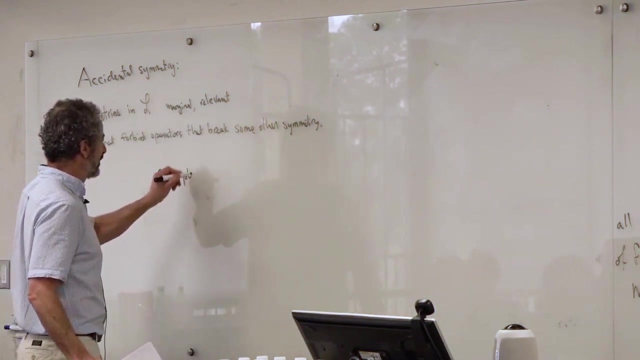 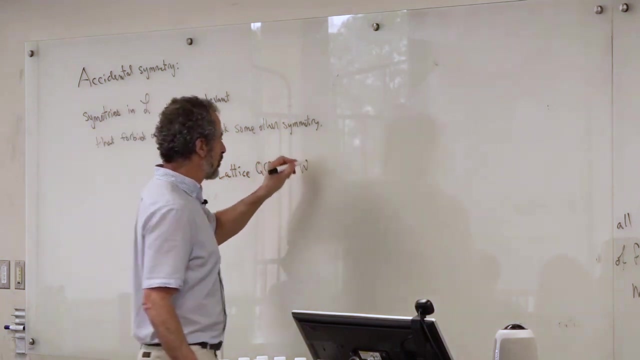 cross u1. that also breaks lepton number or bearing number. it cannot appear in the standard model except for three irrelevant operators. so therefore those conservation laws, bearing number and lepton number will appear to be symmetries of our low energy world. what guarantees Lorentz invariance? 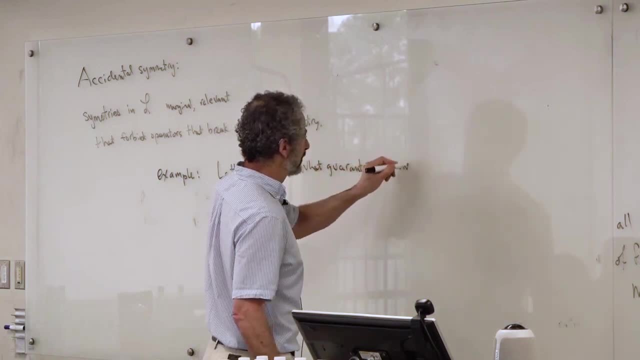 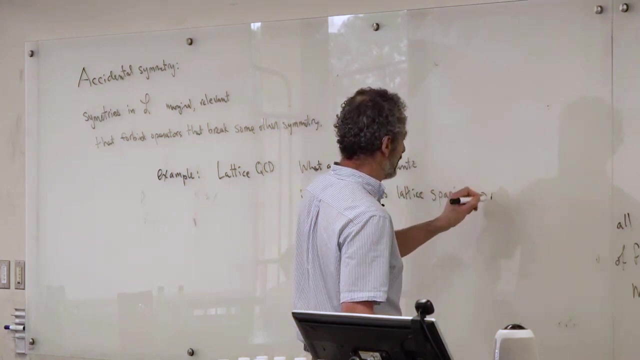 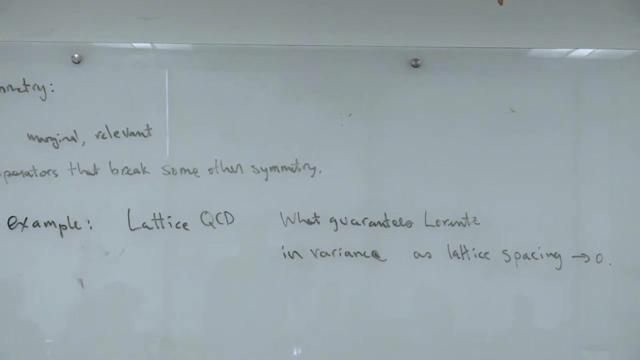 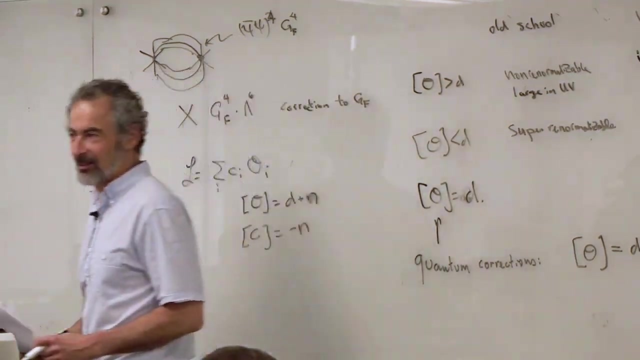 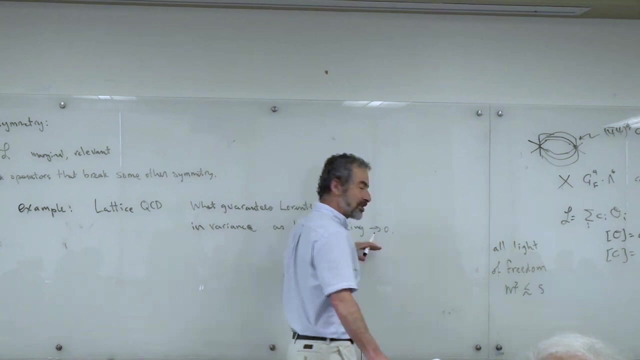 as the lattice spacing goes to zero. that is definitely not a symmetry. you've got in your lattice area right. your lattice area only has this one, so you can get Lorentz symmetry in the long run. how do I know I'm going to get Lorentz? 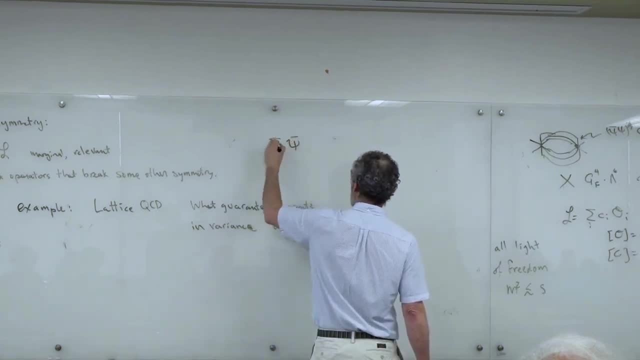 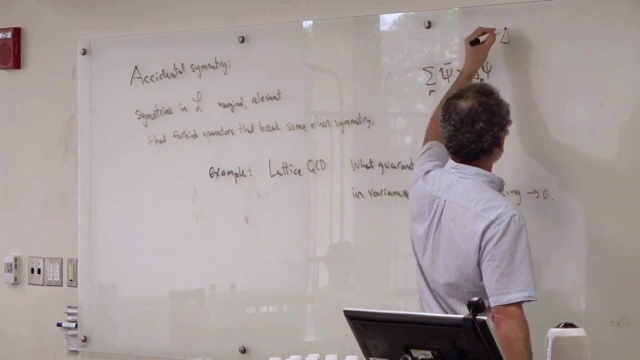 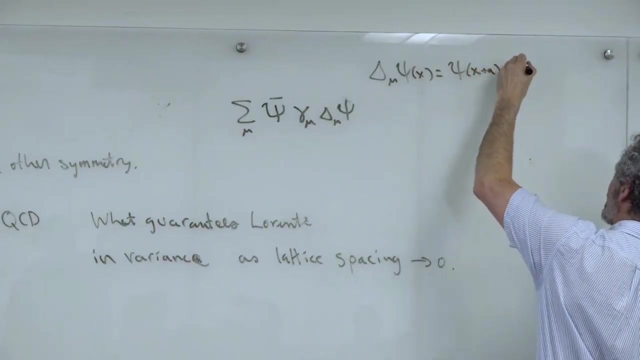 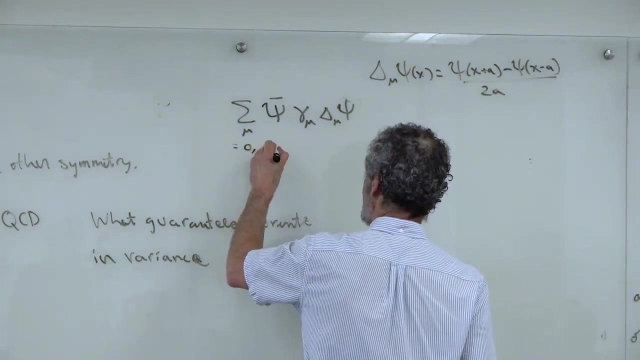 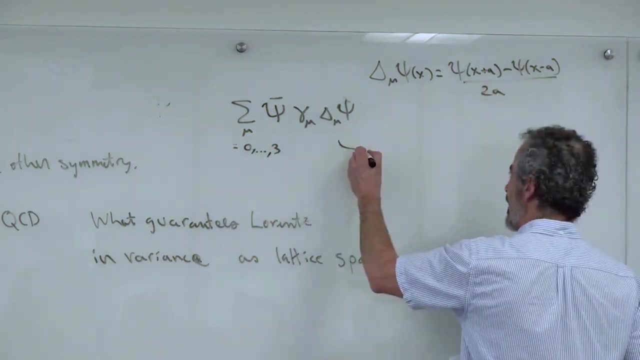 symmetry. well, let's take, let's try to write down an ell mu psi of x is psi of x plus a minus psi of x minus a over 2a. that's my lattice derivative. this is a hyper cubic invariant. I'm summing over the four. 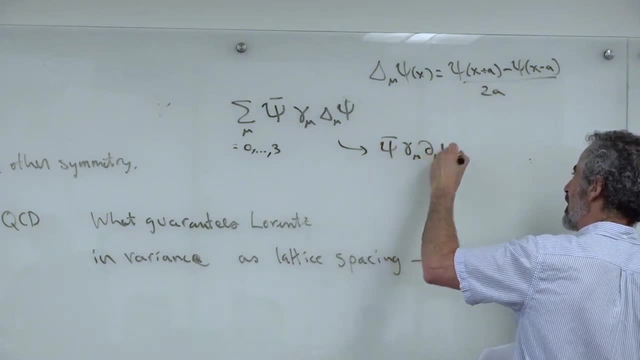 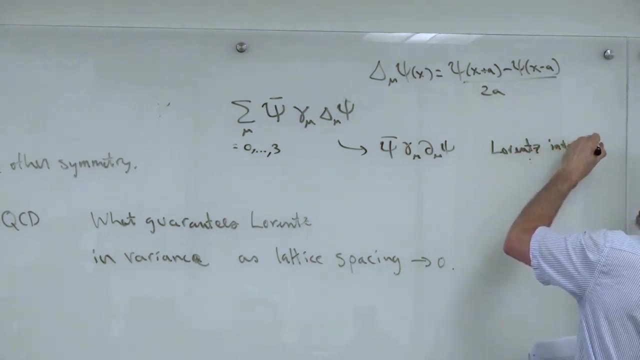 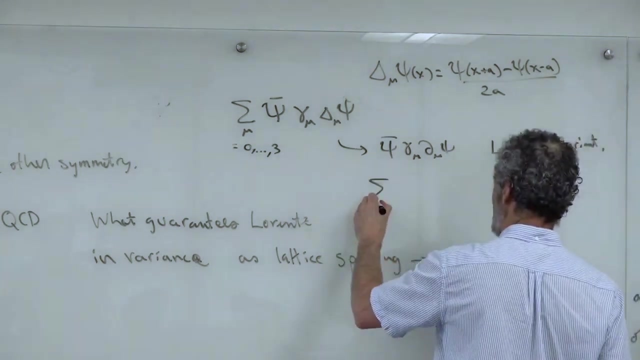 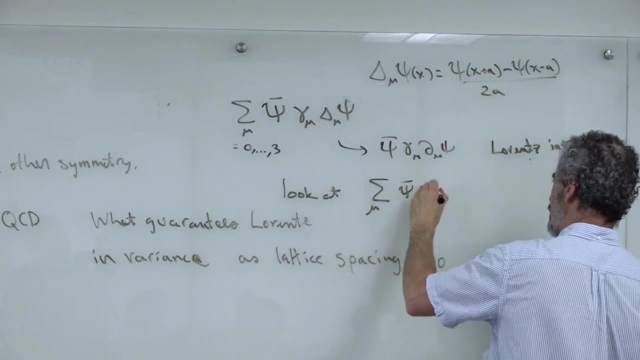 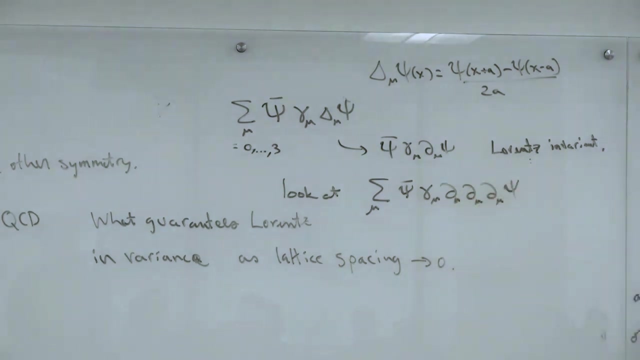 you get psi bar gamma, mu, d, mu, psi, which is Lorentz invariant, it turns out, if you want to try to write down a term, that breaks the Lorentz invariance. so this violates the usual index summation convention. I have four of the same. 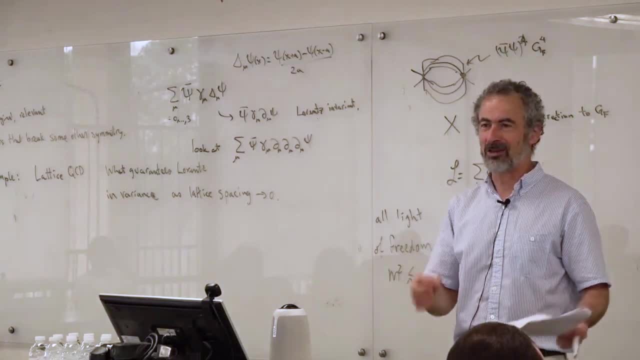 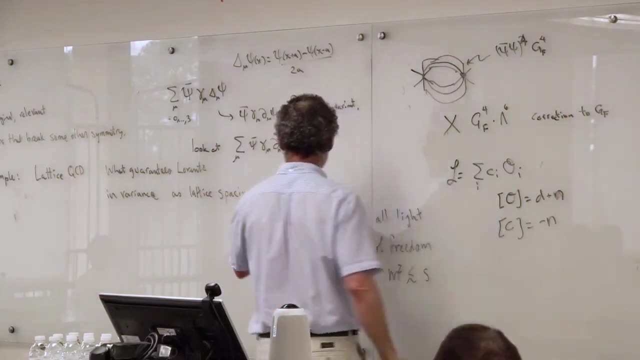 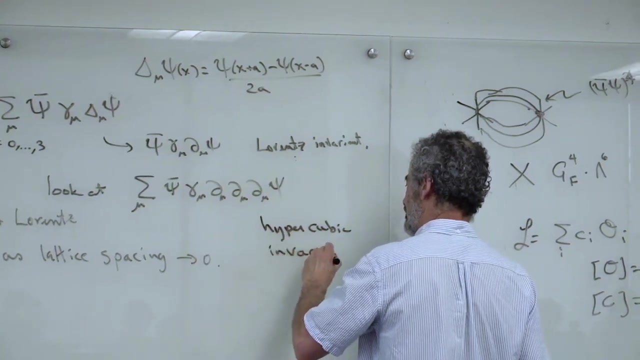 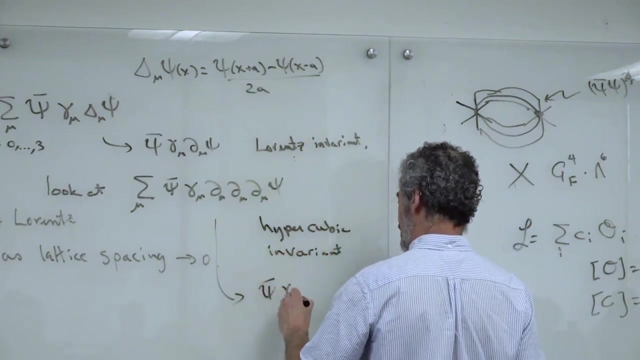 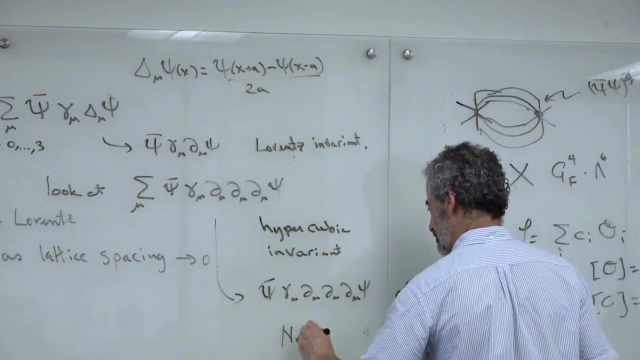 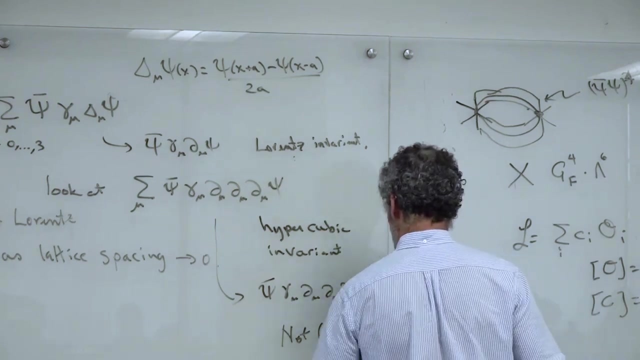 indices that I'm now summing up. this is hyper cubic invariant. you can sort of see it because it looks like if I change mu from mu into mu and I should be able to write a Oklahoma here, and if you were to write this in the continuum. 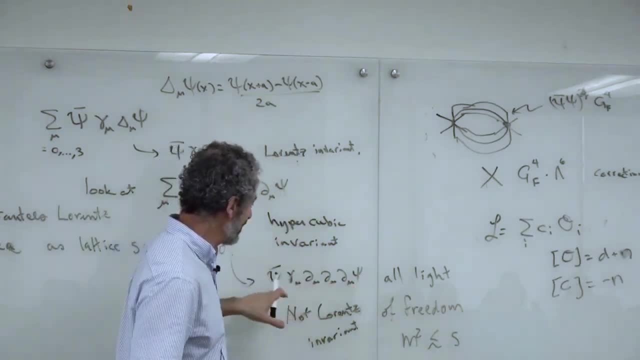 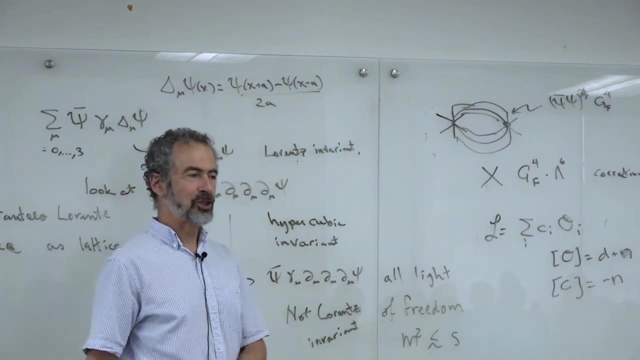 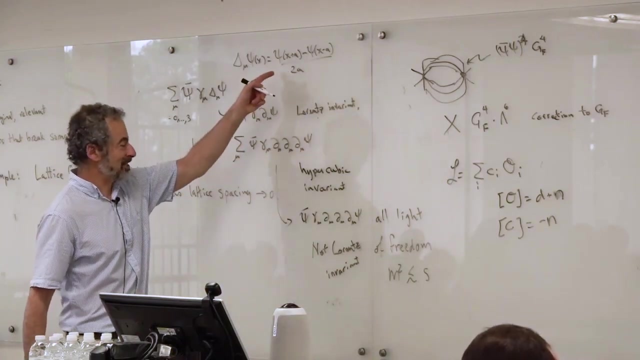 limit, it would turn into this: three derivatives, So it's dimension three, four, five, six. So its coefficient has to have dimensions one over mass squared or length squared. And what the lattice does is, if you actually just put this in and set A to zero, you find that you'll get an A squared out. 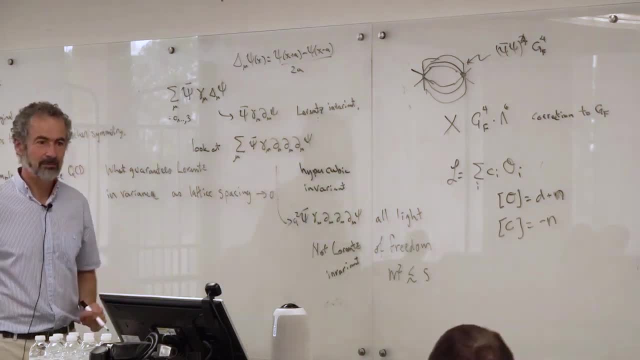 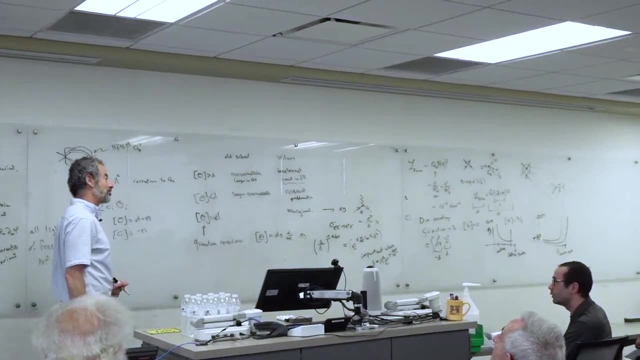 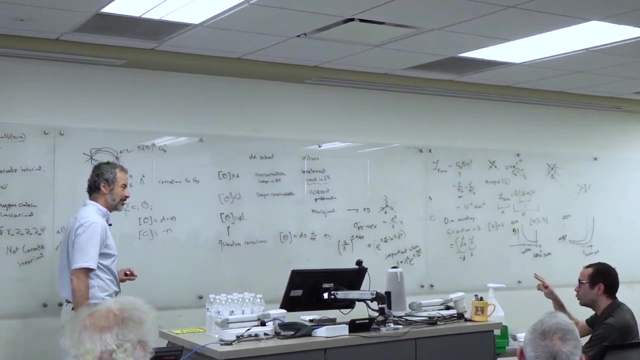 in front. Yeah, I'm sorry. I'm trying to write down an operator which is hypercubic invariant and is not Lorentz invariant. That's OK, But wouldn't that happen also with just two derivatives? So If you have three mirrors, that would not be right. 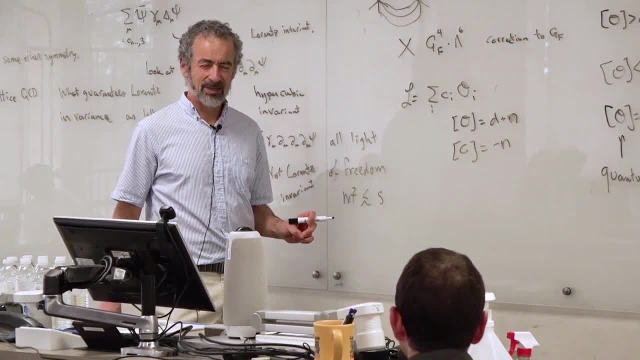 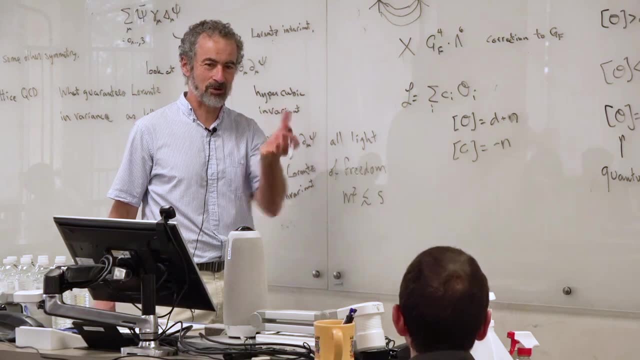 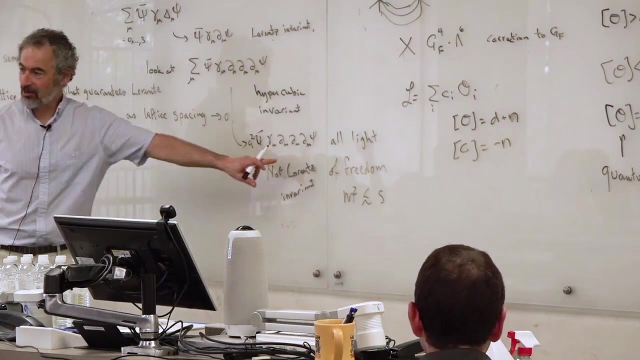 Right With two derivatives, though that's the problem. No, I think that would not be a hypercubic invariant You need. it's the fact that there are four indices and a four space time lattice. Yeah, So this has to have something a dimension length squared in front. 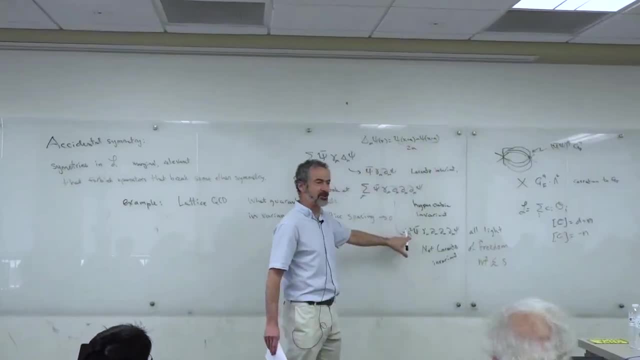 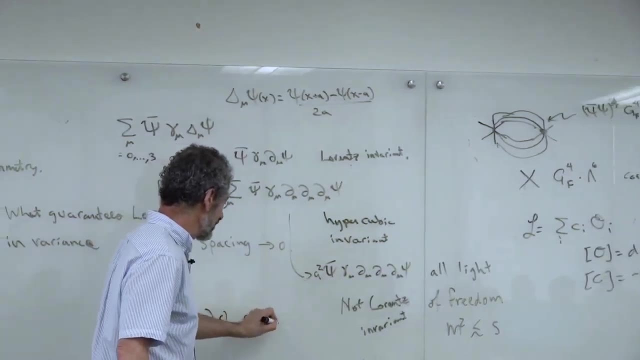 So what appears when you take, Yeah, the small A limit, is that this has an A squared out in front where A is the lattice spacing. So in the limit that A goes to zero, this goes to zero as A goes to zero, And so you. 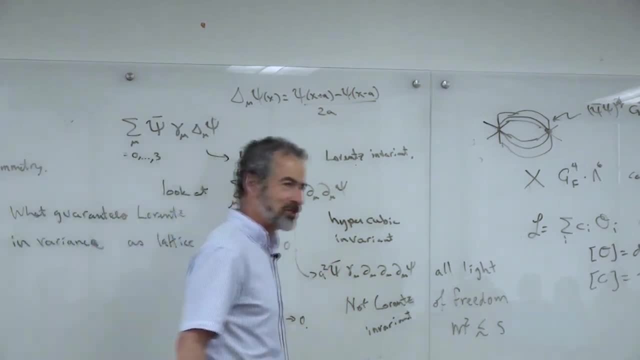 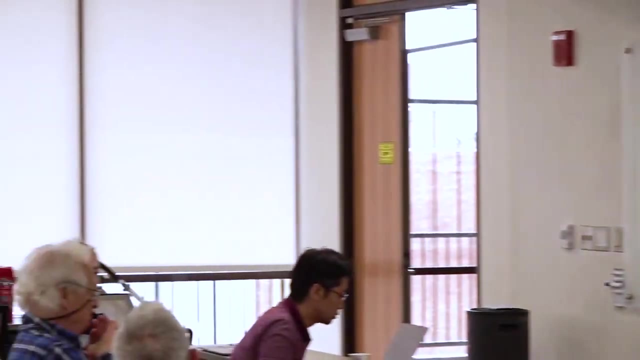 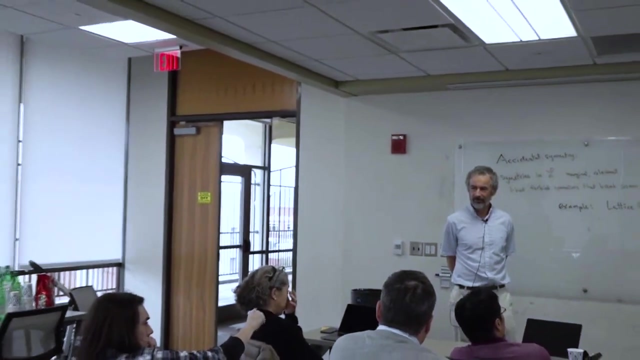 find that, even though your lattice theory is not Lorentz invariant, your continuum theory is Yes. Oh sorry, Just waving OK, So I'm a little bit confused. Are we adding three? I guess? lattice derivatives: Yes. 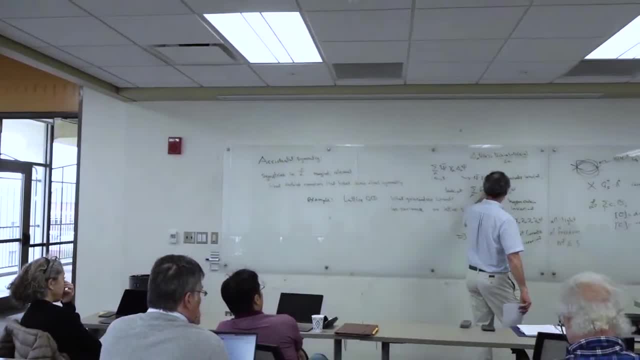 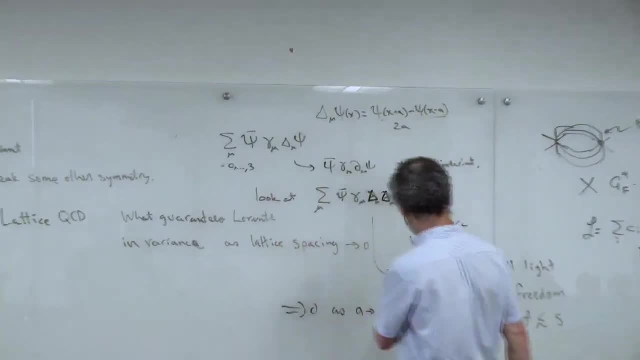 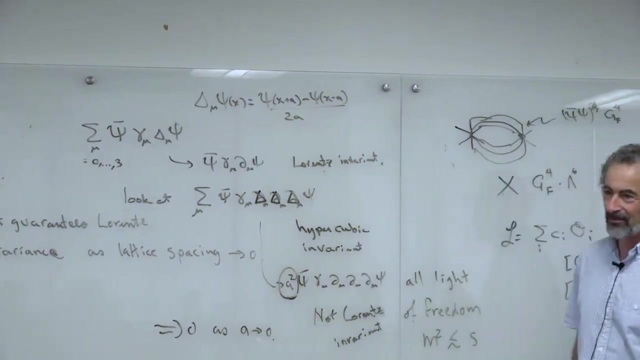 And then say Sorry, yeah, this is OK, Yeah, these are OK, Sorry. And then we're taking that same limit, saying: And then you take the continuum limit and what you find is this thing as A goes to zero. Yeah, And because of this term out in front, the thing goes away. So this is an, so, Lorentz. 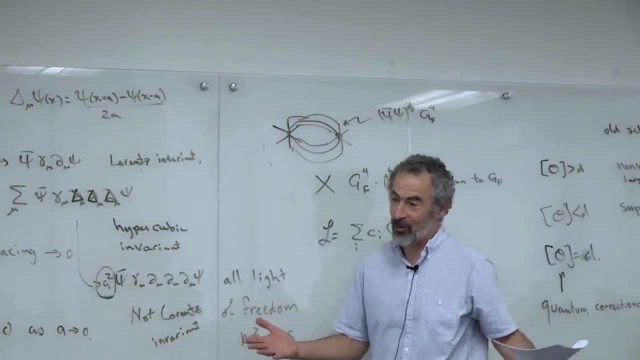 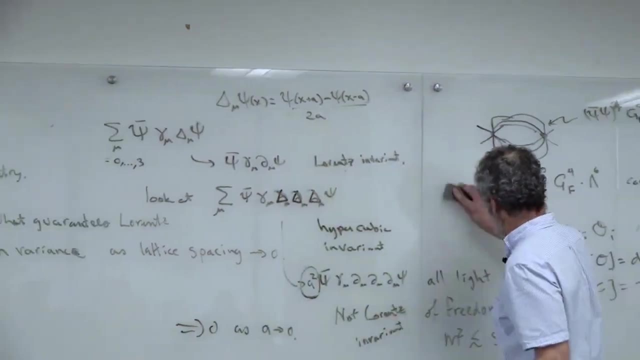 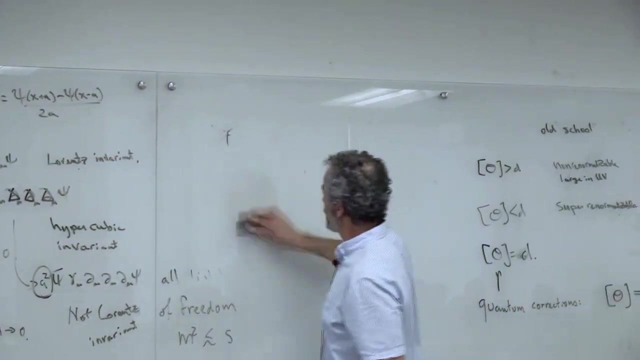 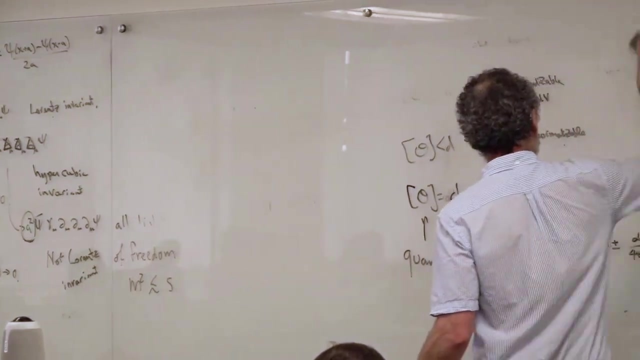 invariance is an accidental symmetry of lattice QCD. That's what makes it useful. If it wasn't, it wouldn't be very useful for describing the real world. So what Weinberg did? he's a very systematic guy. I remember as a grad student I noticed 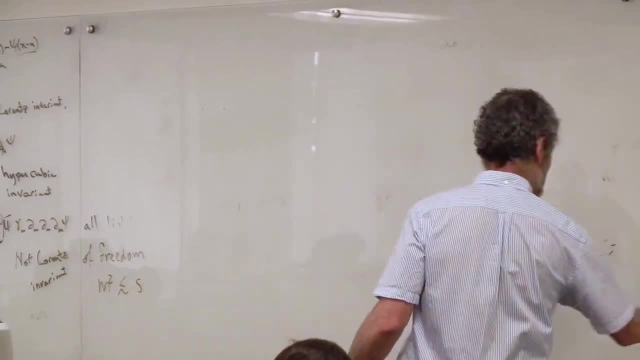 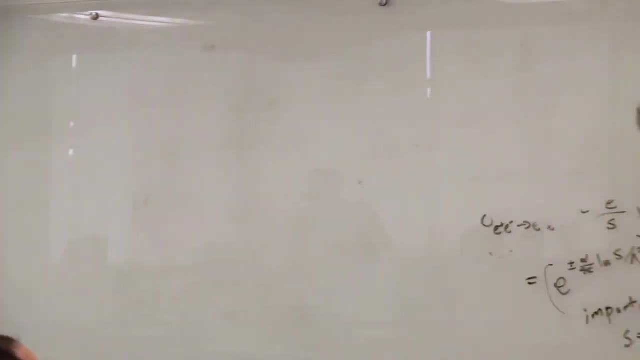 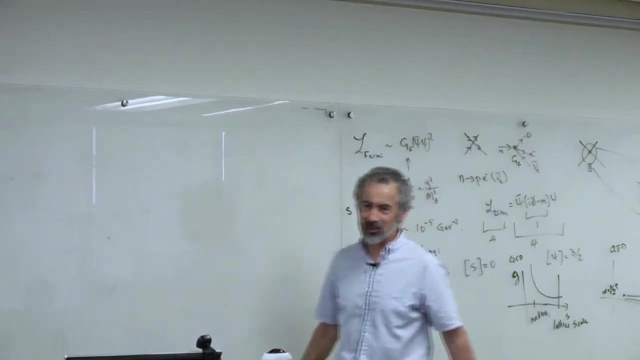 that all the Harvard faculty were very liberal with the exception of Weinberg. And I asked my advisor, Howard George, I said: is Weinberg going to vote for Reagan? And George, I said: well, his politics is like his physics: He has all the wrong instincts. 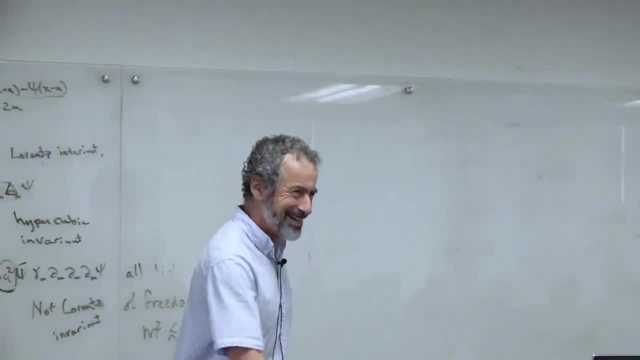 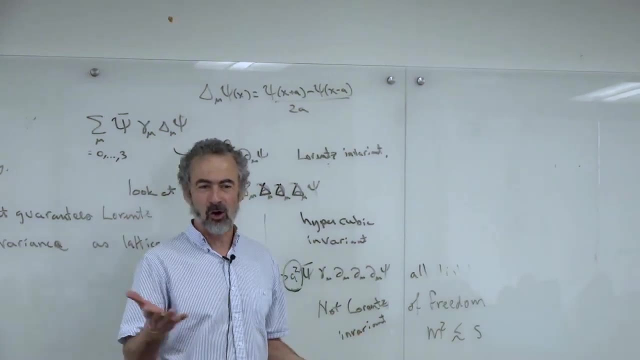 but he's too smart to come up with the wrong answer. And it's true. You know, you go to all these lectures and you see all these great physicists doing incredibly elegant things on the board. So Sidney Coleman was an example where you sit in every day. in quantum field theory, was this work of art? And you'd come out and you'd. 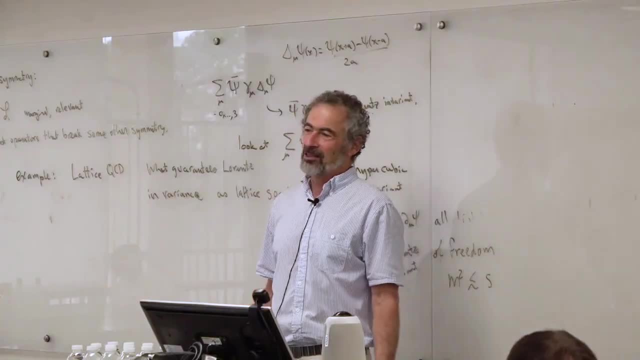 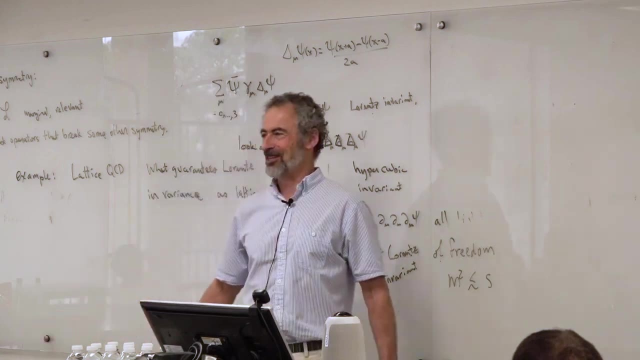 say: wait a sec. I don't know how to do that. Weinberg would use the worst notation and it would grind through these incredible algebraic calculations on the board and get to really cool answers at the end, But the process was so painful Anyway. so he's very systematic. 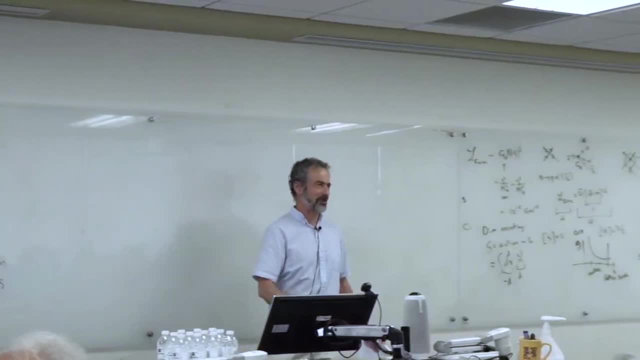 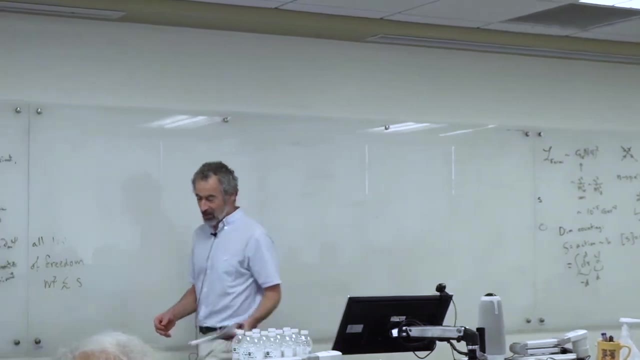 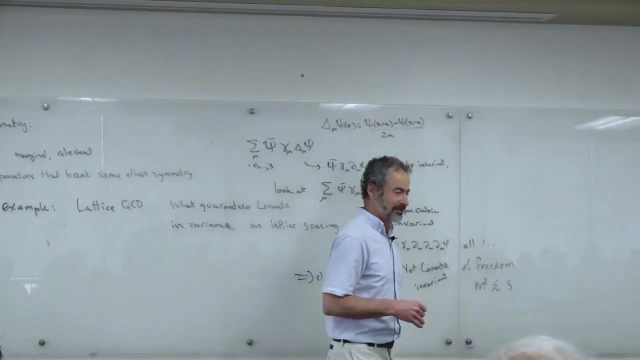 So he writes on all the operators of dimension five, Then he writes down all the operators of dimension six and so on. My very first experience with Weinberg was I'd come up with some idea and, George, I said, oh, you should go tell Weinberg, He'd be interested. I said really, So okay, I was a second year. grad student And he said: well, I don't know how to do that, I don't know how to do that. And I said: well, I don't know how to do that. And he said: well, I don't know how to do that. 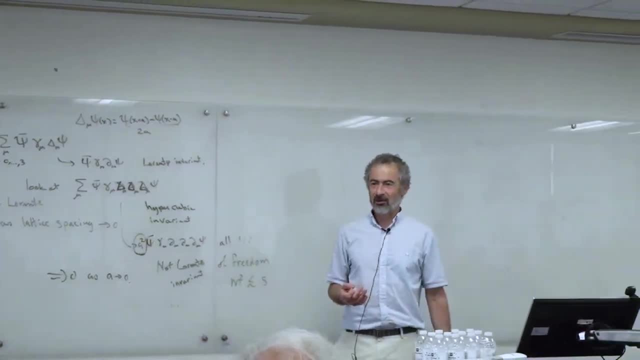 And I said, well, I don't know how to do that. And he said, well, I don't know how to do that, So I go knock on his door And I made the mistake most grad students do, which is they. 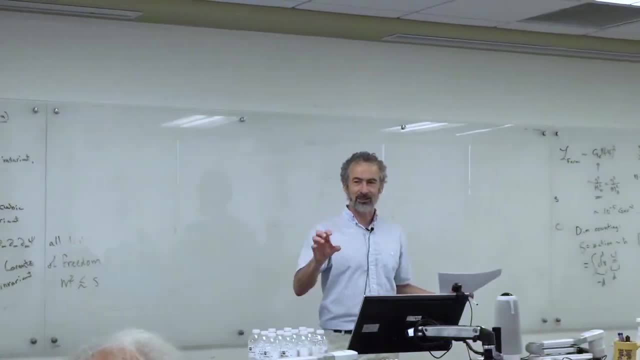 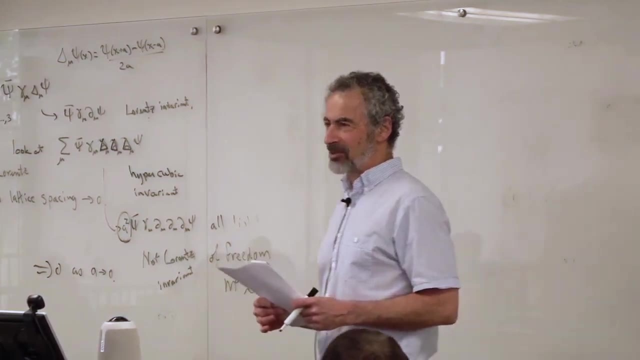 think that the big professors know everything And so you should just sort of telegraph your idea and not actually waste their time by explaining it in any detail. And within half a minute he was saying: I don't have time for this shit, People come into my office. 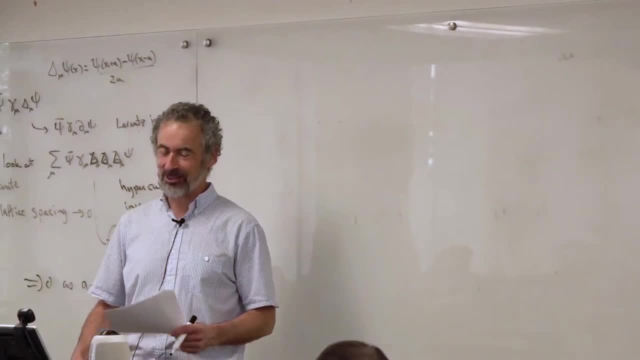 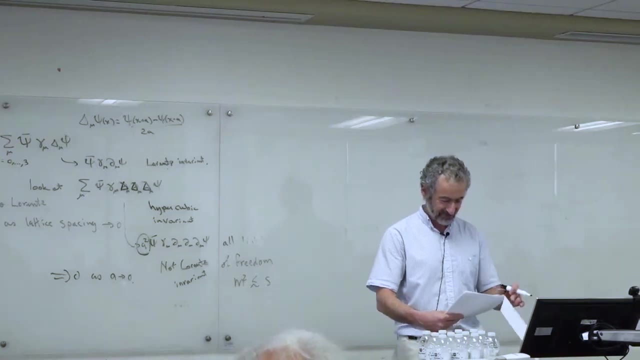 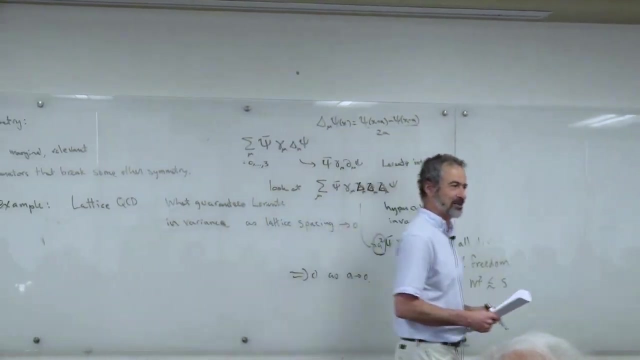 all the time I got to work Get out of here. I went back to George and said, was that really necessary? But later we had many good conversations when I became an adult. That was not uncommon to be yelled at at Harvard When I first arrived as a prospective. 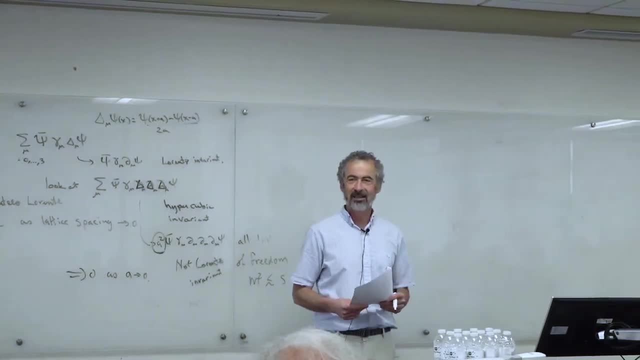 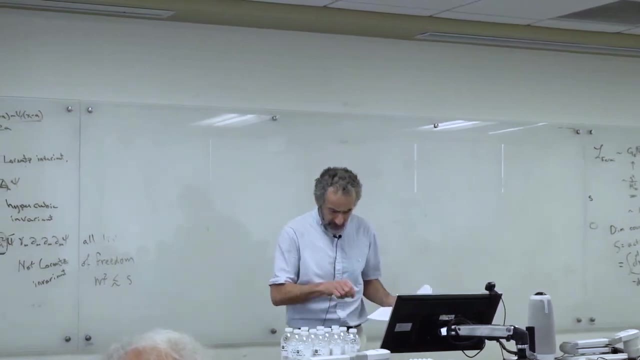 student. I'd gotten into grad school And I was visiting to see if I liked it. And I was ushered into Shelley Glashow's office And the secretary said we have a prospective student. He's sitting there writing And he says: go away, You won't get in. I said well, 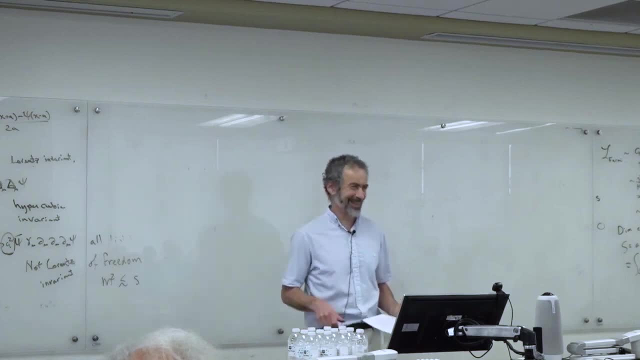 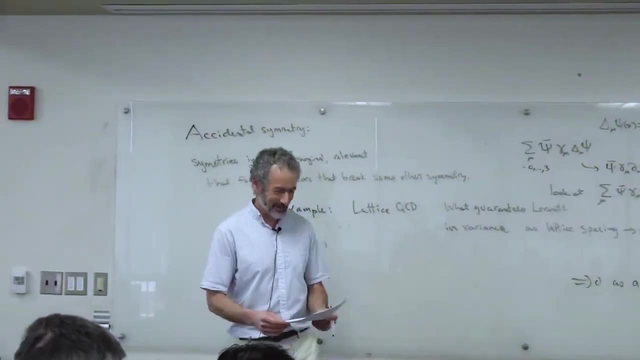 I'm already in. He said: OK, then come, Now go away. It didn't deter me, You get a thick skin there. You still went, I still went, yeah, Yeah. it does train you, though, to not burst into tears when somebody. 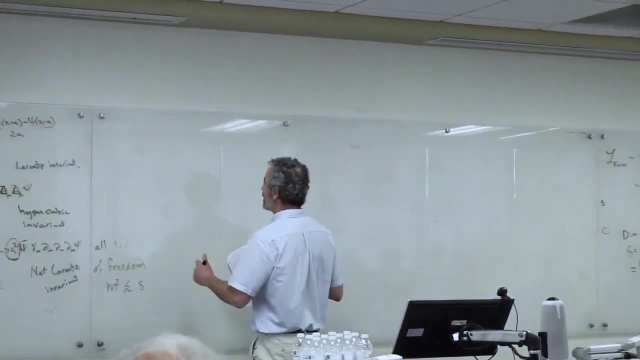 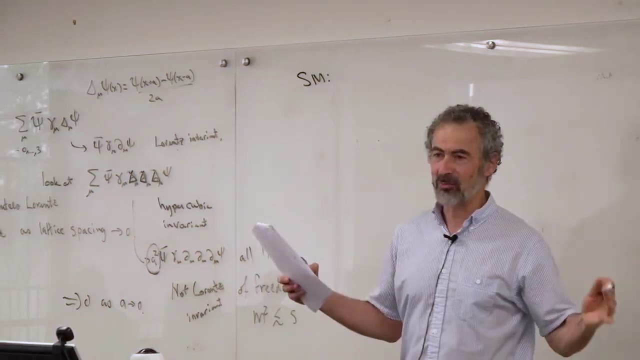 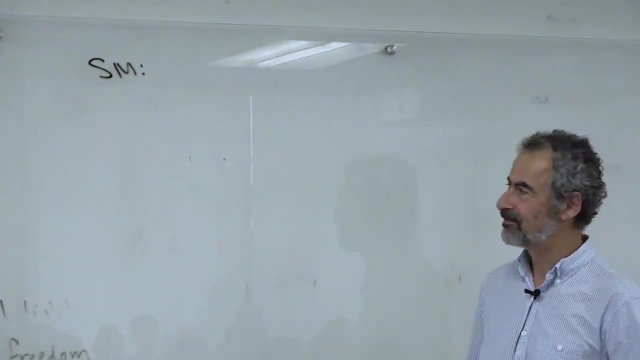 yells at you. OK, so the standard model. The standard model means basically all the dimension four and less operators. So that's the gauge interactions: SU2, cross, SU3, cross, U1.. It's got quarks, Higgs, leptons. 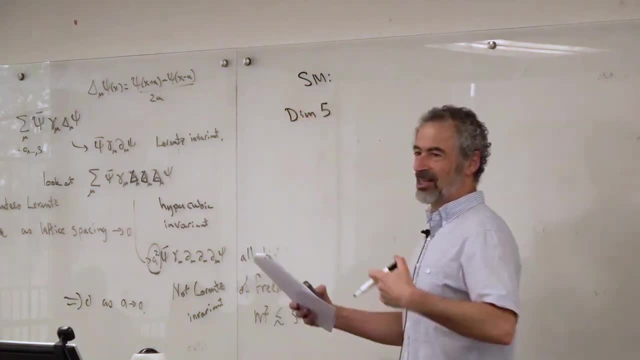 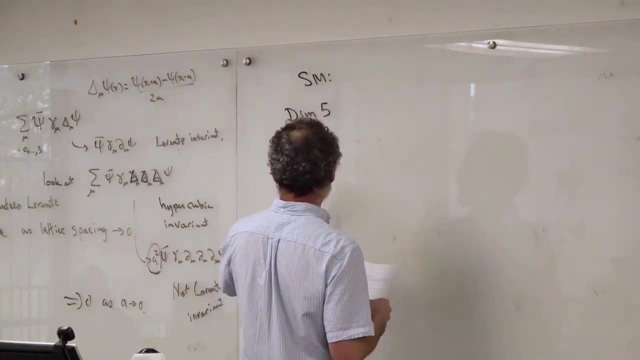 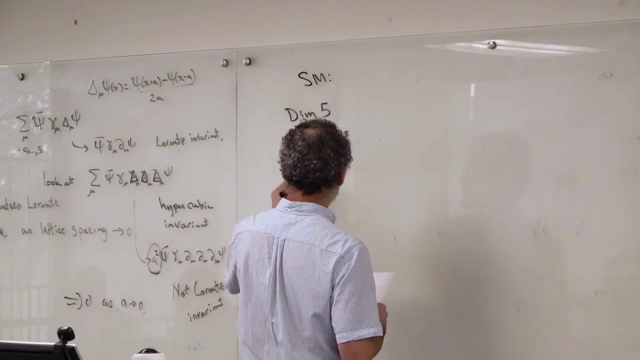 Let's look at dimension. five operators- That's the lowest irrelevant operator you can write down. It turns out there's two types, And the one that's interesting is you take a lepton and a Higgs star. This has quantum numbers. These are: 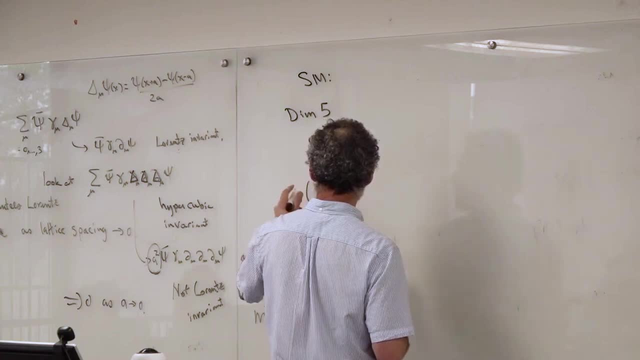 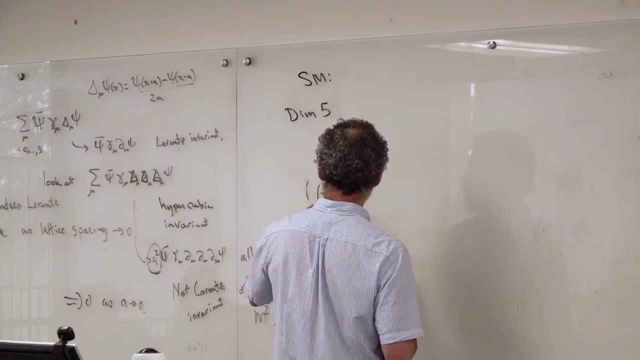 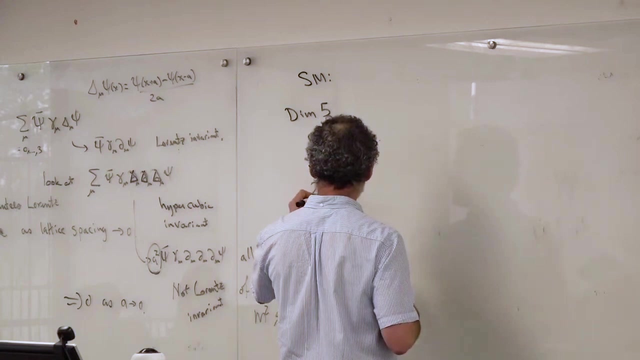 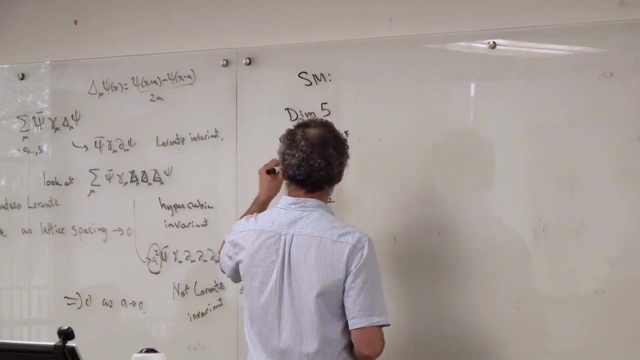 both neutral under color, Under the weak interactions. this is a half with a charge of minus a half, So I'll write this as a 2.. Sorry, So it means it's a doublet under SU2 and a charge minus a half under the U1.. And Higgs. 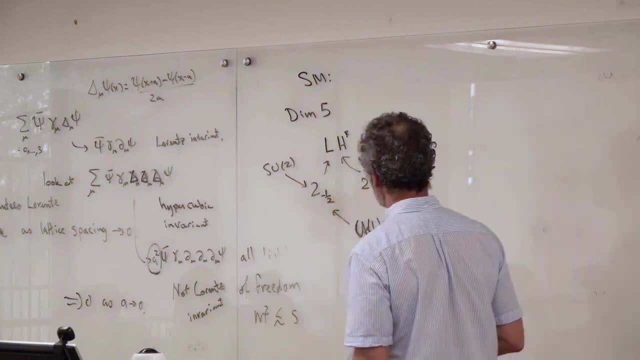 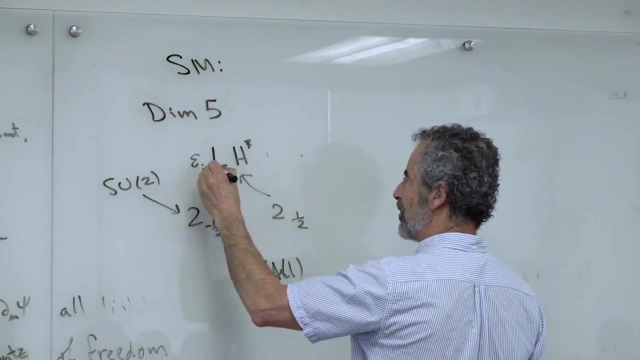 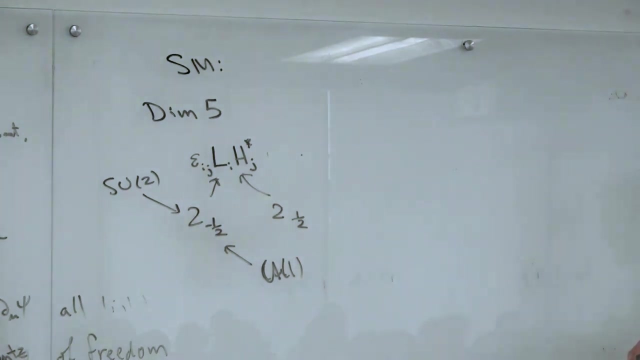 star is a doublet and charge 1 half And you can make an SU2 singlet, as long as you put an epsilon IJ coupling to two. Oh, I see, OK, the SU numbers. So now you get an SU singlet. Okay, so that is dimension, three halves plus. 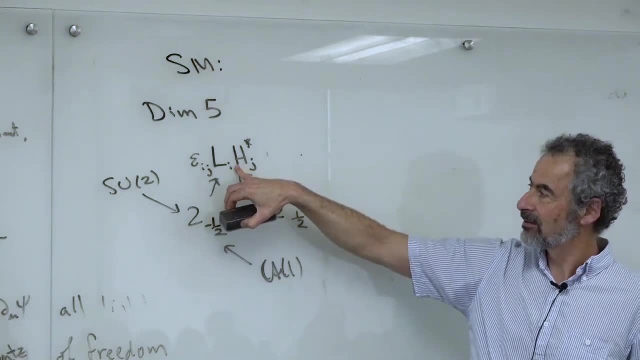 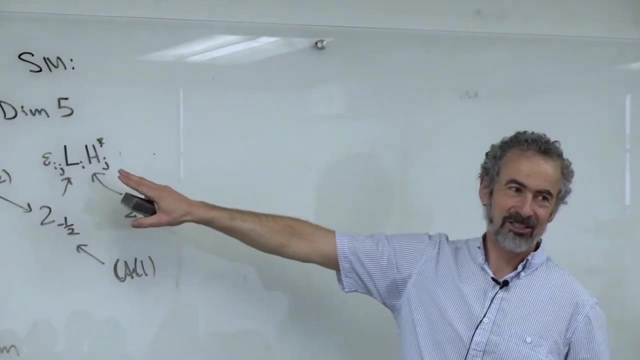 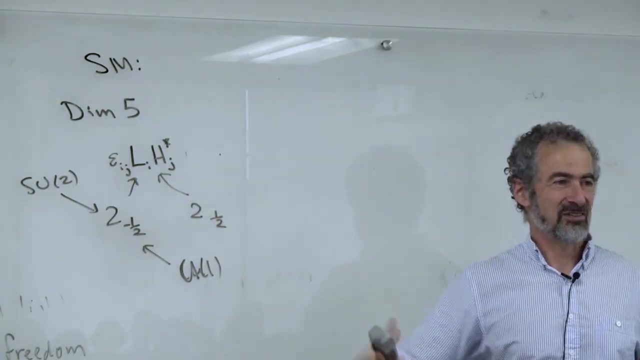 one. So dimension four halves, sorry, three halves plus one is five halves. But you can't add this to Lagrangian, because this is a fermionic object. This is a fermion, that's a boson, So the spin is still a half and you can't put that in Lagrangian without breaking Lorentz. 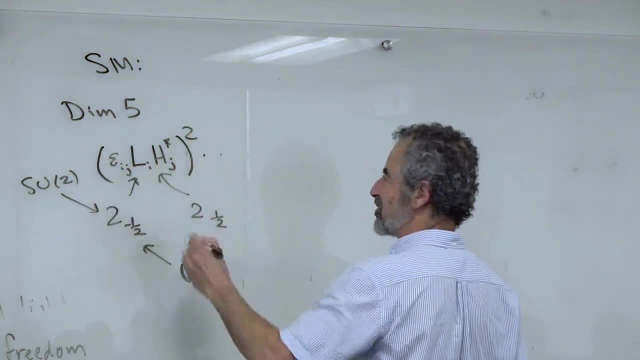 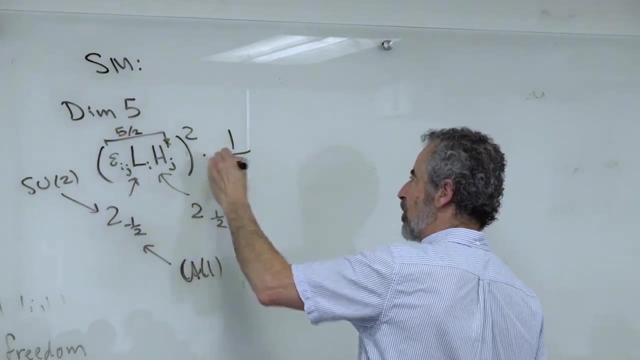 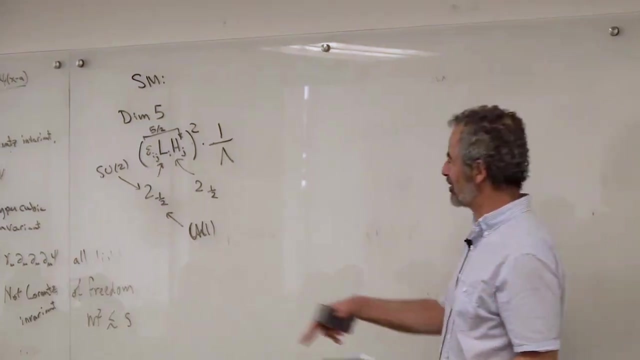 invariants. But you can put this thing squared and since that's dimension 5 halves the whole thing is now dimension 5. So it has a one over lambda, and lambda is some new scale. This is the equivalent of G Fermi For some unknown physics. we have not seen this yet. 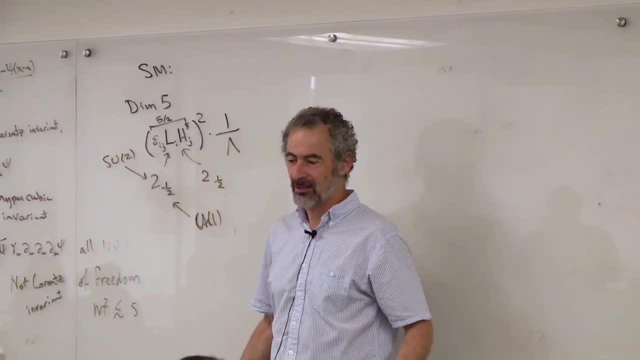 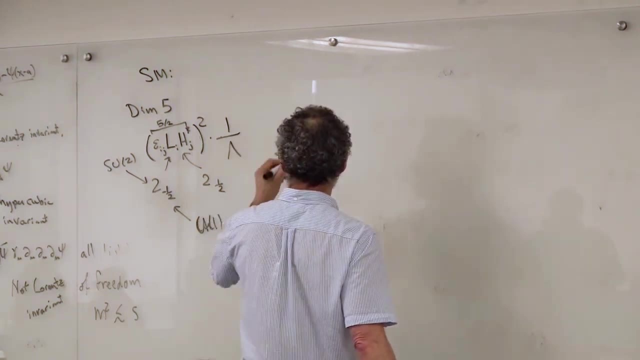 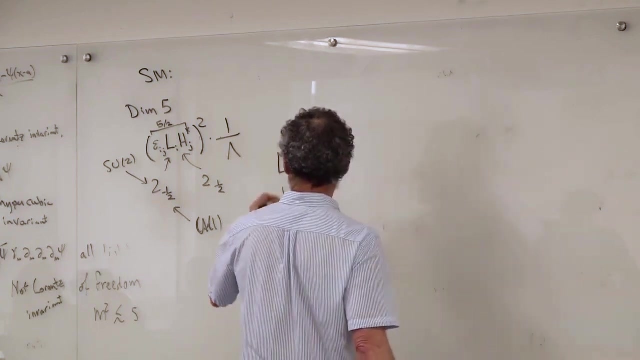 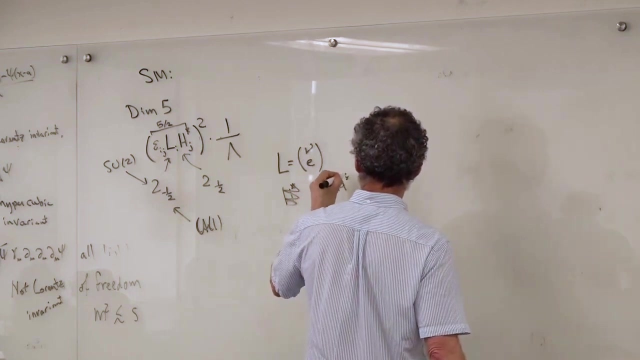 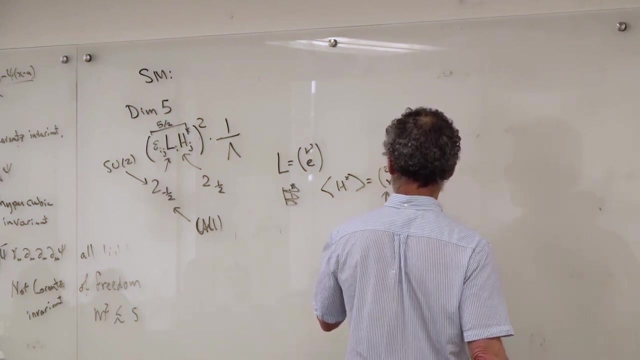 Weinberg had not seen this yet when he wrote this down. What's interesting, though, is that this gives neutrino masses, So L looks like a neutrino electron and H star. so when you give a Vav to H star, it's 0 V, where V is like 250 GeV. 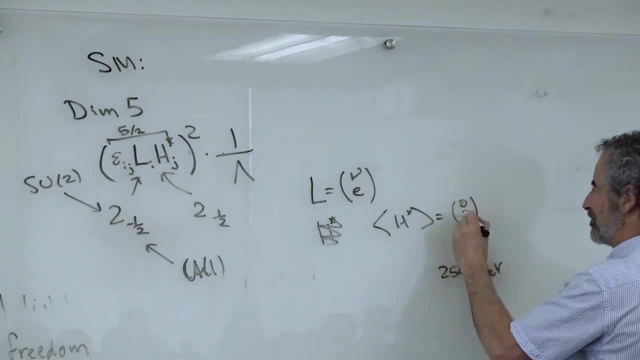 And when you contract with an epsilon- let's call this F- you get something that looks like nu, nu, F squared over lambda. So this looks like a neutrino mass. What's cool about it is that it's a neutrino mass from an irrelevant operator, so what? 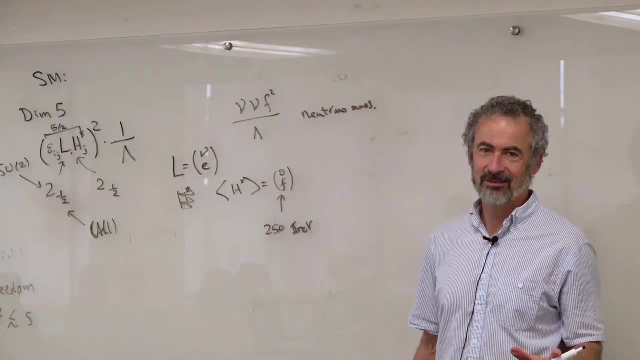 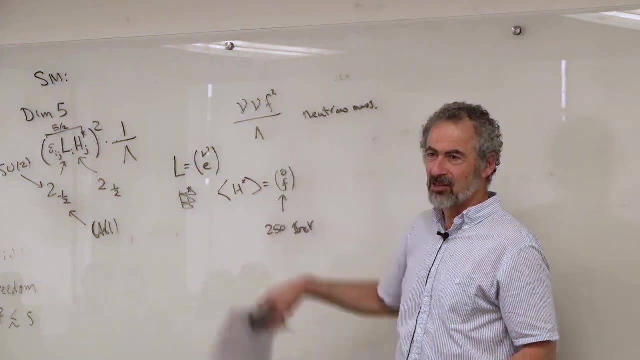 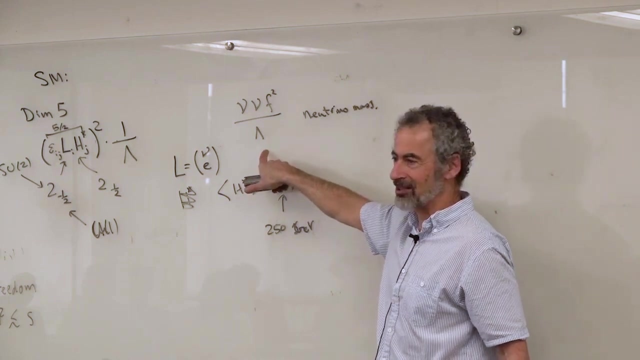 does that tell me about the neutrino mass 0. Very small, typically. If lambda is big, this will be extremely small. So this this is basically what's called the seesaw mechanism, which is that as lambda gets bigger- the scale of new physics- the neutrino mass gets lighter. 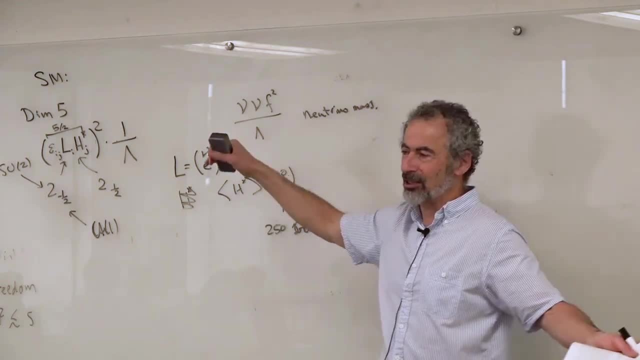 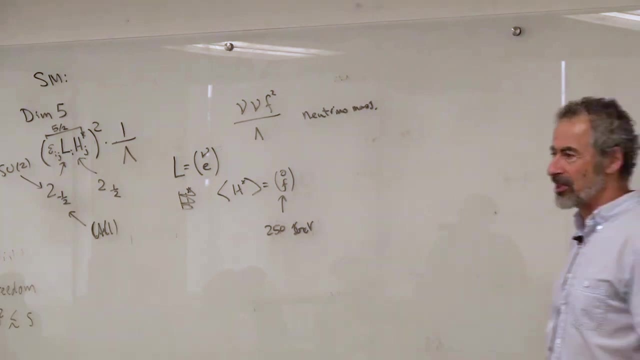 And in fact, if you take lambda on the order of 10 to the 13 GeV or something like that, you get neutrino masses that are very much around the scale that we see. So this suggests, when you now see neutrino masses, 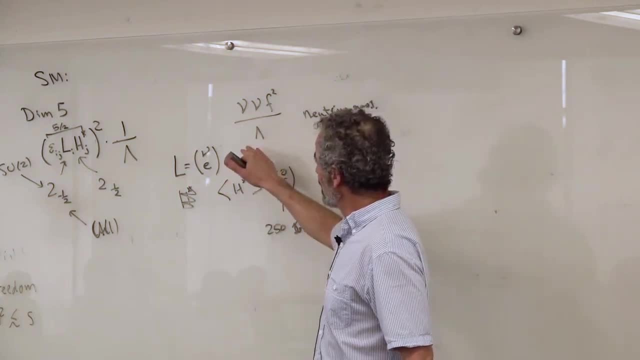 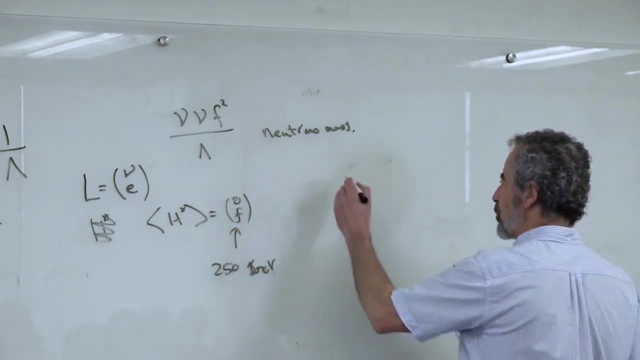 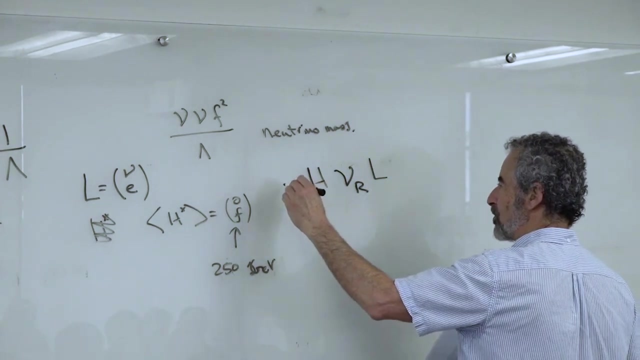 It suggests that you're going to. it's possible, but not necessary that you're looking at this operator. Why is it not necessary? Well, there could have been a right-handed neutrino in your theory, in which case it could couple to the lepton in the Higgs with the Yukawa coupling in a dimension 4 operator. 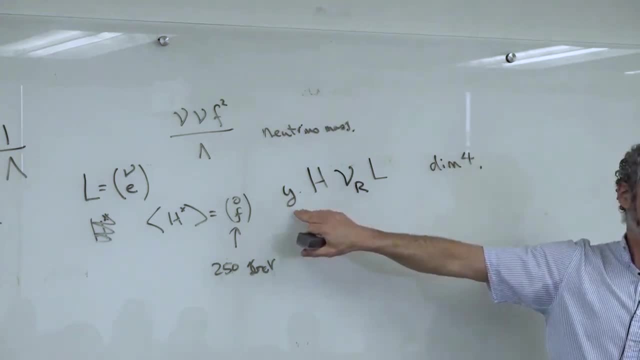 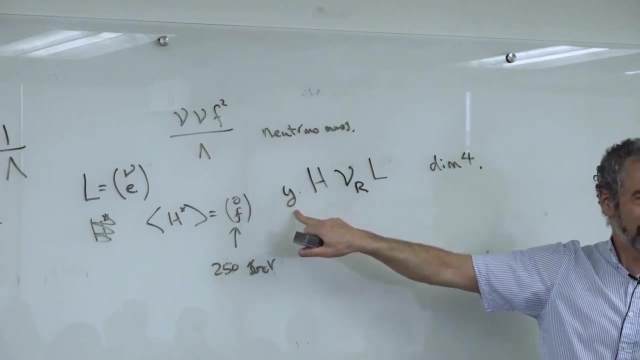 If you did this, then, given that the neutrino is around an Ev and the Higgs Vav is 250 GeV, this would have to be a really, really small number to explain a light neutrino mass. So you have to fine-tune this coupling to be tiny in order to get a light neutrino mass. 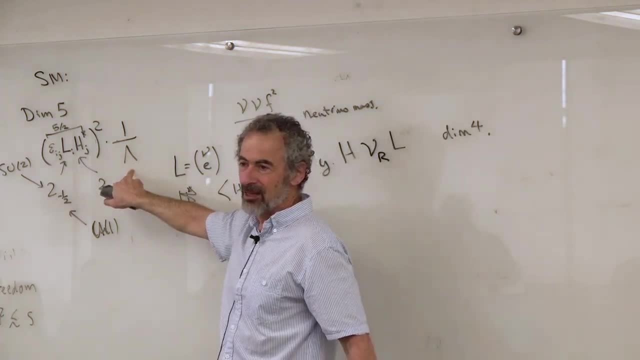 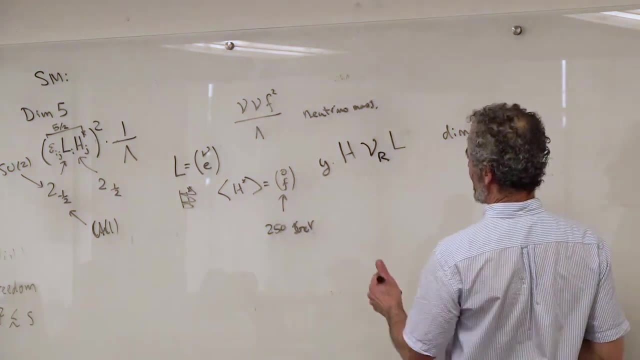 Well, here it's automatic if lambda is just a big scale for new physics. So the prejudice is that this is what we've got and not this. and there's another reason, besides saying that y has to be small: it's because I could just write nu R, nu R, you. 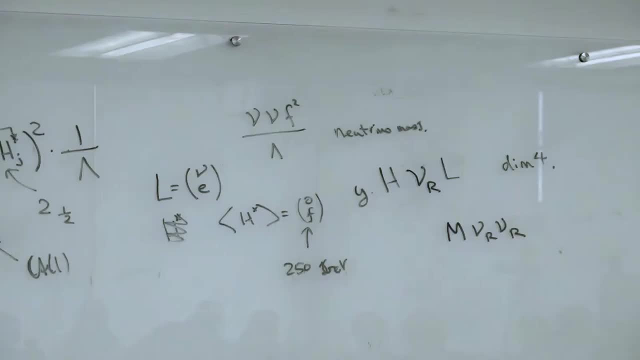 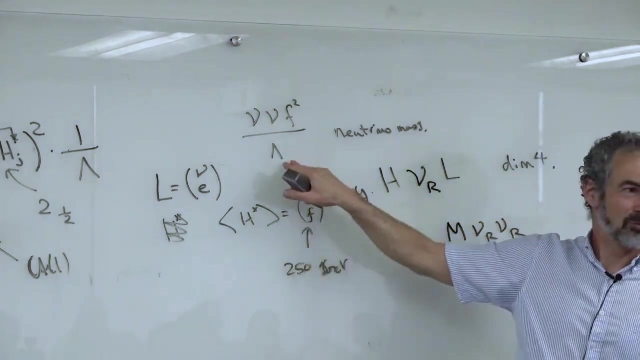 see, because the right-handed neutrino carries no quantum numbers Under the SU3 cross, SU2 cross, U1,, and so there's nothing to forbid me from putting it a big mass like the Planck scale, And so this seems unlikely, while this seems much more reasonable. 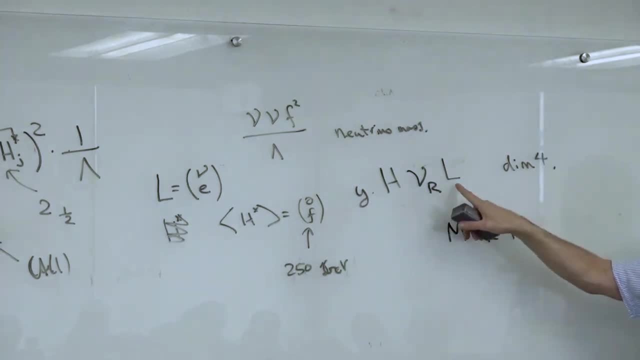 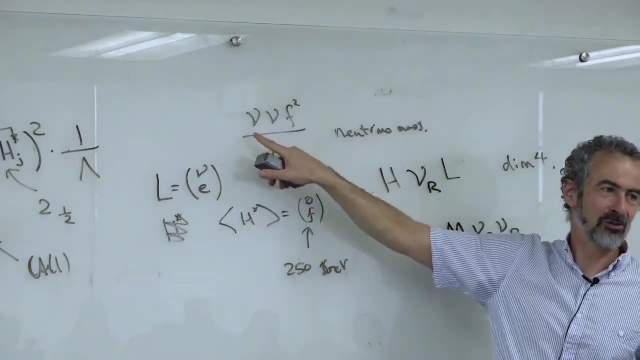 And you can tell the difference because this has a lepton number symmetry where this has charge 1 and this has charge minus 1, or vice versa. Well, this one does not. There's no rotation I can do on the neutrino. that leaves this invariant, because they're 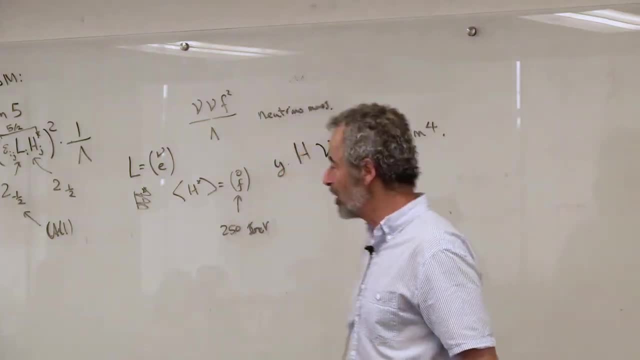 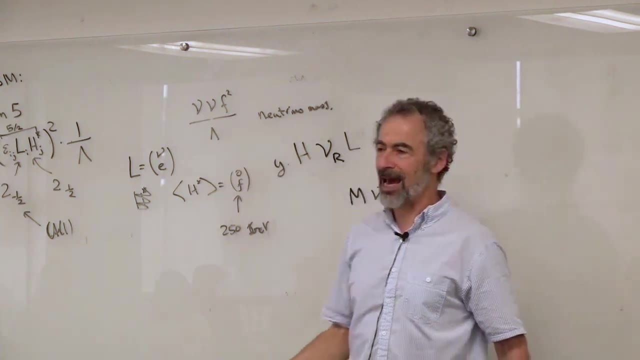 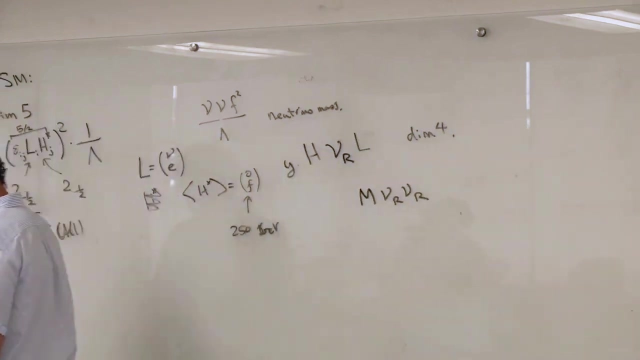 the same object. there they're not conjugated, So this involves lepton number violation. this does not. This can be seen in a neutrino. that's double beta decay, which couldn't happen unless there's a lepton number violation. So there are experiments to try to look for these things. 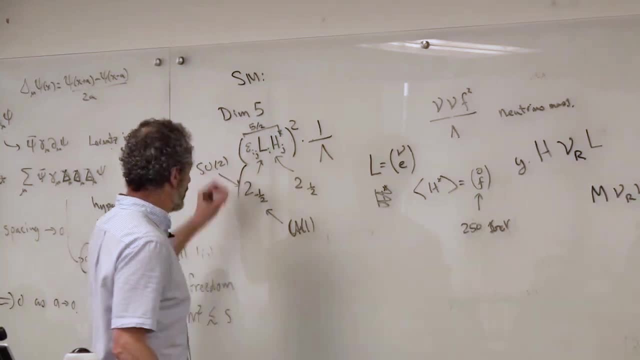 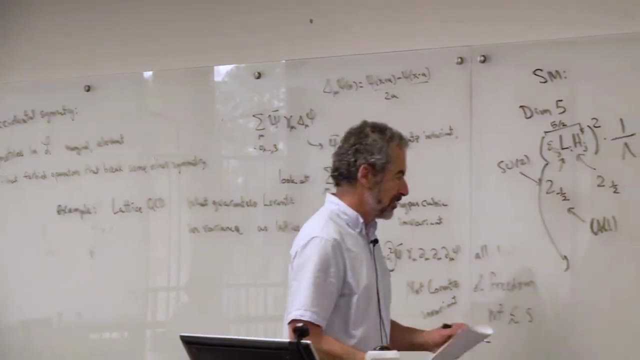 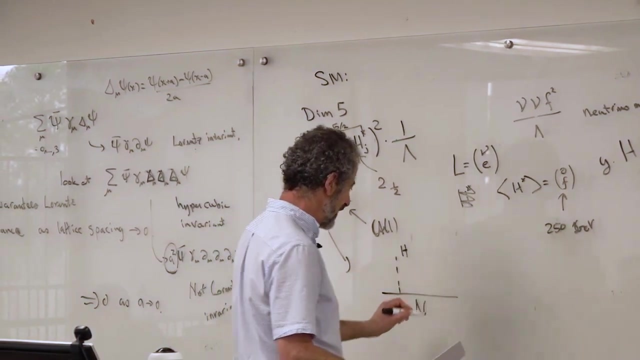 How would this come about from short distance physics? Well, there are basically two ways. you can draw a tree diagram that will give you that I could have my lepton And my And my Higgs And a heavy particle which I'll call n. 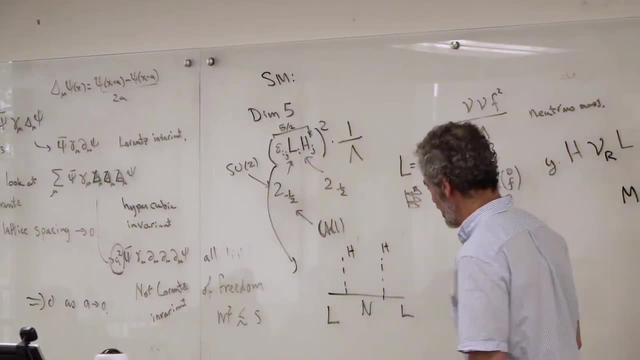 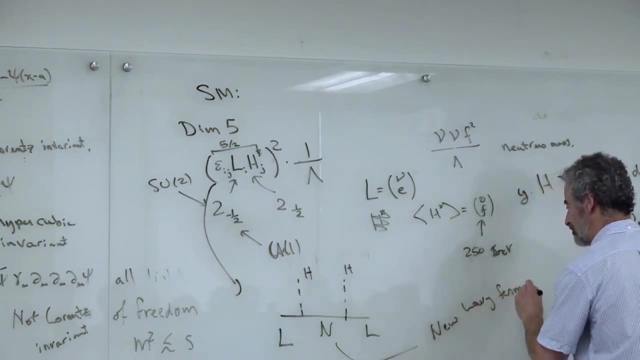 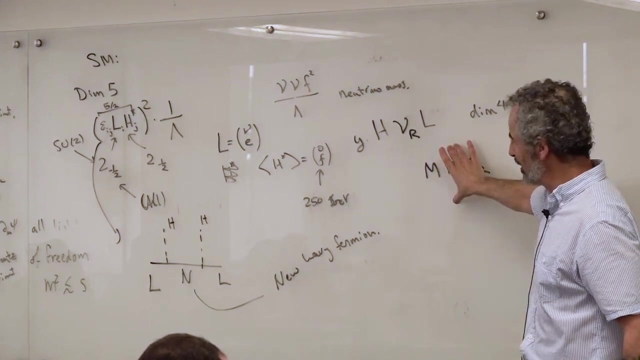 And a Higgs And a lepton like that. So that says that there is a U heavy fermion. In fact, if I had a Yukawa coupling to a right-headed neutrino with a heavy mass, then the low energy theory wouldn't have the right-headed neutrino in it because it's heavy, the effective theory. 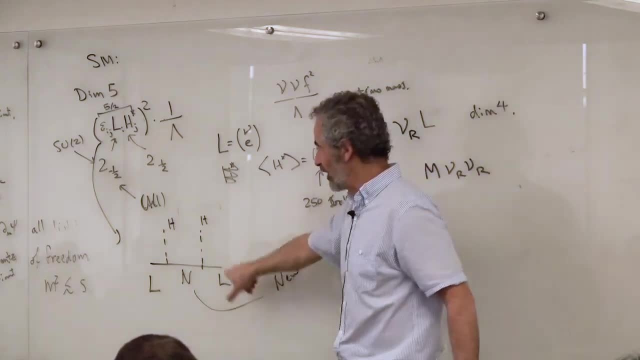 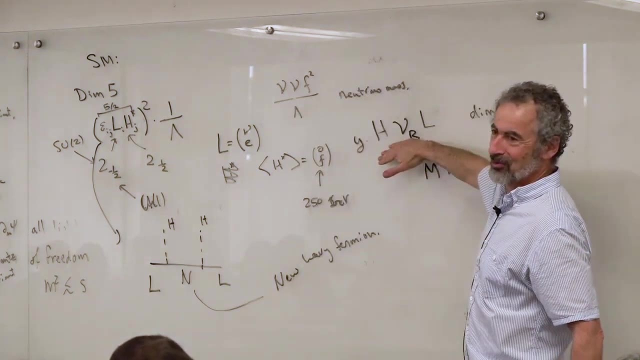 And the effect would come from this diagram. when I get rid of it, it would give me this operator. You say well, Wastelink. I thought you said that this preserves lepton number. It does, but this does not. 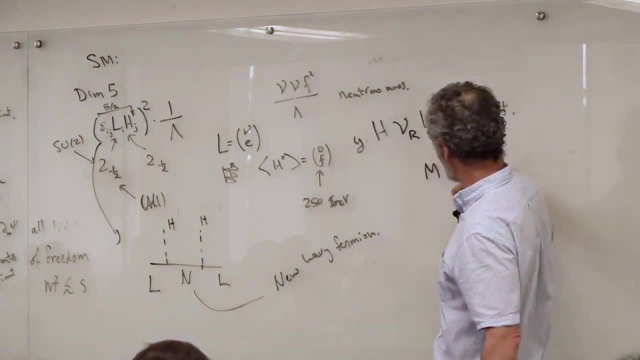 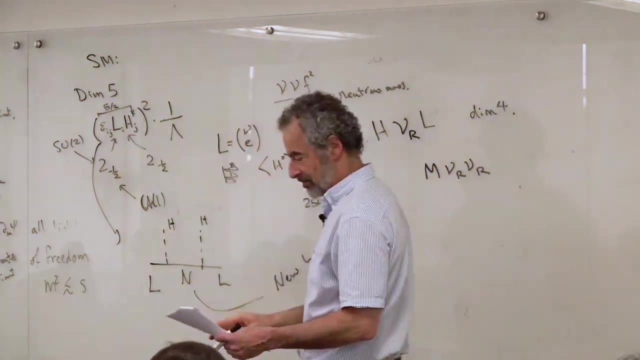 So this would come from a high energy theory that does not preserve lepton number. You integrate out, you come up with the effective theory. with no right-headed neutrino, this shrinks to a point. you get that operator. Well, Another problem. 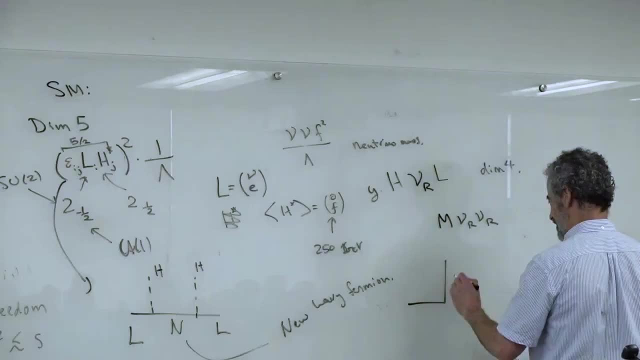 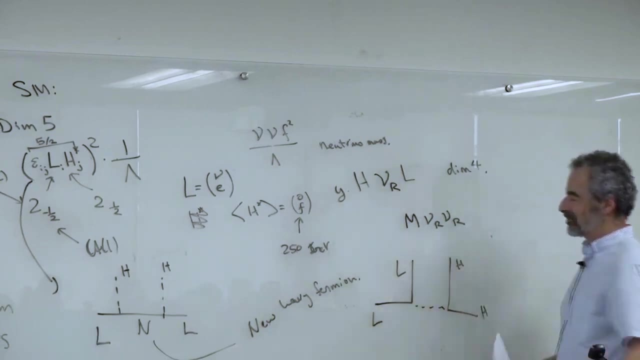 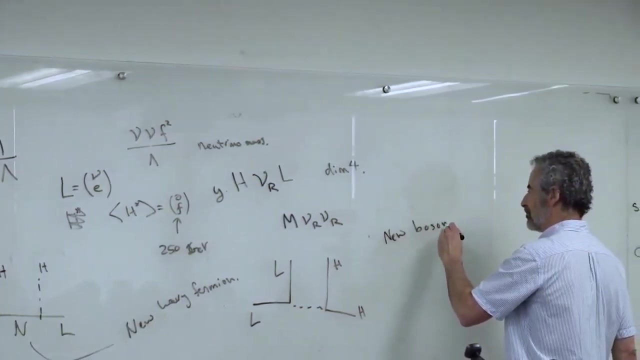 Another possibility would be: There's some object that is exchanged between a lepton pair and a Higgs pair. Well, this is a scalar, That's a scalar. So this would have to be a scalar, And I believe it could either be. 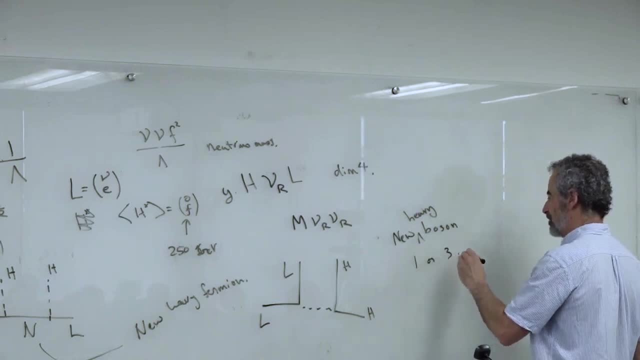 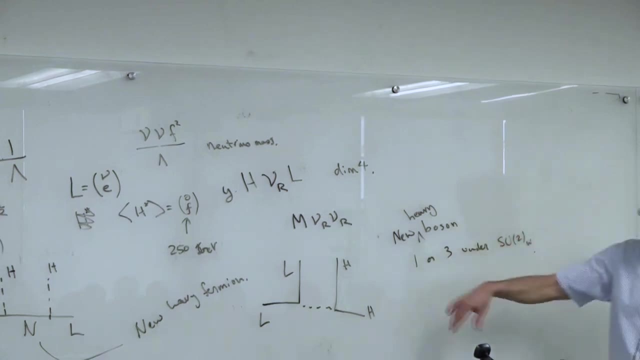 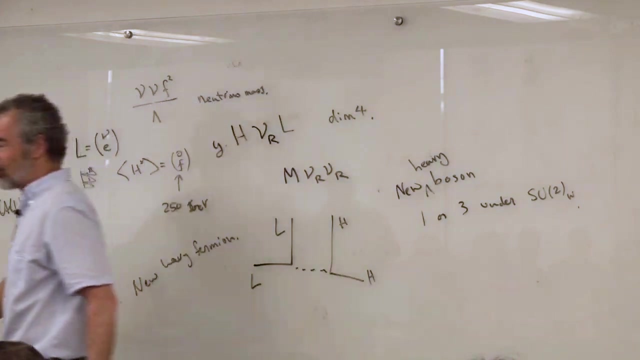 A 1 or a 3 under SU weak. So there are two different types of models. There's the singlet-Meyeron and the triplet-Meyeron model. So we don't know. We think this operator exists. we're not even sure. 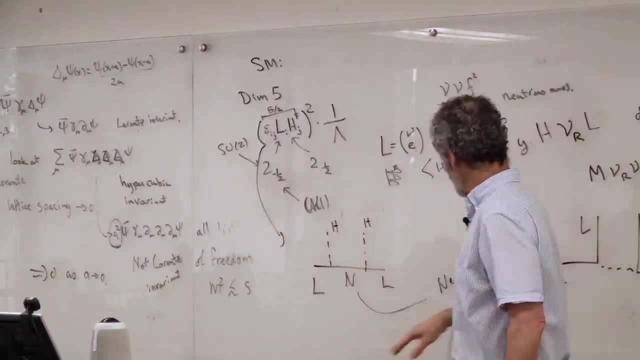 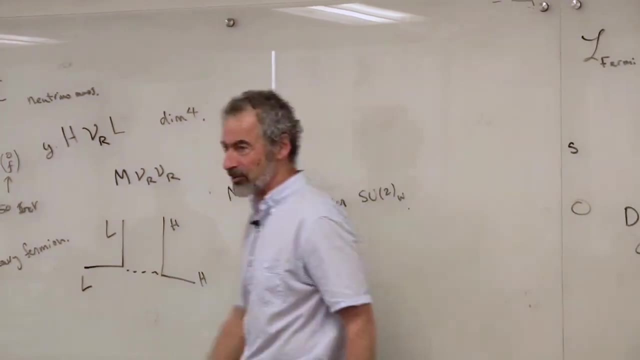 We certainly don't know where it came from. But you can start looking at these different models and say: how would that affect cosmology? Is this helping with baryogenesis or other things? And so People play around with this, And this is an example of the short-distance physics giving us hints about the long-distance. 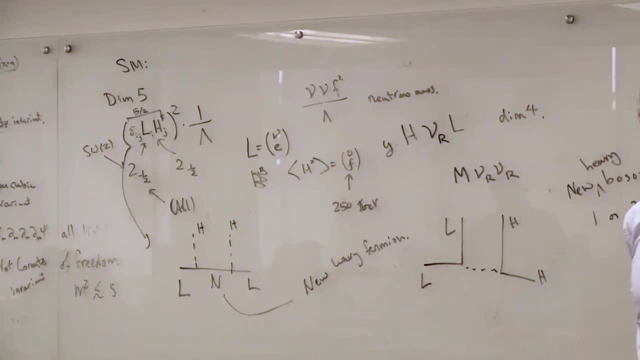 physics: Yes. What's the suggestion for the scale of lambda? I'm sorry, My hearing is terrible. Please speak up. What's the suggestion for the scale of lambda? for lambda, What's the Suggestion for the value of lambda? 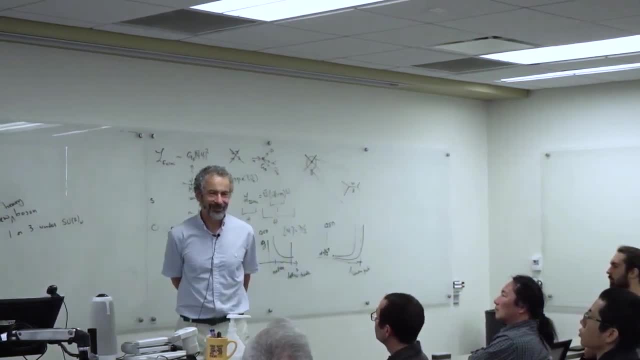 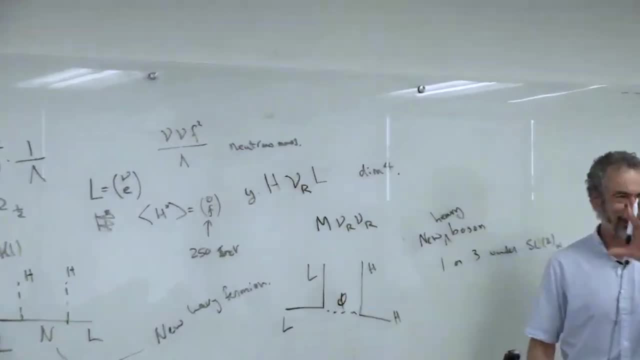 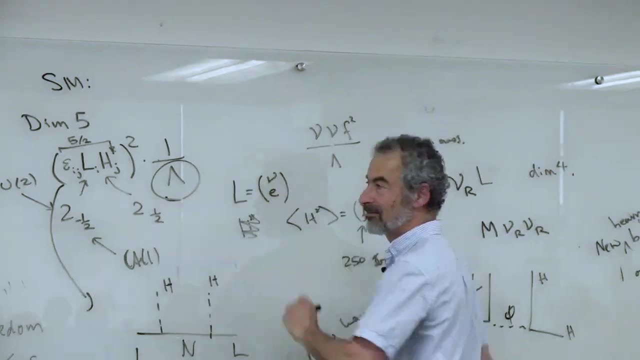 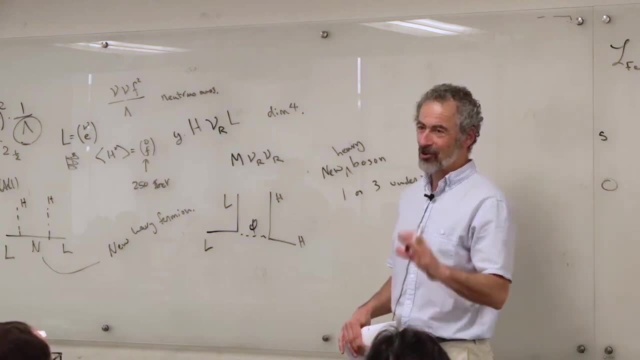 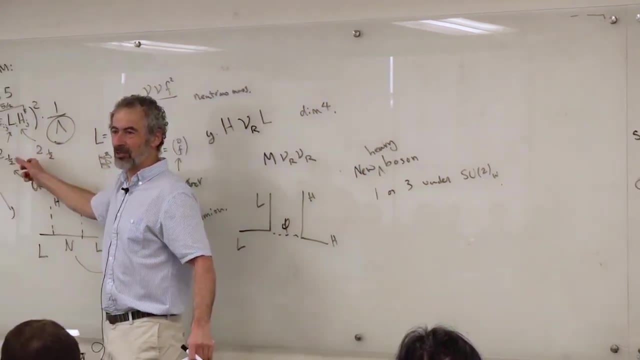 Ah, so numerically we don't know, OK. But we know from neutrino masses that we know there aren't any neutrino masses that say 10meV, so we know this has got to be bigger than something. OK. 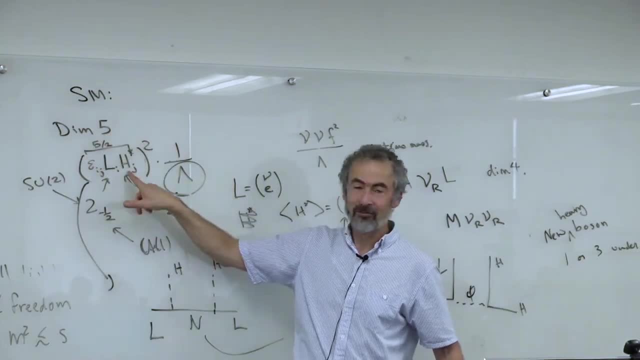 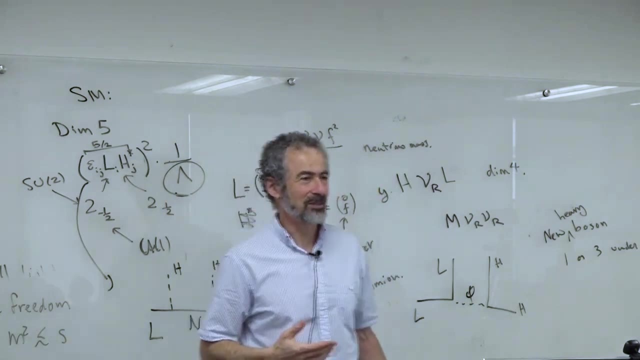 And if you want to get this, to give you the right, since we know the VEV of the Higgs and we know that the neutrino mass splittings are on the order of 10 to the minus 2 eV, something like that. 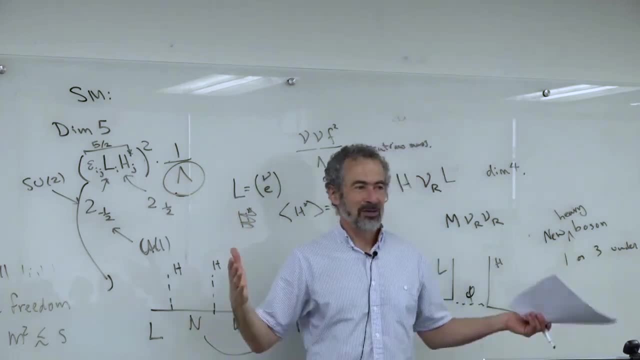 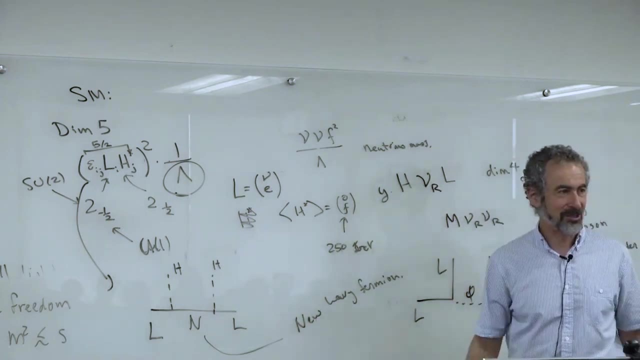 then we can get an estimate for lambda. that it's somewhere, and it'll depend on the coupling constants too. It could be higher scale and smaller couplings, but probably above 10 to the 13 JeV or something Interestingly close to the same scale you see in grand unified. 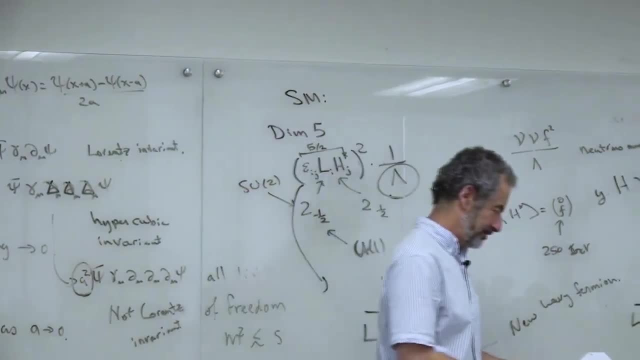 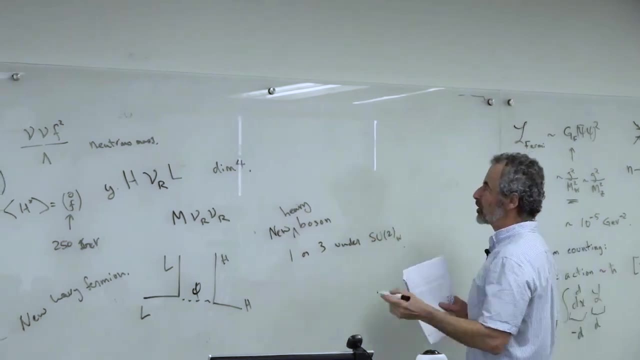 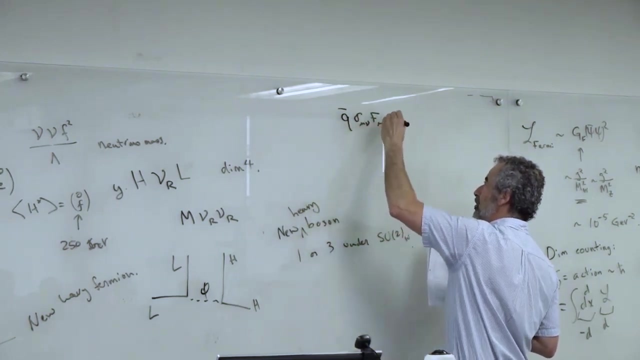 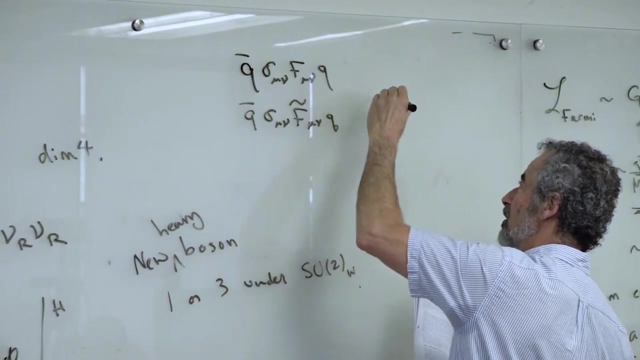 theories which I'm going to come to. next. There's a couple other dimension 5 operators you could write down, which are: Q bar sigma mu nu F, mu nu Q and Q bar sigma mu nu F, dual mu nu Q or Q are quarks. Well, actually they could be also leptons. 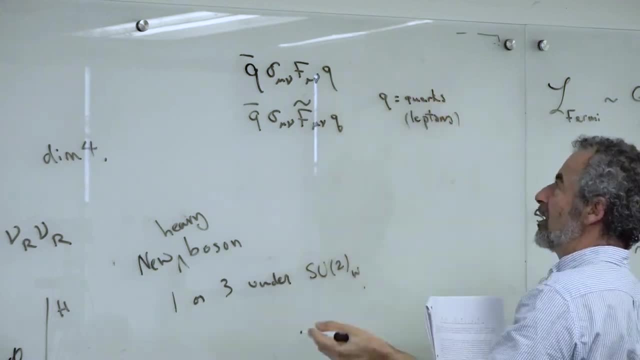 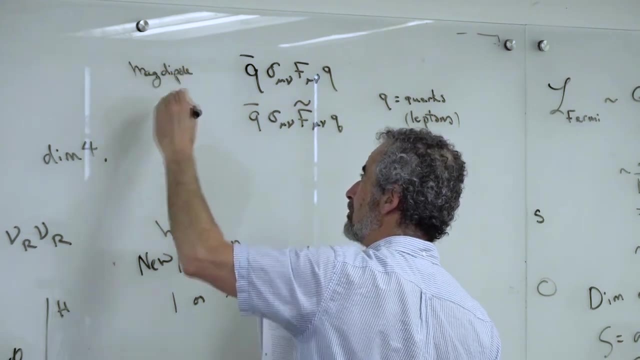 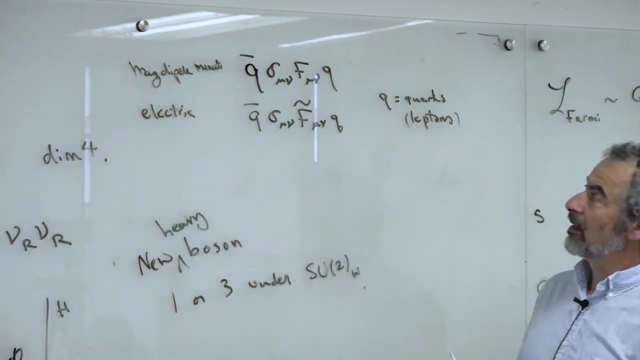 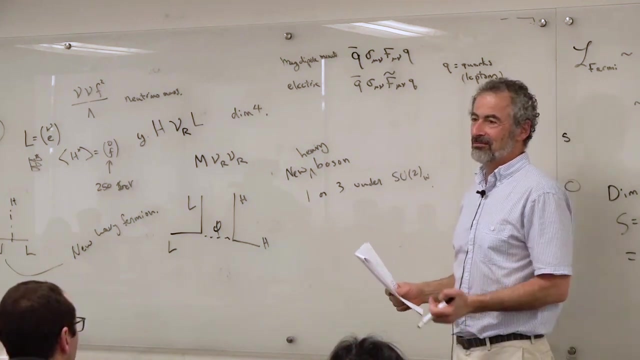 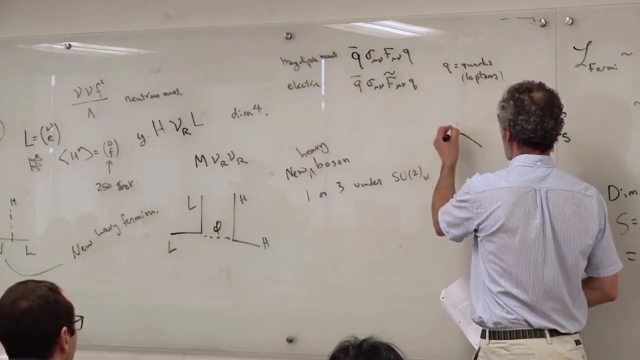 And this contributes to a magnetic dipole moment And this is the electric one. Now we know that at very low energy. we know the neutron has a magnetic moment but it's chargeless. So the usual way of getting a magnetic moment from a coupling like that doesn't exist for the neutron. 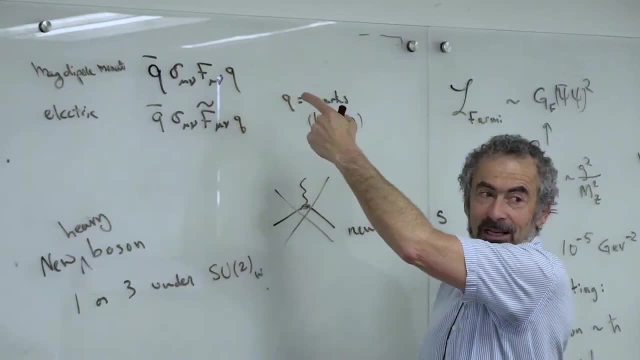 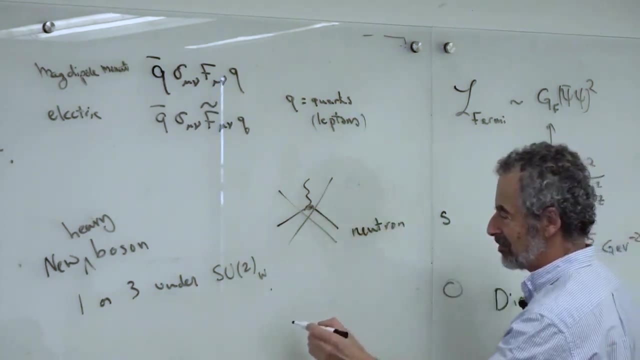 So the neutron magnetic moment would have to come from an operator like that, if you're looking at a low energy theory And you can explain this by saying: well, there's some say that there was a charged particle here. so the neutron turns into a proton and a pi. 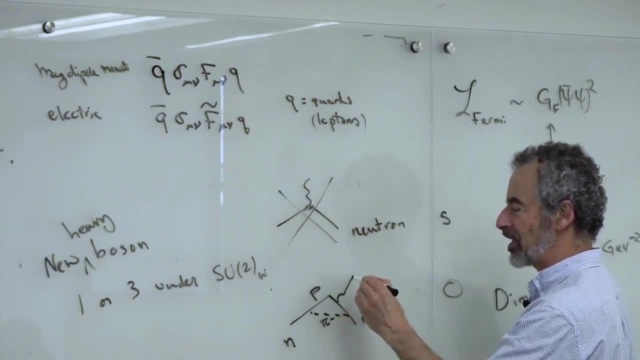 minus and then back into a neutron and then the photon could couple here or the photon couple there, because those are charged particles And that could be the origin of the neutron magnetic moment, When I think it was Robby who discovered that the magnetic moment of the proton wasn't. 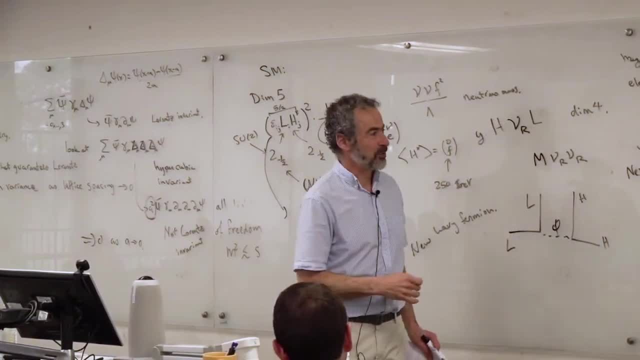 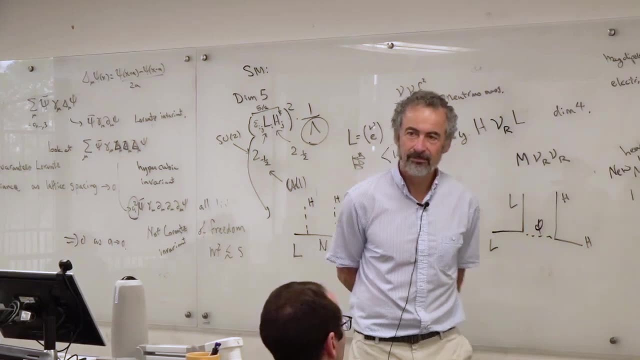 g wasn't equal to 2, which is what the Dirac theory predicted. it was the first evidence that the proton is not a point particle but could be described with the Dirac equation. Yeah, So are you saying that the particle is not a point particle? 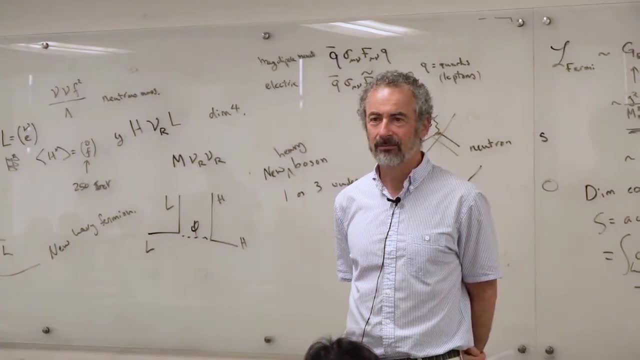 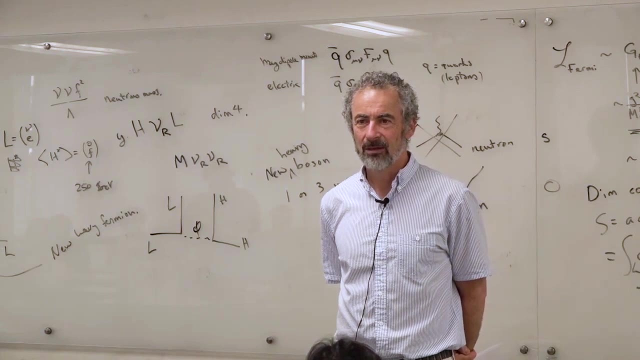 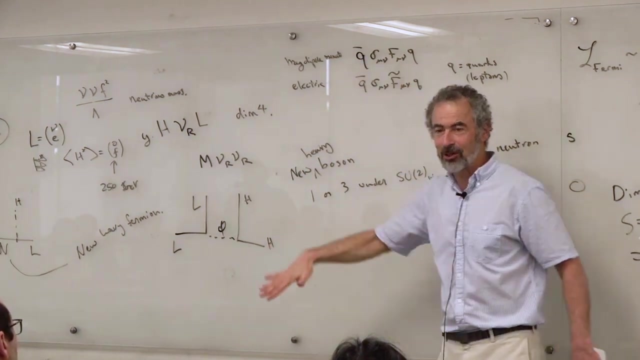 Yeah, So are you saying that the particle is not a point particle? If I'm at low energy, I can write down an effective operator like this, and if I'm at extremely low energy, say below the pi in mass. this is sort of a picture of what short 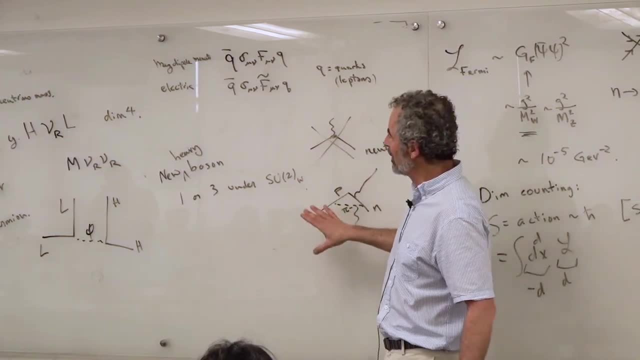 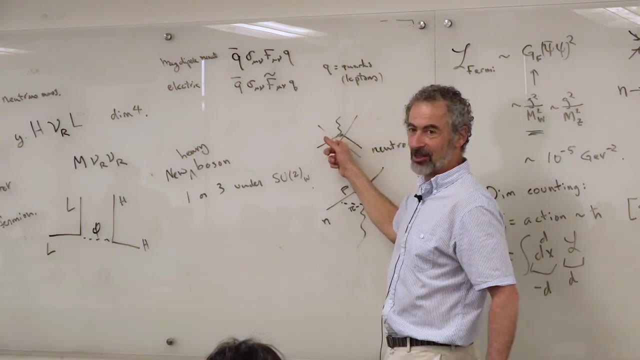 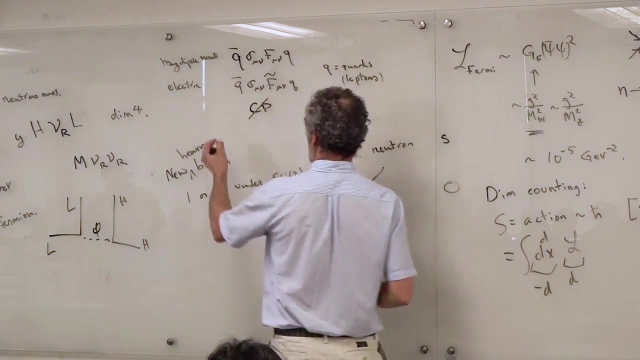 distance physics could have given rise to it, But this is not that interesting because magnetic, especially for charged particles, because they already get a magnetic moment from this operator here. This, however, violates Cp And in particular it gives an electric dipole moment to the. 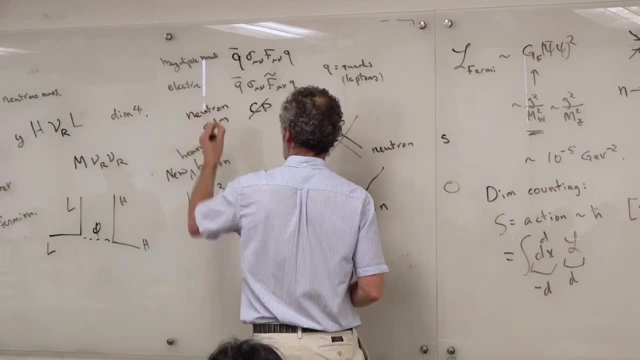 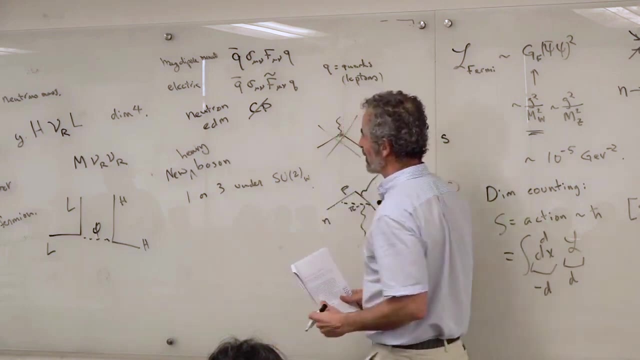 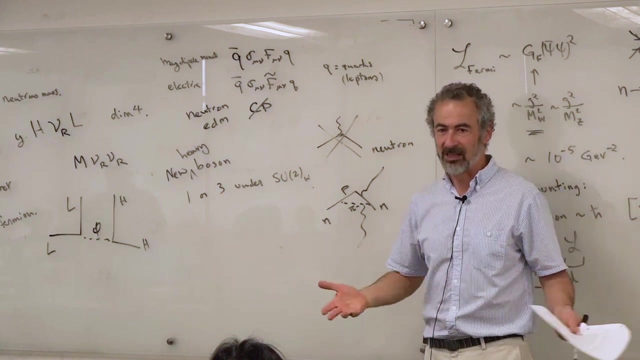 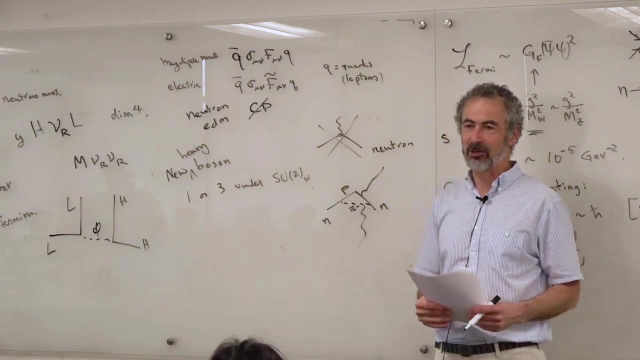 neutron, And so there are extensive experiments, many experiments, looking for a neutron electric dipole moment, because we've seen Cp violation in the standard model through, say, k-on decays, and we know we need Cp violation if we want to explain the origin of matter in the universe. 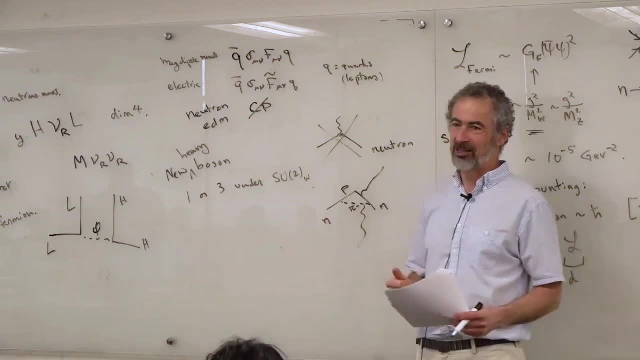 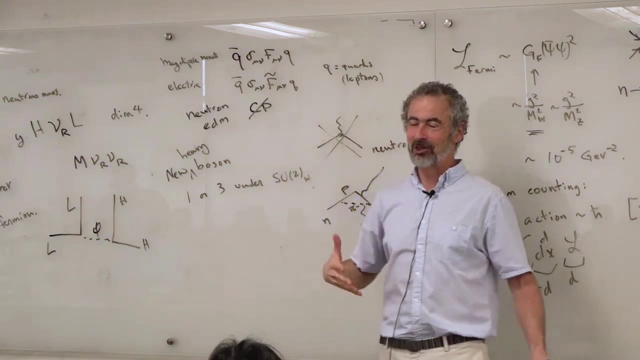 baryogenesis coming from scratch because baryons violate Cp. If you start it off- for I mean because if you do a charge conjugation transformation on our universe, it turns into antimatter and doesn't look the same at all. But if it starts from equal matter and antimatter, 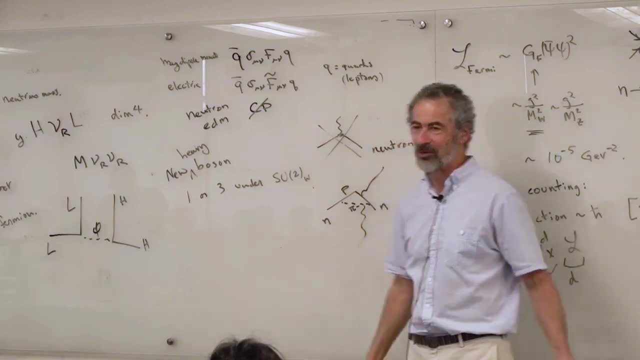 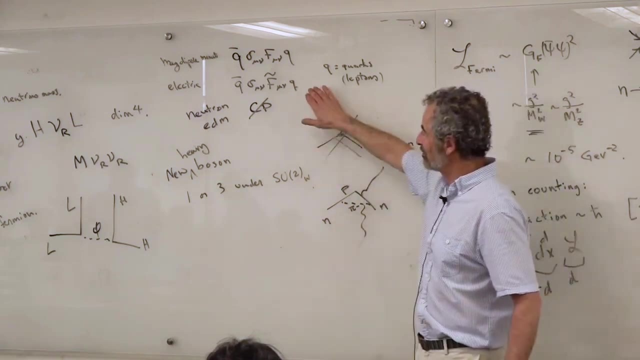 then somehow charge conjugation must have been broken, and it turns out parity too. So it's interesting to look for new sources of Cp violation, And so far they haven't found it. They've put bounds on this, So this is a tricky operator. It looks like it should have a 1 over lambda in front of. 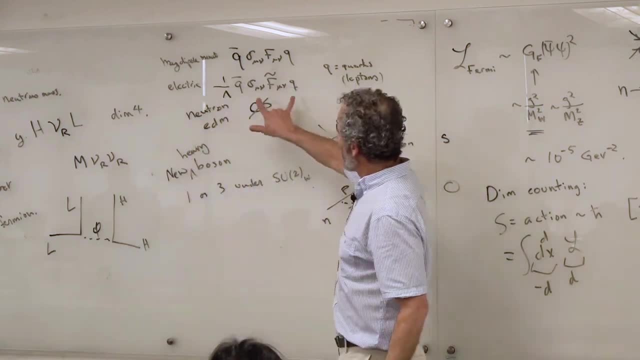 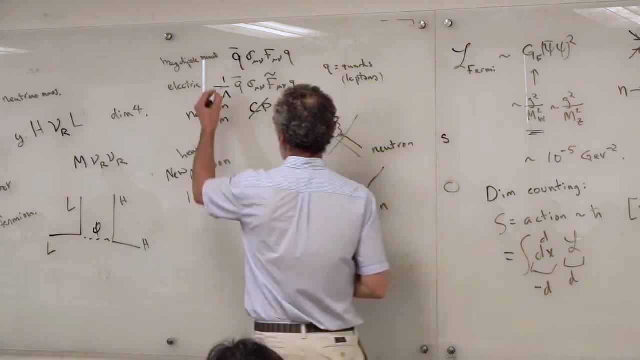 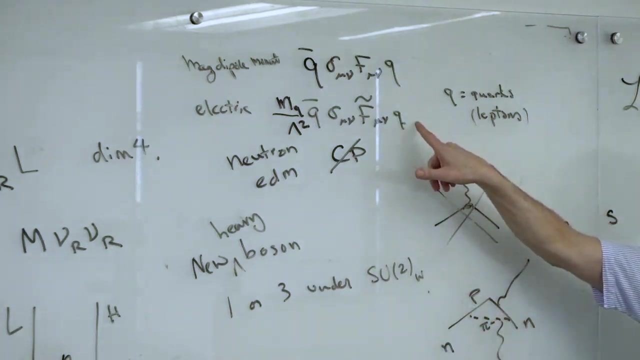 it because it's dimension 5.. But it violates chirality. It mixes left and right. So in most diagrams you could write down: you get a factor of the mass of the quark upstairs and you get a lambda squared downstairs. So usually this behaves like a dimension 6 operator. 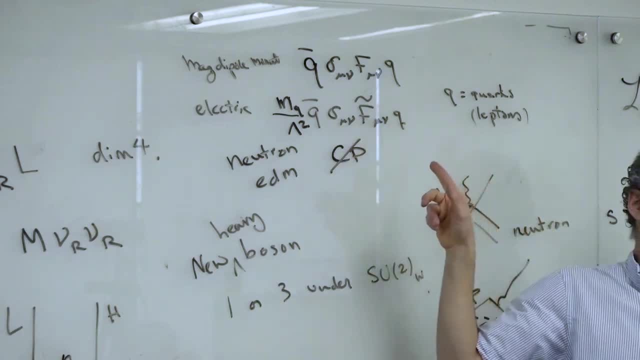 because the only way that chirality works is if you have a 1 over lambda in front of it. The only way that chirality can be violated in your marginal and relevant operators is through the quark mass. And so if you look at a diagram that connects the left to a right, 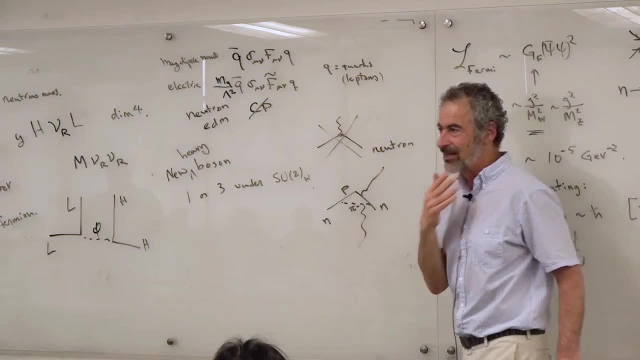 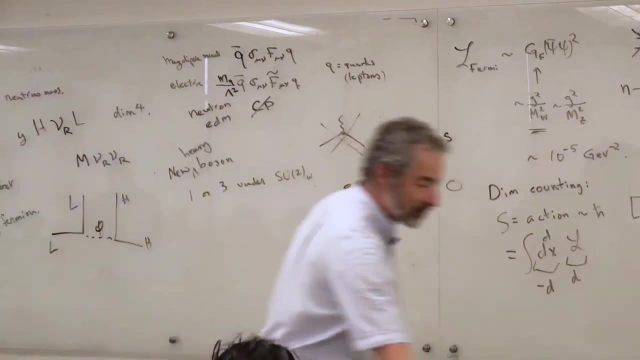 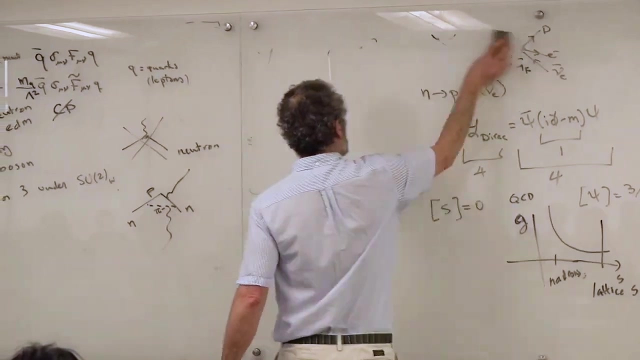 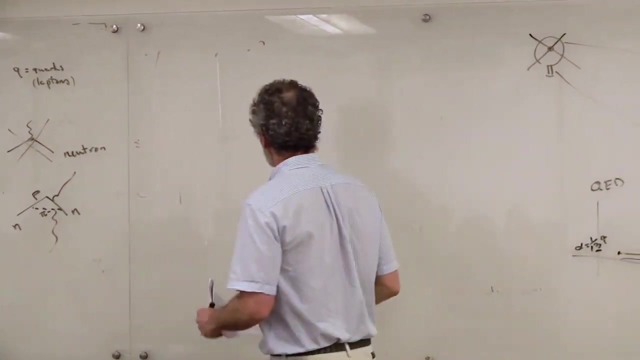 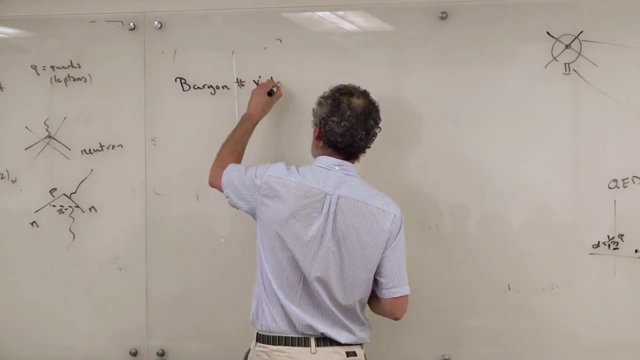 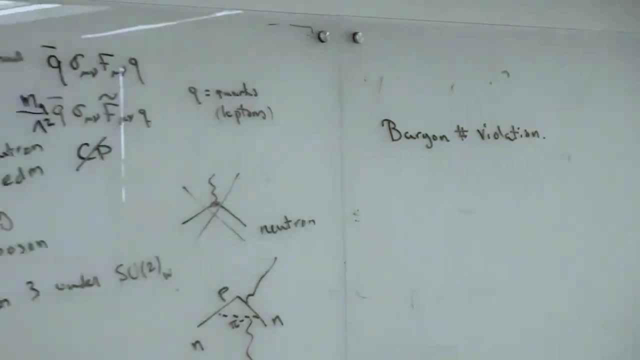 headed quark, it typically will have a power of the quark mass in it, So this behaves like dimension 6.. Other dimension 6 operators, though, are fascinating. We'll go over that in a minute. Barrier number violation: Conventionally we think of a proton as a stable particle. 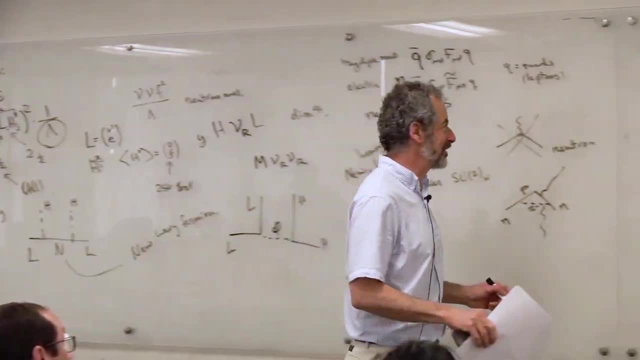 but it might be radioactive. it might want to decay. For example, if barrier number wasn't conserved, it might be able to go to pi 0, or something. But this sort of thing doesn't make sense. Now, when we're looking at regular particles, you might want to decant them. 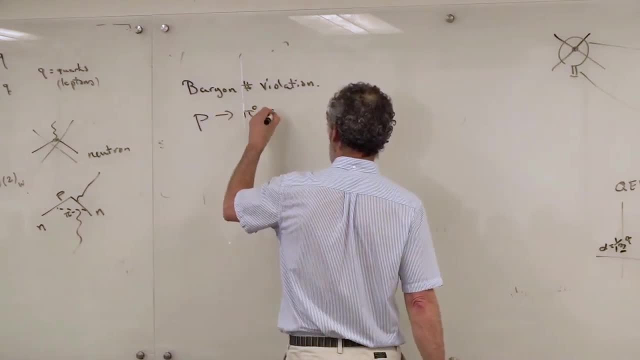 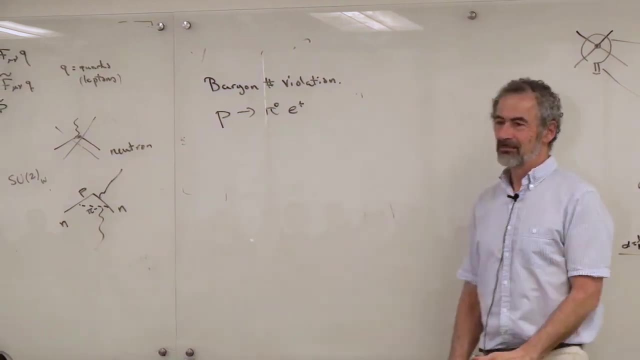 So well, this probably isn't the best way to do it, Not that you need a boundary number violation, But we think of it as a stable particle, just zero, and a positron That conserves charge. It's got a fermion on both sides That would. 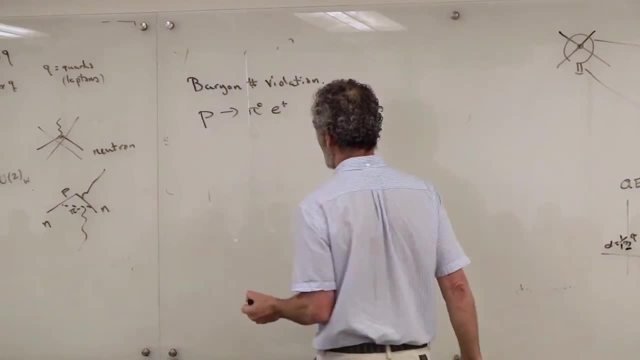 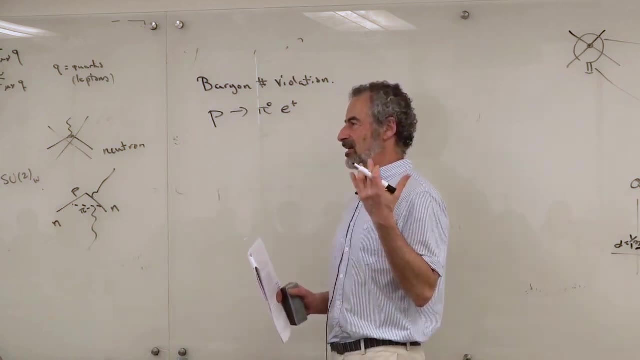 be a disaster for us if it happened at any speed at all. Well, I can write down an operator that violates baryon number, but it's going to have to have. the quarks are colored and in order to carry a baryon number I have to have quarks and not quark and anti-quark. 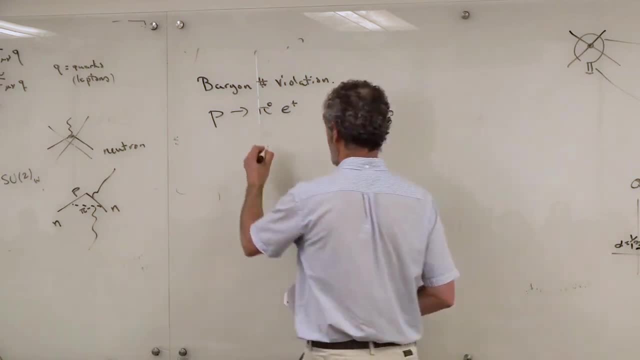 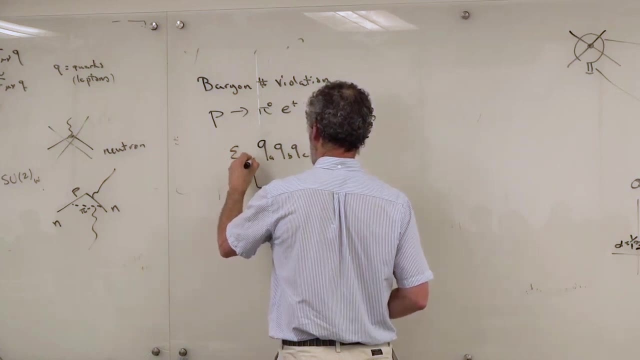 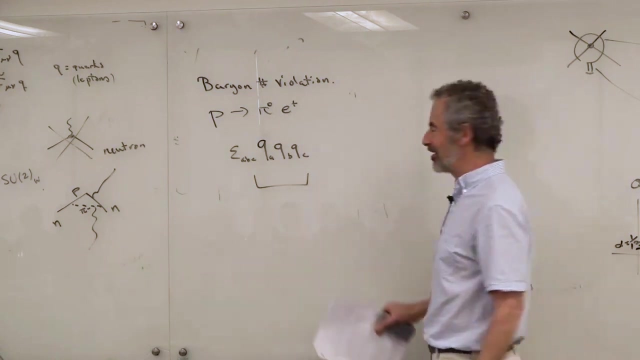 So I have to have at least three of them to make a color-neutral object. So this would be a, b and c with an epsilon to make it color-neutral. And now that's a fermionic operator because it's got three fermions. so I need another fermion in there So I could. 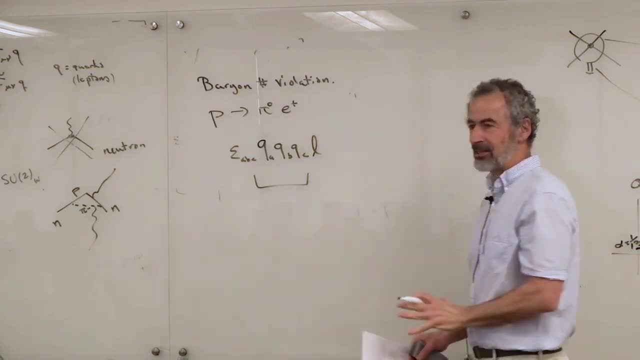 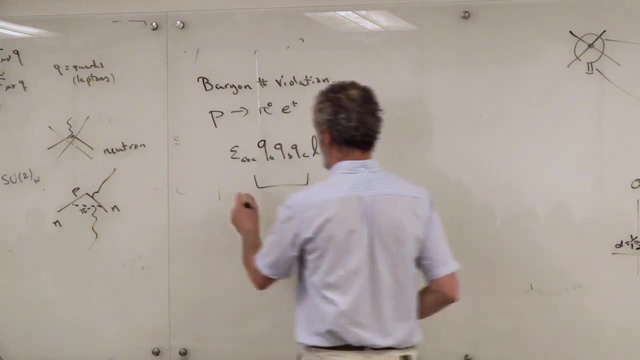 put a lepton there And it turns out you can make operators like this. There are quite a few, especially when you include multiple different types of flavors. Many operators like this. This is four fermions, so it's dimension six And so it's going to have one over lambda squared in front of it And it can be used. 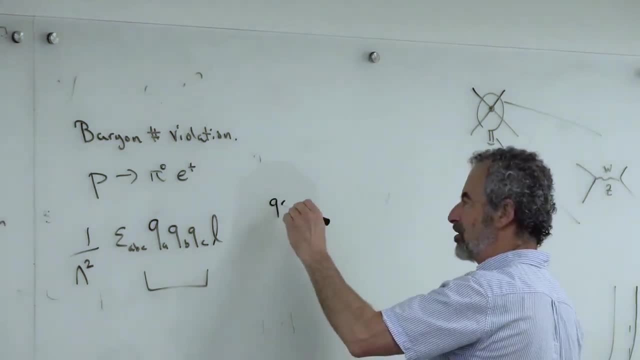 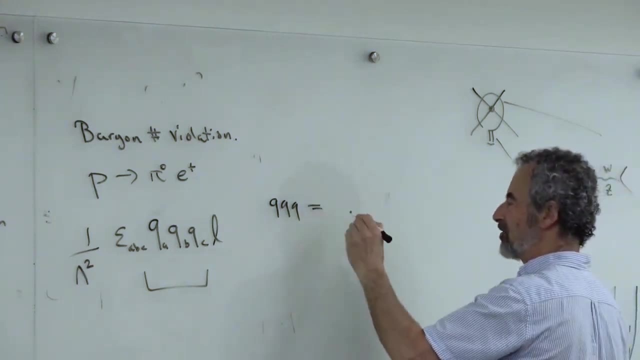 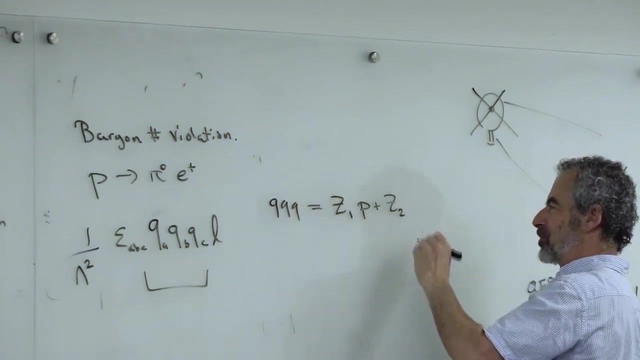 to do something like that because I can write q, q, q, That operator. when I go down to an effective theory of the strong interactions, I can think of that as with some amplitude z1 producing a proton plus some amplitude z2 producing, say, a neutron and a pi plus. 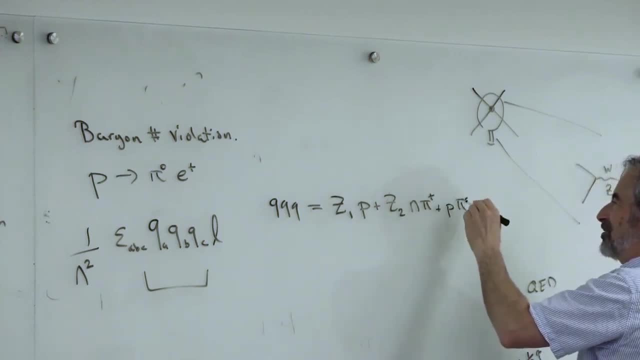 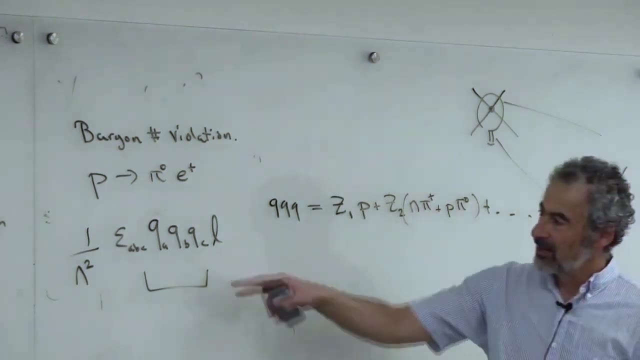 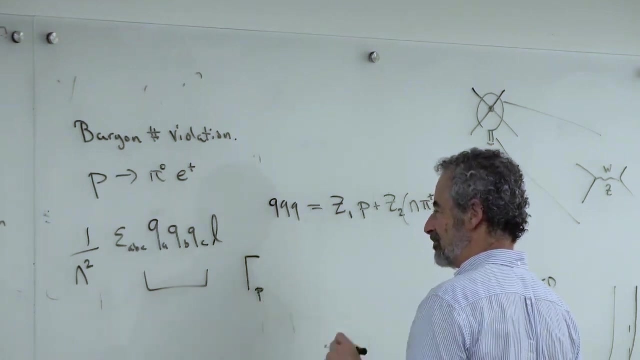 or a proton and a pi plus And a pi zero, And so on. So dimensional analysis: What is the proton lifetime? Well, let's look at the proton width. You get this from squaring a Feynman diagram, So it's going to have to go like one over. 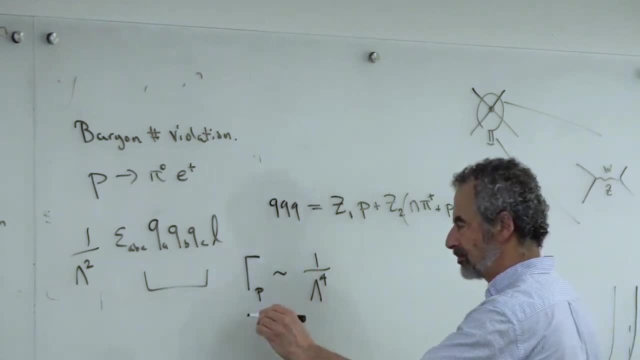 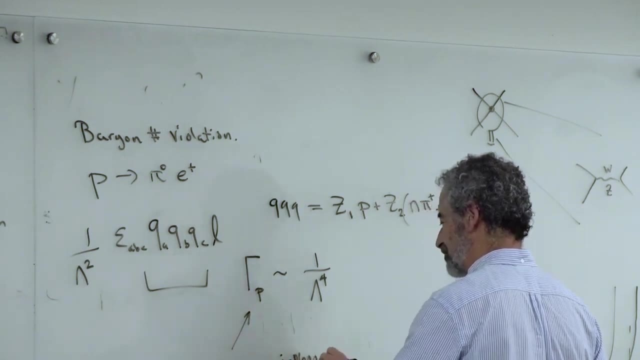 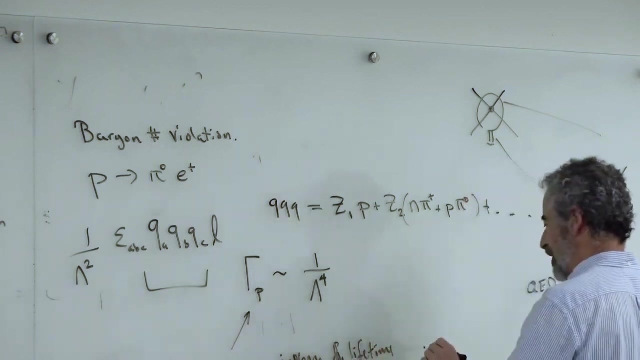 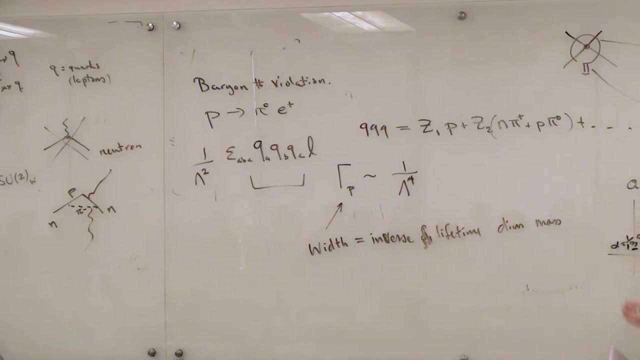 lambda. to the fourth: This is the inverse lifetime, So its dimension is mass, Because a lifetime is a time which has dimension, inverse mass. You have an inverse lifetime, So it's got to have some mass. to the fifth out in front: 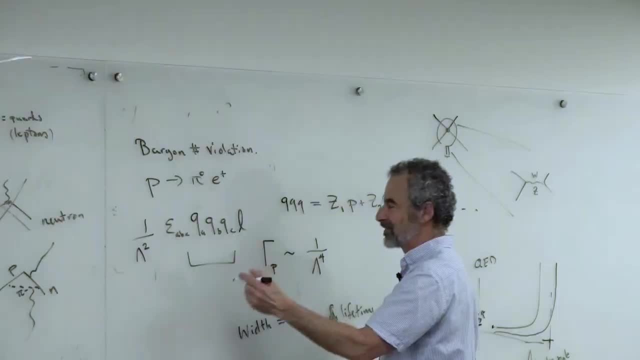 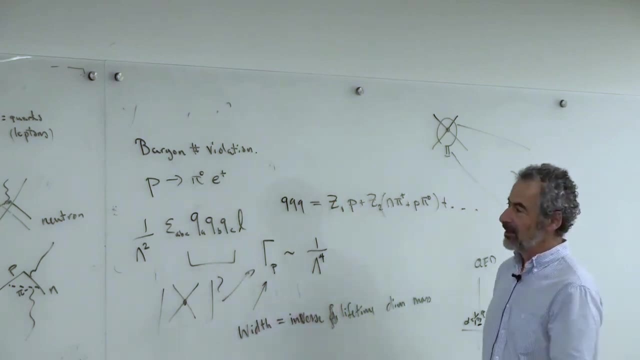 Suppose you're looking at it and it must come from phase space. So here's the diagram. It looks like a Fermi interaction. I'm squaring it To get that. well, again, phase space. So let's imagine the pi zero is. well, it is. 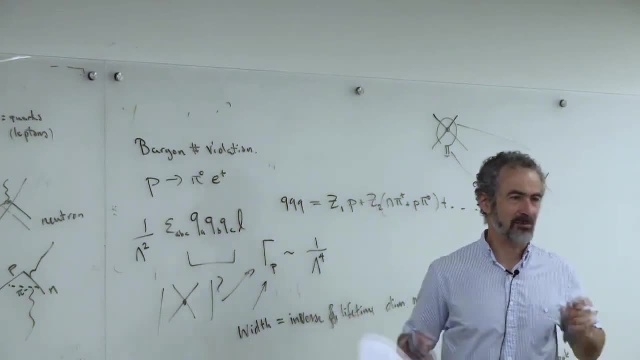 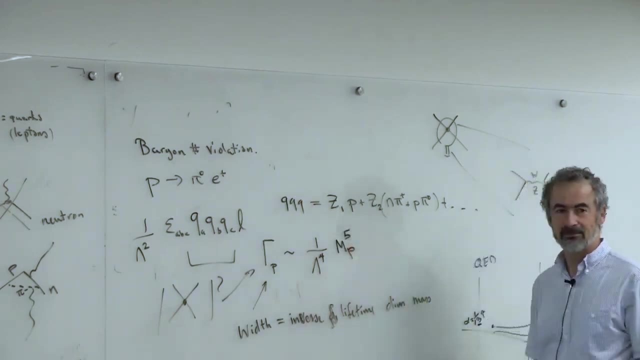 much lighter than the proton. So the only scale around really is the proton mass, That's how much energy is going into the outgoing particles, And so you expect something that goes like m proton to the fifth out in front, And we have phase space integrals and so on. You also get one over four pi's and so on. 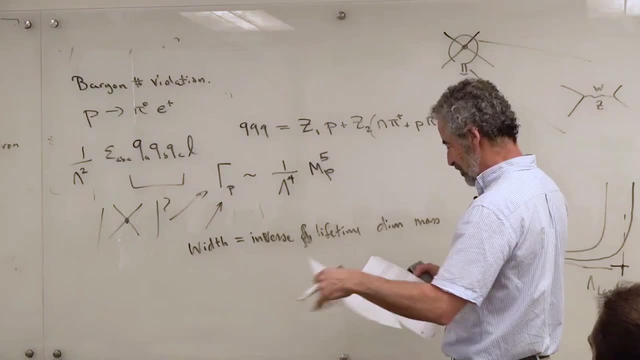 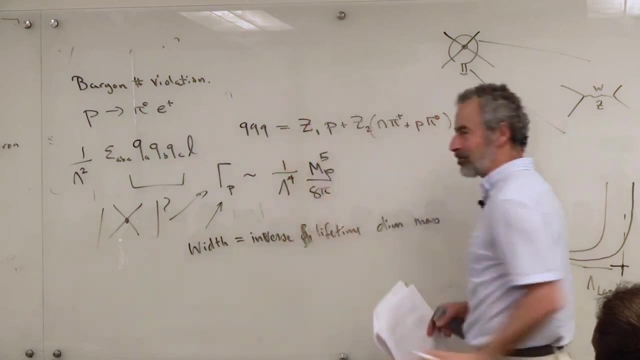 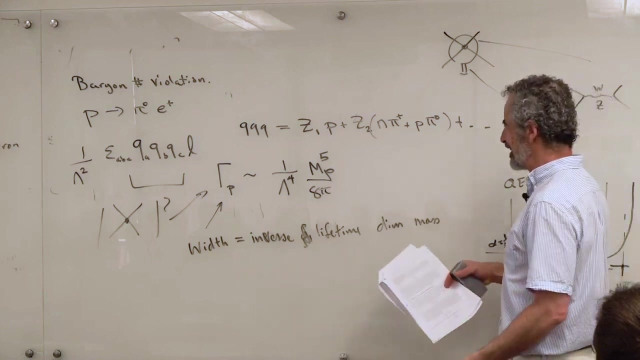 I won't try to estimate those, But Okay, All right. Well, actually, for two-body finals, you typically get a one over eight pi. Counting pi's is more of an art than a science, Unless you do the calculation. 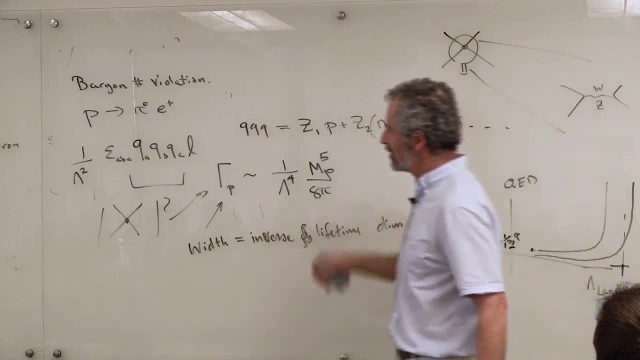 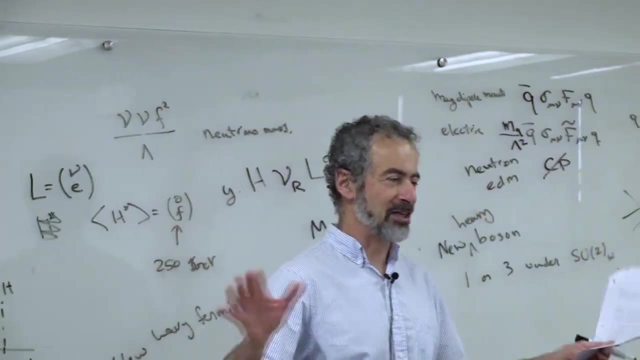 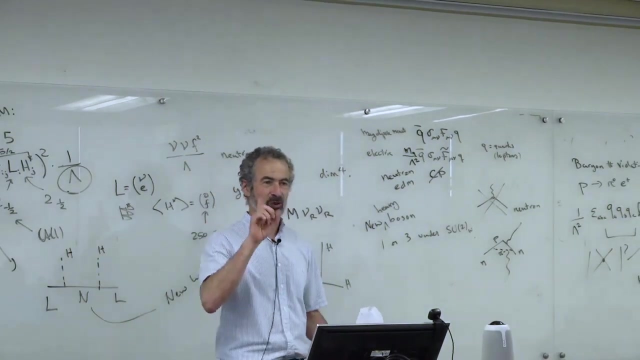 So when grand unified theories were first discovered by George and Glashow, they worked out the group theory together. It was really cool. You could put all of SU3 cross, SU2, cross, SU1 in a single group, SU5.. There's only one coupling constant. 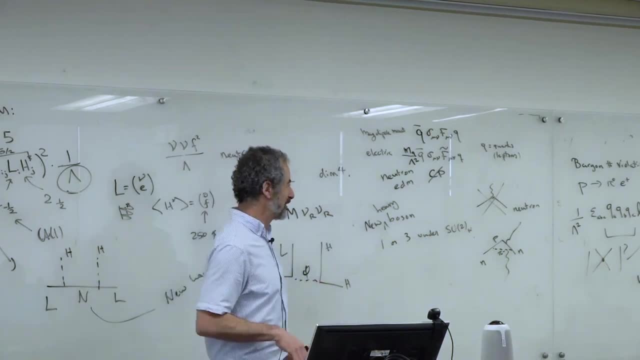 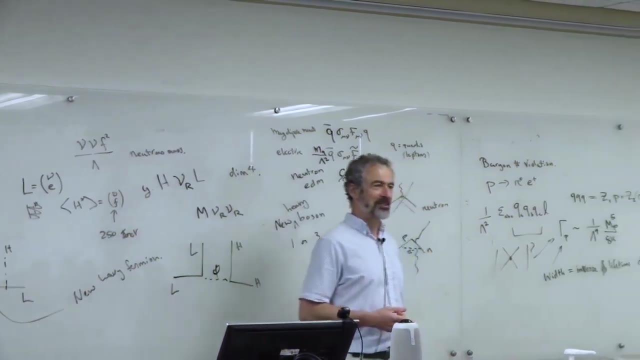 So you can relate the electric coupling constant to the weak to the strong Seemed really cool. Georgia goes home after dinner, sits down to work out some details of the theory and discovers: oh no, it violates proton number. Proton number. 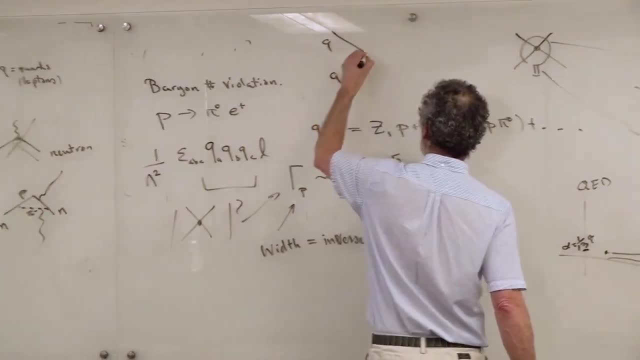 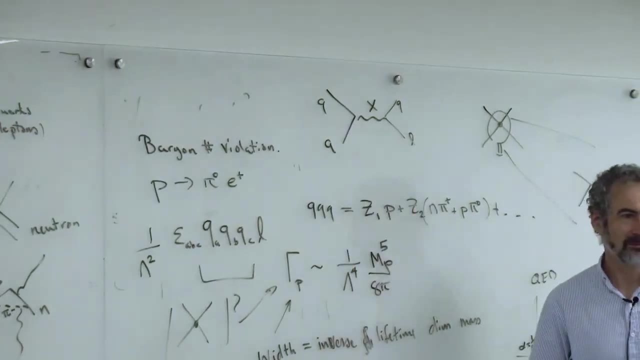 Barion number, Because there were graphs where you could have a Q and a Q, And then they had colored gauge bosons, which I'll call X, which could turn into a Q and an L. Yeah, All right, All right. 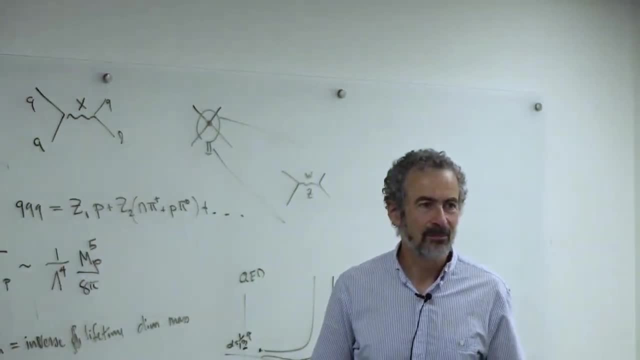 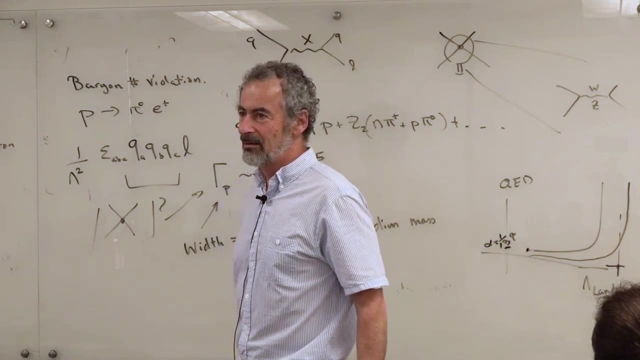 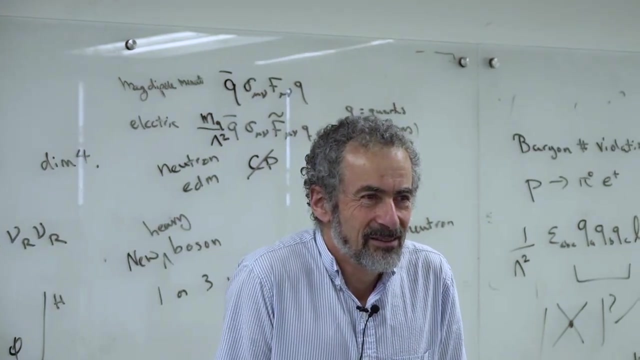 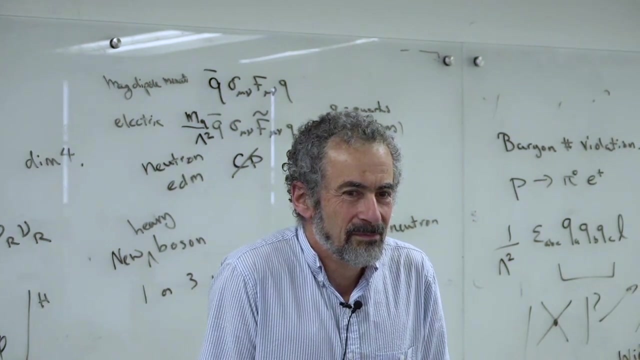 So. So the basic assumption is that some UV completion to some higher energy theory that is renormalized. Is this assumption that the theory for any of these operators is renormalizable at some higher energy scale? and this is some UV situation of this. 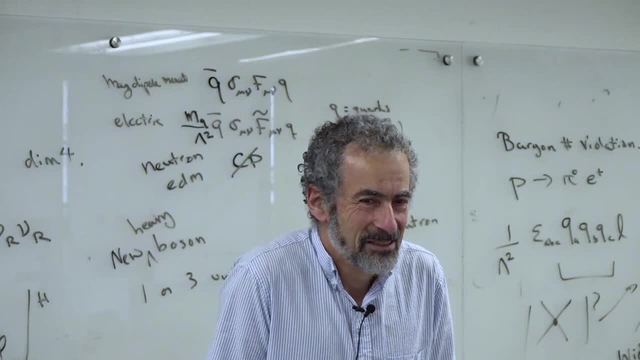 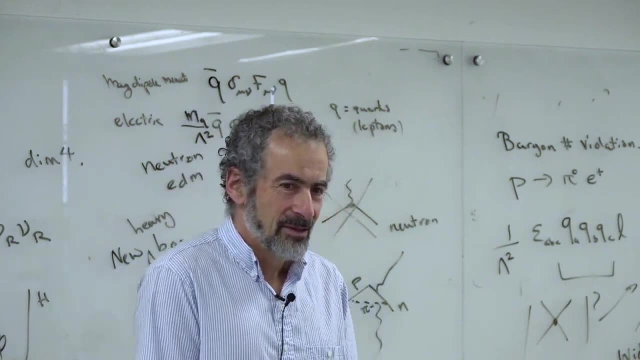 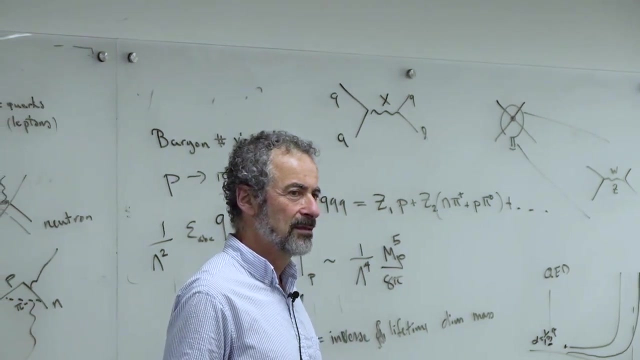 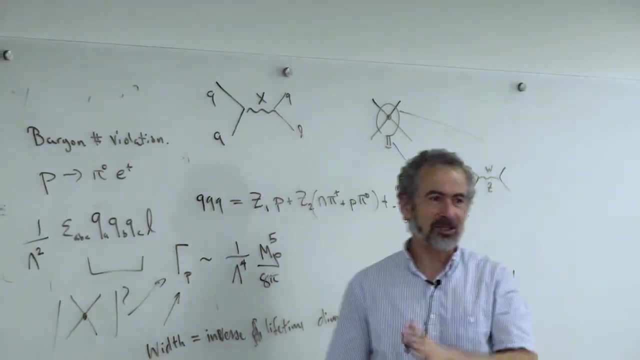 Sorry. Good So that even if it's not renormalizable at low energy, it is renormalizable. it is some approximation of renormalizable, Yes. So in the grain unifying theory, where this is due to an exposon, this is now an asymptotically. 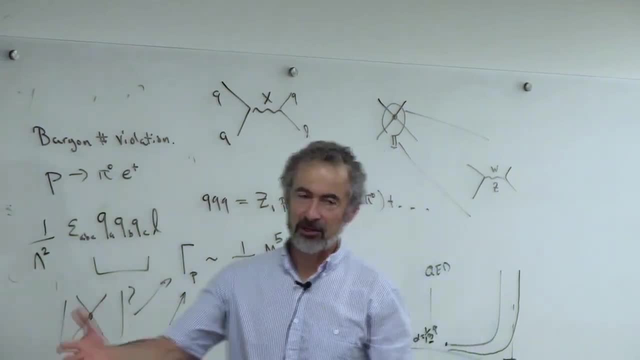 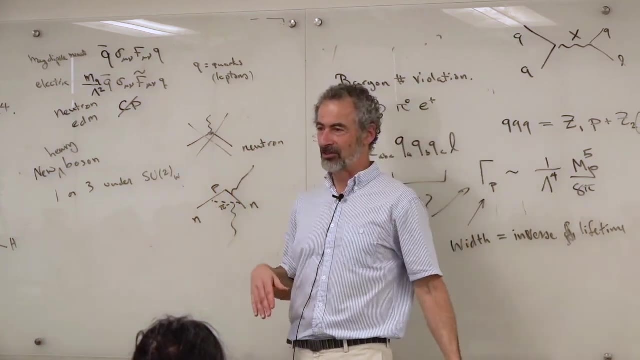 free renormalizable theory, Just like the Fermi interaction is not renormalizable. but it doesn't matter because you're going to take it up to the scale lambda and then you can start going to the theory with gauge bosons and then it becomes renormalizable. 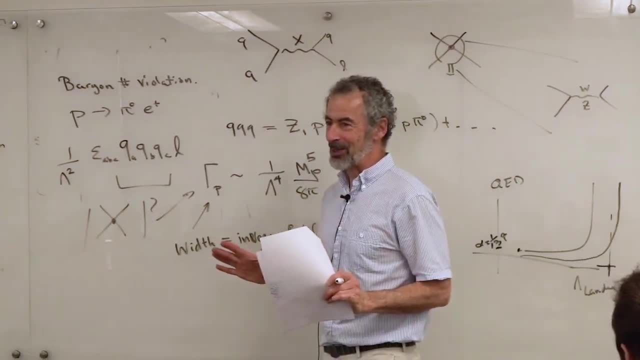 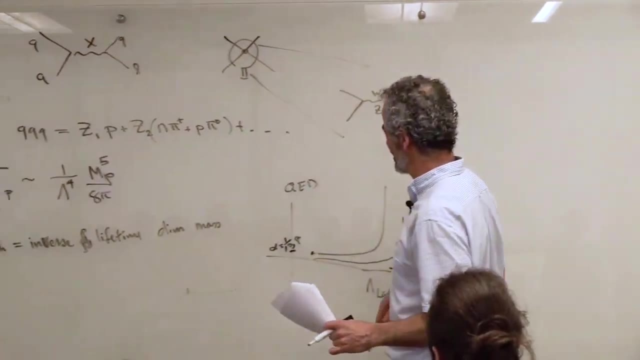 So don't get too happy, because we still have quantum gravity. We don't know how to renormalize that, okay. So there's still a lot of mystery. what's happening up there? Anyway, Georgiou came home and then he saw this diagram and said: oh no, the proton decays. 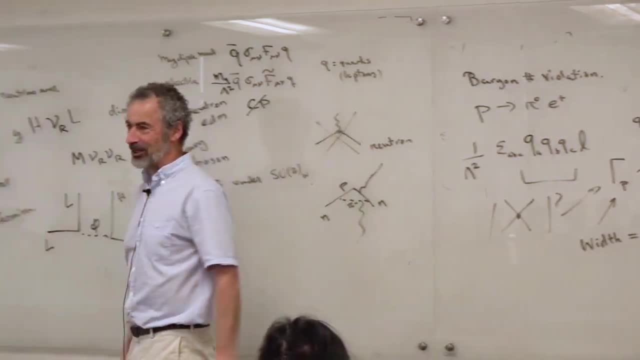 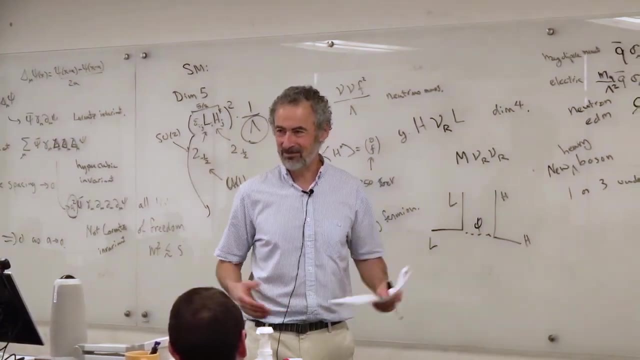 and he felt miserable because it's such a beautiful theory and now he'd have to throw it out. So he had a glass of scotch And that loosened up his inhibitions and he said, ah, let's make it really heavy. 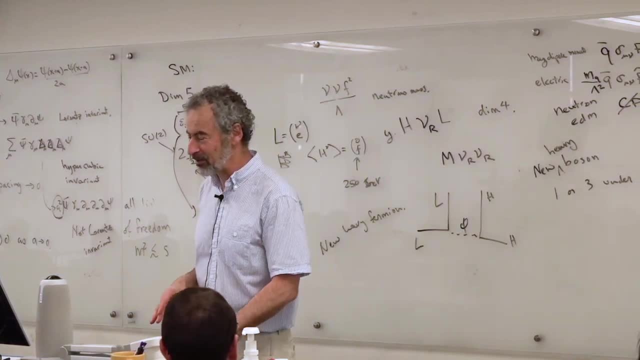 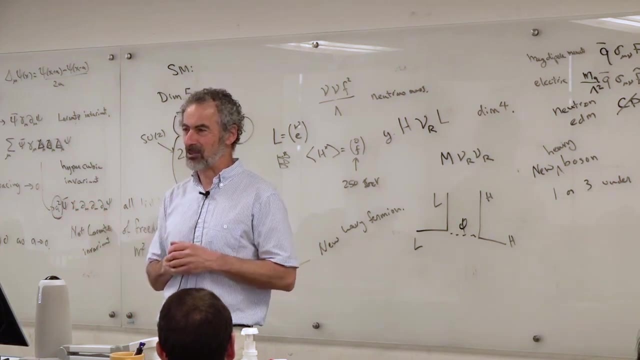 Now you have to understand that. so when I was a grad student, I remember seeing papers that said maybe there's a top quark and maybe it could be 10 GeV, which is why we haven't seen it, And that was considered ridiculously high energy. 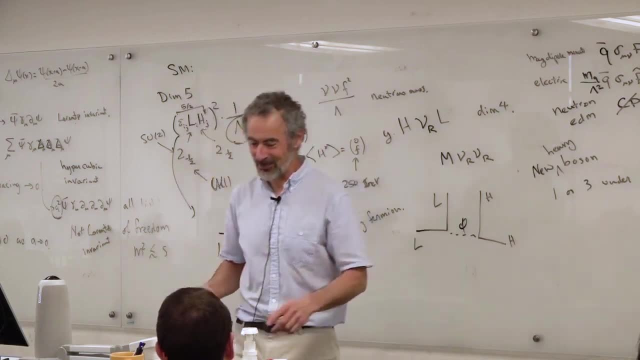 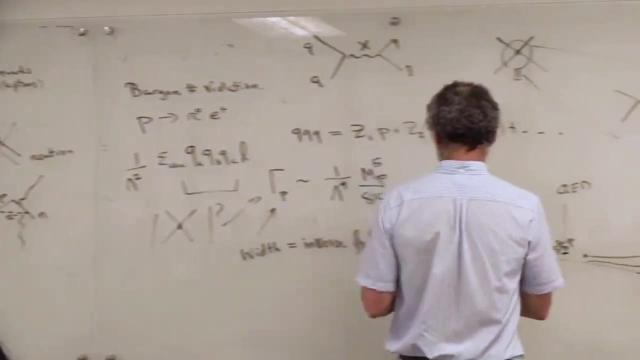 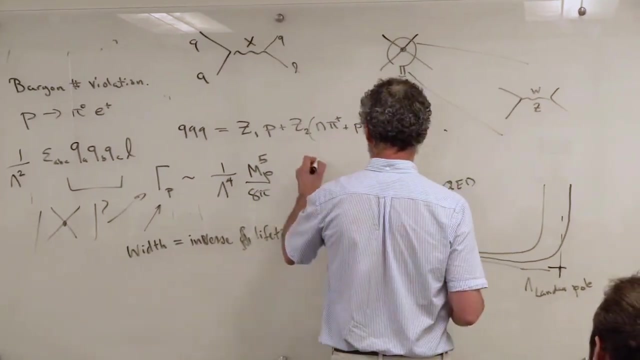 That was so, so daring to say that there's a particle at 10 GeV, But what's the mass of the X to make this viable For a lifetime of a proton, lifetime bigger than 10? to the 34 years which is, I think? 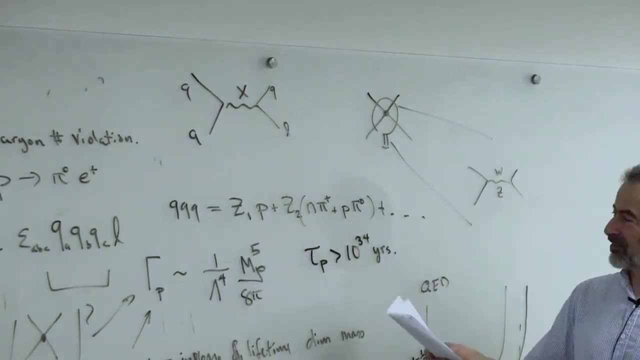 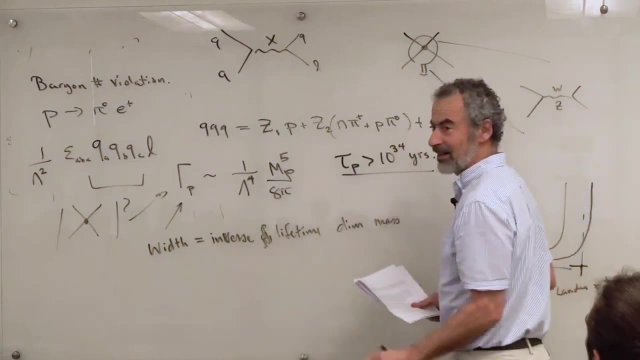 current experimental balance, at least for some decay widths are up to 10 to 35 or so. If you say that this is the experimental requirement and you use something like that, you find that lambda has to be bigger than or in the order of 10 to the 15 GeV. 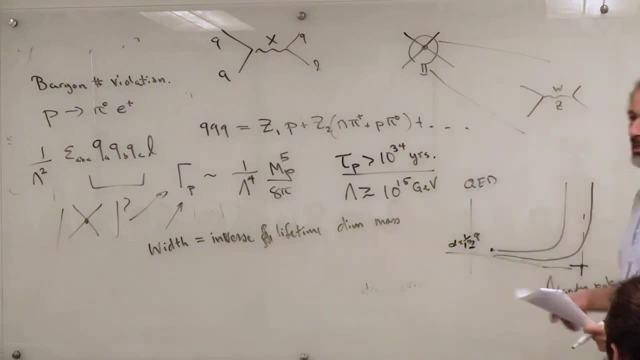 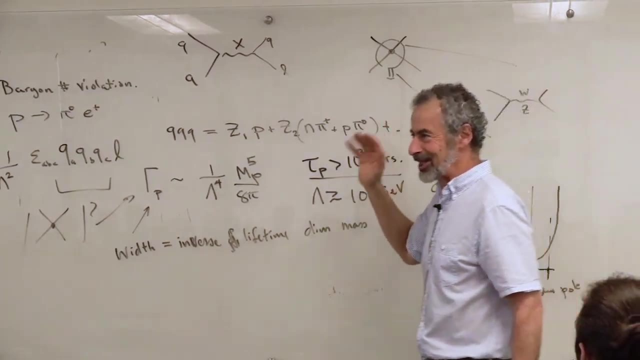 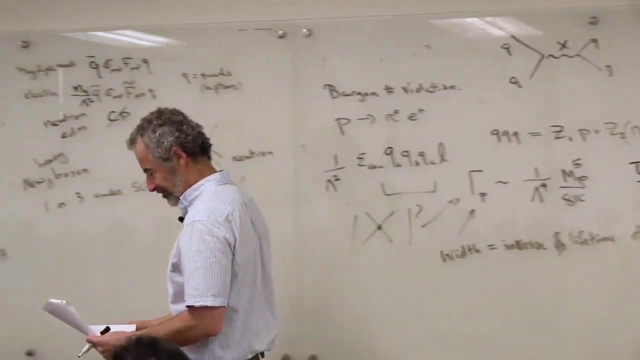 A ridiculously high scale, sort of tantalizingly close to the Planck scale, which is 10 to the 19.. But so he said, OK, we'll just make it super, super heavy, OK, And then we'll tell the experimentalists to go look for it, to look for proton decay. 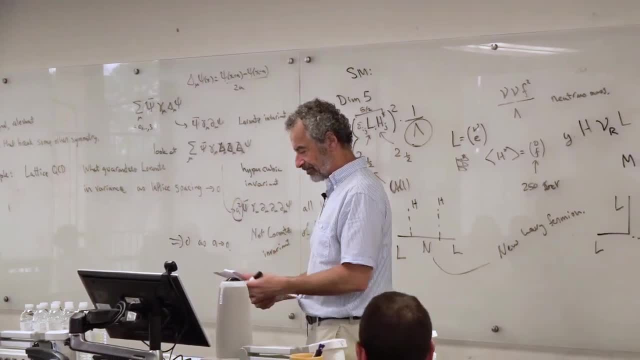 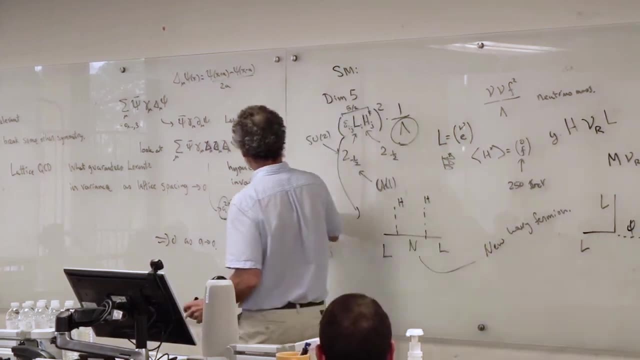 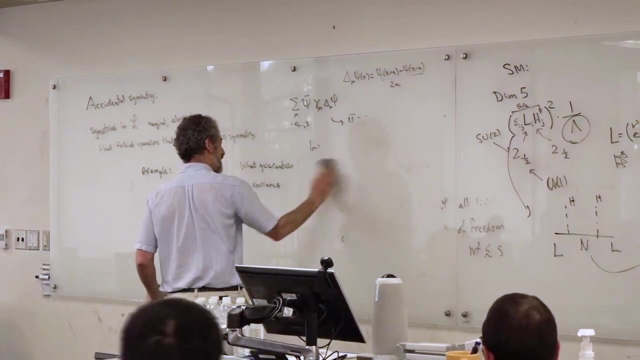 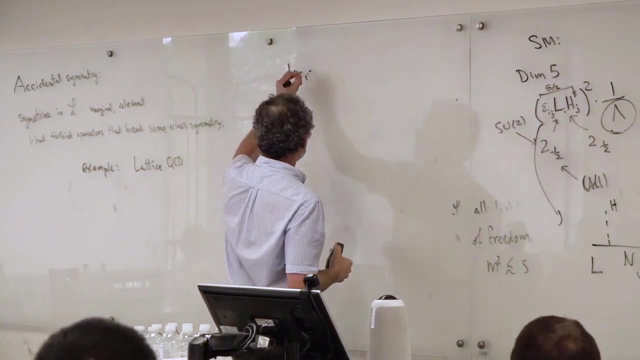 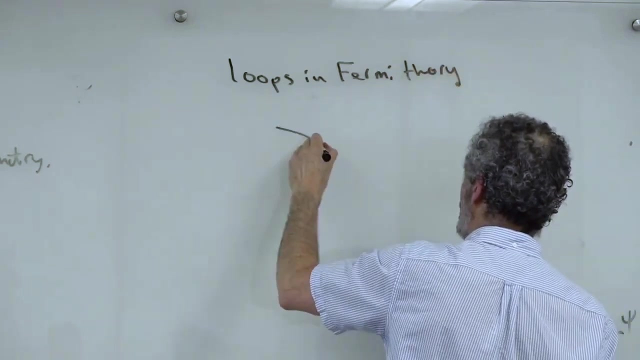 Yeah, I want to return to one thing that was sparked a bit by air, A question, I think, about how the effective theory turns into the high energy theory. So let me just go back to loops in the Fermi theory And let's look at this correction again here, which this goes: like G Fermi squared. 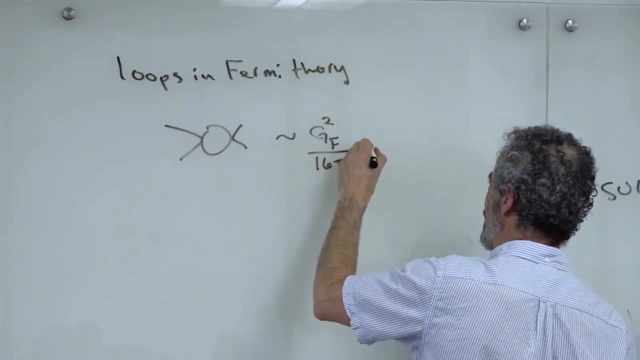 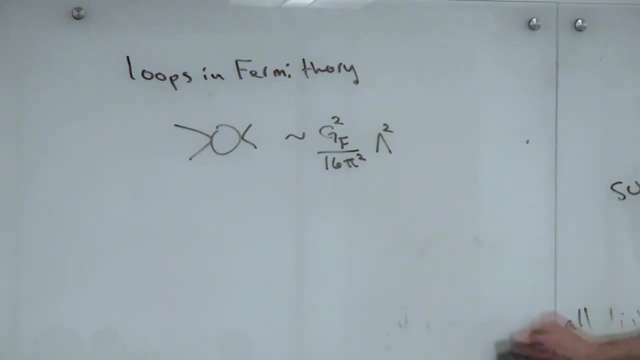 And then it's a loop, so typically a 16 pi squared. And then we said there had to be a lambda squared. Sorry, you can't see the answer. Sorry about that because of the pillar. OK, well, let's remember G Fermi. we know from the standard model is really something. 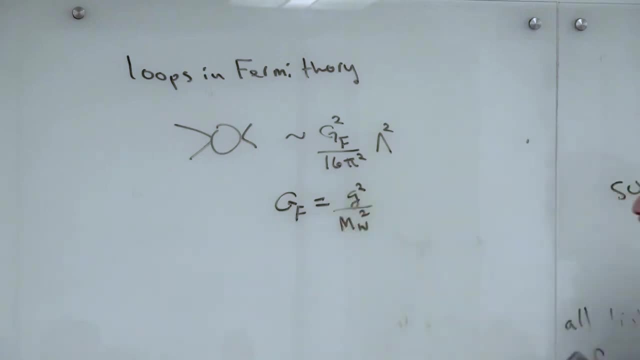 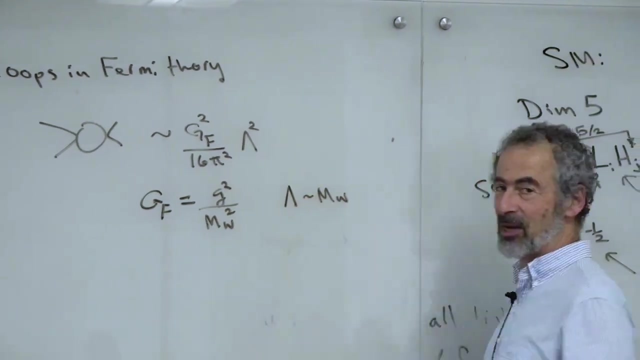 like G squared over, Mw squared or Mz squared, And I tell you that lambda has to be on the order of Mw. I can't take my cutoff higher than Mw because I'm not putting the W in my theory. 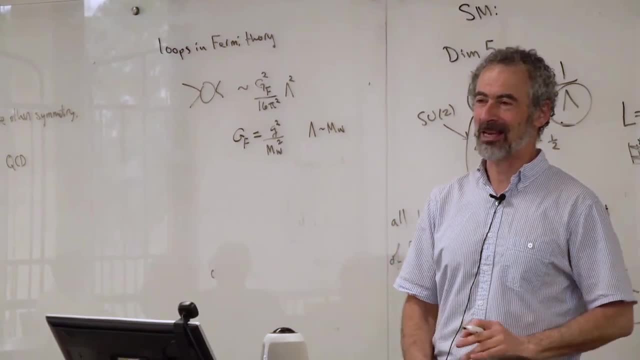 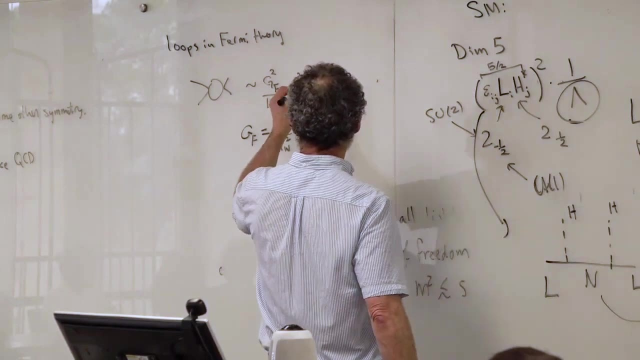 Remember the rule was you have to include all the particles lighter than lambda in your theory, And I'm not putting the W in, So this is the highest lambda could be. If I look at the correction then this goes like G to the fourth. 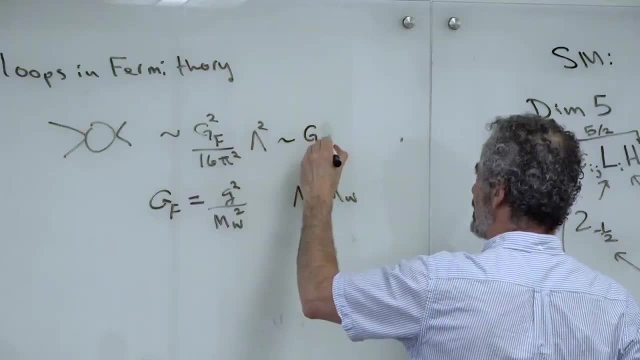 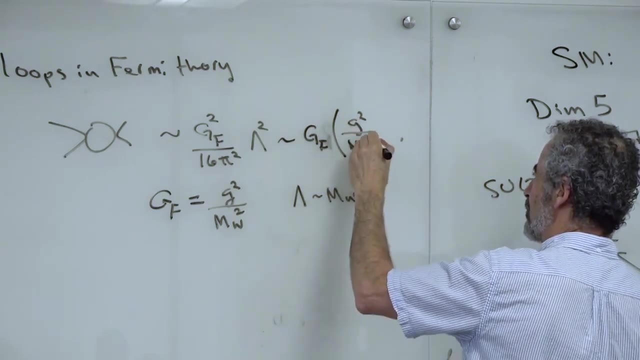 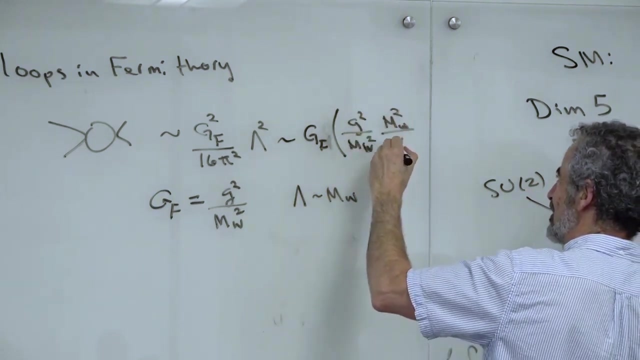 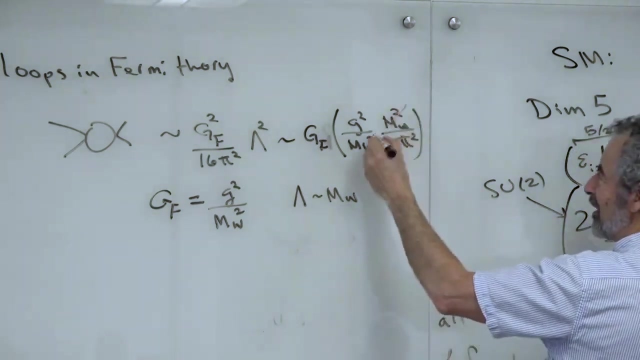 Well, let me pull out one factor, G Fermi, which is the tree level result. And then it's times G squared over Mw squared from the other G Fermi, and then an Mw squared over Mz squared, Say 16 pi squared from the loop, Mw's cancel. 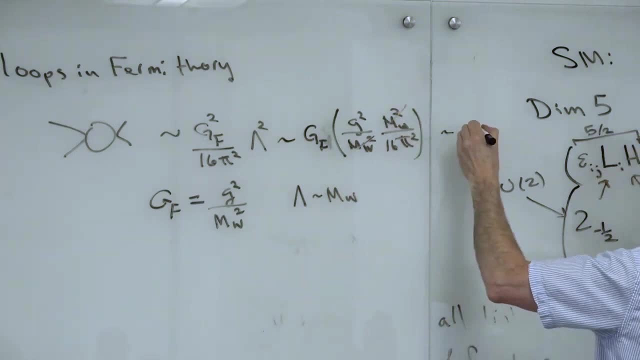 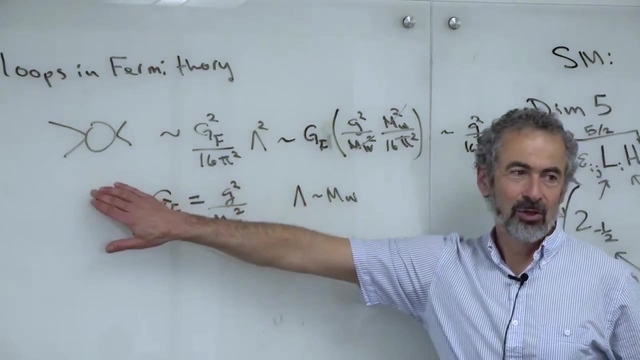 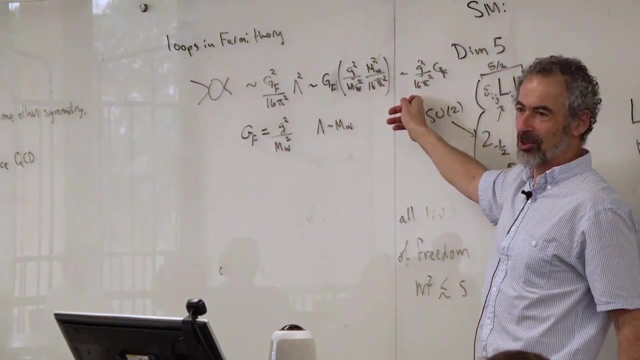 And you see that this is something that goes like G squared over 16, pi squared G- Fermi, And so, in fact, this is a correction which is big or small compared to the tree level one, depending on whether the high energy theory is perturbative or not. 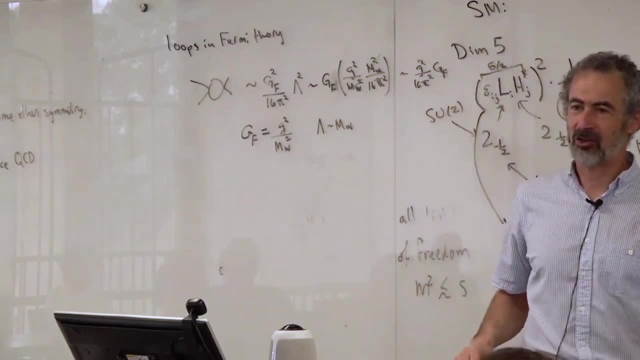 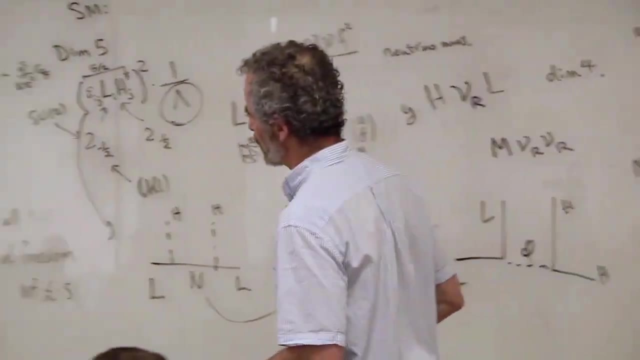 And so it moves smoothly into the perturbation equation. OK, So you have the momentum expansion of the high energy theory if the high energy theory is weakly coupled, So you sort of have two expansions going on at the same time in your effective theory. 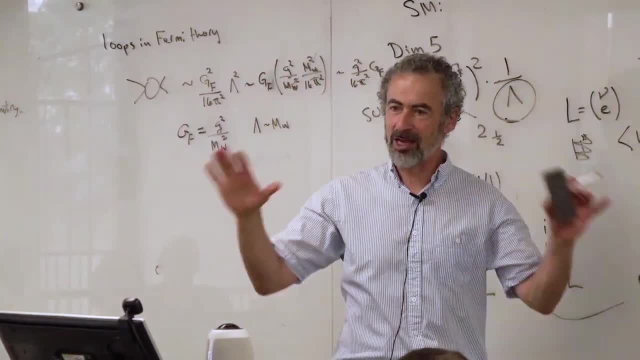 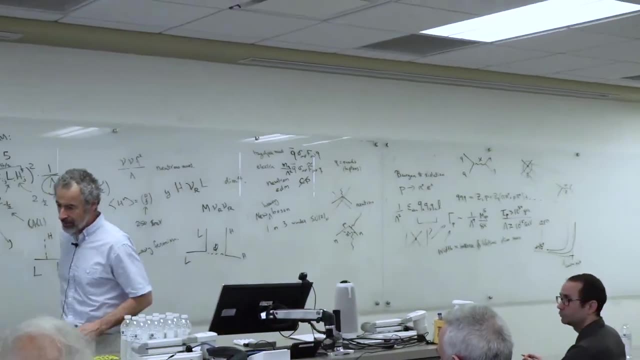 You've got the momentum expansion, but you also have the underlying perturbative expansion of the short distance physics. OK, I'm out of time, So I'll continue next time. No, you can. I'll answer questions, but I won't continue with my lecture. 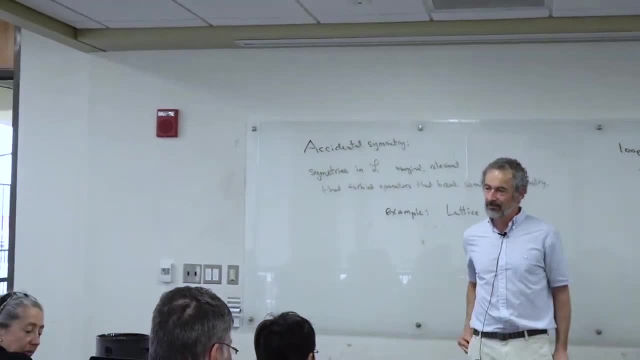 So then we were just talking about this. Does that imply that if we had a short distance physics, we would have a perturbative expansion of the short distance physics? Yes, OK, So you're saying that if we had some type of strong coupling with whatever interaction? we're trying to model that we would lose any silence of, say, renormalizability. We'd lose part of the expansion. We'd lose the perturbative expansion. We'd still have the fact that higher derivatives give you smaller and smaller answers at low. 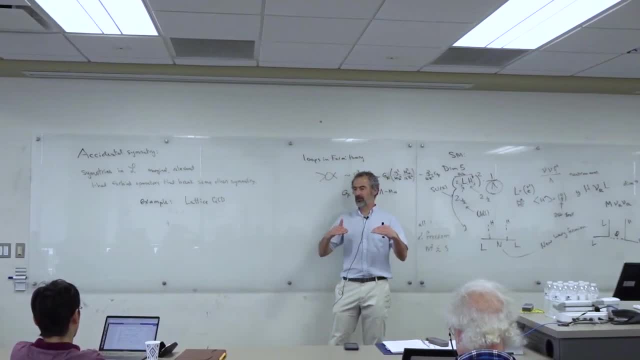 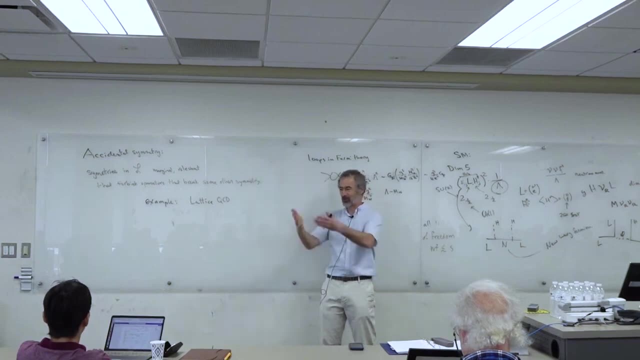 energy. But when the theory goes to higher energy, everything would break down, because now all the higher dimension operators are just suppressed by powers of g squared over 16 pi squared, which you told me is order 1.. Yeah, And an example of such a theory is chiral perturbation theory, where we look at the 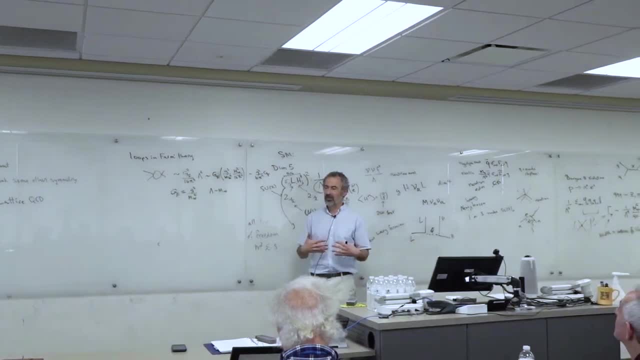 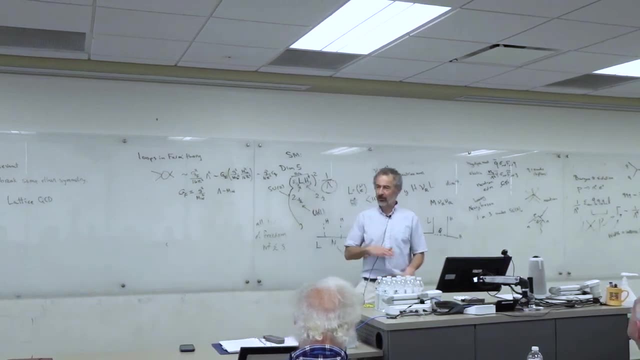 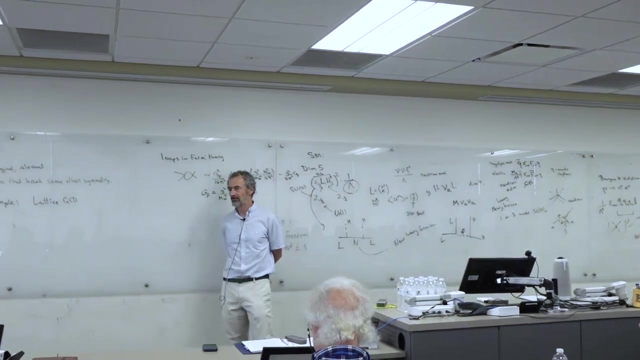 effective theory of mesons below the scale of QCD where when you get to the cutoff it's a strongly coupled theory. So we still have the derivative expansion, but it really breaks down when we go up to higher energy. So I guess, was it still like, useful or effective in predicting some level of phenomenology? 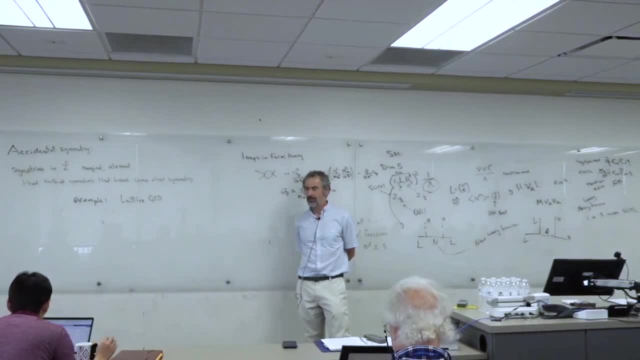 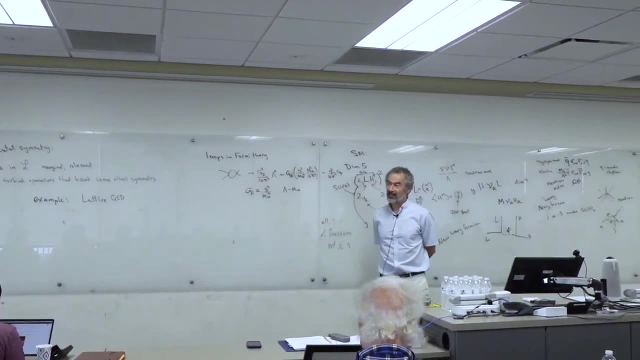 even though it breaks down. when we get like the whole expansion seems to break down, Right. Well, the expansion breaks down in a funny way. It's that it looks like operators renormalize each other and therefore in a way that you 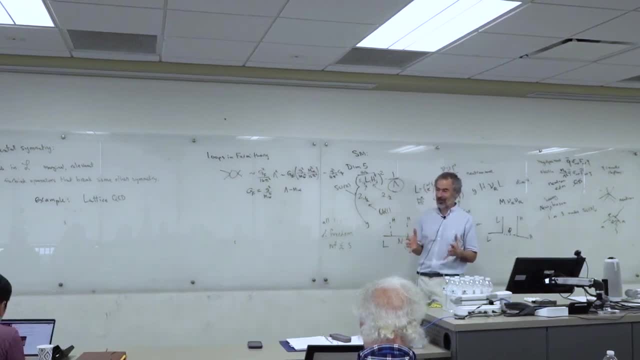 can't control. But it turns out that this is where dimensional regularization comes in. that dimensional regularization ensures that operators only renormalize higher dimension operators. So if I say I'm only interested in the first four operators For operators in my expansion, I'm not interested in the higher dimension operators, I don't. 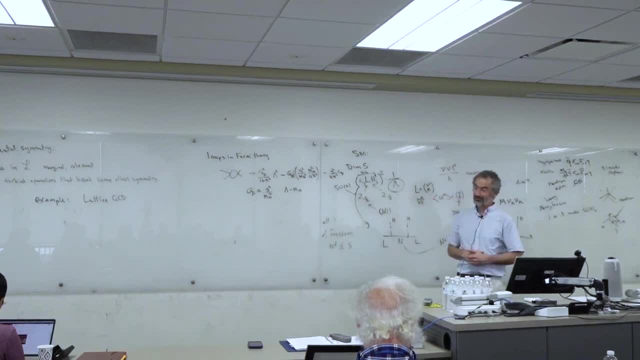 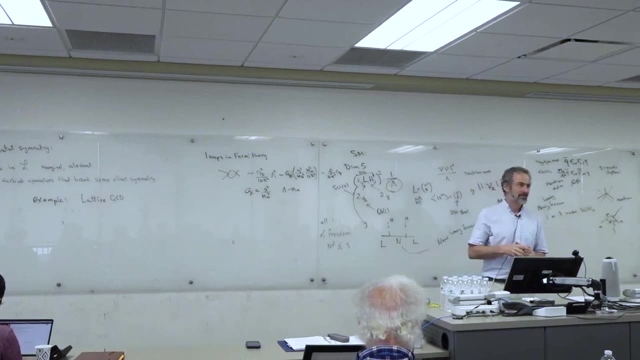 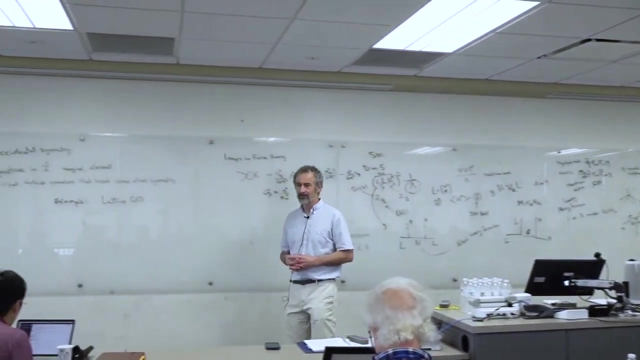 have to worry about those things. I'm excluding renormalizing the ones I'm studying, So that's a technical thing. but that was a contribution from Weinberg that was useful. Other questions: Yeah, So I have a question about the land of all QEDs. 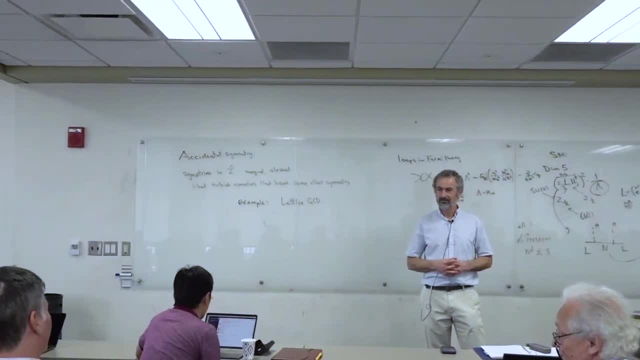 So you said that its existence would imply that the coupling in the IR is essentially zero, But strictly speaking, I would assume that it's not. I assume that there must be some mathematical problems. It just means that the extrapolation from the UV to IR is not stable, and you can get. 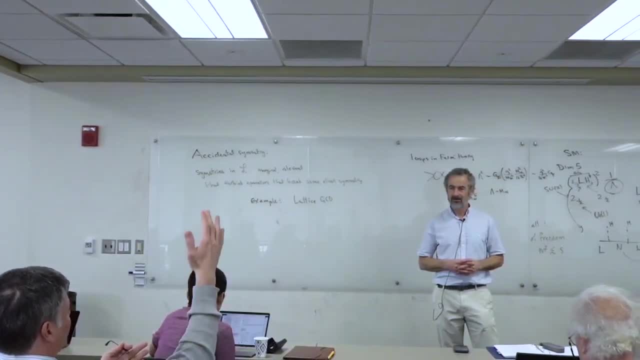 whatever you like, Or is it not true? No, I don't think so, Because the thing is, it's not just that it gets bigger and bigger in the UV, It becomes infinite at a finite scale in the UV. And so if you just try to imagine, like Wilson, how would I put that on a computer? okay, and 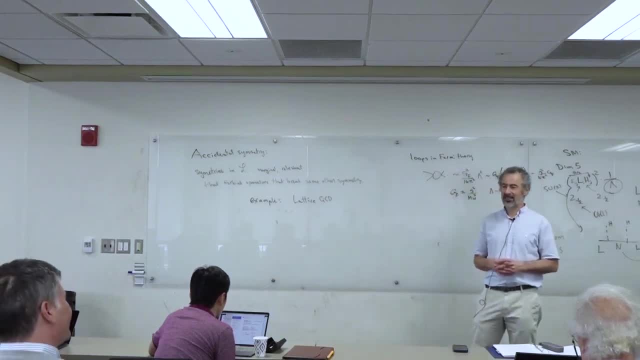 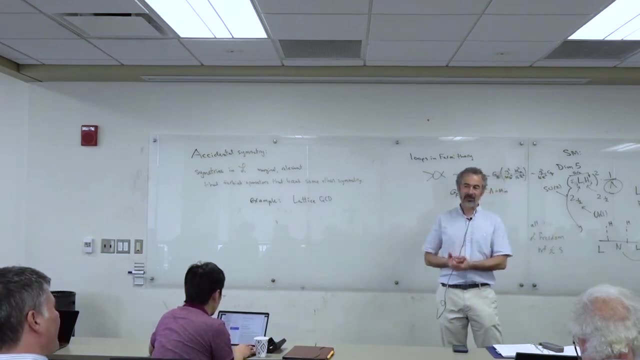 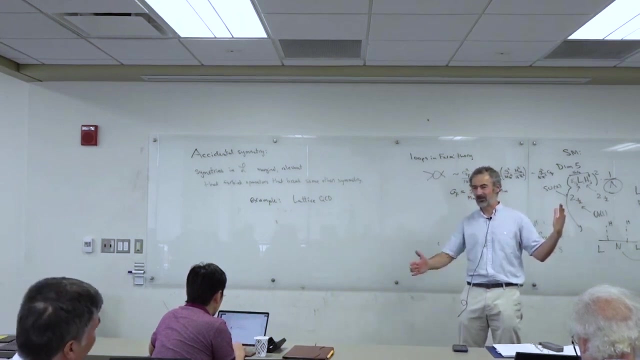 I want to take the lattice space smaller than the Landau scale. I can't put in a coupling that's bigger than infinity. If I put even infinity at a scale that's much higher than the Landau scale, I get zero at long distance. 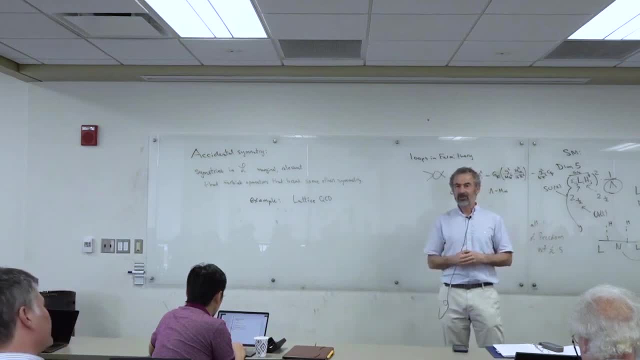 Or another way of saying it is that if you wanted to look at the interaction between charges, say static charges in QED at arbitrary long distance, you'll find that there's no interaction at all. It doesn't fall off like 1 over r. 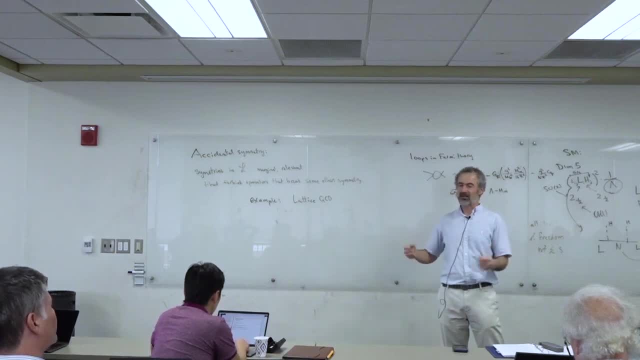 It falls off faster than 1 over r at long distance And we understand that perfectly well due to screening The E plus, E minus pairs in the vacuum screen, this charge, so that actually when you're far apart you don't see the same charge. 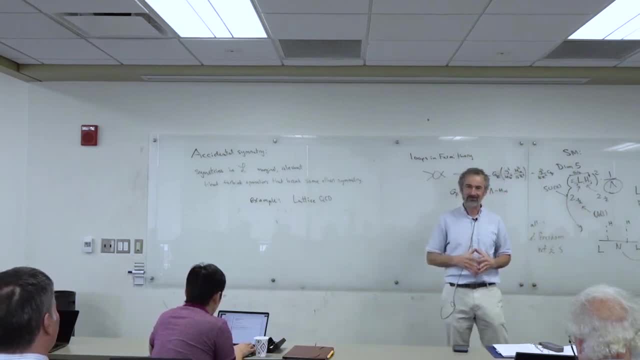 So that's what's going on. It's just screening. But screening means that you can't take away the cutoff and have a theory that has interactions, because our scale- whatever scale we're doing the experiment in- looks infinitely long compared to the cutoff. 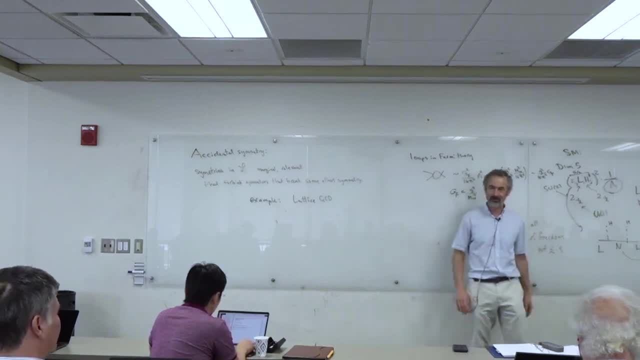 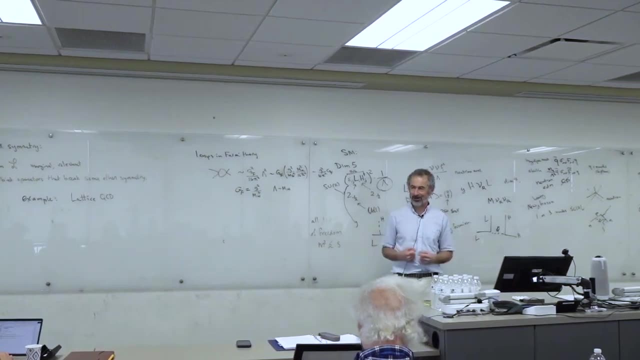 And so you always have an infinite amount of screening or total screening of your charges. What's weird about QCD is that there's anti-screening. The gluons make the color charge look bigger and bigger at longer distances. Maybe more questions for Davis. 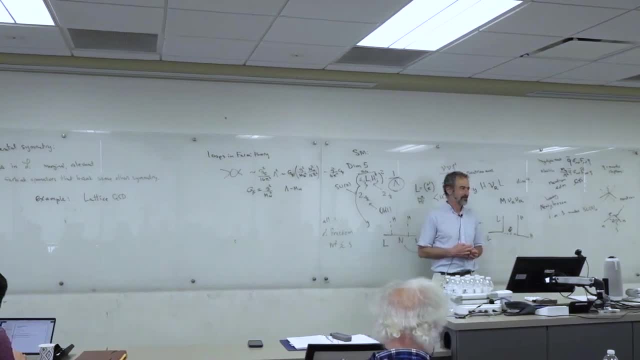 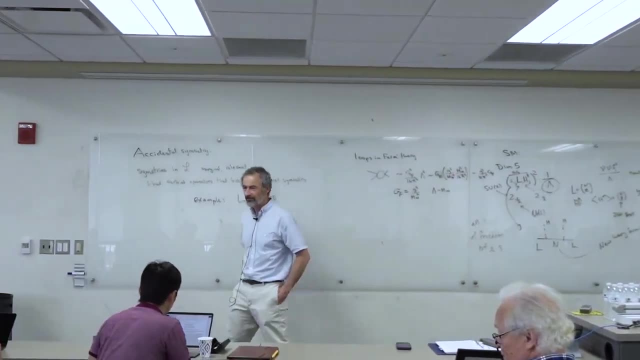 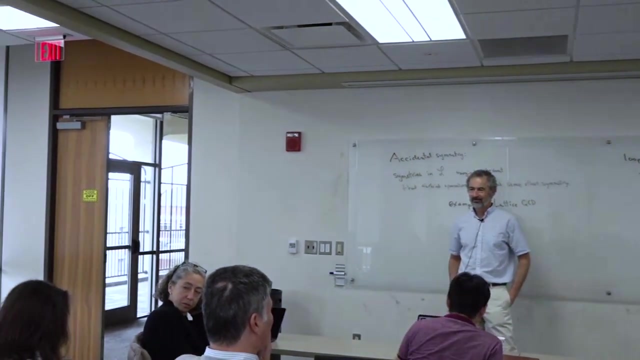 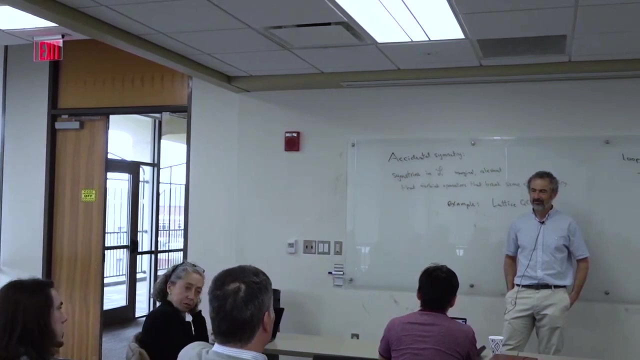 Hi, I have another. So going back to when you were talking about the old school, I guess thought versus Wilson's kind of understanding. When we're talking about theory, Wilson is essentially saying this is irrelevant because the IR corrections are irrelevant. 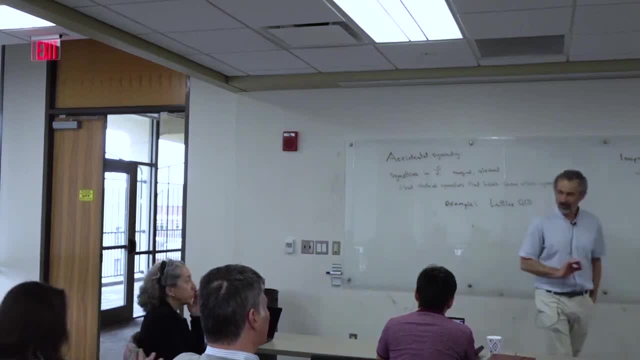 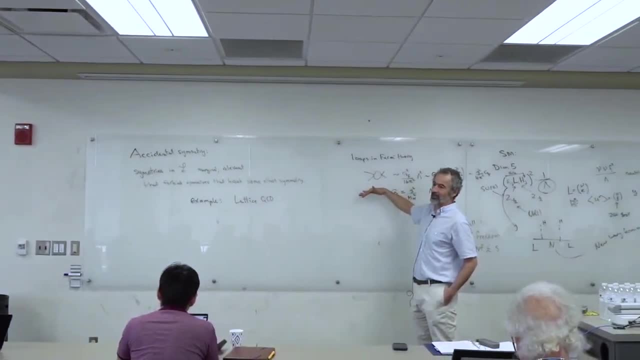 Right. So at low energy they're very small And through this argument here, if your underlying theory is perturbative, then it'll still be perturbative all the way up to the cutoff And you don't have to talk about physics above the cutoff. 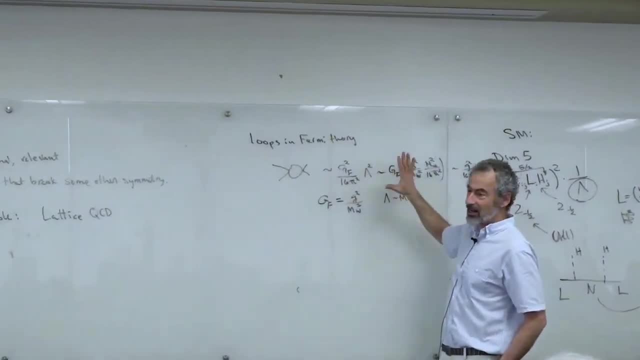 And if he wants to do QCD, he's willing to get rid of this. He's able to say: I'll set the coupling on the order of G, squared over 4 pi, squared on the order of 1, if you wanted, if you wanted to have a low cutoff. 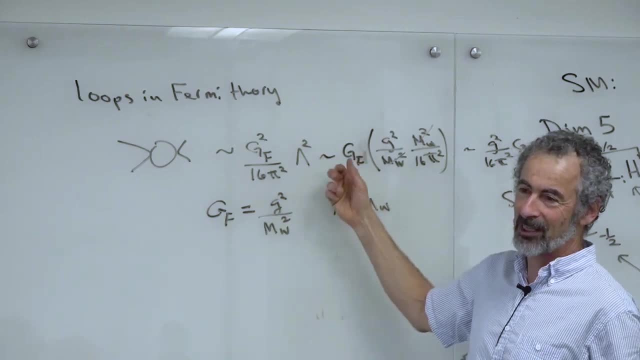 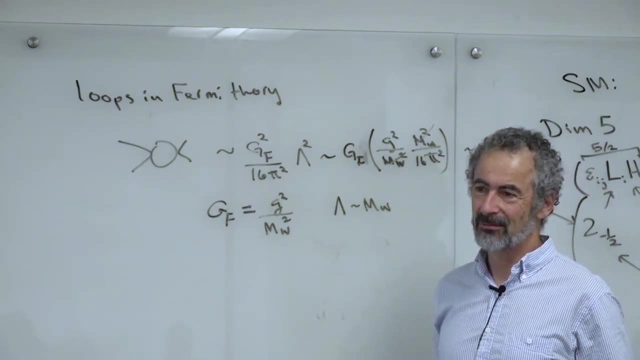 But the cool thing about QCD is I can go to a higher cutoff and G squared over 4. pi gets smaller and smaller because of asymptotic freedom. So he's literally saying that as far as like this effective field theory approach goes, there's not really like a relevance whether or not like the theory we're trying. 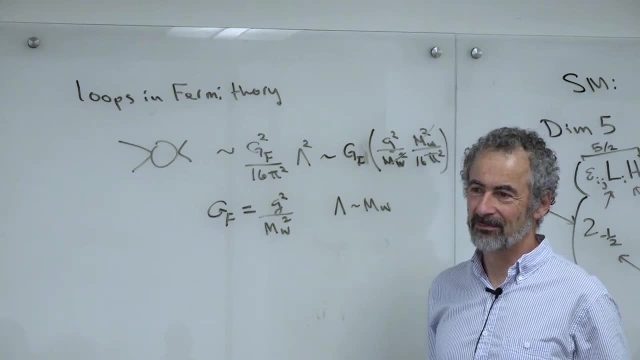 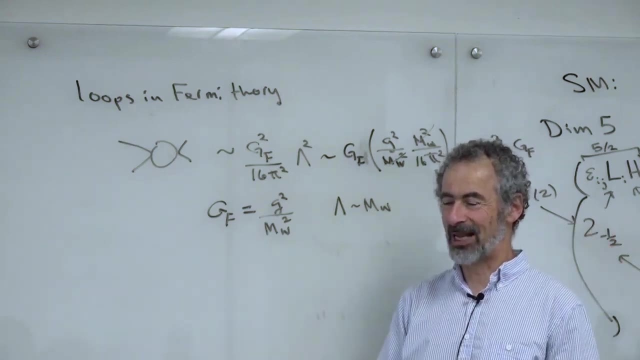 to model is, I guess, classically renormalized, Right, OK, As long as it. I mean, if you really want to be able to talk about overall scales, it would have to be asymptotically free. But we don't worry about that, because we think QED is probably embedded in a grand unified 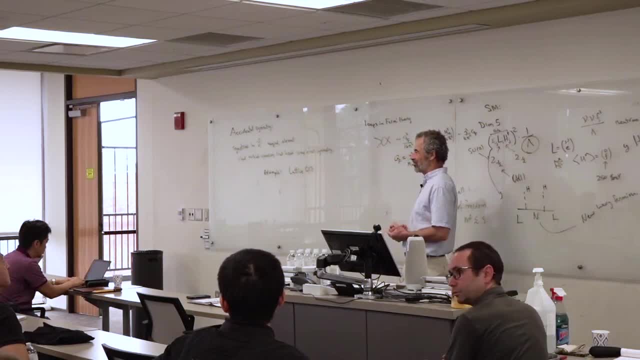 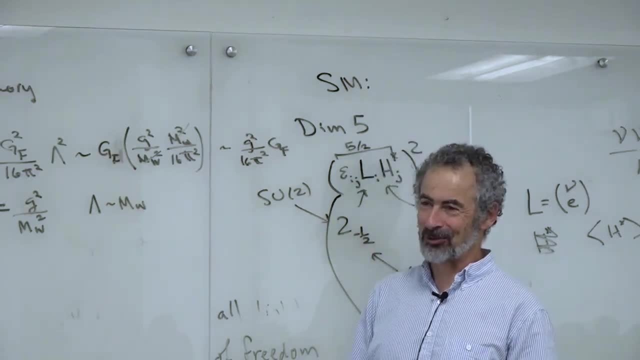 theory that is asymptotically free because it's a non-abillion gauge theory. So that happens well below the Landau pole And this is just an example, which is: you know, don't your, don't get your panties in a twist over stuff you don't see. experimentally. 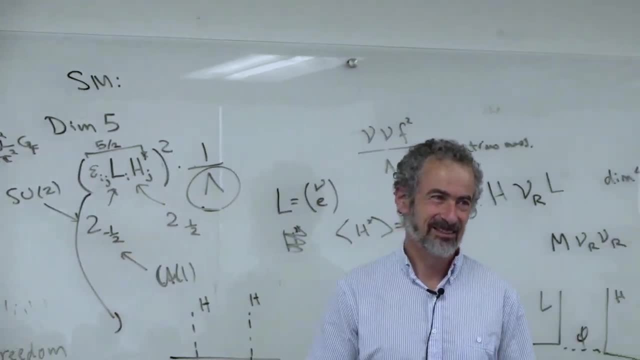 OK, OK, Yeah, Mark, Since you mentioned the Landau pole, at what energy is that expected? Because I assume, when you look at the coupling constants and you talk about the grand unified theory, do you want to bring that up. No, 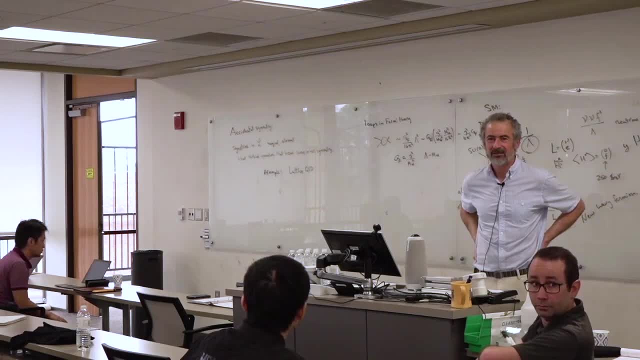 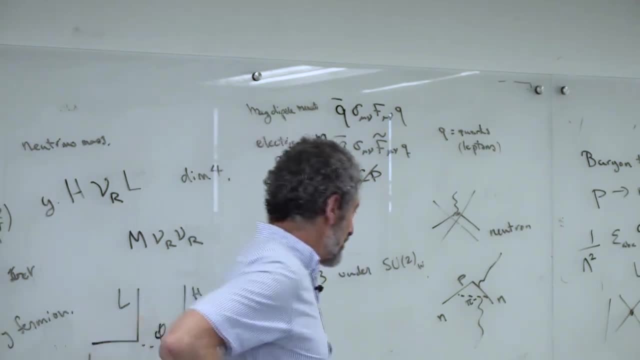 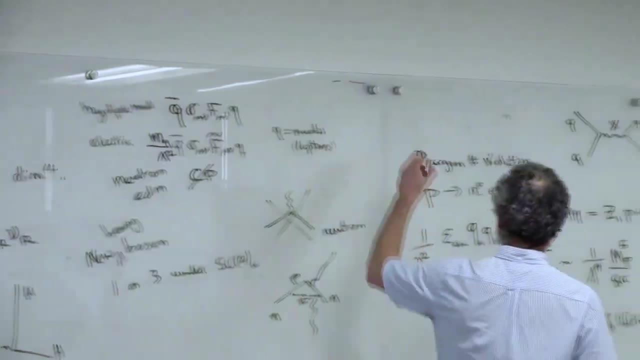 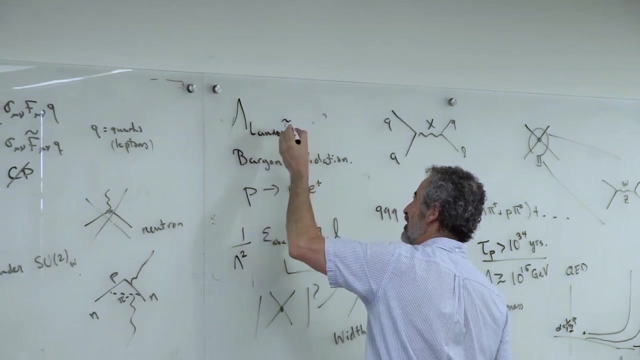 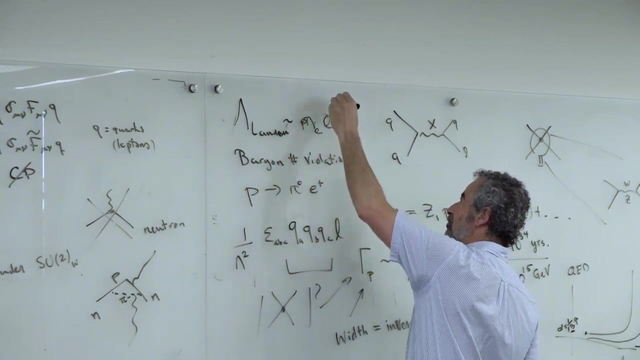 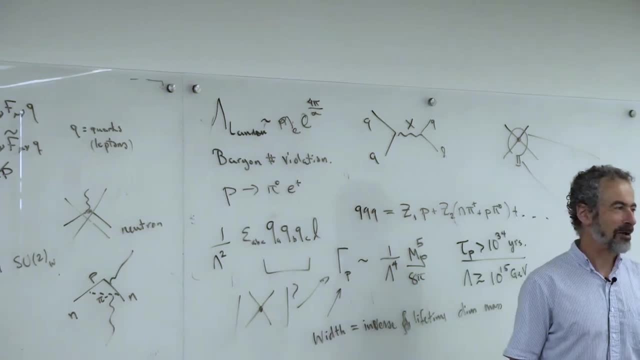 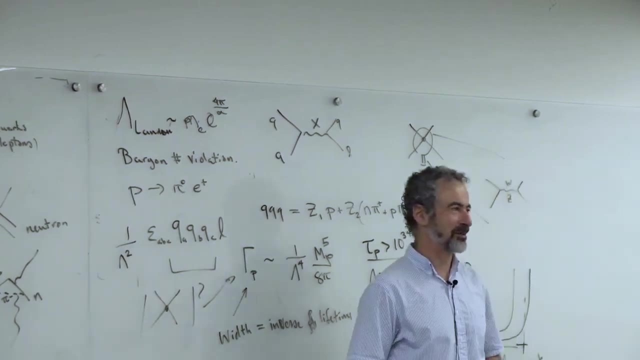 Four pi over alpha is a thousand. So you're talking about ten to the one, e to the one, thousand times the electron mass, times the electron mass. So it's way above the Planck scale, which is 10 to the 19. 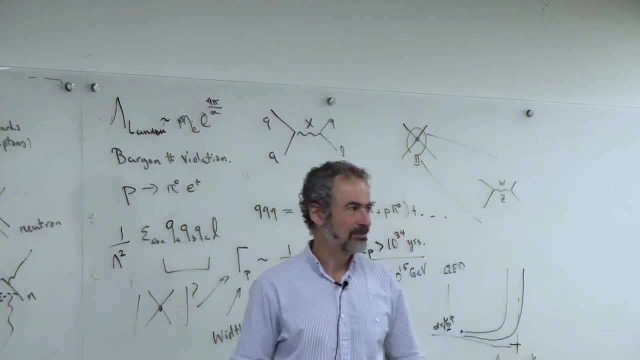 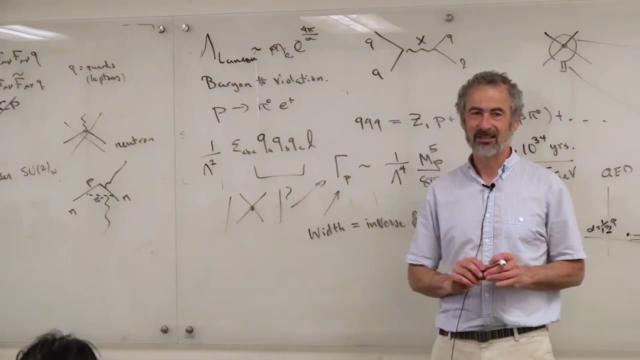 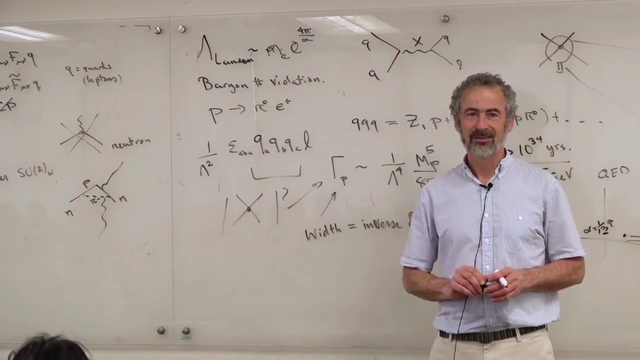 jiv. So it doesn't have any real realization Because every time the ECD coupling constant right where it basically blows up. that's the regime of nuclei and neurons that you talked about, But the Landau-Pole doesn't have anything where you'd say. 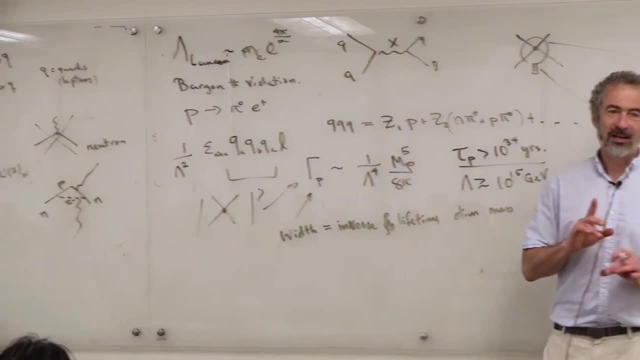 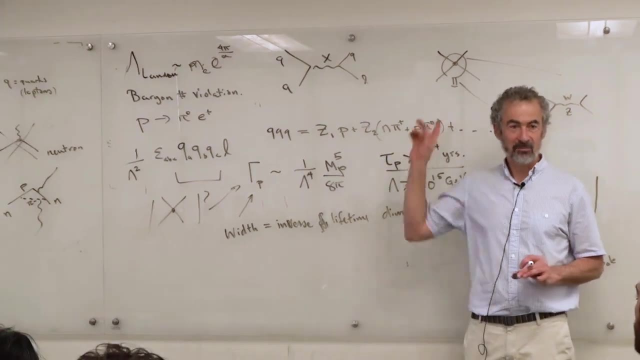 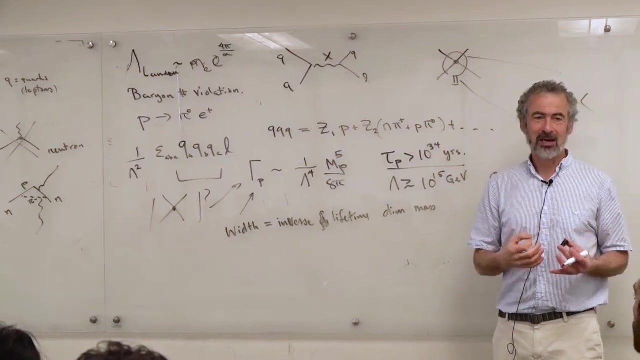 this is what happens. There is an example of a theory that could have been where it would have been important, which is that in the standard model, the 5 fourth coupling of the Higgs behaves like this If the 5 fourth coupling was large at the W scale. 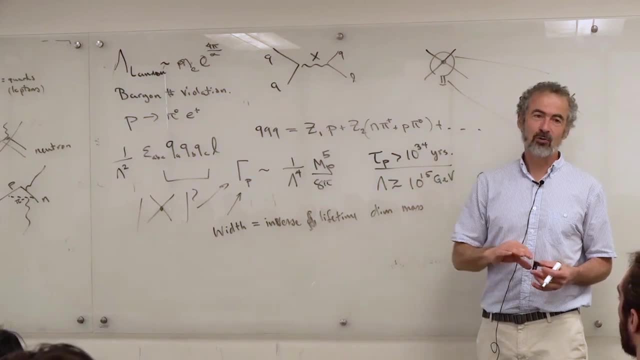 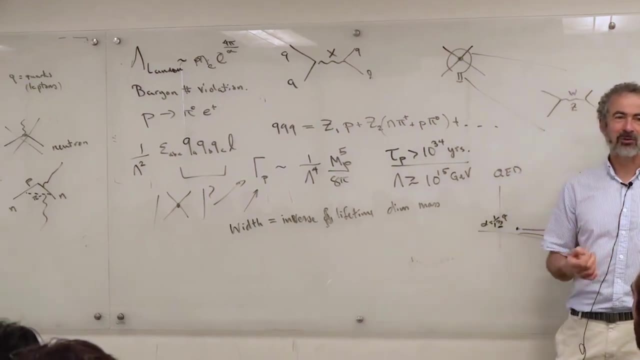 which means the Higgs was heavy. it would get strong very quickly. It would be strong at a TeV. So it was known that if the Higgs turned out to be heavy there would have to be new physics coming in relatively close to the W mass. You wouldn't have to go up very far. As it is, the Higgs is light enough so that you don't run into problems until you get up to the gut scale. But again, the gut scale up here is the place where you better fix the Higgs mass.